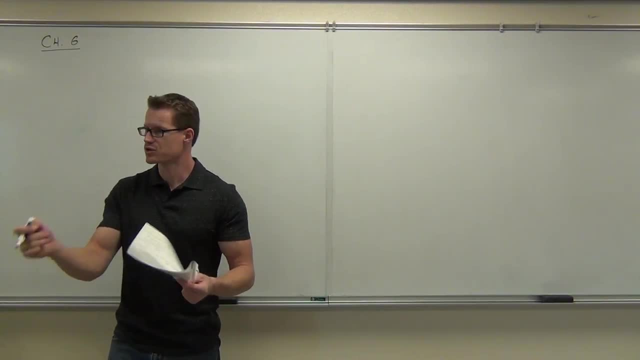 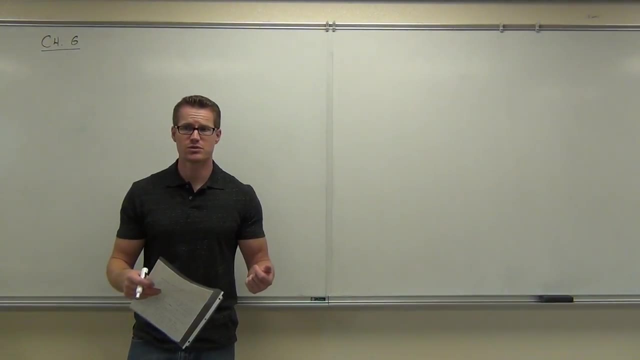 as what your measuring tool allows. So it's not like you can count measurements. They're not in any particular order. What's the next number after 3.01? You go, well, I don't know, It's not 3.02.. You can do 3.010001.. That's in between there somewhere and you can't count. 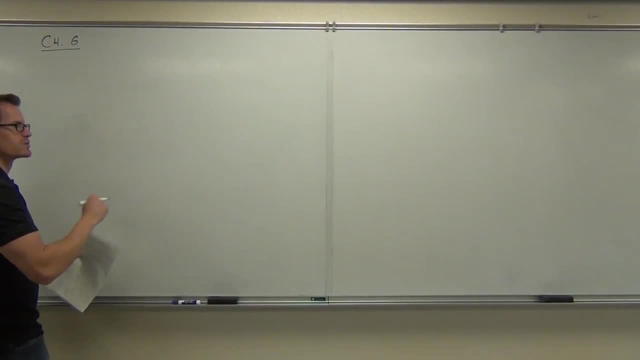 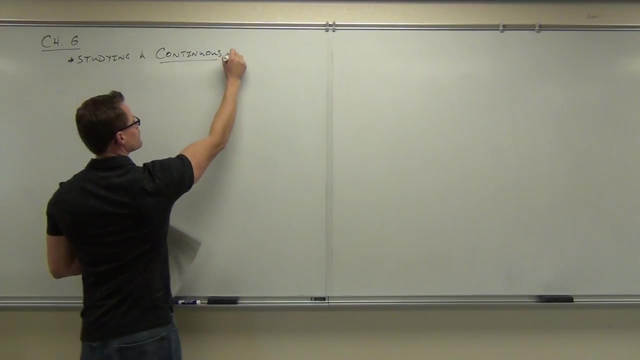 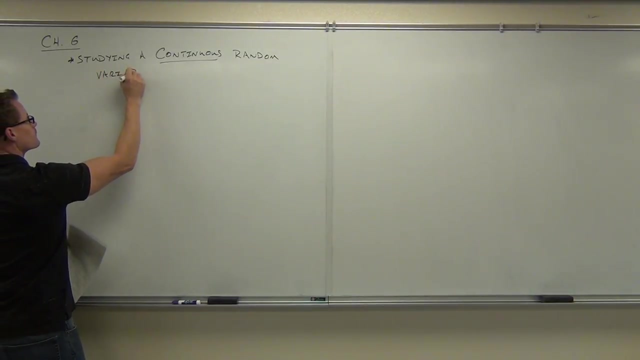 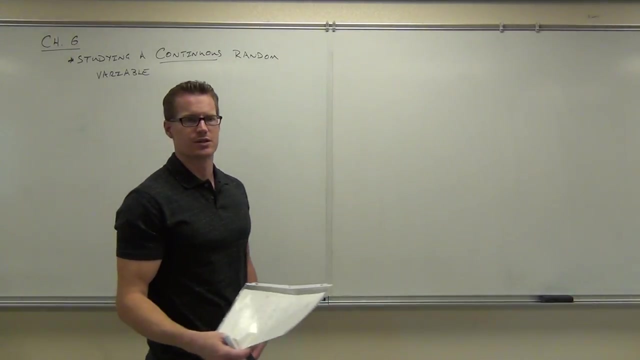 that. So that's what we're studying here is a continuous random variable. So that's what we're studying here is a continuous random variable. So that's what we're studying here is a continuous random variable. Firstly, before we actually get on to continuous random variables, I've got to tell you that. 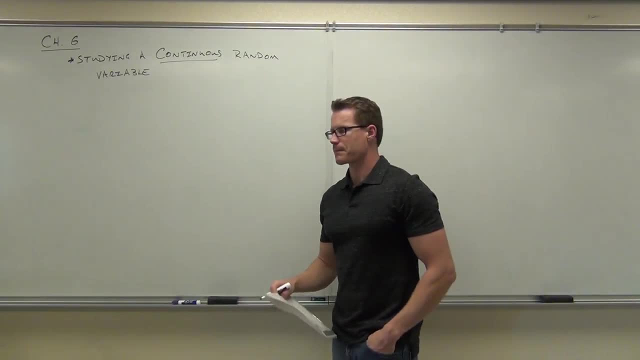 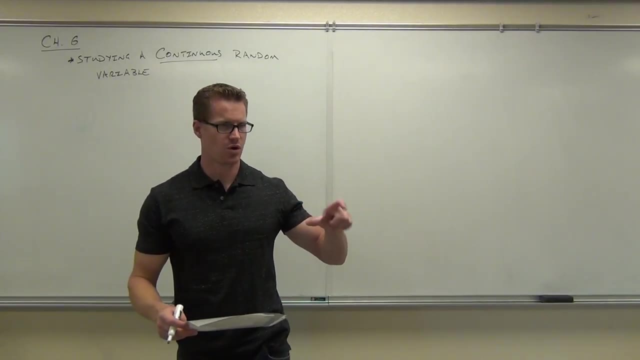 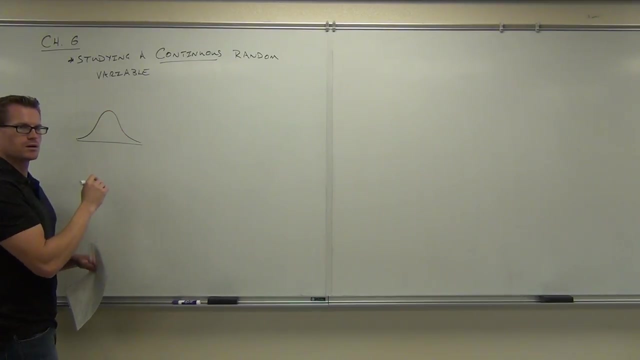 if the continuous random variable has a symmetric bell-shaped curve. do you remember what the symmetric bell-shaped curve was called when we had something like this: Normal distribution. Say it again: Normal distribution, Normal distribution Called it normal. That's exactly right. So if we have a normal distribution or a bell-shaped, 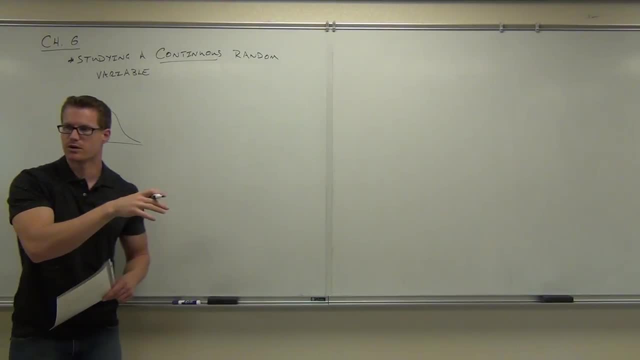 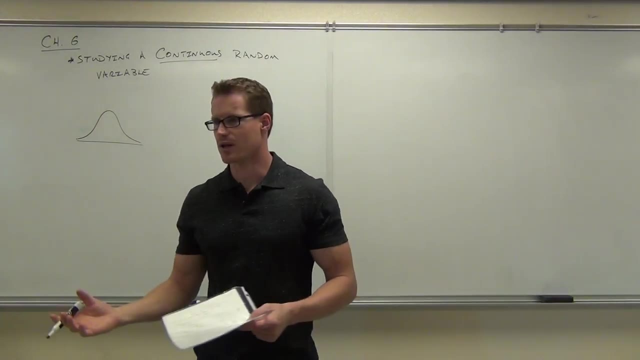 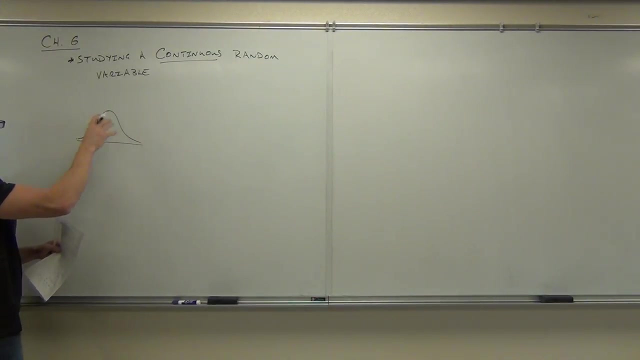 curve. that's really what we're looking for in our chapter six- is something that's going to be normally distributed. If we don't have a normal distribution, none of this stuff really applies. So what we need out of this section, out of this chapter, is for our continuous random variable to have a symmetric, bell-shaped curve, otherwise known as a normal distribution. 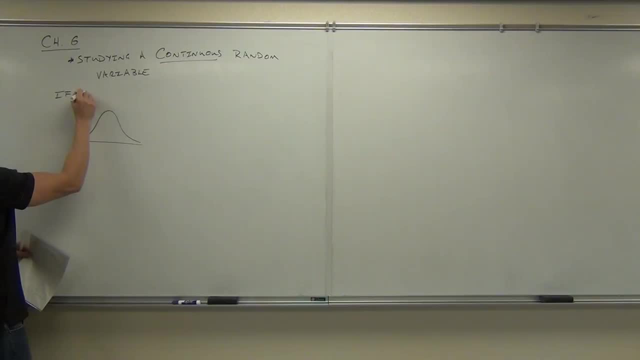 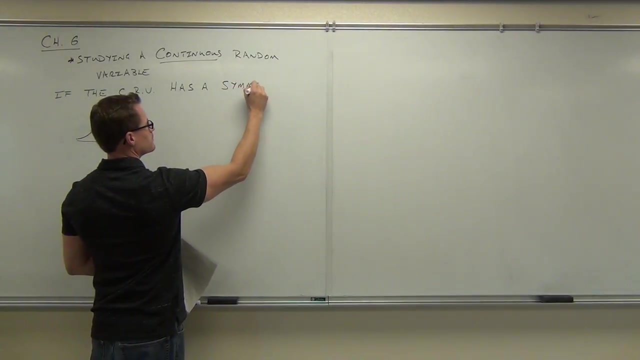 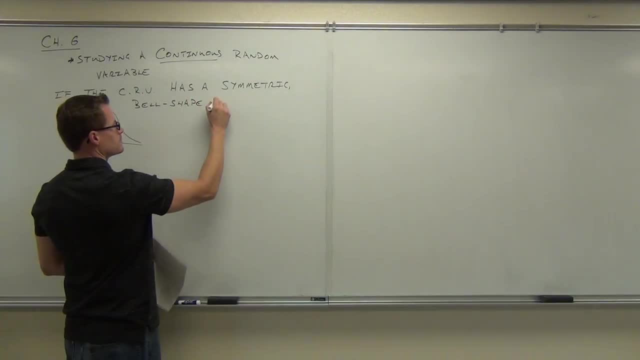 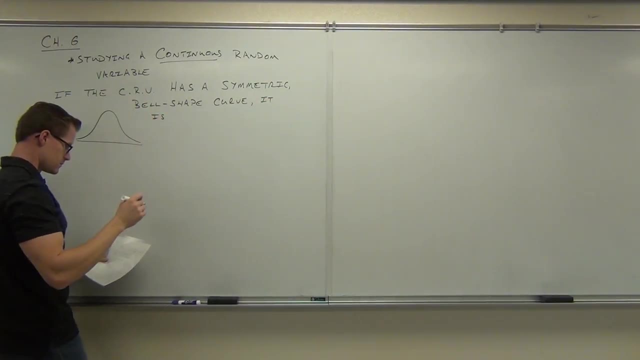 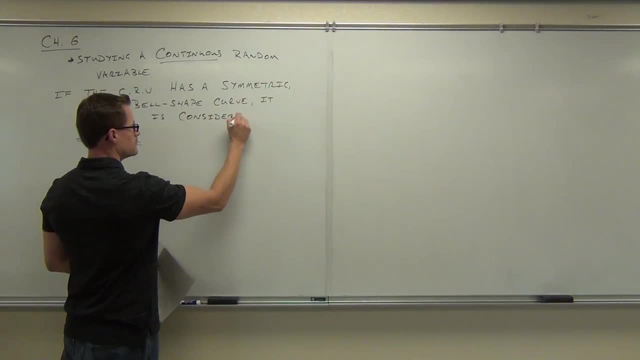 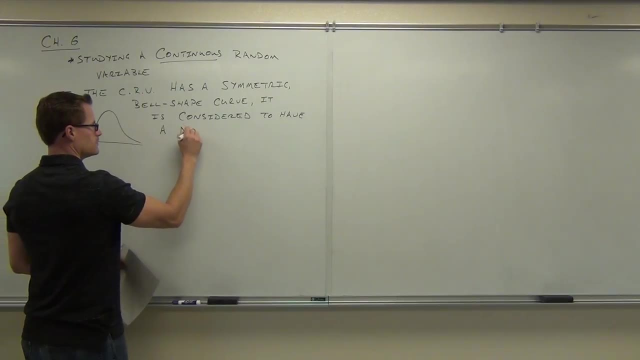 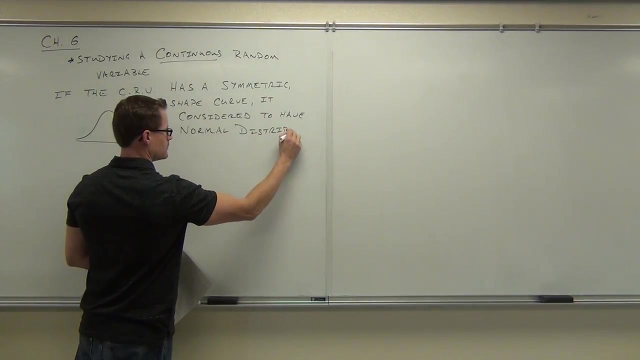 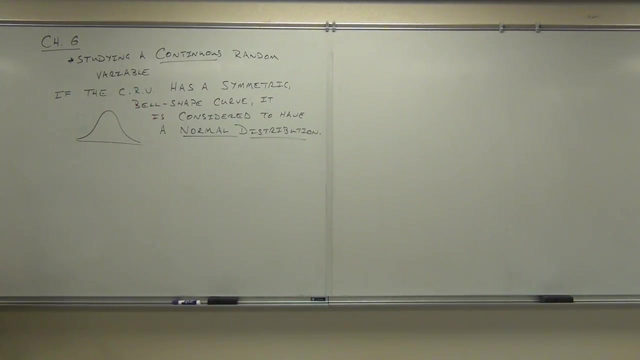 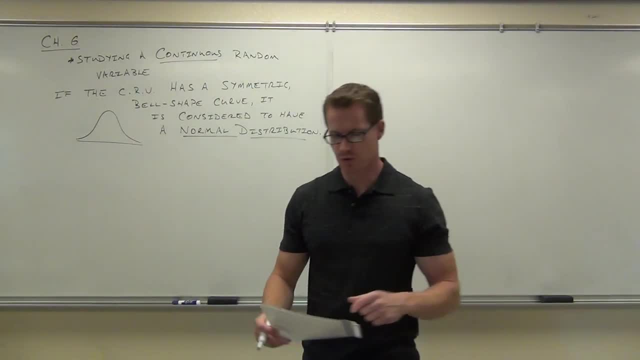 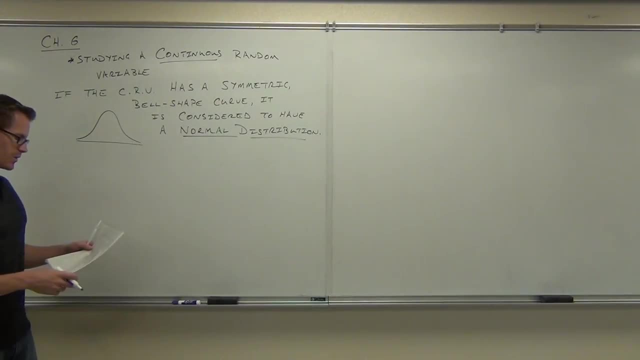 a normal distribution or be normally distributed, And that's what we're looking to have happen In section 6.2,. what we're going to be looking at is something called the standard normal distribution. Now I'm going to introduce this concept of a distribution with continuous random variables. 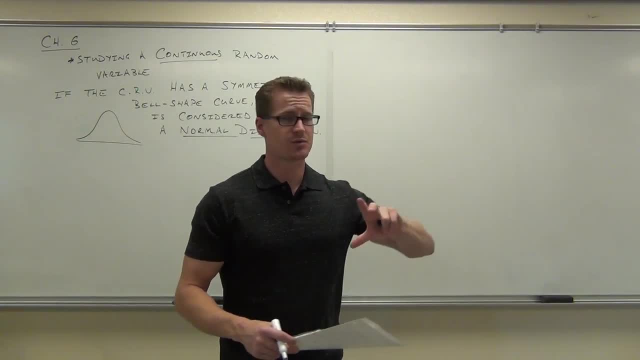 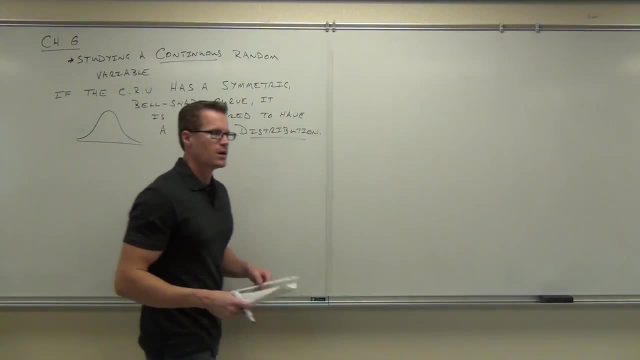 in just a little while and I'll kind of build from what's called a uniform distribution to a standard normal distribution, so you can kind of see the differences and understand what we're going to be doing Basically. here's our idea. You remember the whole z-square idea, right? 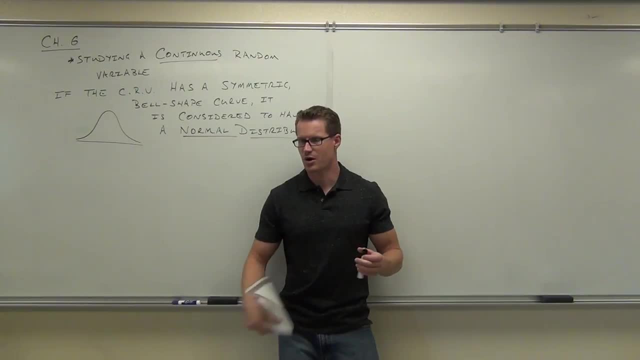 I hope so. If you don't remember the formula for z-square, no problem, I'll give it to you in a little bit. But what we're going to be doing is combine the idea of the area under a curve which, if you've had calculus, you know that you can find the area under a curve. 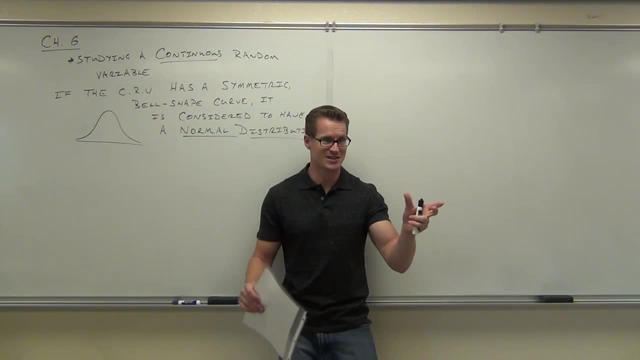 Now, this is not calculus-based statistics, but you could do calculus-based statistics. There is such a class which sounds awesome, right For those of you? I don't know how many people. how many people have had calculus in here? Oh, almost all my students. 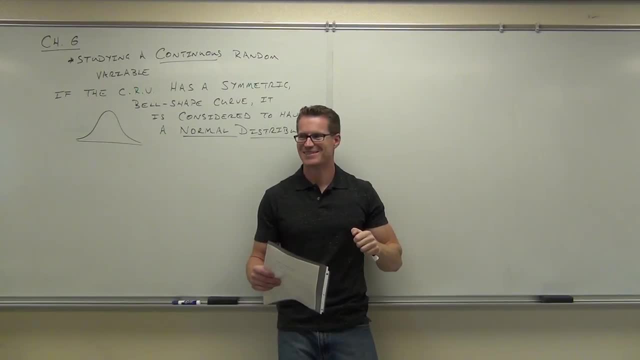 You didn't have the opportunity to take me. I'm sorry for you, But the rest of you, yes, Fantastic. I'll give you my calculus. I teach next semester. Isn't it a good class? Just lie. Anyway, what we're going to be doing is we're going to combine the ideas of area under a 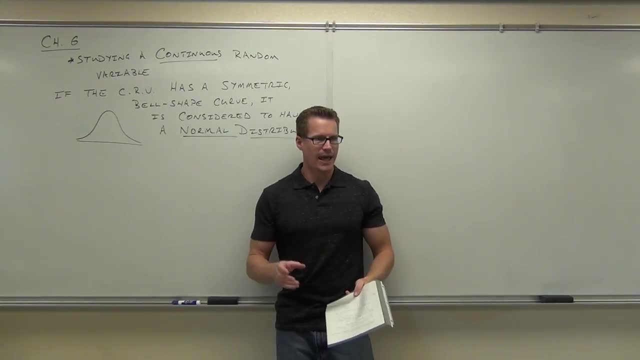 curve with that of the z-score and probability, to tie all this stuff together. That's the goal: The idea of area as being a probability combined with our z-score, And what we need to realize is that the areas ultimately under a curve are going to represent 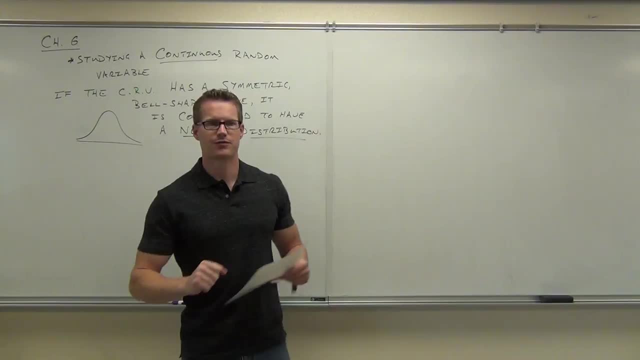 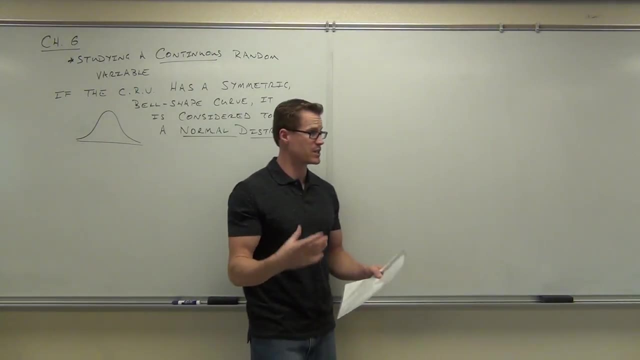 probabilities for us. So we're going to tie those concepts together and be able to figure out probability simply from a z-score and the fact that we have a normal distribution. So this is a really big idea for us that we are dealing with a normal distribution. 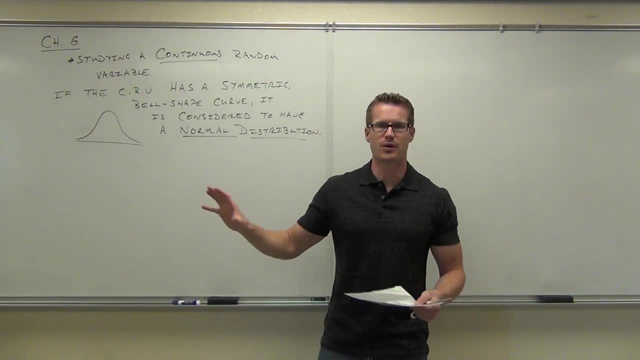 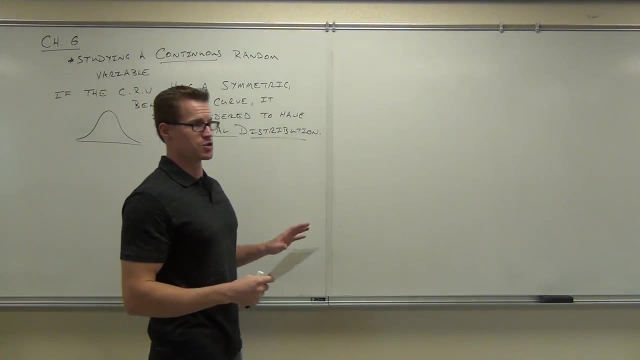 If we don't, if we have a skewed distribution, it's not going to happen for us. We need something that's symmetric for this to work. Now, before we get on into a normal distribution and a standard normal distribution, which is where we're headed, what we're going to need to talk about first is a uniform distribution. 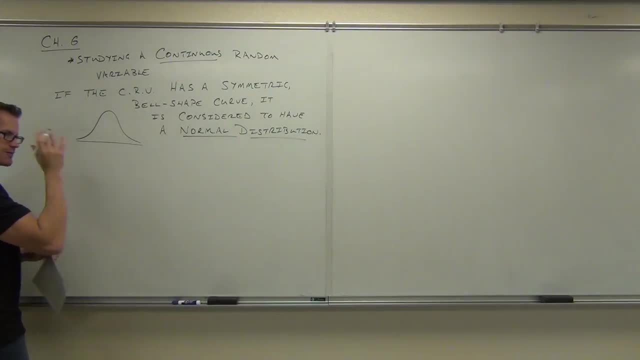 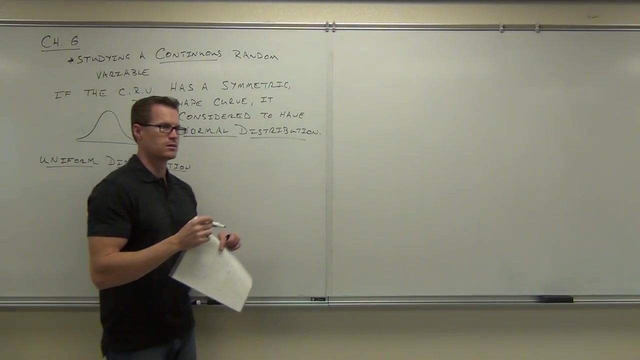 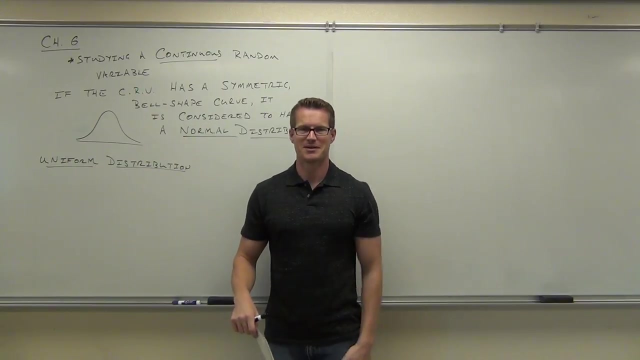 Because I want to get the idea of area combined with the z-score. I want to get the idea of area combined with probability to kind of fit in your head. What's uniform mean, by the way, What's uniform mean? That thing you put on when you go into the military, it's a uniform. 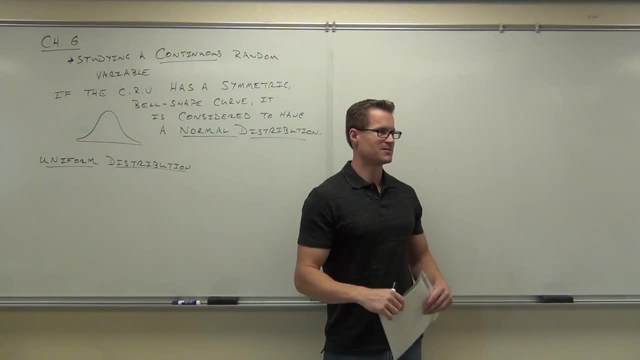 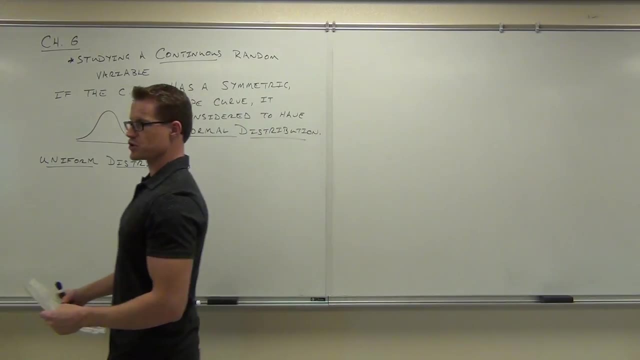 Why is it called a uniform? All of them are identical. That's right. All of them would be the same. Uniform means the same, So in a uniform distribution, all the outcomes are exactly the same. So if you look at the distribution, it would just have a flat line. 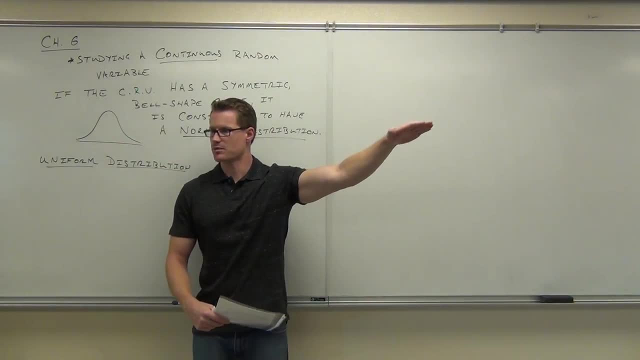 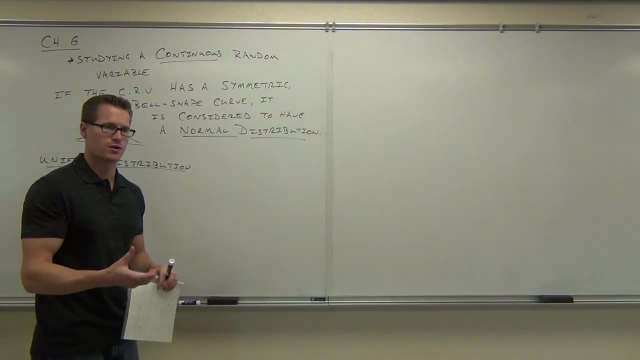 It wouldn't go up, It wouldn't go down, It would just be the same all the way across. You with me on that. It's the most basic type of distribution that we can have, So all the values would have the same probability of occurring if we were looking at a uniform. 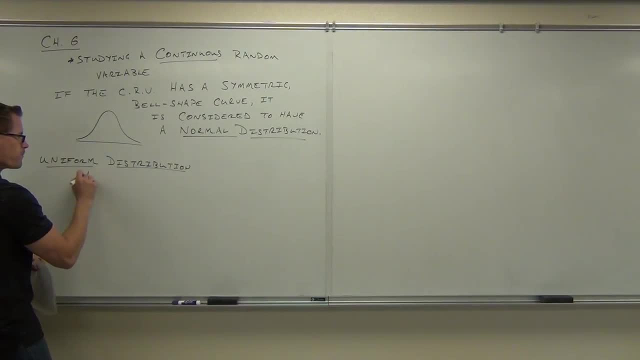 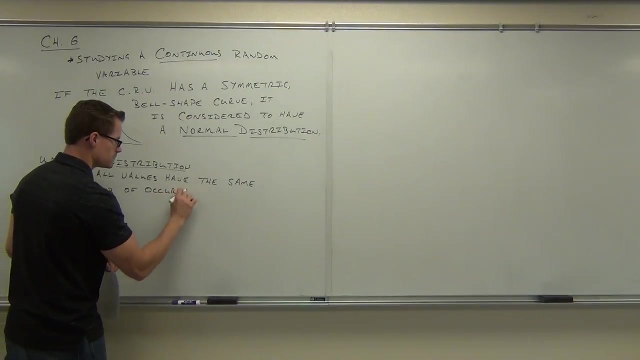 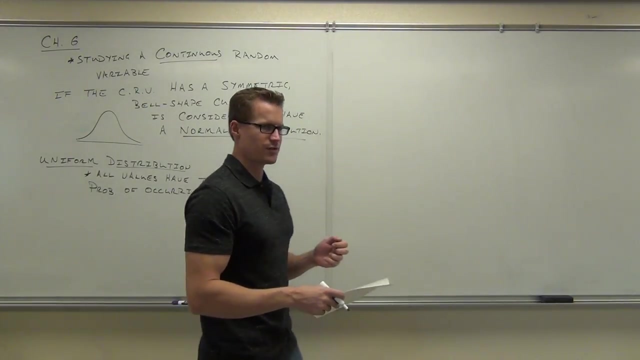 probability distribution, So all values have the same probability of occurring. So I'll give you an example for this uniform distribution. if you want to see one, Okay, We'll do an example over here. Okay, Let's do this example. This will be a fun one for you. 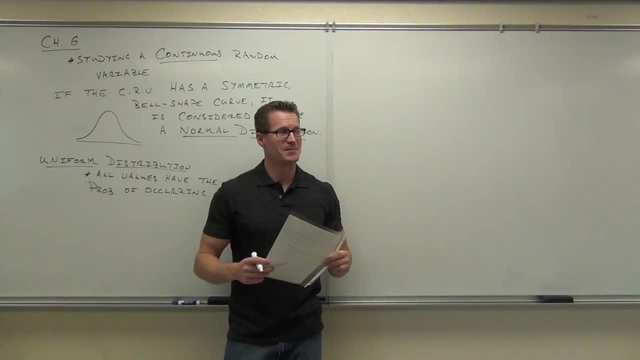 Have you noticed that I typically go over class sometimes? Have you noticed that By like 30 seconds to like a minute, Maybe two minutes, if it's a good day. Five minutes, Not five minutes, Never five minutes, But I usually start like two minutes late. 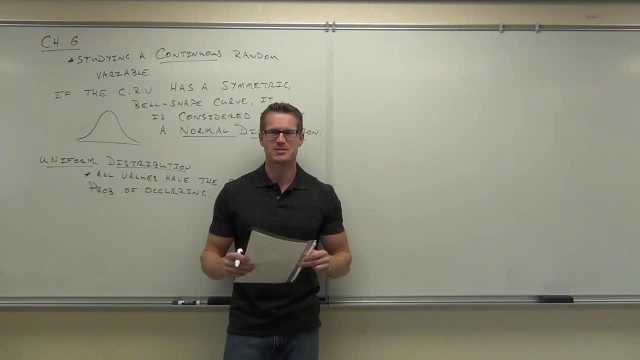 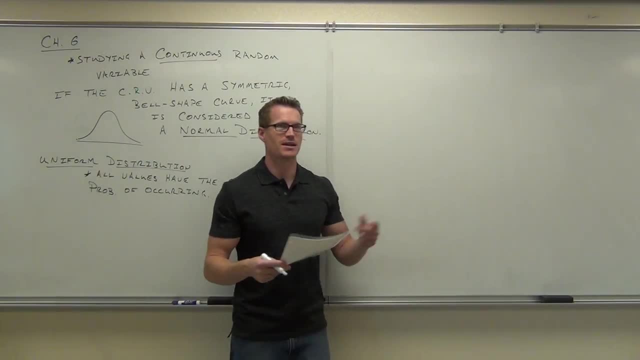 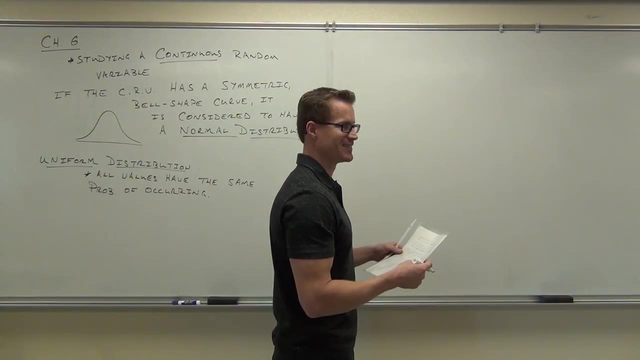 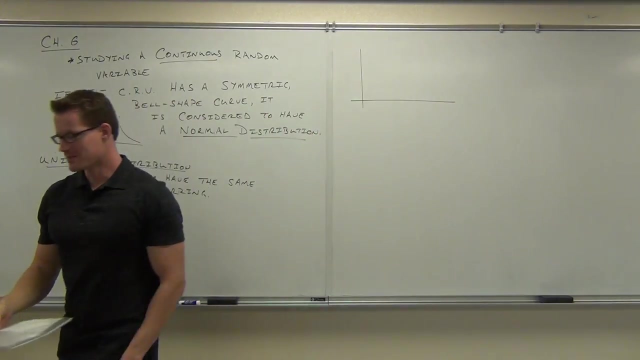 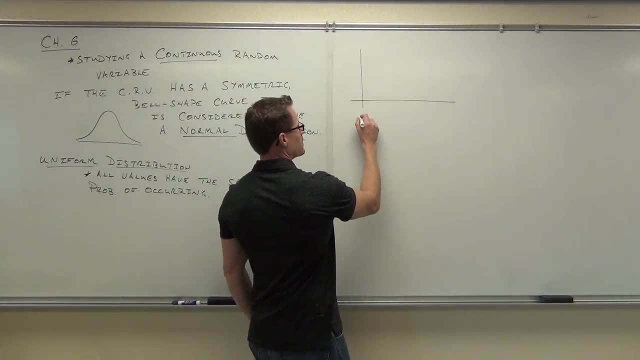 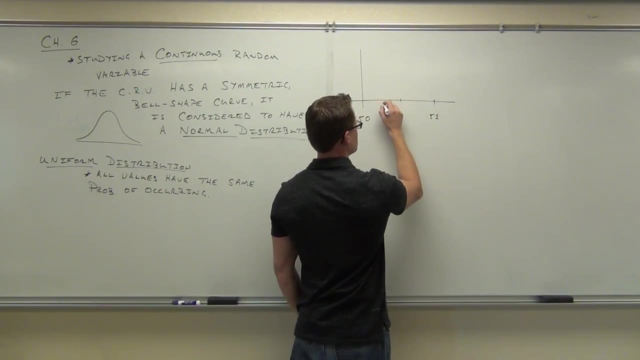 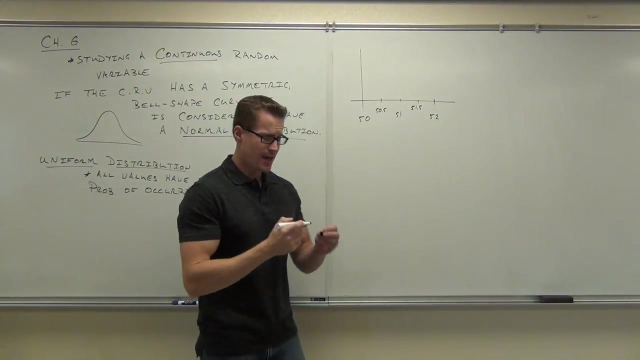 That we get out of class anywhere between 50 minutes after we start to 52 minutes. Here's 51.. Here's 50.5.. 51.5.. We get out anywhere. we never end. We never end before 50 minutes, right. 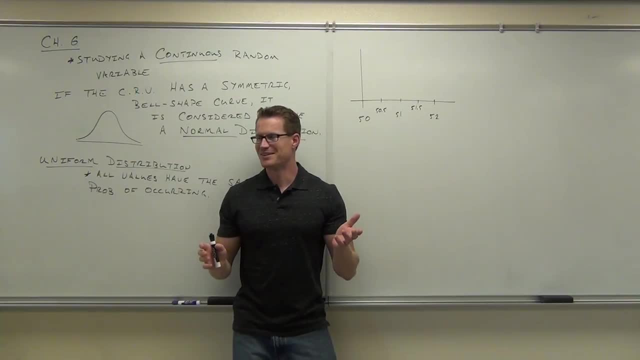 Right Ever, ever, ever, ever. So it's always 50 minutes or after. Usually I try to make it right on 50 minutes, but sometimes the stuff is just so important we have to say like two more sentences and that takes two minutes sometimes. 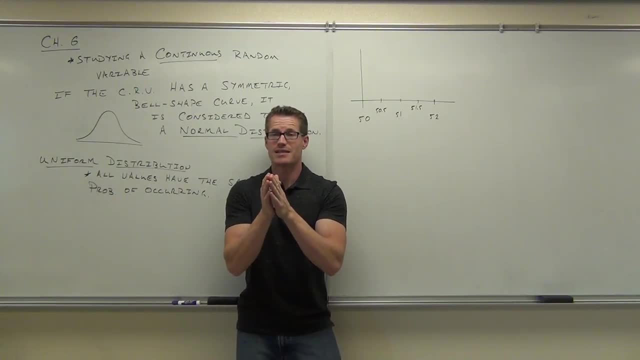 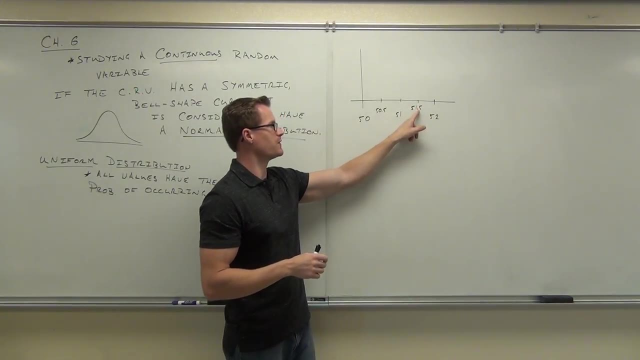 Well, anyway, we end somewhere between 50 and 52 minutes, and the likelihood that that's gonna happen is even across the board. Sometimes we end at 52 minutes and sometimes we end at 51.50, and sometimes we end in here, right? 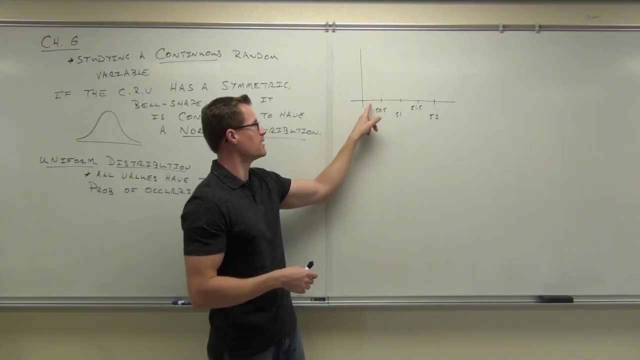 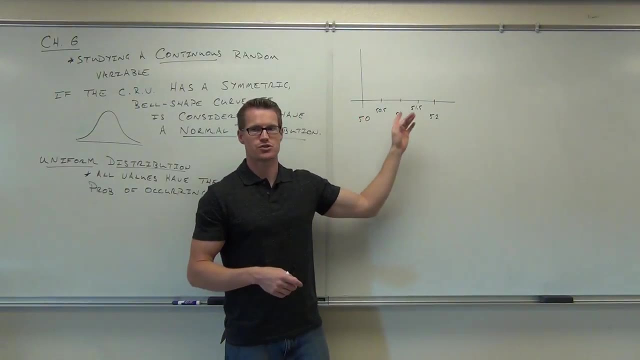 At 51.9 seconds, And sometimes we end it right at 50 or 50.001.. Notice that I could give you any time in this range. true, I could give you any time, So you have to duck a little bit lower this time. 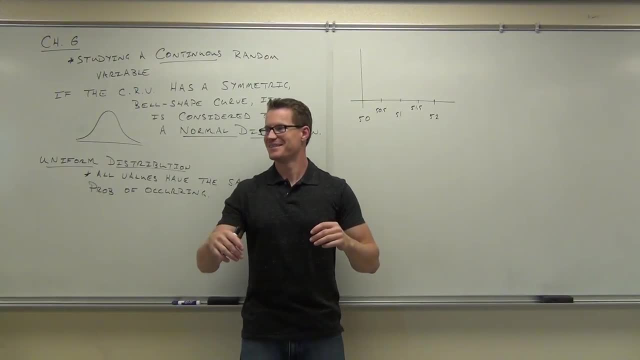 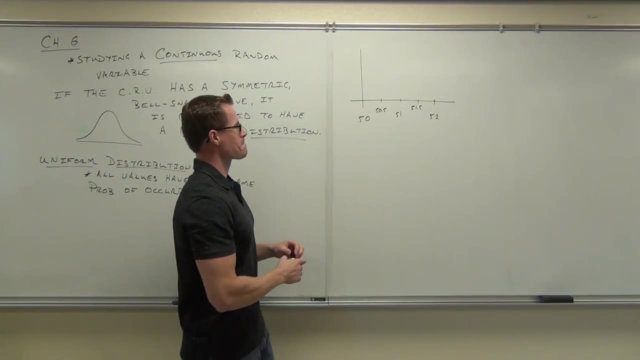 That way in the video. See, let's try it. Do the limbo Like that. Oh, I got you, Got you at the end, Got you right at the end, Anyway. so at any point on this scale you could give me a time that I could end class. 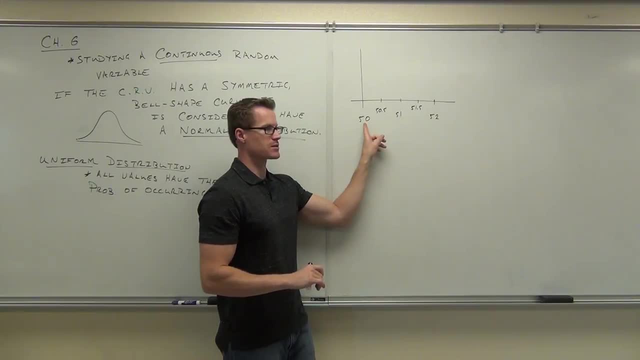 Right. Do we end precisely at 50 minutes? Do we end precisely at 50.5 minutes? 50 minutes to 30 seconds? No, we end somewhere in here, usually, Or here or here. What we're gonna do in this example is say: 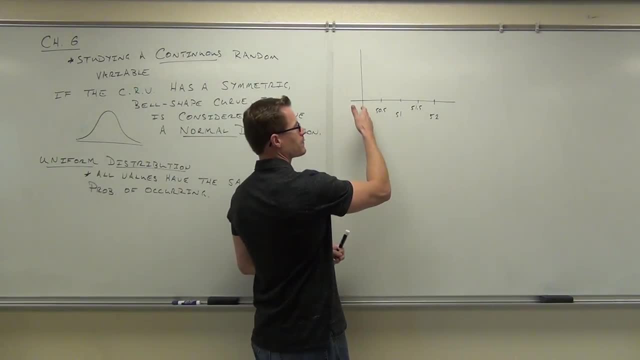 well, let's pretend that the likelihood of ending at any given time is the same for this two minute range. So we could end anywhere, and the chances are equally likely that we end at 50 seconds or that we end- sorry- 50 minutes. 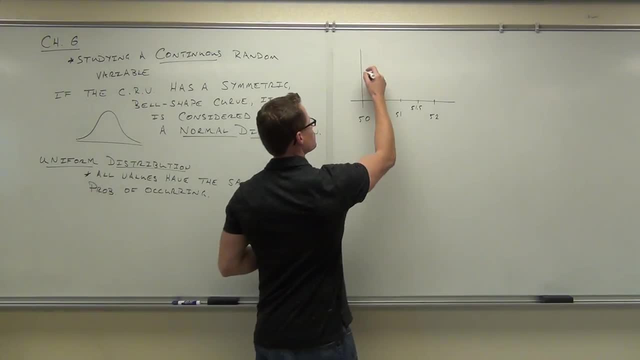 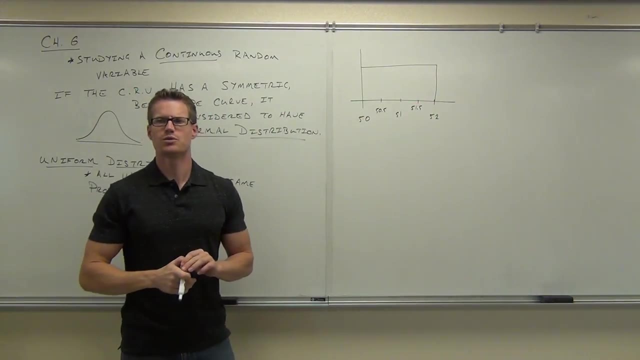 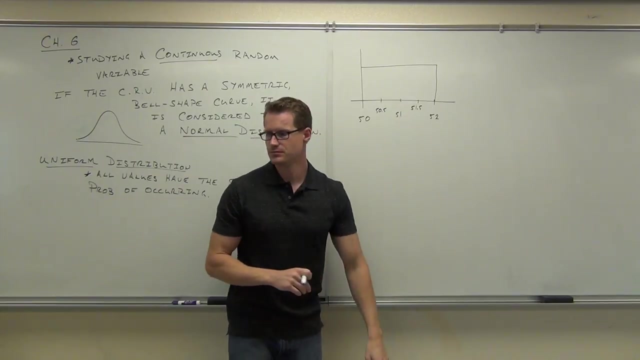 Or 52 minutes, Or 50 minutes and two seconds. So we're gonna say that it's equal all the way across. So it's uniform. The probability of this time occurring isn't equal to the probability of this one occurring, or this one occurring or this one occurring. 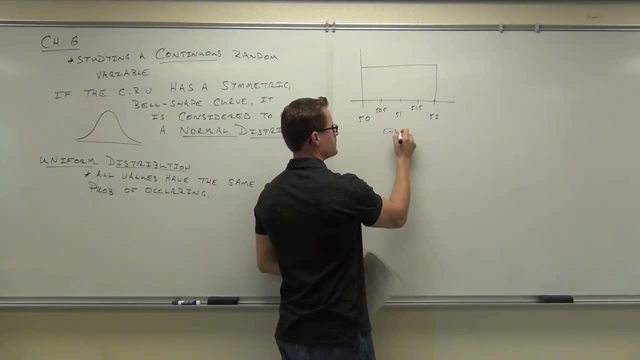 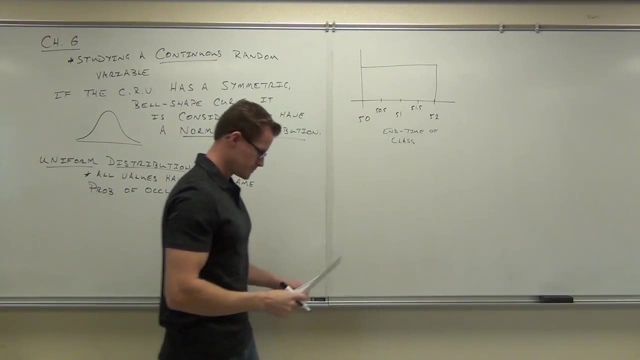 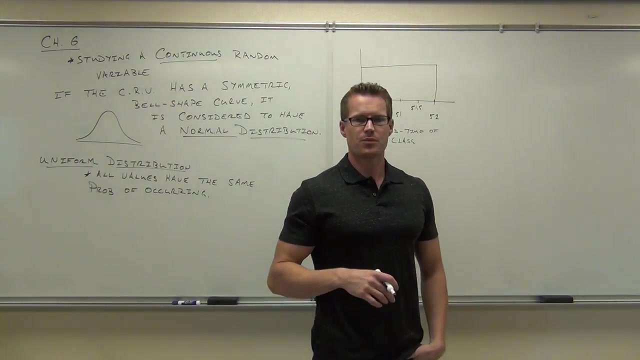 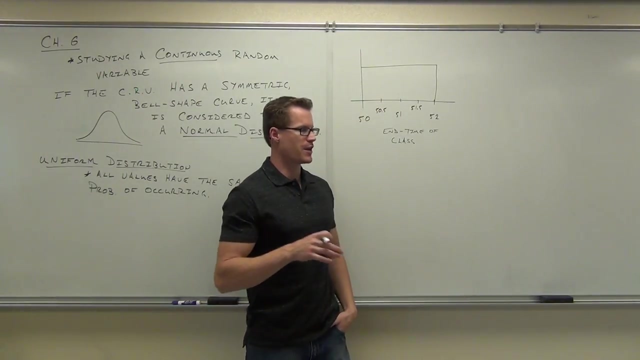 So this is the end time of our class. Now here's what I'm going to do. With a uniform distribution, or any distribution, the ultimate goal is: you want to make the area under the curve equal to one. You wanna make it equal to one. 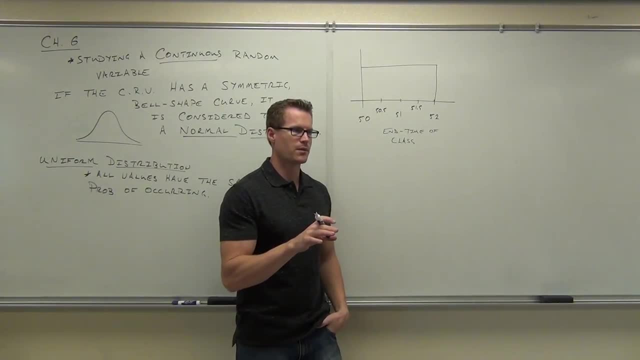 And the reason why I'll tell you in a second. We wanna make it equal to one, because what we're gonna do is associate the area with the probability. Did you know that the area under the curve equals 1?? know that every probability has to be between 0 and 1?? 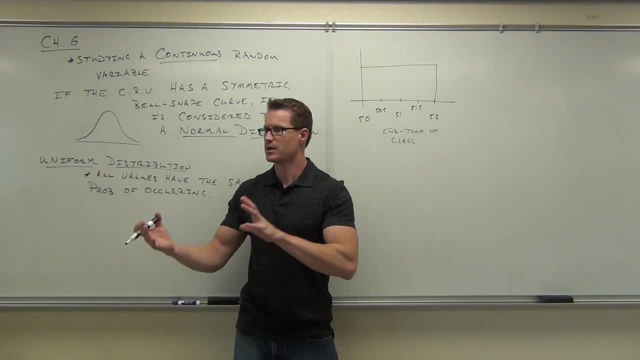 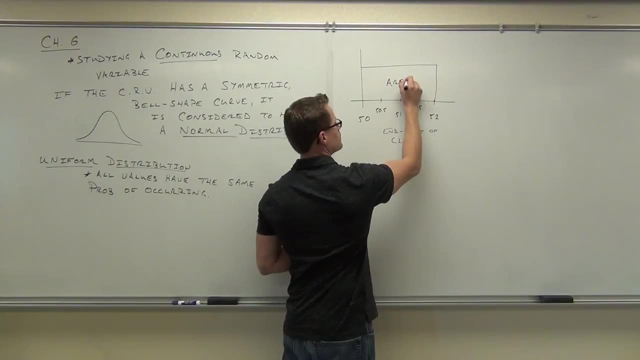 If we make the area equal to 1, then we have a direct correlation between probability and area 1 to 1.. Does that make sense to you? So we're going to try to force this area to equal 1.. We're going to force the area to equal 1.. 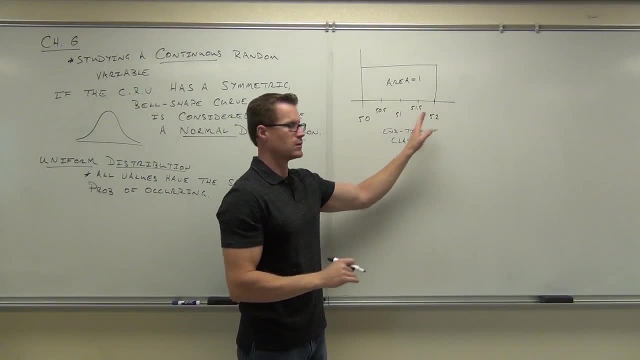 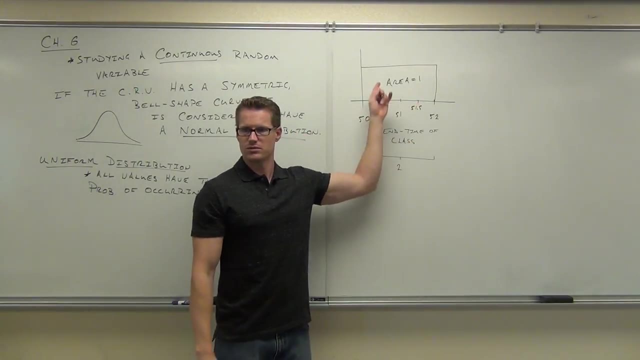 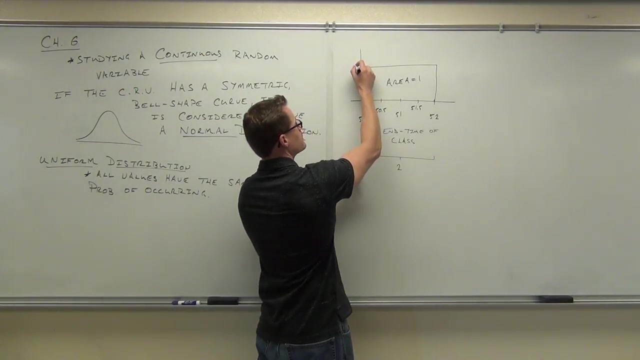 What's our width for this interval? So our width is 2,. OK, Width is 2.. This is a rectangular shape. true, To find a rectangular shape, you take the base times the height. So if my width is 2,, what do I need this value to be up here? 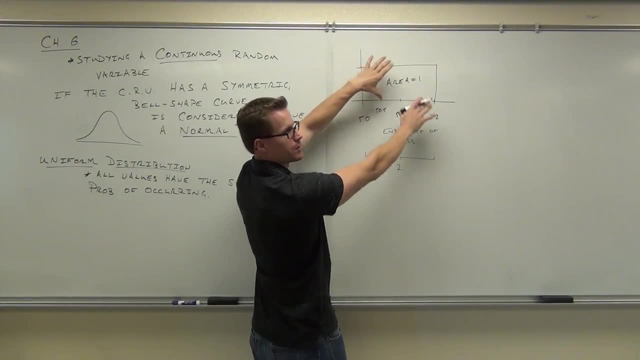 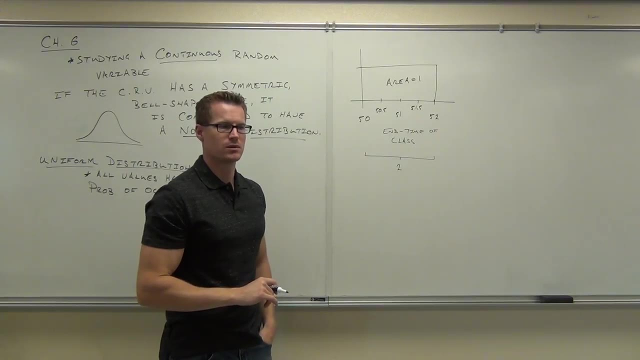 so I take the base times the height and it gives me 1? 2 times 2 would be 4.. 1 times 2 would be 2.. 1 half 0.5.. Where's the 0.5 coming from? 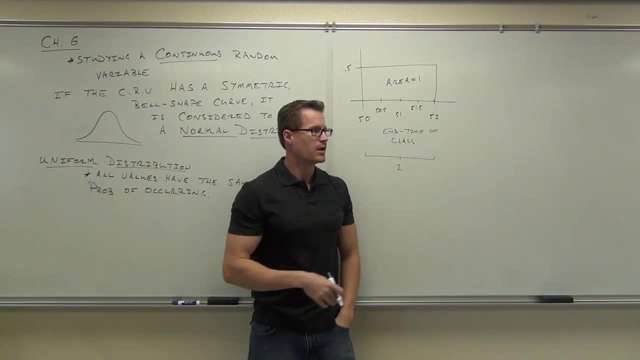 0.5 is coming from. I need the area to be 1.. Doesn't mean that You can't say that every single probability has 50% chance of occurring, right, You can't even say that because there's an infinite number of values. 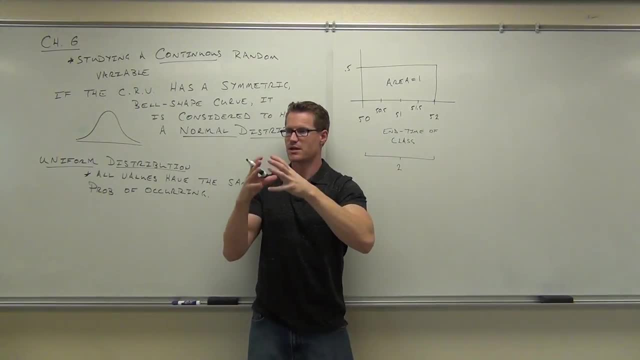 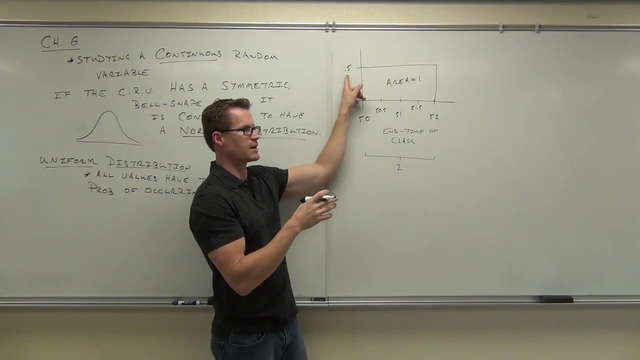 If everyone had a 50% chance of occurring. add those all together you're going to get an infinite number times 50%, right? It doesn't even make sense. So this probability is kind of or this thing right here. that's not really the probability for each value to occur. 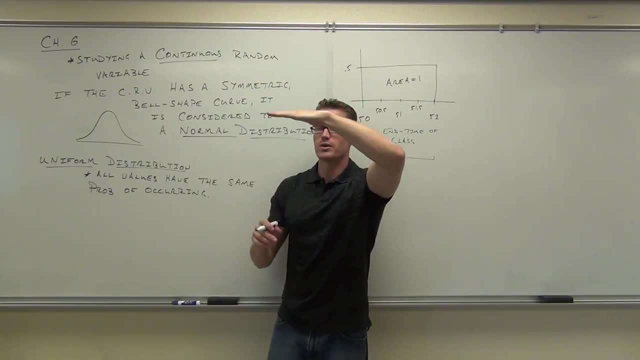 All we're saying is we have an equal value or equal probability for each of those outcomes to happen. We're forcing this thing to be a level of 0.5 because we need the equal 0.5. Because we need the area to be 1.. 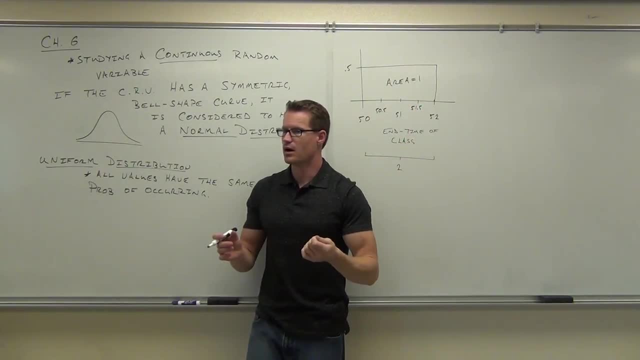 That's where the 0.5 is coming from. It's not just a made up number. It has really nothing to do with the probability for each one of these things. In fact, if you think about this, I really do want you to think about this. 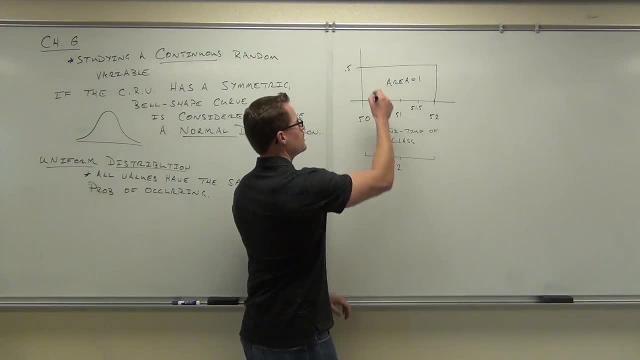 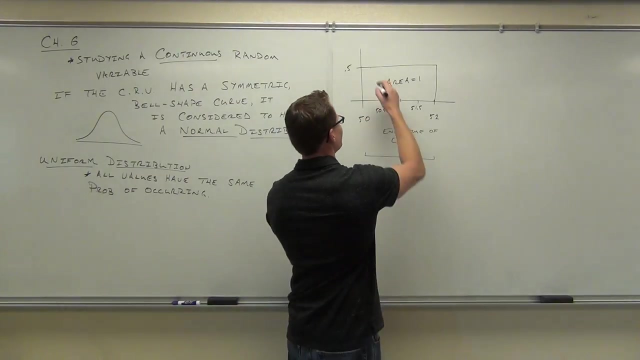 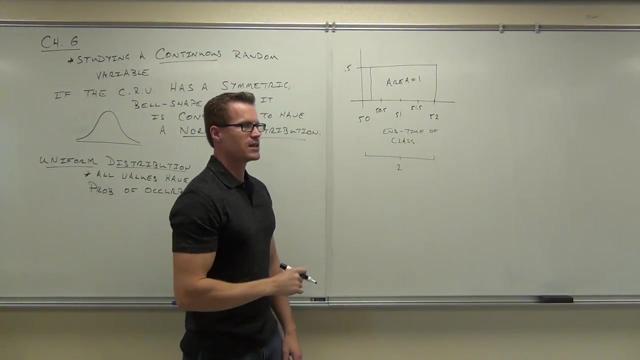 This actually has a calculus concept behind it. What's the probability? oh shoot, that's supposed to be straight. Got to stop drinking vodka before class. Wow, Just kidding. just kidding. Can you tell me what's the probability of getting exactly this time? 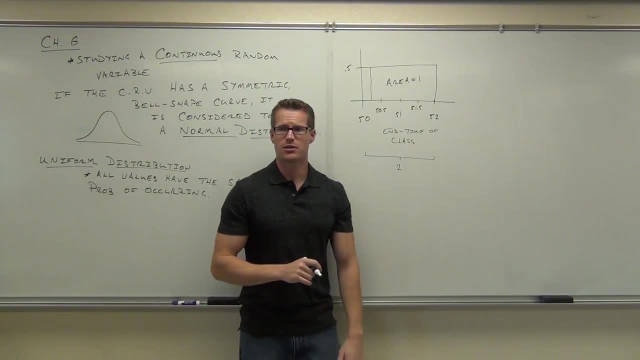 Let's say this is 50.452783.. What's the probability of getting exactly that time, that the class ends on Exactly that time? What do you think? How many possible values do I have between here and here? Don't tell me a 4.. 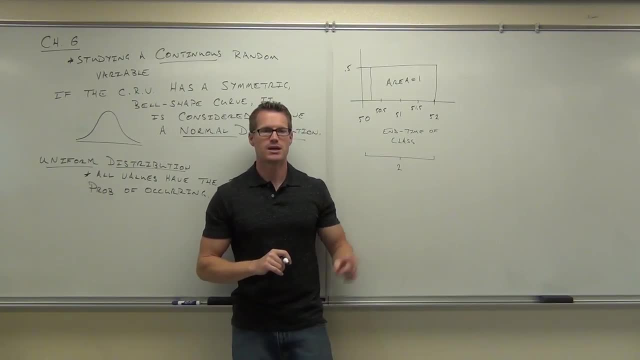 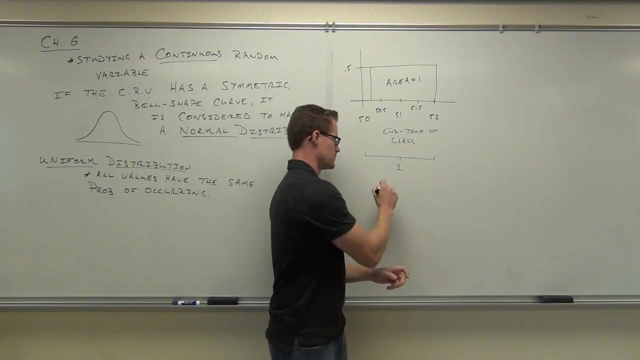 In 5.. In 5. I'm picking an infinite number. I'm picking 1 out of an infinite number. What's 1 divided by infinity? How much is it? What's 1 divided by 10?? I talked so long, my pen dried up. 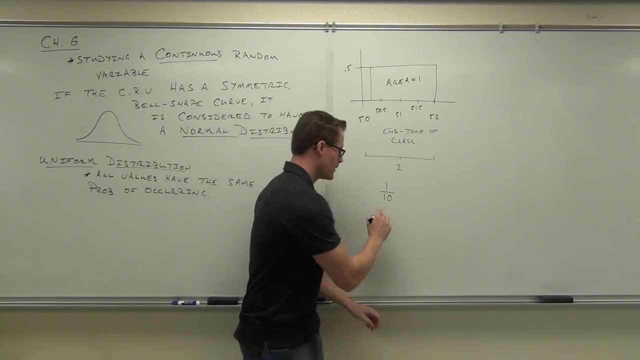 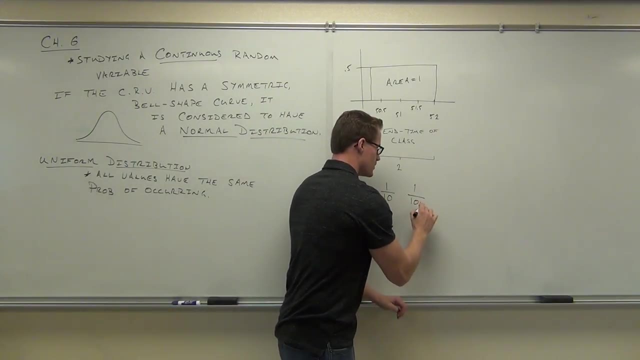 What's 1 divided by 10?? Square root of 0.. This is .1,. yes, Okay, you know how to do math, true? What's 1?? 1 divided by 100.01.. What's 1 divided by 1,000?? 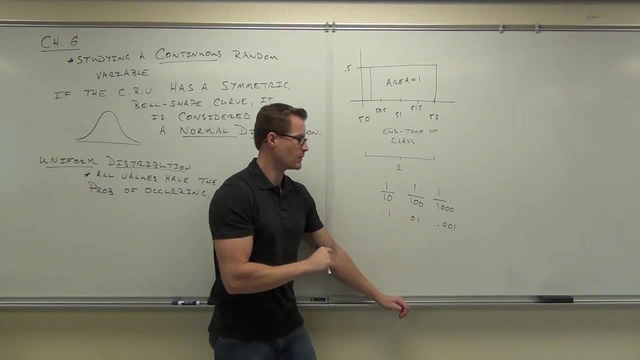 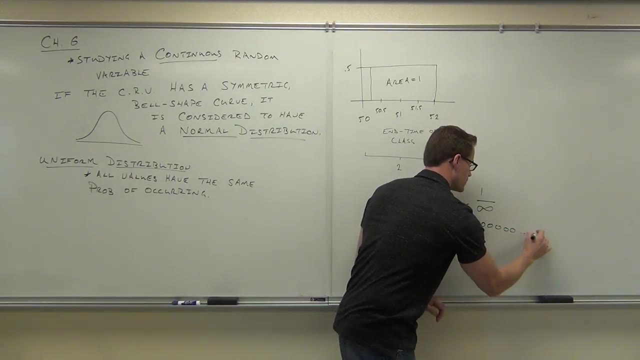 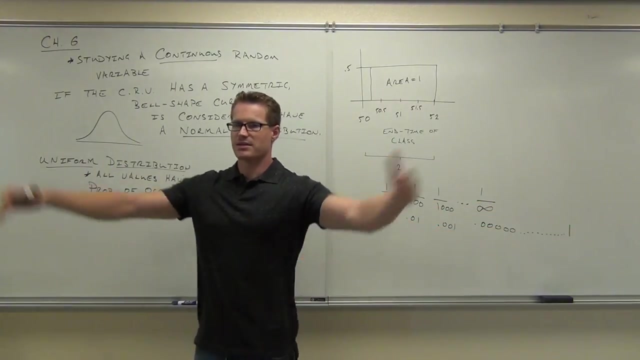 .001.. Are the numbers getting bigger or smaller? Smaller: What's 1 divided by infinity: .001.. Whatever I stop at, actually it's not even that. It doesn't actually ever end, because infinity is a massive number. It's not even a number because I'm forever. 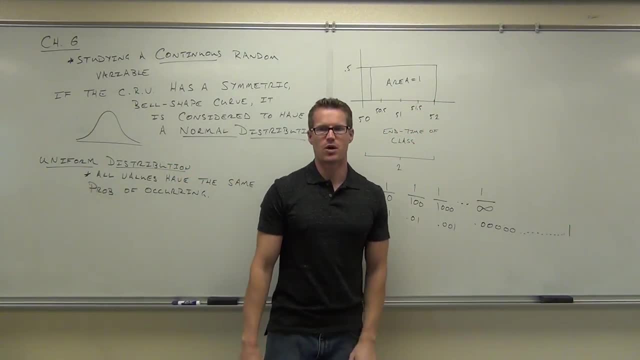 You can't ever reach the end of it. So what's happening to these numbers? Are they getting bigger or smaller, Smaller, Smaller and smaller, Smaller, Smaller, Smaller. And, starting off, if I've, instead of something bigger, 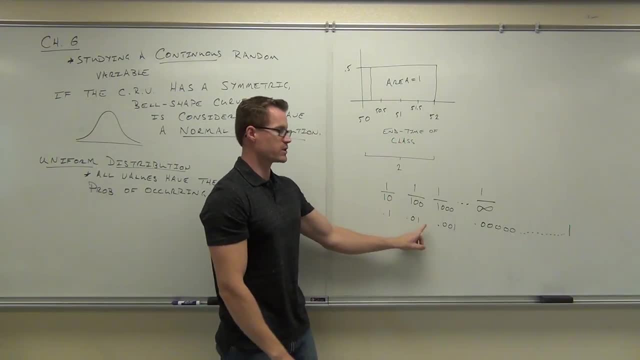 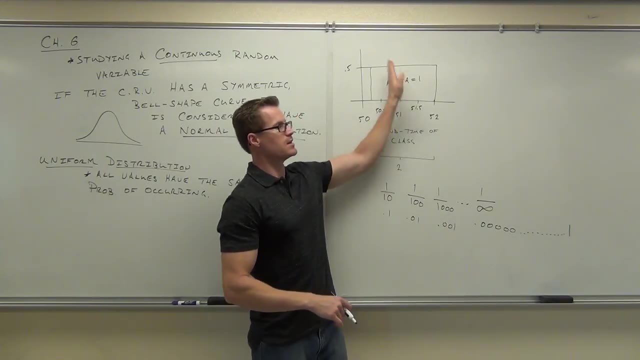 I've got a little bit bigger. So what's the difference when a number is around? Well, one number gets one little bit bigger, or the other number gets 4 or 5.. I make 5 more moves. Yeah, I've got an infinite number of segments. 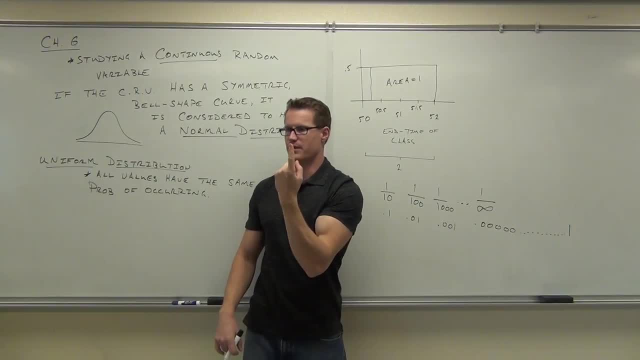 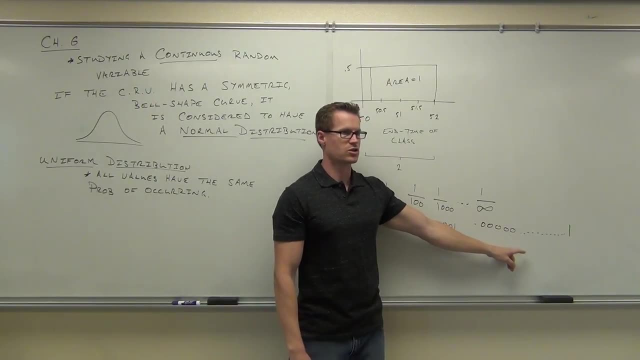 What's the change in the probability of this? This is a probability, right? If I had ten segments, the probability of choosing 1 of them would be .1.. I'm going to get one of them, or this probability is 0.1, 0.01, 0.001.. 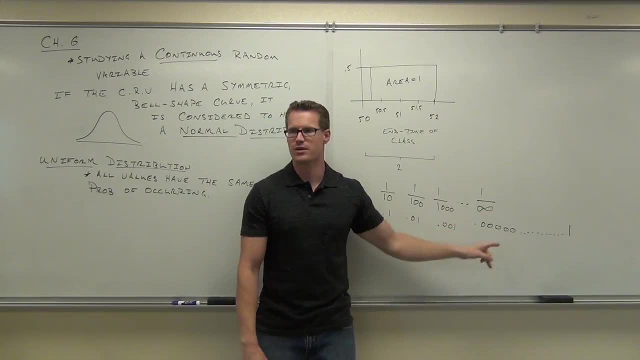 What's the probability that I'm going to pick one item out of an infinite number of them? It's like finding a needle in an infinite haystack. Are you going to do it with one guess? Are you going to go in there? let me find this needle. 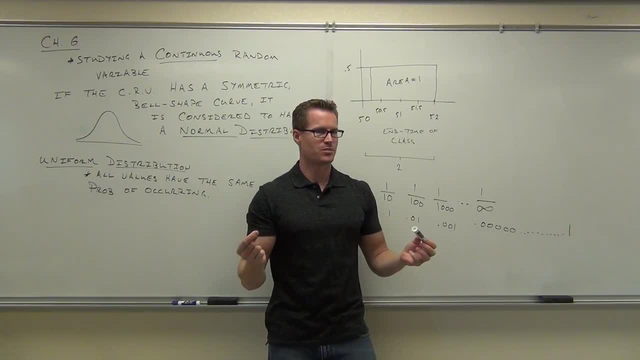 Oh, I caught it. Is that going to happen? Is it? Are you going to find a needle in an infinite haystack, One needle in a stack of hay that's bigger than the earth? Can you do it With one try? Probably not. 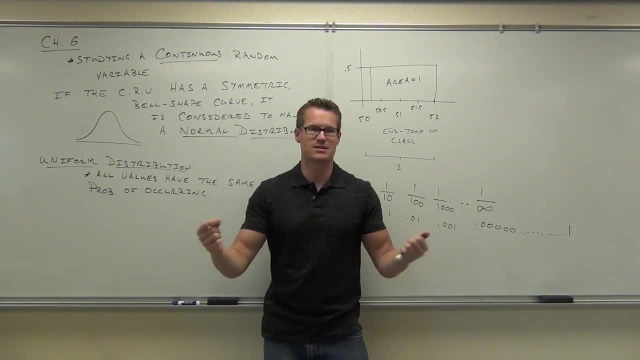 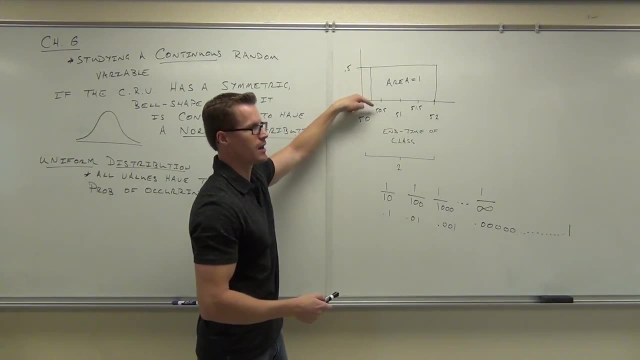 Your probability is very close to 0.. Very close, In fact. it's 0.. If you take it to infinity, it's 0.. So this probability of actually finding one time, one specific time, the probability is 0. 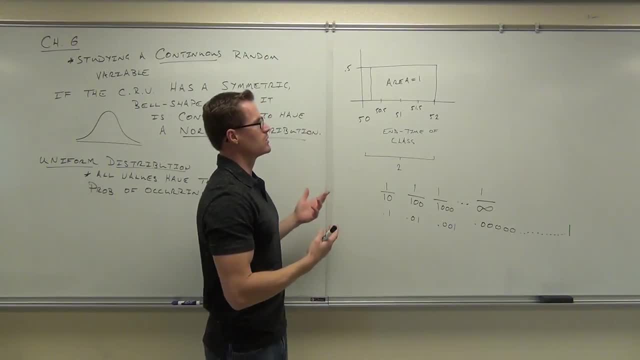 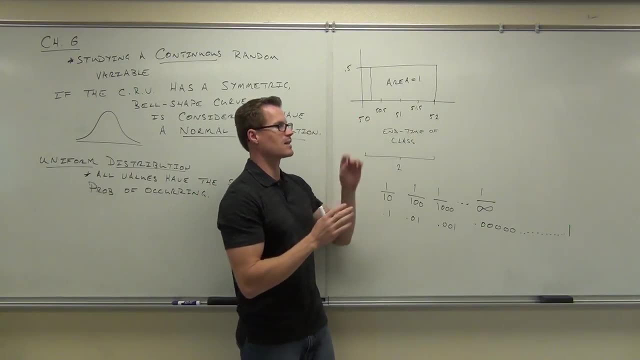 Raise your hand if you understand that That probability is nothing. So, instead of actually looking for one time, what you have to say is: I'm going to look at a range of times. What's the probability, Instead of ending at exactly 50.43.? 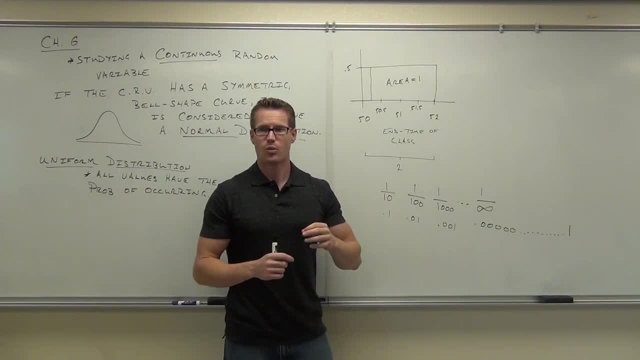 2,, 7,, 8,, 9 seconds or minutes. we're going to say what's the probability that this class is going to end somewhere between 50 minutes and 50.5 minutes. You have to give a range of numbers, because one specific one doesn't even calculate. 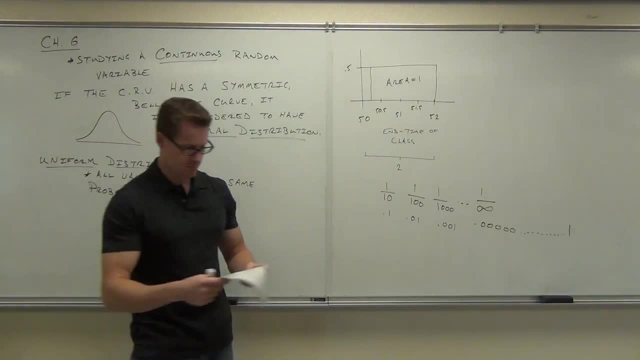 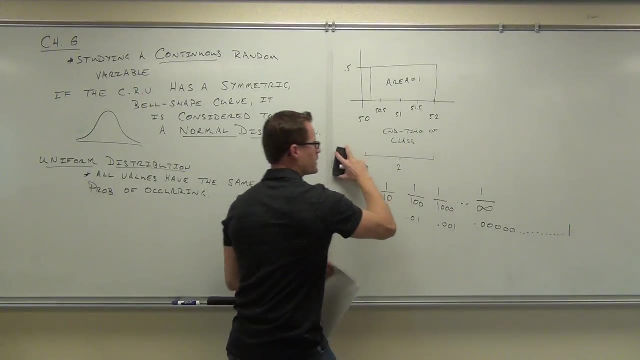 You get 0 every time. So where this number comes? because we're forcing the area to be 1, our width is 2, our area is 1.. We can't find the probability of any specific given number, because that's like finding a needle. 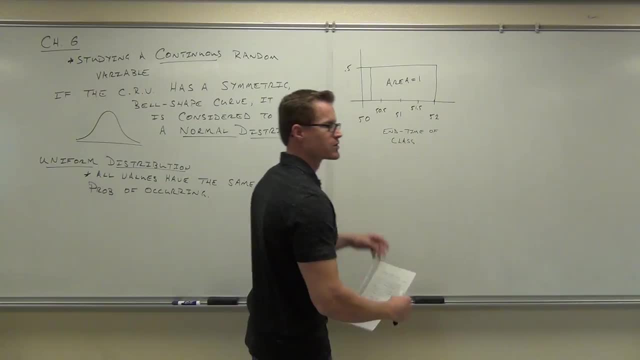 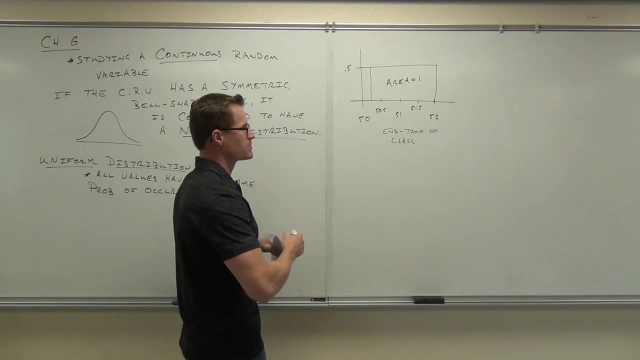 In a haystack bigger than the universe. it's not going to happen. all right, It's 1 divided by infinity. You cannot do that. It's 0.. It's 0. There's no probability in that. So instead, what we do is we realize a couple things about this and then we calculate the probability of a range. 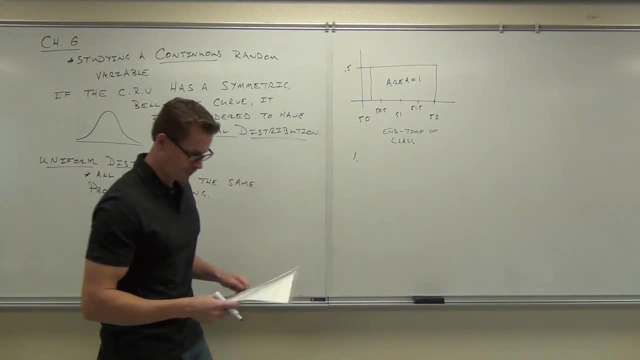 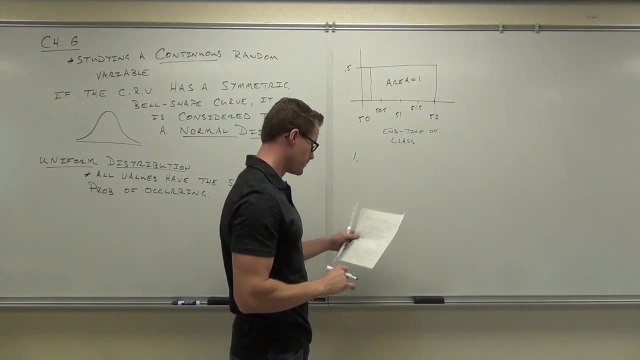 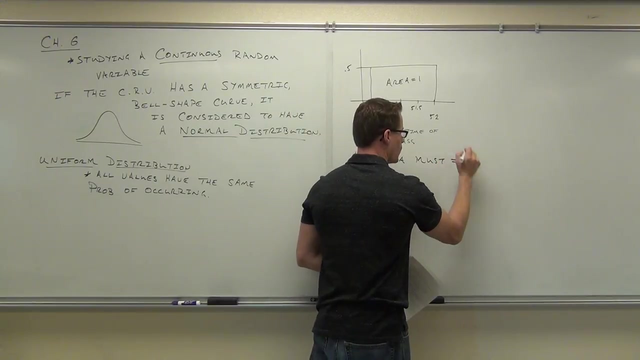 First thing we're going to realize. it's called a density curve. A uniform distribution is a type of density curve. Density means like an area curve. Firstly, the area. It must equal 1.. And the reason why it has to equal 1 is because we're going to associate the area with the probability. 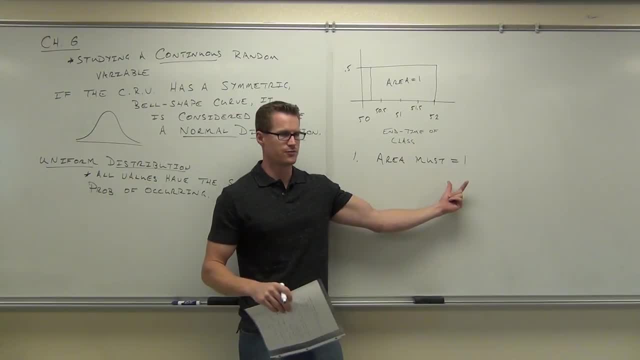 We're going to get a proportion of this area right like 0.3 or 0.25 or 0.5. That's how much area we're going to have covered in here. If the whole thing equals 1, part of it is part of 1.. 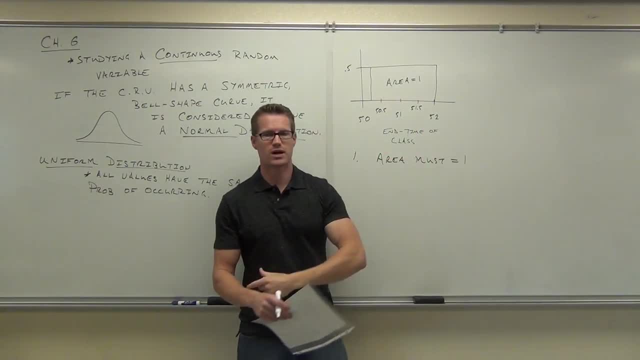 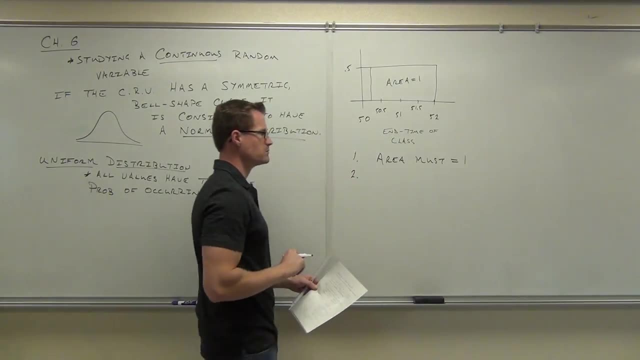 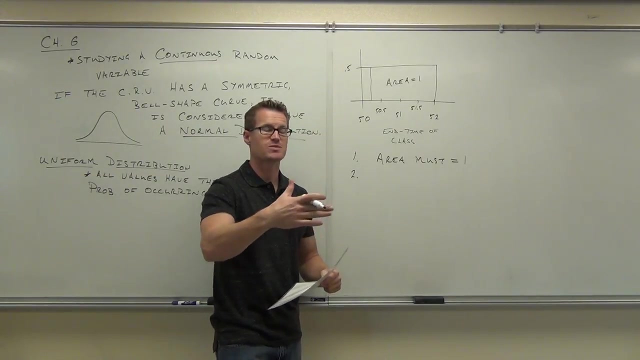 True, If our area equals 1, we're going to associate that directly, in a 1 to 1 correspondence, with our probability, Also because we're going to have a distribution. we're going to have a distribution Because we're associating this with a probability. the height of each individual value has to be less than 1, less than or equal to 1.. 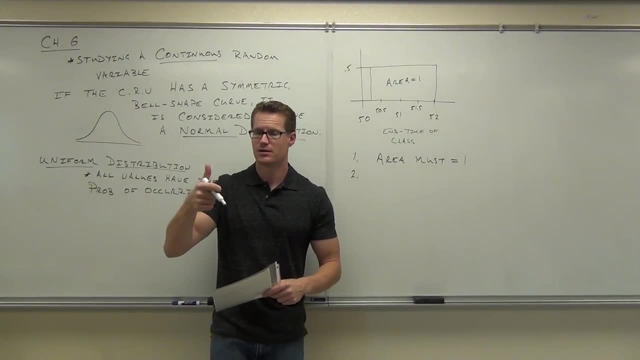 Can you ever have a probability that's greater than 1?? No, By the way, this is a good kind of segue- not a segue, but a little side note On some of your homework that I graded and I'll pass back to you in a little bit. some people gave me probabilities of 2.937 or something on one of your problems. 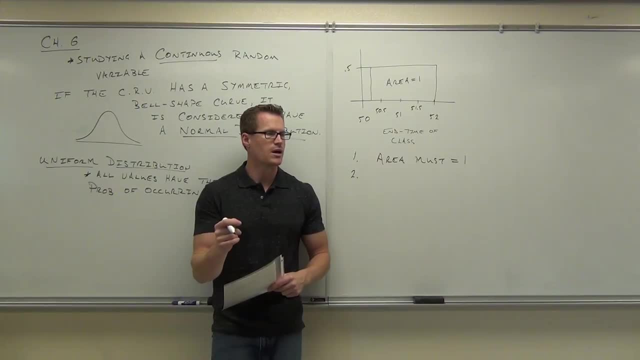 If your calculator says 2.937 for a probability, you need to have a probability of 2.937.. If you need to read a little bit further, it might be saying times 10 to the negative 4 or something. Did you see that on some of your problems? 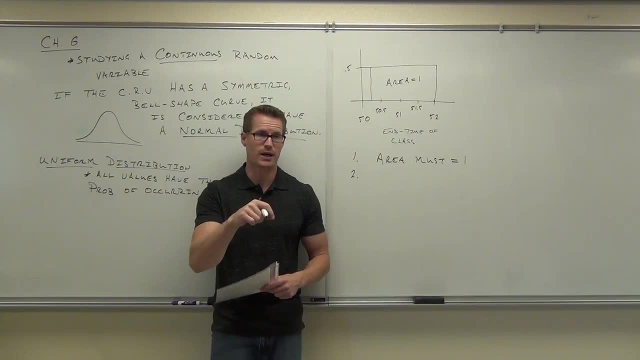 Because what that means is you need to move in a decimal place. Don't give me 2.937.. That's not the right answer. If you have 2.937 times 10 to the negative 4, it's .000297.. 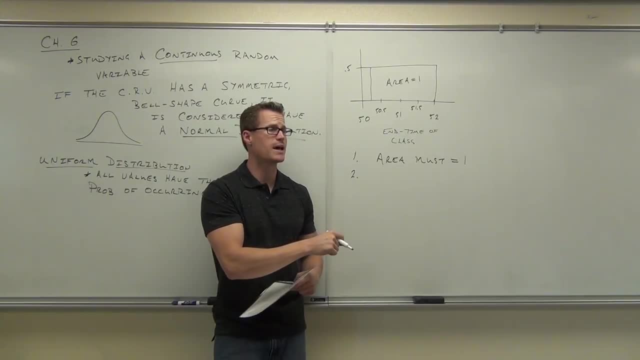 Okie dokie. So know how your calculator works. Your probability will never be greater than 1, ever. With that in mind, this probability for each individual value will be less than 1.. So the height for each value must be greater than or equal to 0.. 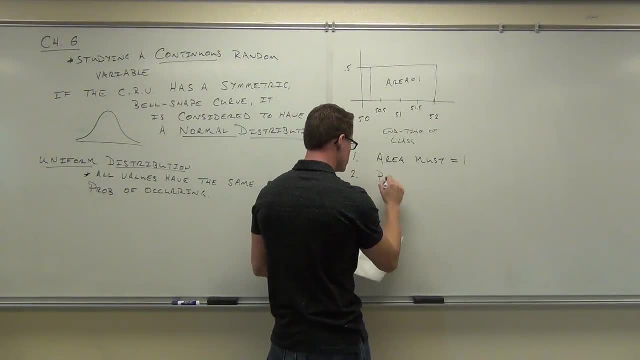 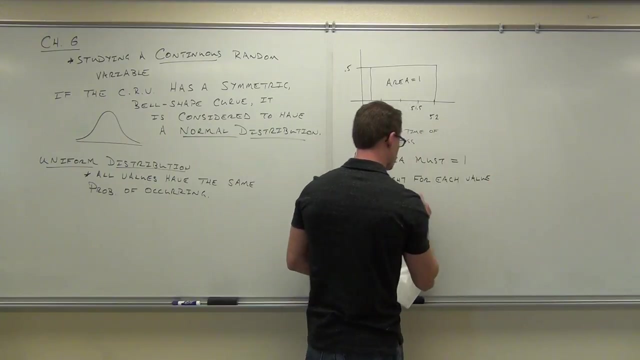 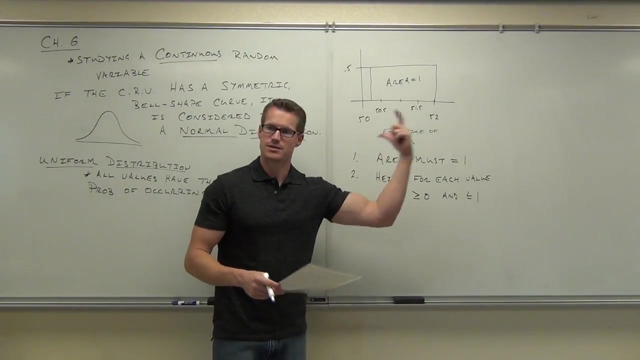 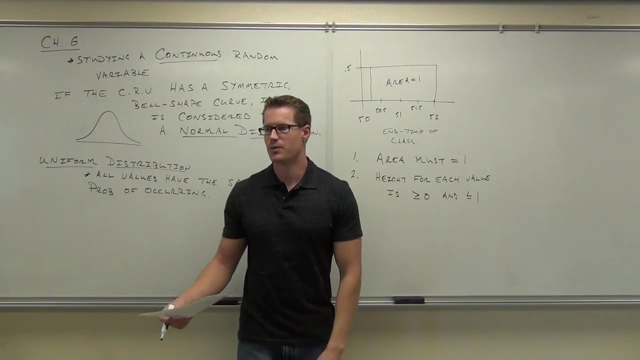 Or less than or equal to 1.. These two conditions- Let our density curve or our distribution- represent our probability, If that is equal to 1.. Probabilities are equal to 1 if you add them all up. Look what we're doing. 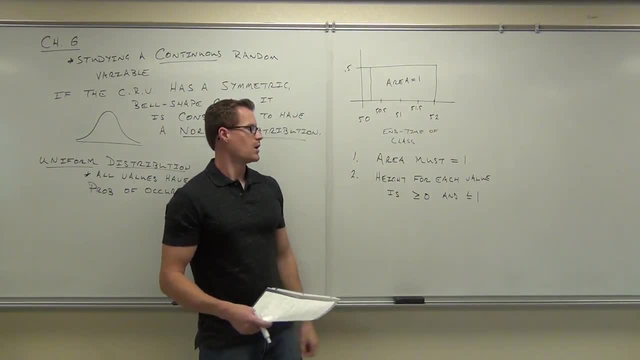 We're adding them all up. right, Add them all up. It's equal to 1.. Also, each one has to be between 0 and 1.. That's true for probabilities as well. That lets a graph represent probability for us. 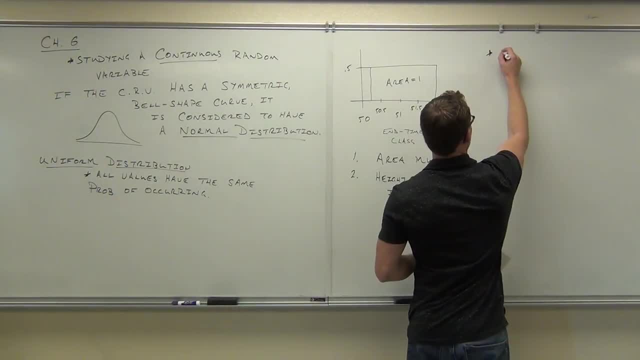 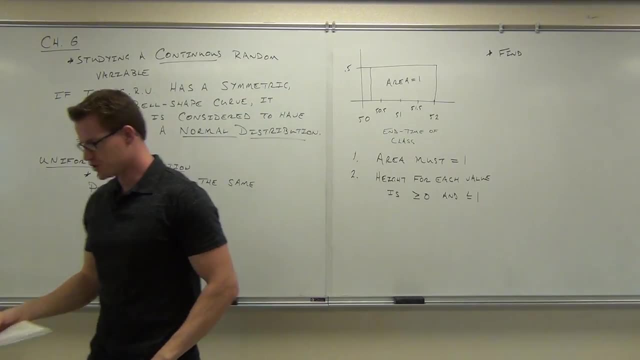 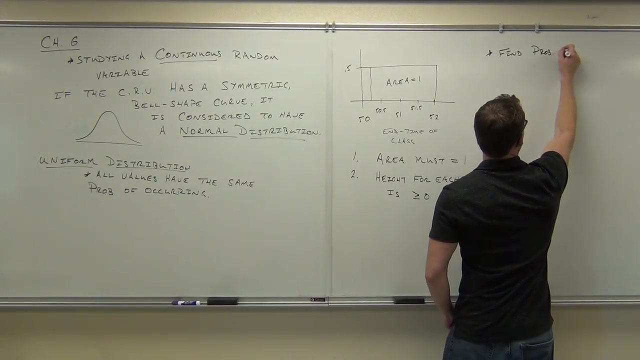 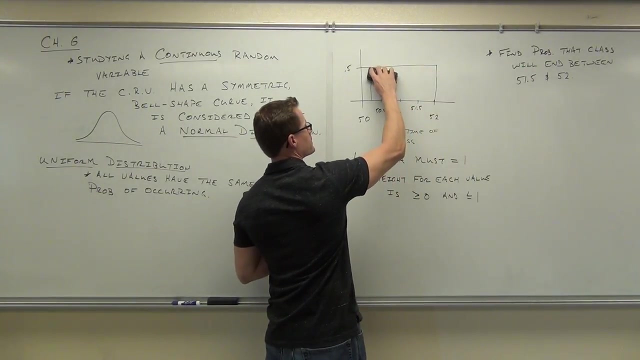 And it lets us solve this question- Find the probability that our class will end between- Let's do- 51.5 minutes and 52 minutes. Hey, let's go over this one more time. First, I'm going to erase the area equals 1, because, well, that's true. 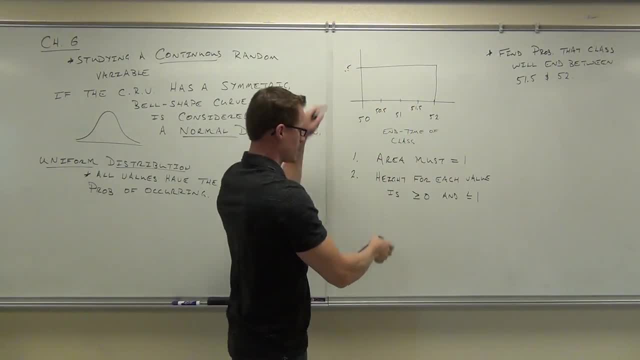 The area does equal 1.. We made it so that it did. We put that certain level there so that our area is equal to 1.. Are you all with me on that one? Feel okay with that. All right, One last time. 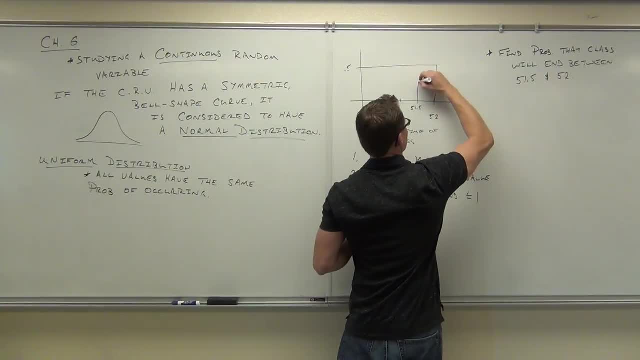 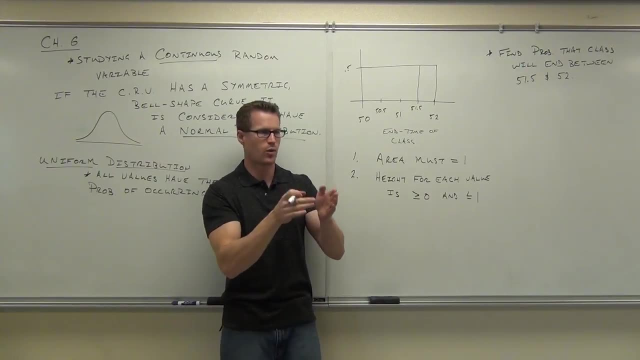 What's the probability of the class ending at exactly 51.5?? What's the probability the class will end right at 51.5?? 51.5, 0, 0, 0, 0, 0, 0, for eternity. 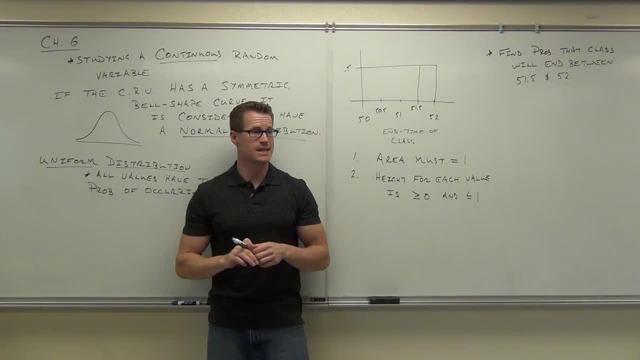 What's the probability of that happening? Zero. What's the probability of any single value occurring in a probability distribution with a continuous random variable? Zero, Zero. The probability of the single value is zero, not your head, if you're understanding that. 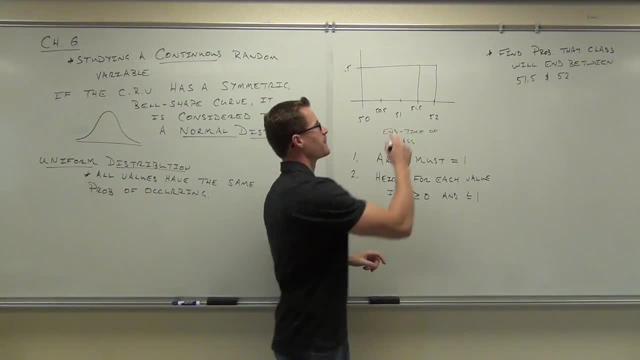 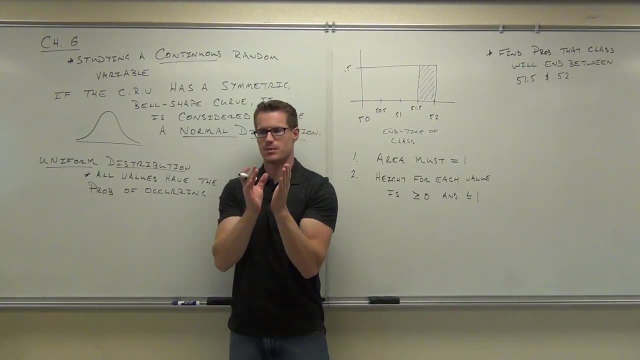 Good deal. So what I'm asking you is not for 51.5, but this range. I'm asking you for what's the probability we're going to end between a couple times Between 51.5 and 52.. That's something we can talk about. 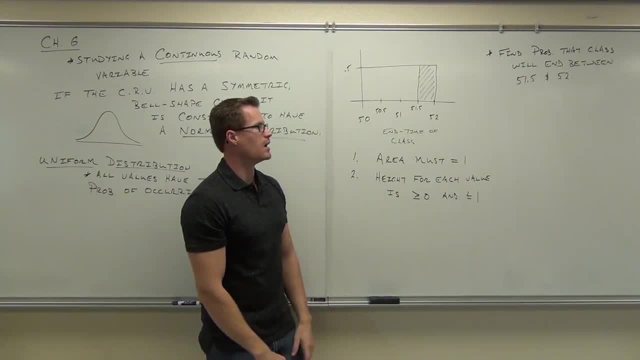 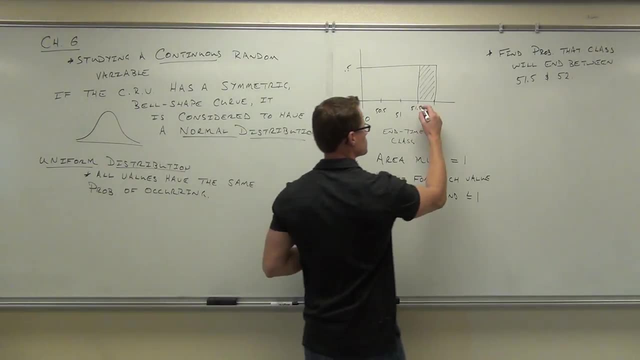 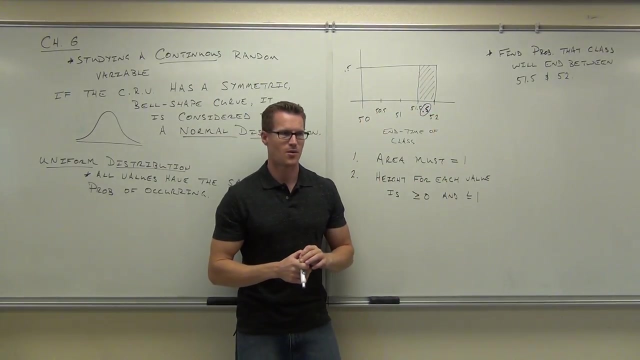 That's a range of numbers, That's an area. Let's see if we can calculate this area. How wide is my rectangle? I think the memory was .5.. At least I hoped it was. How high is our rectangle? .5.. 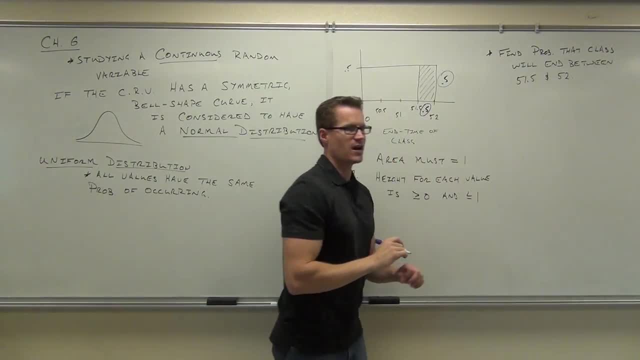 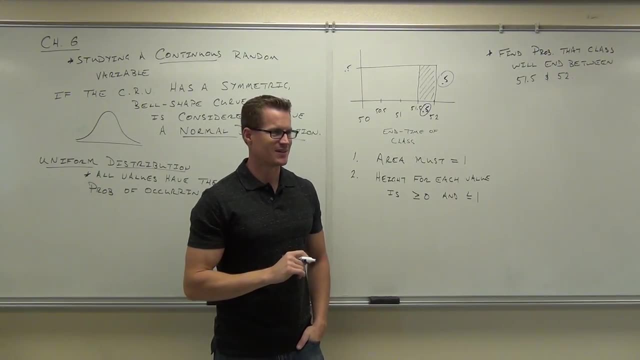 How do you find the area of a rectangle? You can say it louder than whispering: How do you find the area of a rectangle? Length times width? What's our length? .5.. OK, What's our width? Nice, This is actually a square. 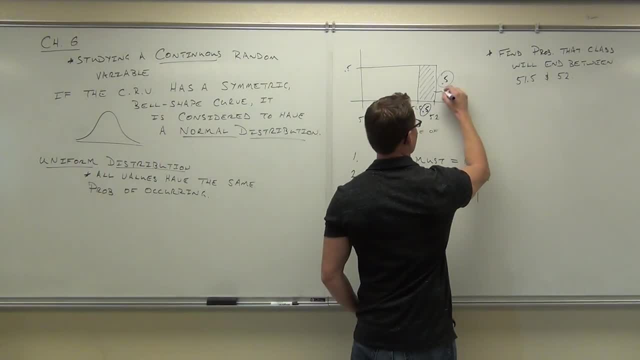 Somehow it doesn't look like a square, but it's a square. Our area is .5 times .5.. We can all do .5 times .5.. How much is that? .5., .5., .5., .5.. 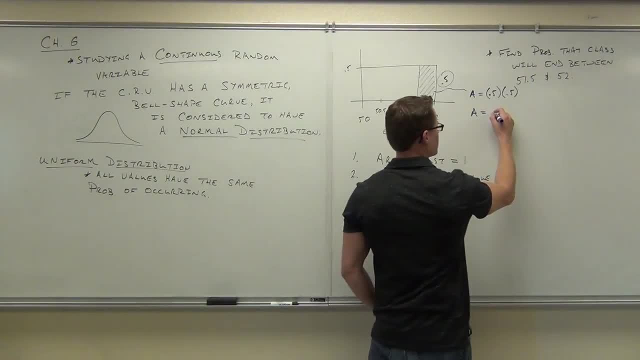 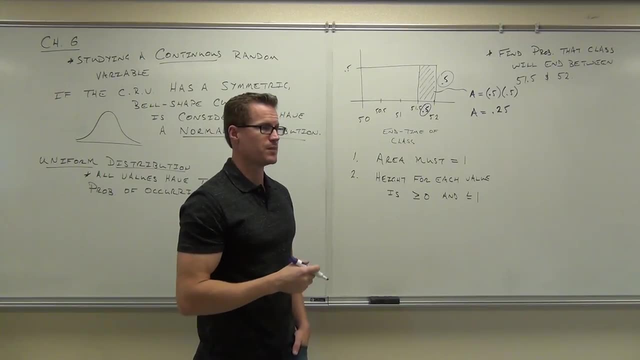 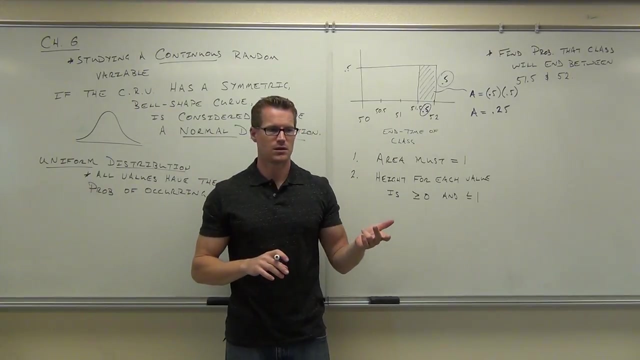 I want you to think about what .25 means. .25 is an area, true, But because the area of the whole entire distribution equals 1, .25 is also a what, A percent or a probability. That's a probability, So we can answer the question: what's the probability that our class is going to end? 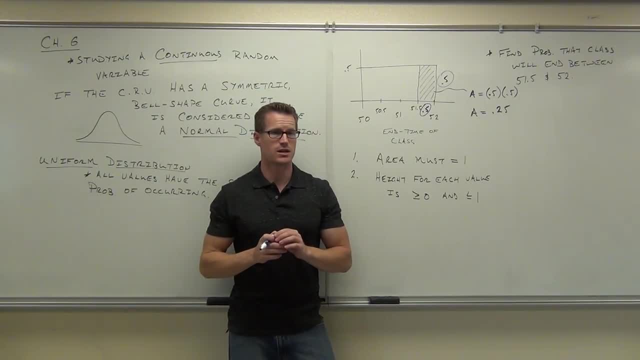 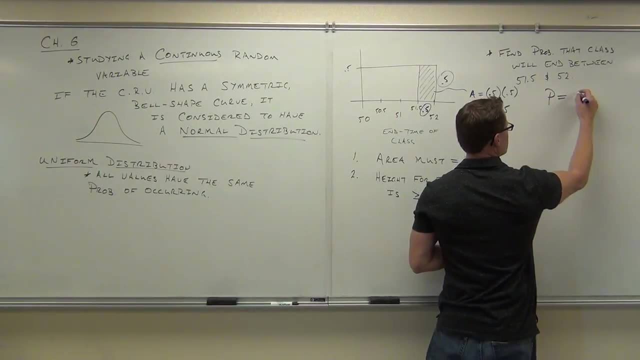 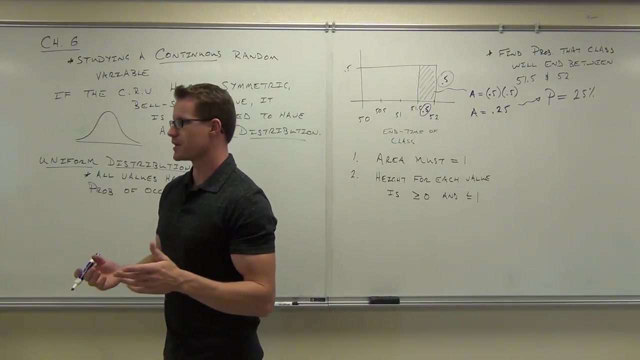 between 51.5 and 52 minutes And you say: what's the probability? .25.. .25 is the probability, So this probability here is 25%. We need to get used to the idea that the area and the probability are one and the same. 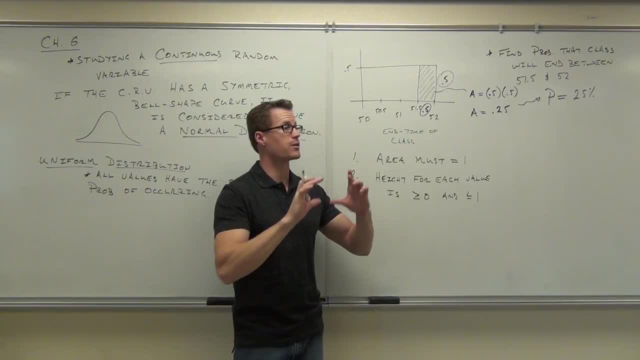 If you have an area equal to 1, you can associate it with your probability. Raise your hand if you're understanding that concept. By the way, you could have 25% for each one of these four segments. Do you guys see that? 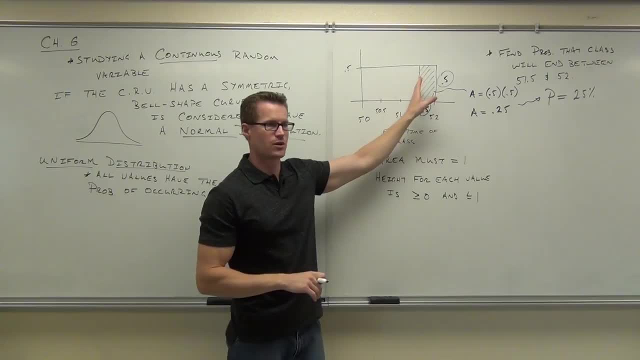 So altogether they do equal 100%, don't they? 25 for each little section. Now this is a nice start off because it's a uniform distribution. It's very easy, because it's a rectangle. We know how to find the area of a rectangle. 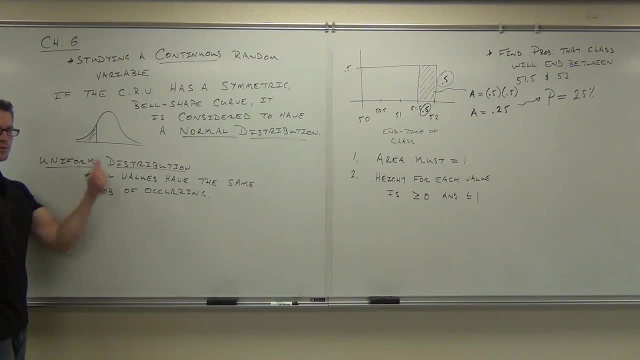 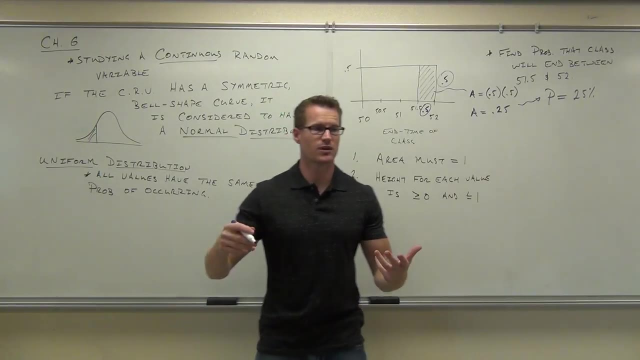 Do you know how to find the area of this? Find that area. You got it Cool, We're done with class. You all know how to do that, right? No, of course not. If you had a calculus class and you knew the shape of this curve, you knew the function. 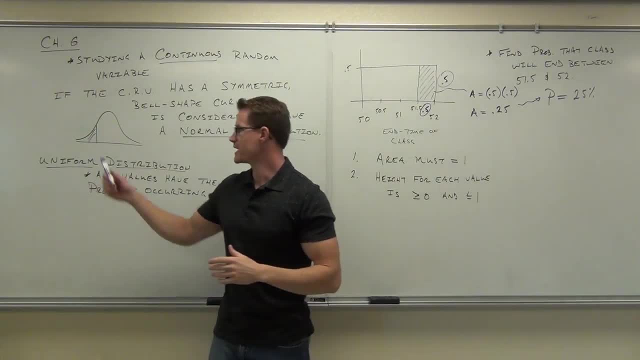 you could do it. You could do it with what's called an integral And you take it from negative infinity all the way up to negative infinity, All the way up to this, to that number, and you integrate that. But we don't have that. 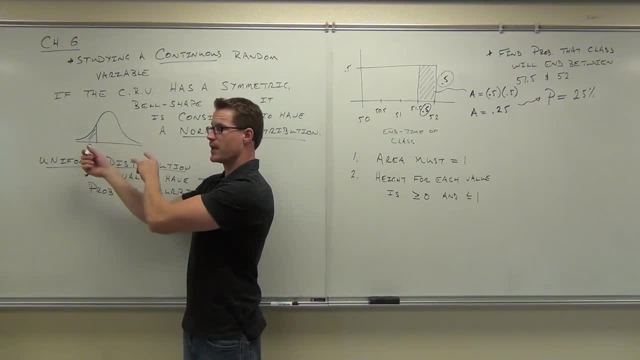 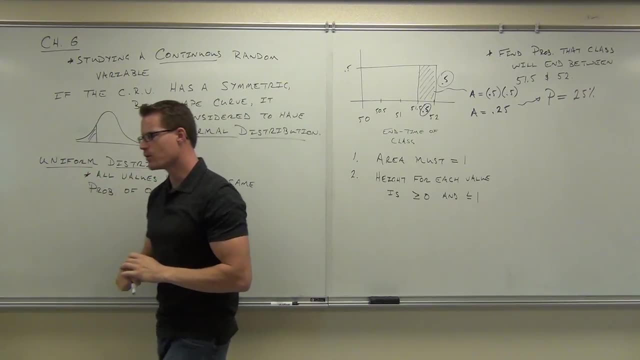 Fortunately for us, some has taken a look at this distribution and already calculated all the possible probabilities, for that Isn't that kind of cool And have a formula for that. So that's kind of nice And we'll look at that in a little bit. 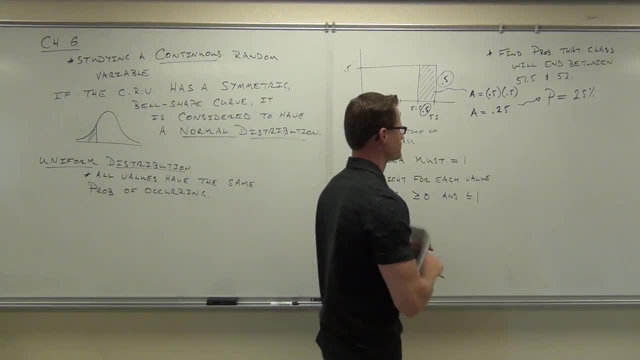 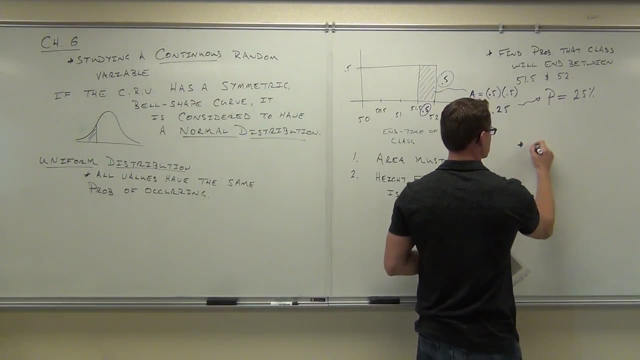 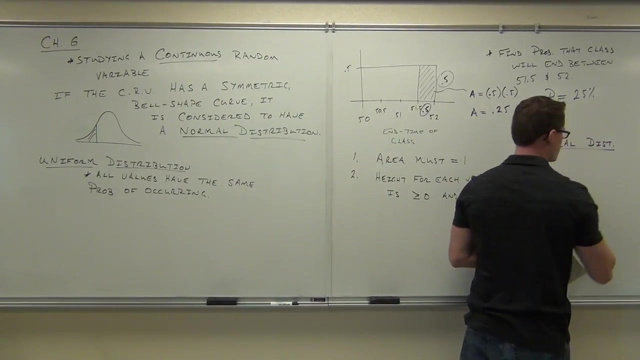 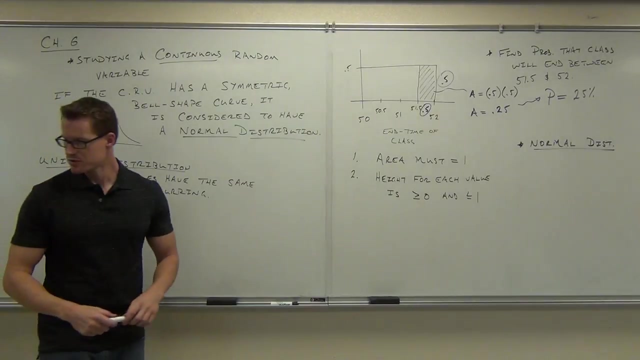 Before we get there, though, we got one more thing to talk about, And that's this: Normal distributions. Wow, most of the rest of our class is going to be spent talking about normal distributions. Here's what I need to tell you, though. 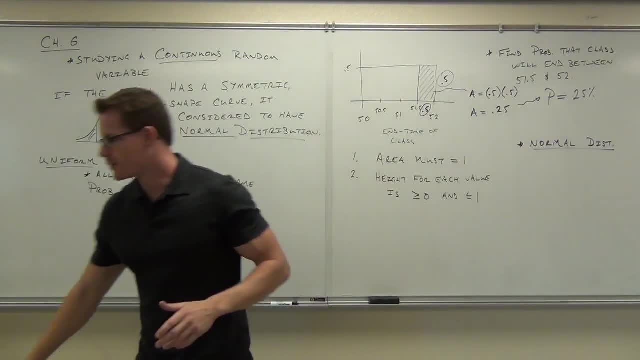 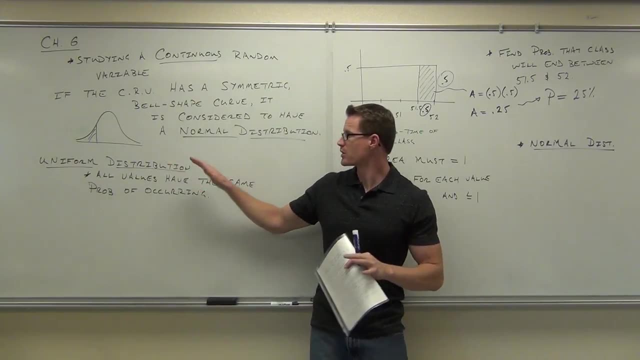 When we talk about normal distributions, we're talking about geez, an infinite number of different shapes here. I want you to think about this. Now, all these shapes are going to look very much like a bell-shaped curve. All right, 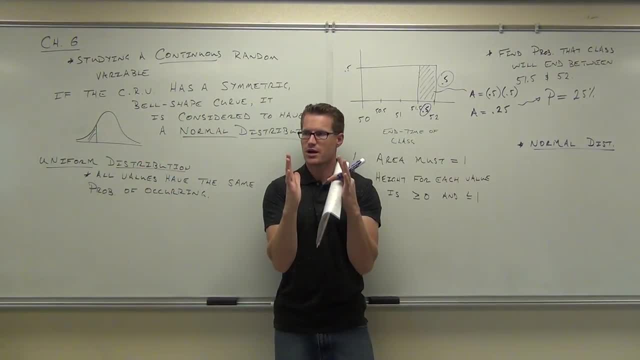 But we can squash those bell-shaped curves And we can widen out those bell-shaped curves. For instance- let me give you an idea about this- If we can compare the average height of women to the average height of men, who's taller? 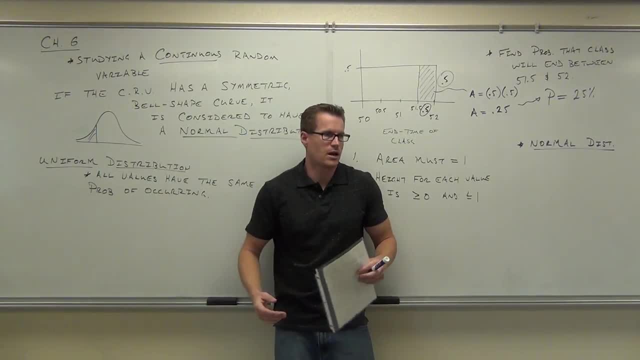 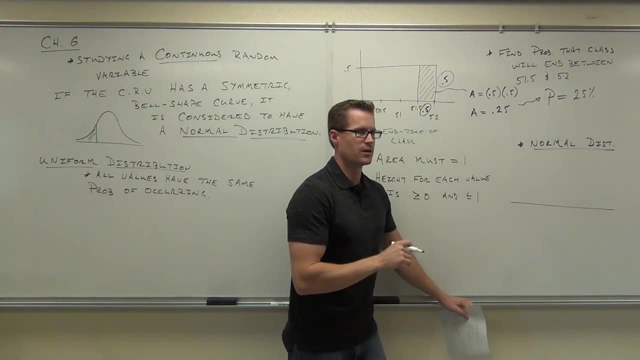 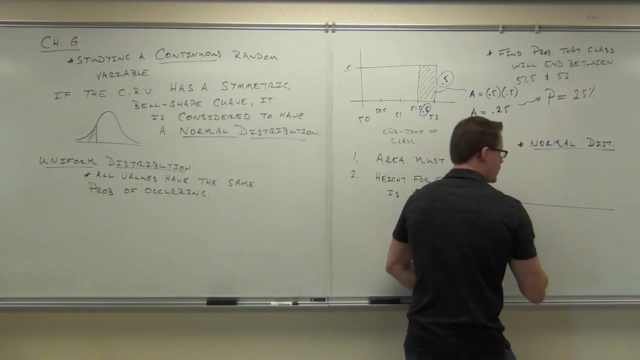 men or women on average. They're generally, on average, taller. So if I were to graph the heights of men and the heights of women with their normal distributions on the same number line, say, We'd get This for- oh, by the way, the standard deviation. 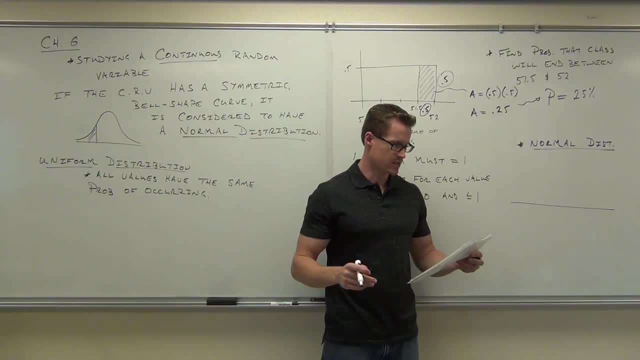 Here's the means of the standard deviations: Women have an average height of 63.6 inches, standard deviation of 2.5.. This is for a certain population, And men have an average height of 69 inches, with a standard deviation of 2.8.. 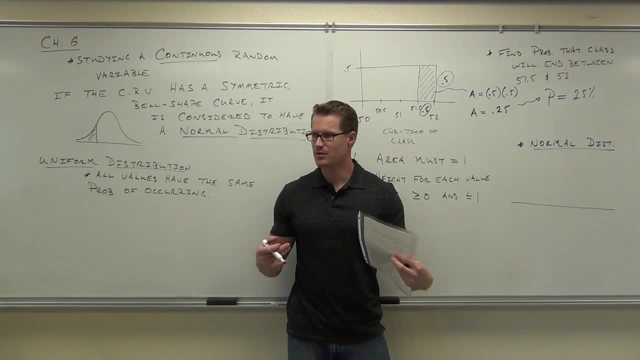 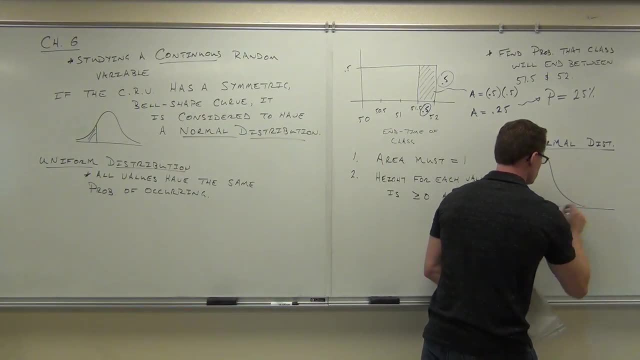 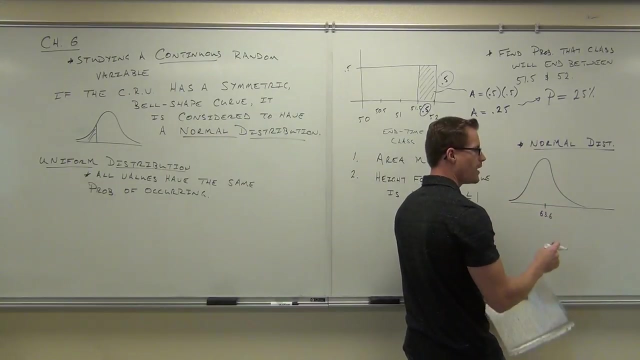 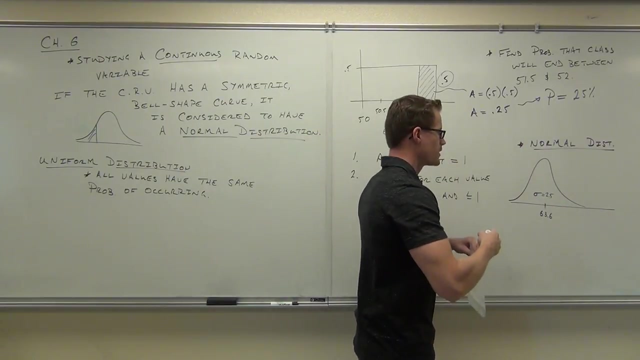 The standard deviation tells you how spread apart your data is. Remember talking about that. So if I have women with a 63.6 average And a standard deviation of 2.5, my data would look like that if I graphed the men right. 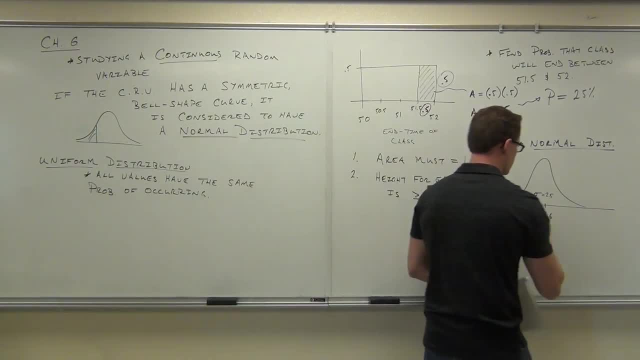 on top of this, Men's average is- what did I say? 69?. That means their peak is going to be slightly over. Do you see what I'm talking about? Their standard deviation is 2.8, which means that it's going to be slightly wider spread. 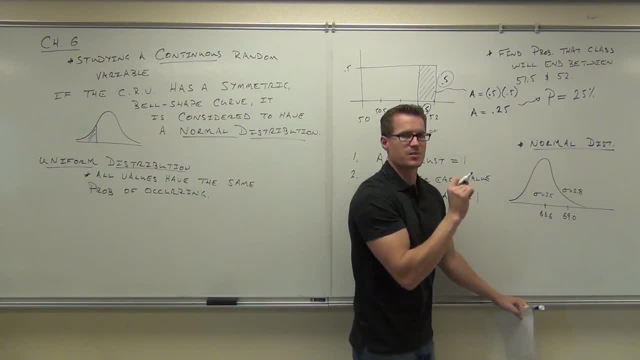 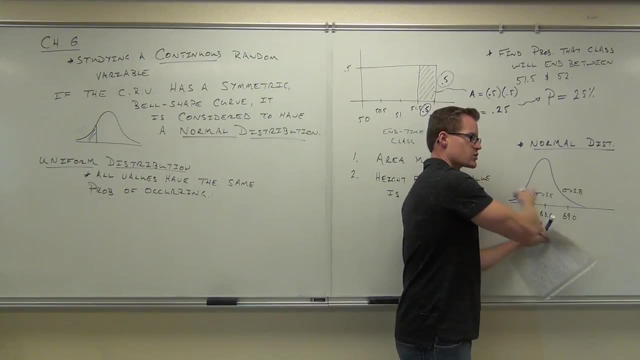 So this peak isn't going to be as high. Notice that the peak, by the way, is the number of people that are really close to that, So the peak is not the 63.6.. That's just where the mean is. 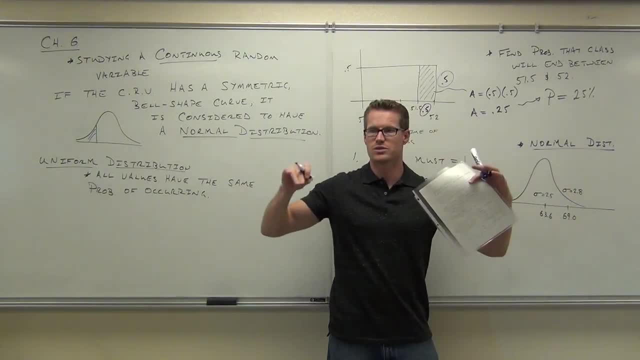 The 69,. that's just where the mean is. The distribution is how those data are gathered. If you took everyone in the world and plotted them on a graph with their heights and tallied them up, Then we'd have The most people around 69.. 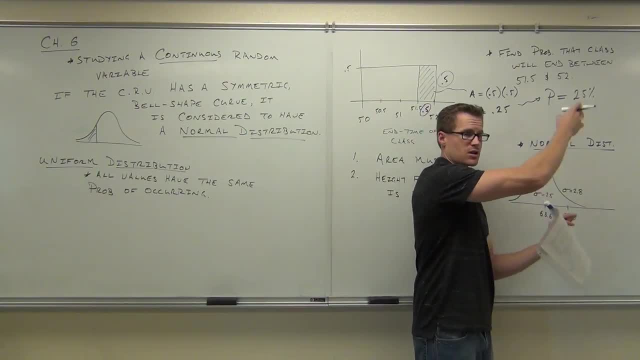 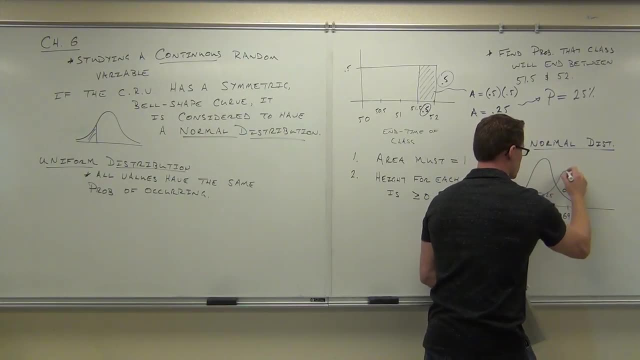 The most women around 63.6.. That's where those heights are coming from. So here our graph would be a little bit shorter, a little bit more spread out. It'd look like this: Oh wow, Not even close. 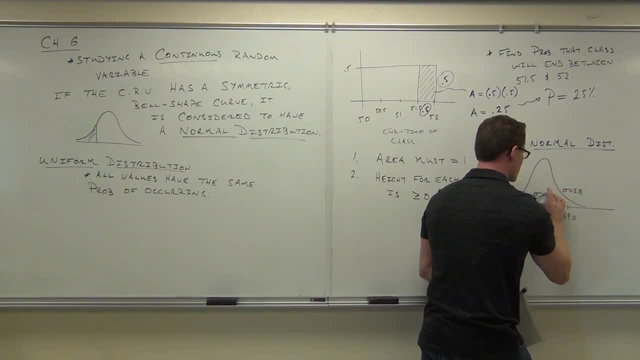 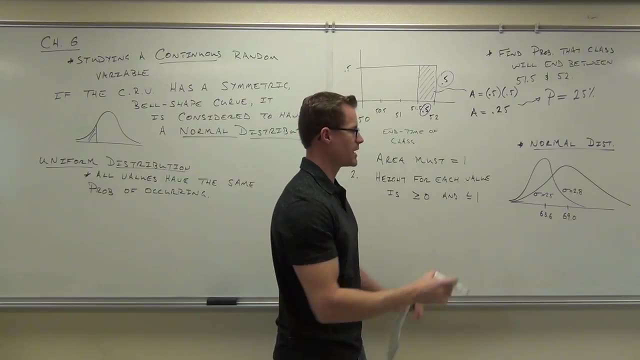 That's horrible. Let me redraw. It's trying to be all cool and stuff. Now I've kind of emphasized the spread outedness. That's not even a word of this graph, But I want you to really see the picture. 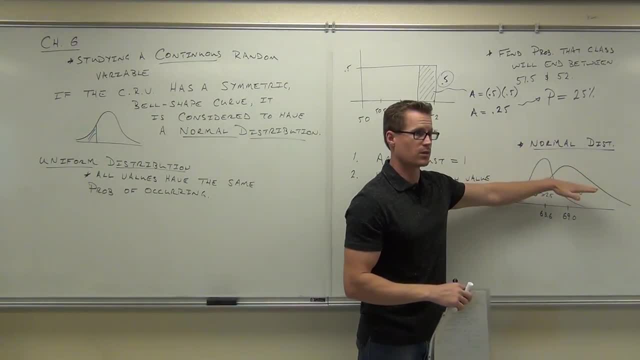 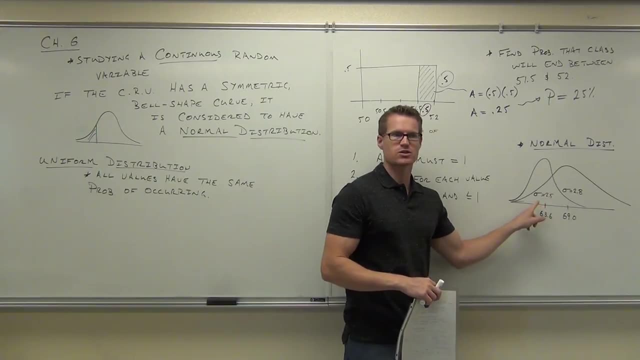 So the height of the graph a little bit lower. There's less people around that 69 because they're more spread out. They're a little bit more spread out than this. one is Not sure if you're following this example here. Okay, 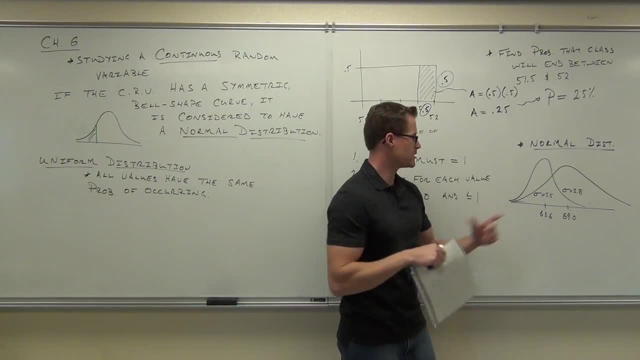 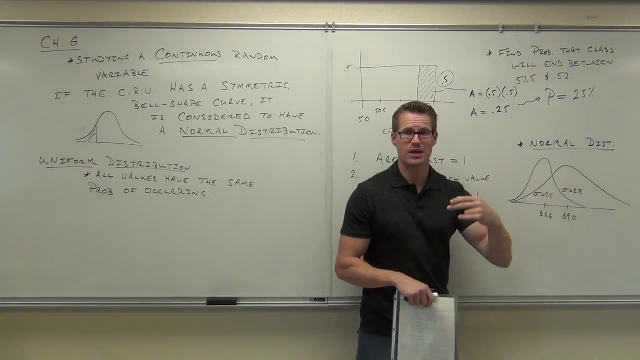 So standard deviation says how close we are to the mean. This one is closer than this one is. The average themselves are different. So this graph is not exactly the same as the women's graph. Even though we have two normal distributions, They're both normally distributed. 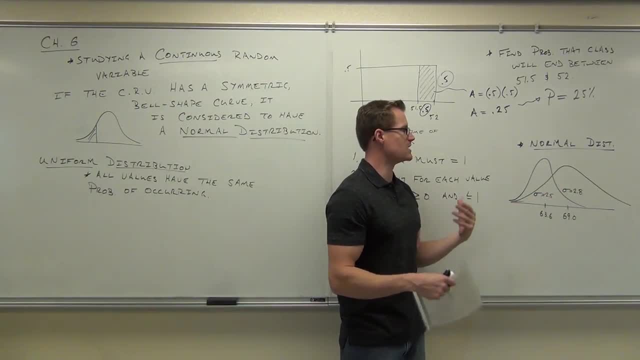 We have a different shape. In fact, with every different situation You're going to get a different shaped normal distribution. You with me on that one. So we're going to have tons and tons of normal distributions. And the person who kind of first thought of this said: wow. 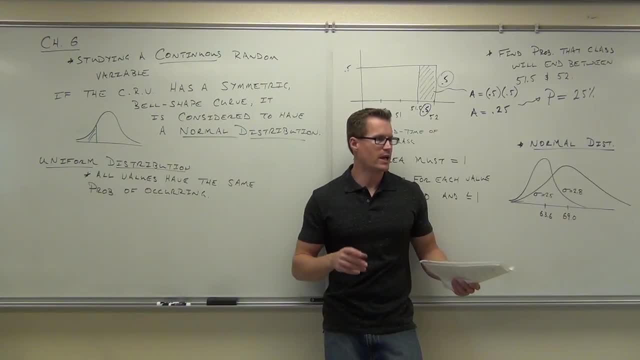 You know, if we have so many normal distributions, We really should have a way to unify them, To make them standard. Standardized Standardized means: take this stuff, Put it on the same scale, basically, Isn't it? That's why everyone in the United States pretty much takes a standardized test in high school. 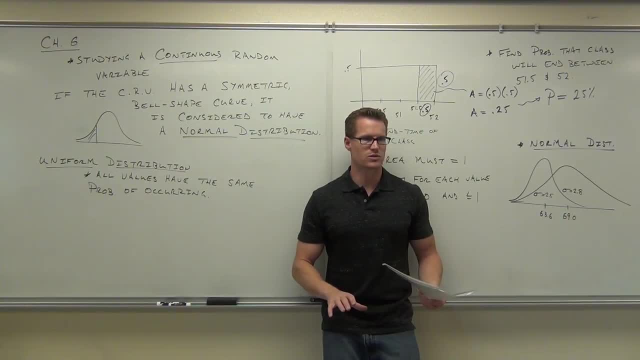 Haven't you taken a standardized test before? If you were in high school you probably did. You took this one test that everyone else takes, Right To put you on the same scale as everyone else, To see how you compare to everybody else. 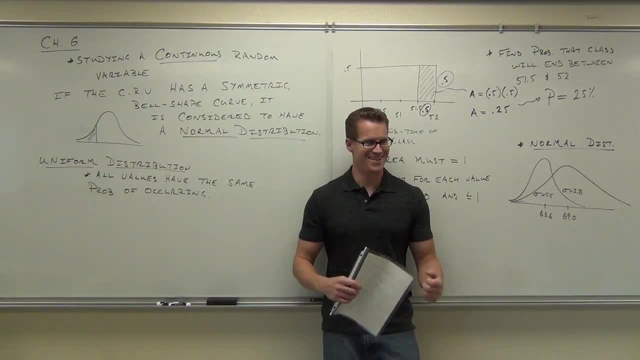 Sometimes it's kind of depressing, Sometimes it's kind of like: alright, Right, But the idea is, it's standard, It means everyone takes it And everyone's on the same scale. now, Well, the person who said this was like: okay. 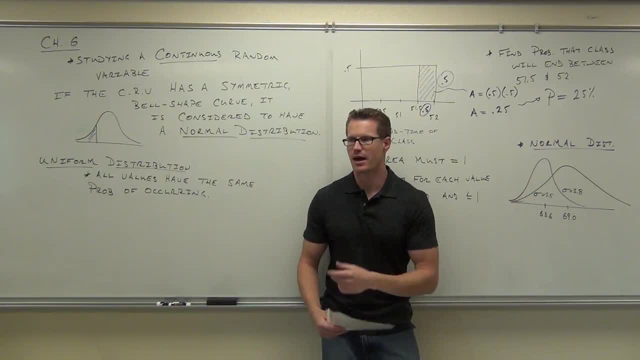 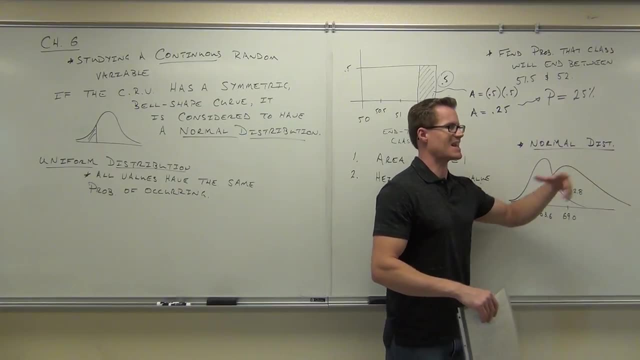 Well, that's a good idea. Let's take all these normal distributions And let's standardize them, And what that gives us is a standard normal distribution. These are all normal distributions: One, Two, Three. There's like an infinite number of them. 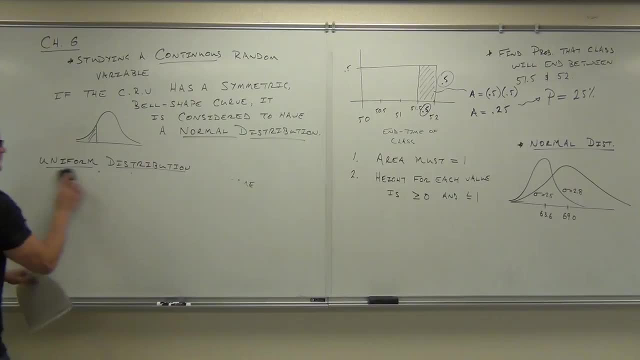 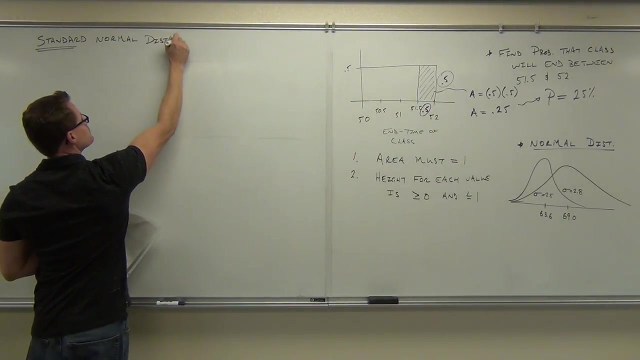 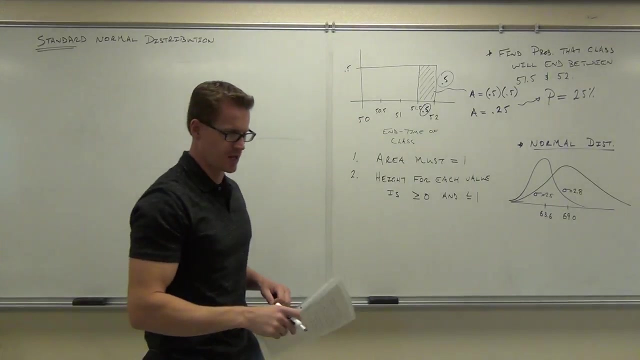 We have an infinite number of situations. What we do now is we have a way to standardize them by using the standard normal distribution. Here's what the standard normal distribution does. It's like a standard normal distribution. Standard normal distribution simplifies our distribution. 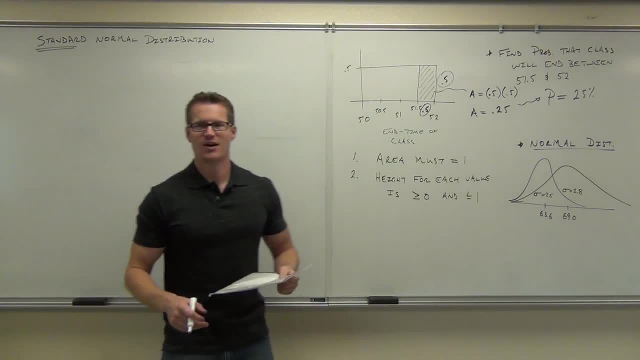 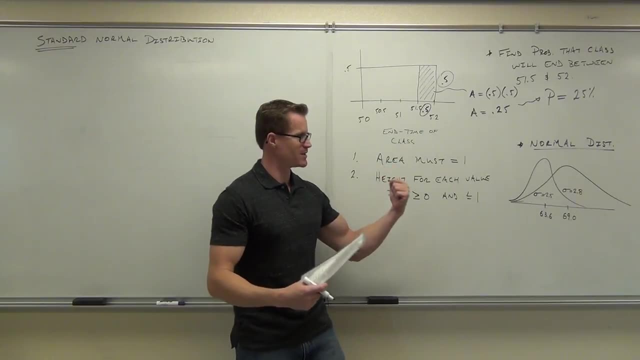 Simplifies the differences between these distributions. It's like the uber distribution, Like the ultimate distribution, It's like the man of man, the woman of woman type of distribution. It's not this one. It's not this one. It stands for all of them. 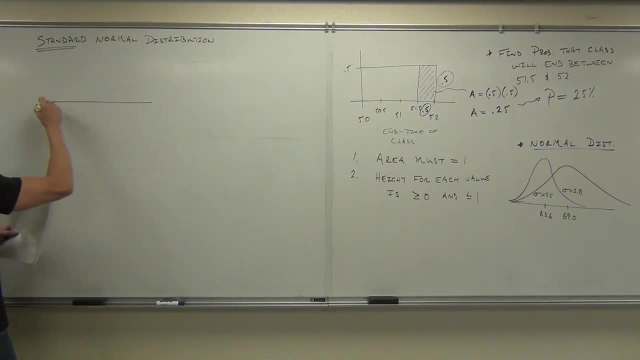 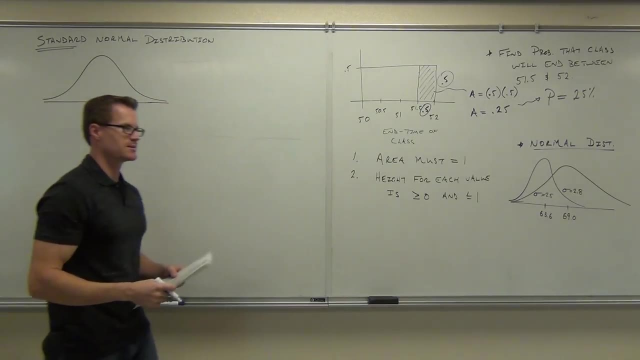 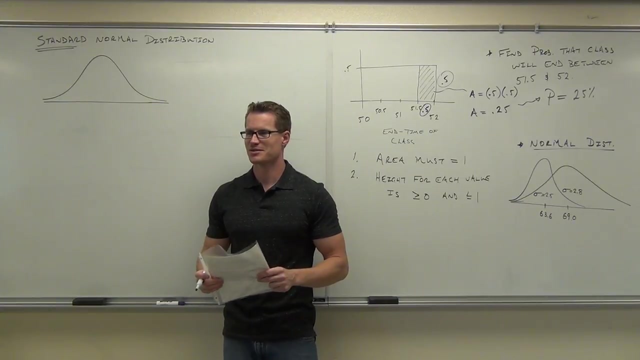 It's awesome, Looks cool, Smooth. It was a person who owned a yacht. It's kind of out there, No, like that one guy who does the Dos Equis commercials. Yeah, that guy, It's that guy, All right. 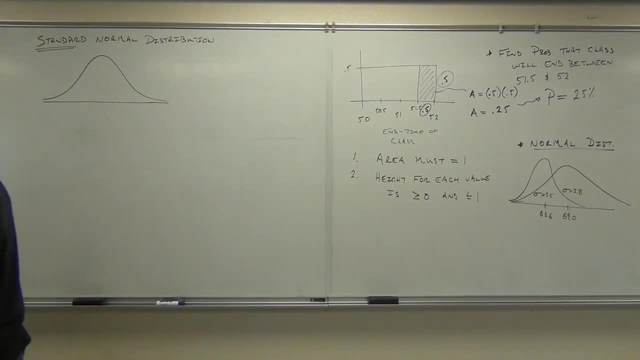 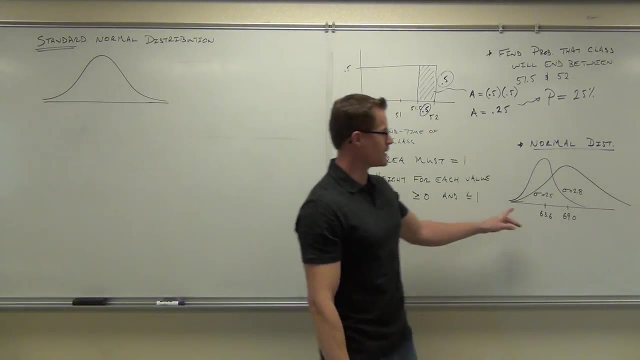 The most interesting distribution you've ever met. Here's how the standard normal distribution works. It says, yeah, all these means for a different distribution. for every situation you would ever encounter, which is an infinite number of them, You'd have a different mean. 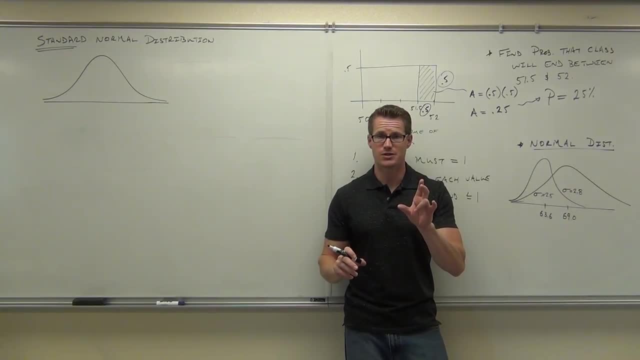 Follow. Or if you didn't have a different mean, you probably had a different standard deviation. So somehow the spread of the day is going to be different, The means are going to be different. You're going to get these different shapes and different distributions for everything. 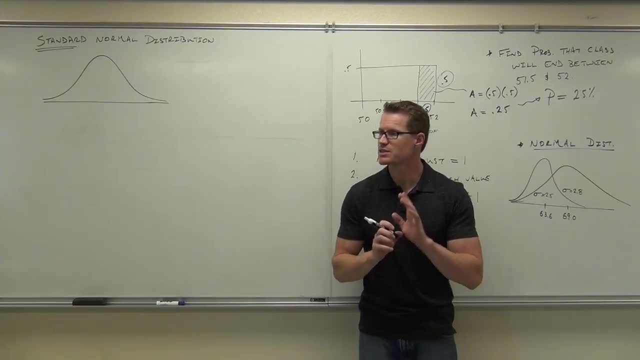 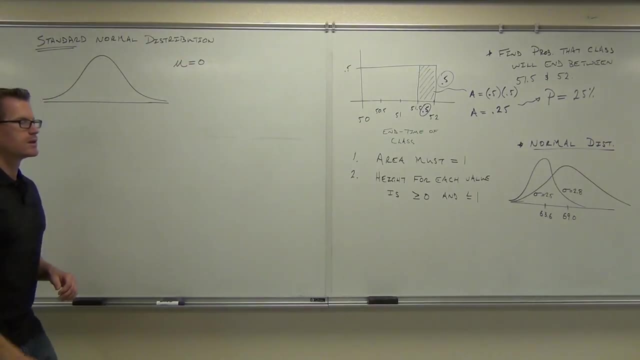 you ever have You follow. So here it says this: I'm going to simplify it by forcing the mean to be equal to zero- That's kind of cool- And the standard deviation to be equal to one. Okay, I'm also going to simplify this by forcing the mean to be equal to zero. 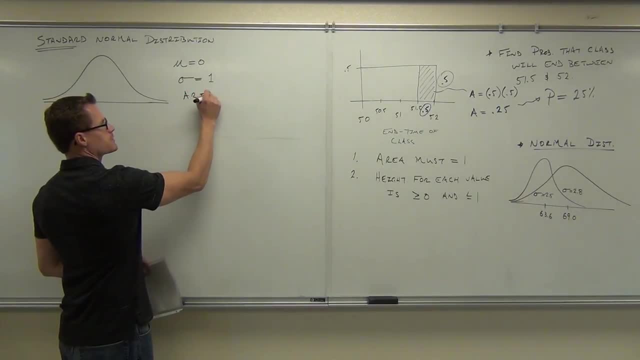 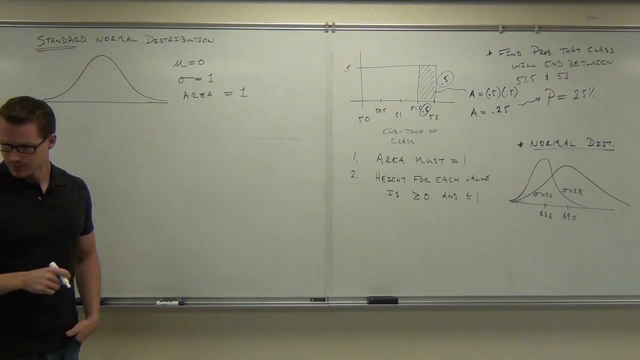 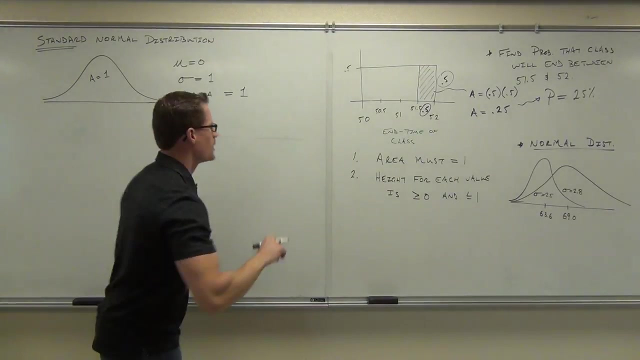 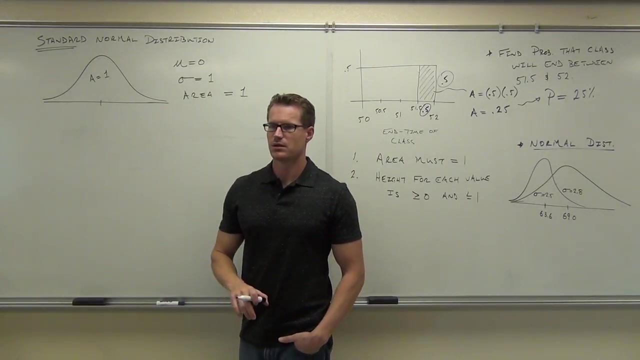 going to force this. I'm going to force the area under the curve to equal one. so the area equals one, there equals one. can you tell me what's the value right here? have to be how much this is this value right here, under the peak of our 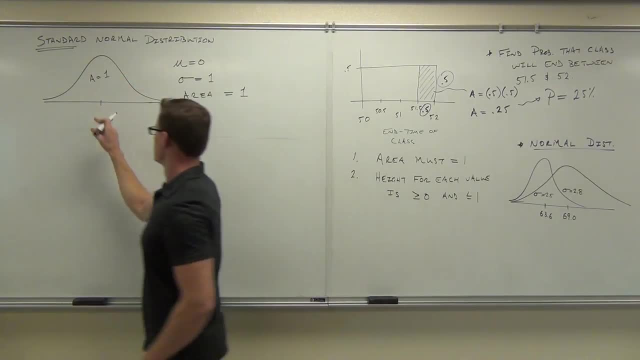 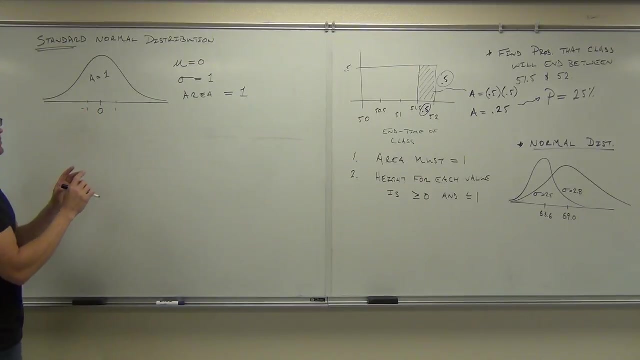 distribution is the mean. how much is our mean means going to be zero, okay. and the standard deviation? standard deviation is equal to one. so over here we have always going to bring up some old concepts here for you. can you please tell me what percentage of the data is between these two numbers? oh, you should know it, you. 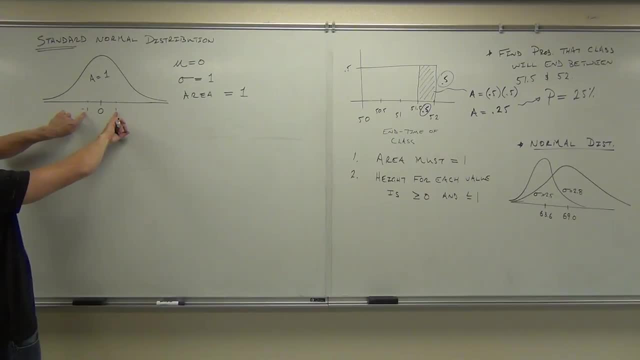 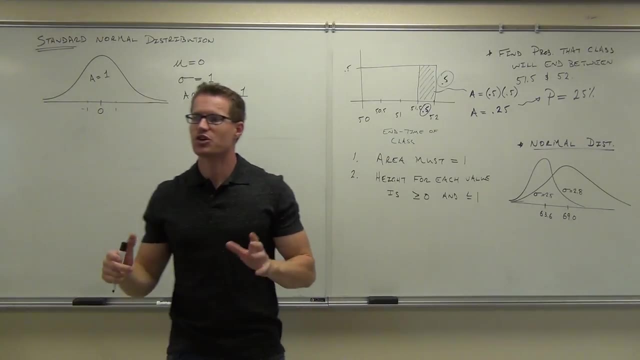 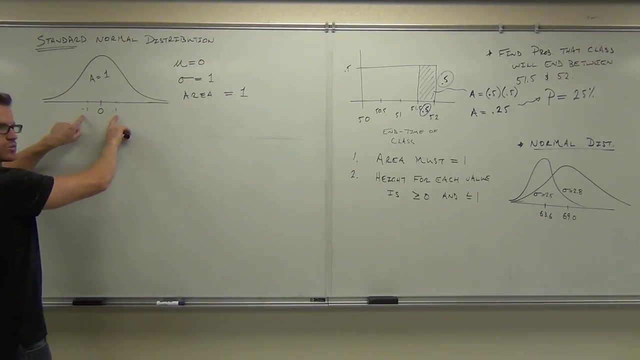 should know it. you got to know it. point there, not point zero five. this is one standard deviation, right 68. this is so cool because our standard deviation is now equal to one. you can just go okay. what's the percentage of data between here? well, this is one. 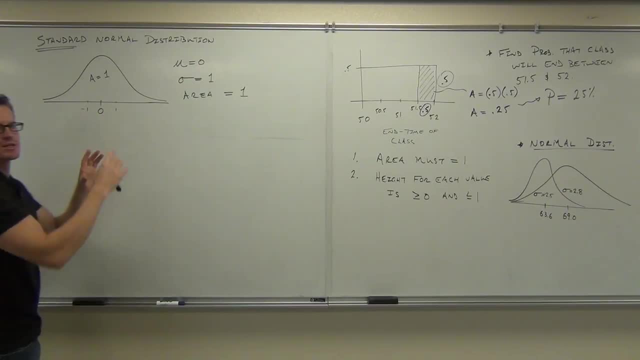 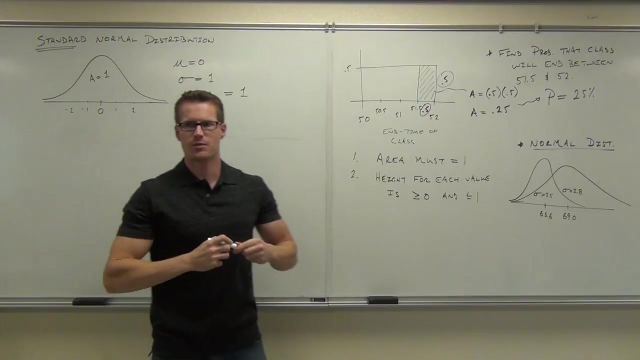 standard deviation to the right and one standard deviation to the left of the mean, that means 68% is going to fall within that range of numbers. yes, no. if I go out one more, two to negative two, what percentage of the data is going to fall between two and negative two? 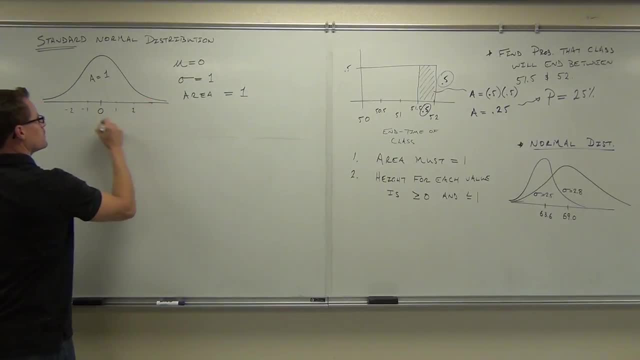 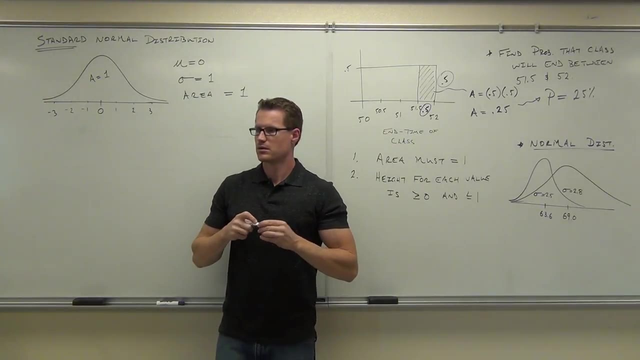 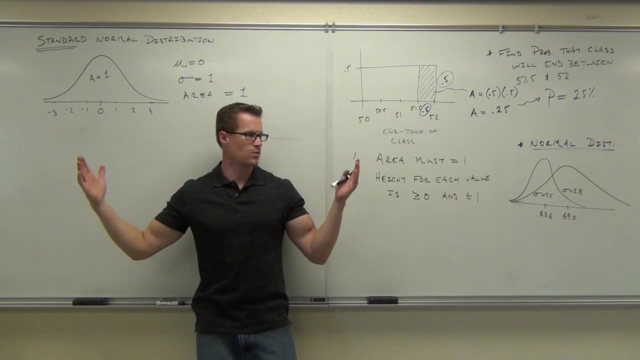 good if I go out one more. what percentage of the data is going to fall between there? 99.7? are you starting to see why I have to make the area under the curve equal to one? I told you the empirical rule a long time ago, right? 68? 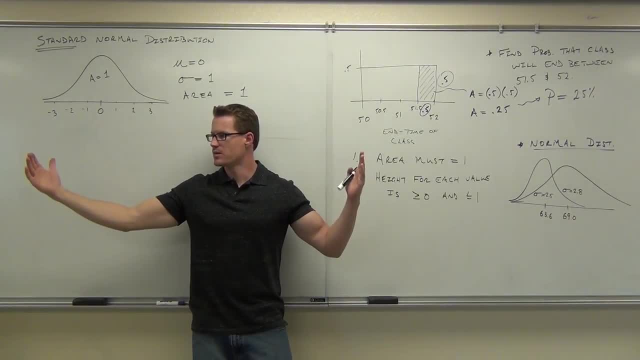 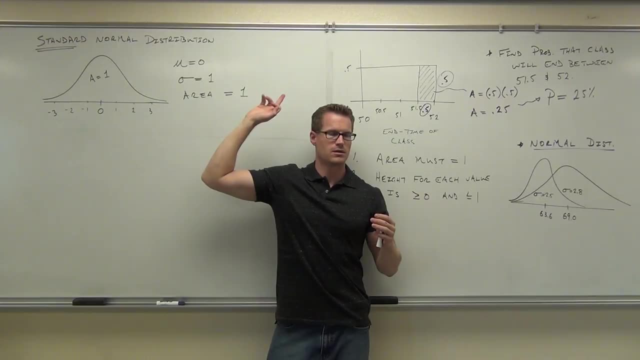 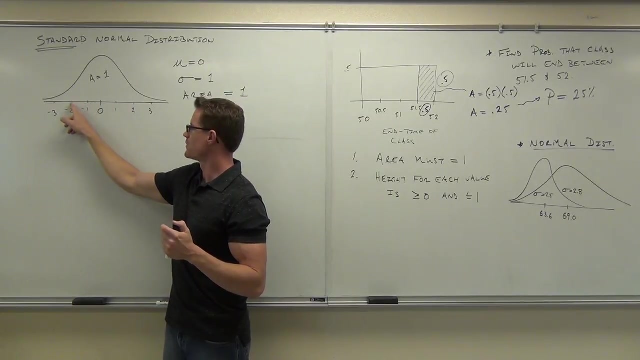 percent falls here. ninety-five percent falls here. point nine five, ninety-nine, point seven: point nine nine seven falls between these ranges. how much falls between negative infinity to infinity? you got to know it, you know how much falls between these two numbers. how much falls between these two numbers. how much falls between these two numbers, how much. 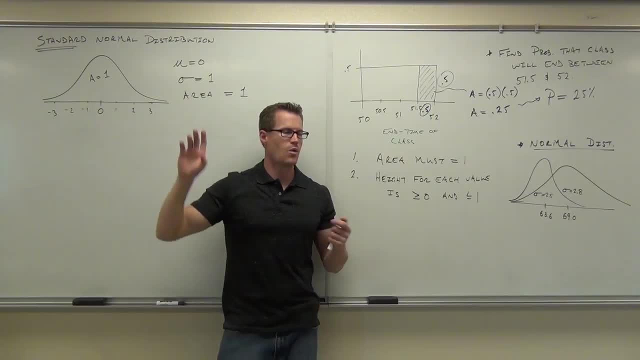 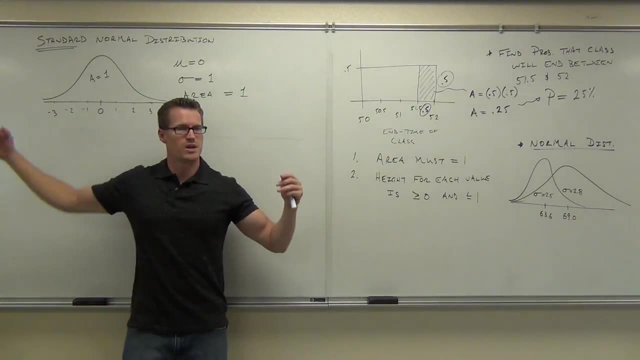 falls between everything. what's the whole area one? so if I go to negative, this curve never ends. right, it's really really small, but it never ends and never ends this way. so how much is from negative thing to infinity? you have one. a hundred percent of the data is going to be between that range. raise your hand if. 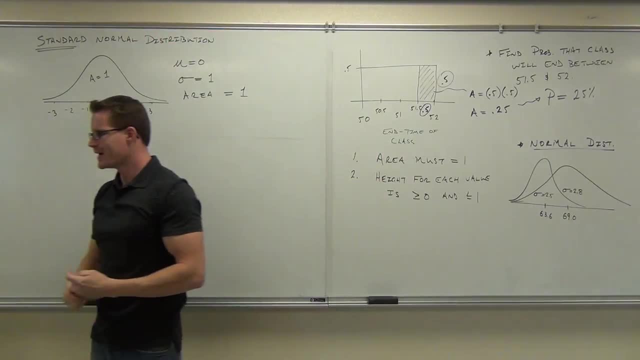 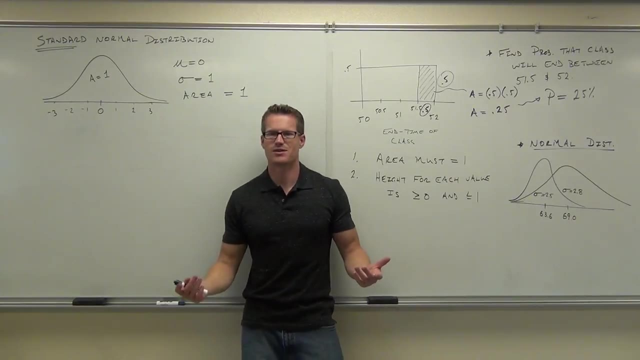 you feel okay with that. it's new for you, right? it's kind of a new concept. now here's the problem: how in the world do we change this stuff into this? because you're thinking: well, this, only this is very specific, right, who has a mean of zero and a standard deviation of exactly one? I'll say, well, 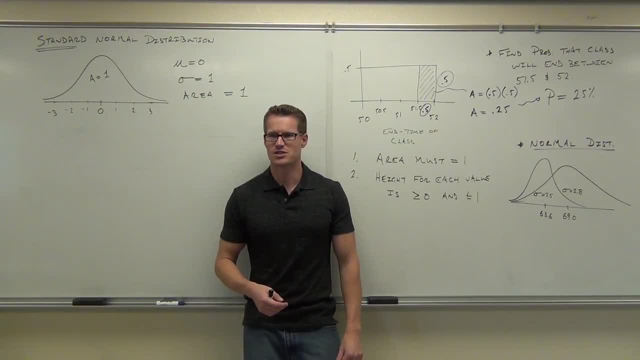 thermometers, but that's just. it's kind of specific. we don't want to just deal with thermometers. thermometers have a mean of zero because the freezing temperature of water for Fahrenheit is zero, right, so their average would be a zero and their standard deviation is: it's actually right about one, so never. 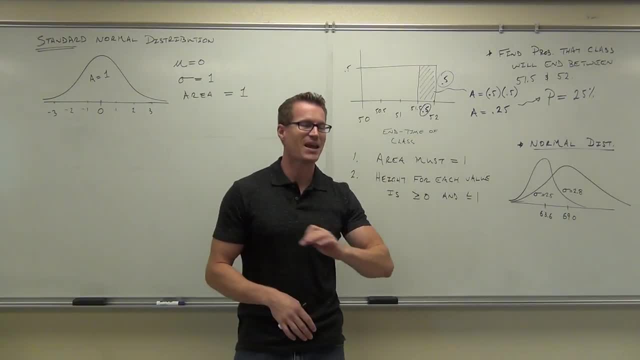 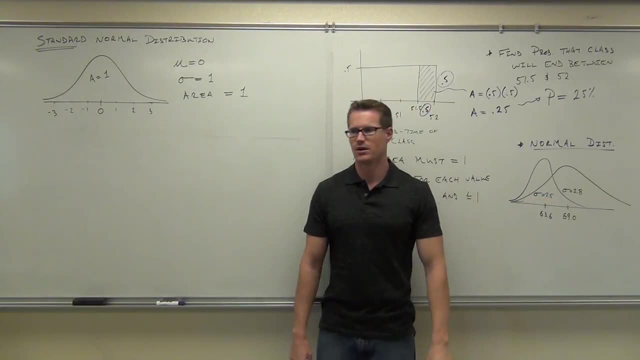 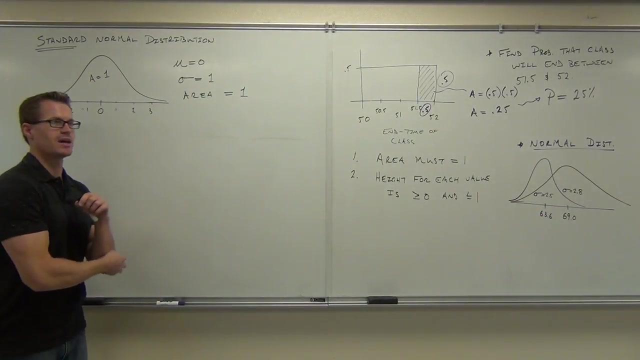 mind. I'll use the example a little bit. it's kind of interesting, but not every everybody has a mean of zero. not everybody has a standard deviation, or every situation a standard deviation of of one. we need somehow to translate this to this. would you like to see how to do it? and we're gonna end there if. 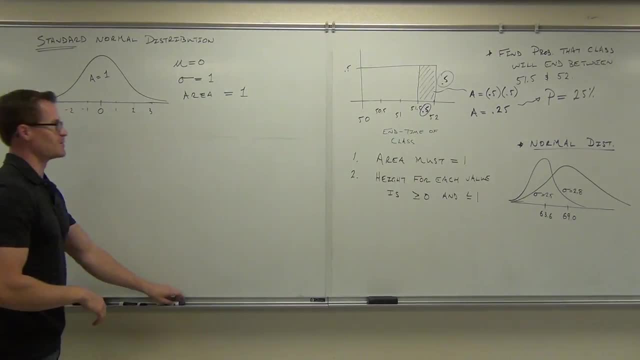 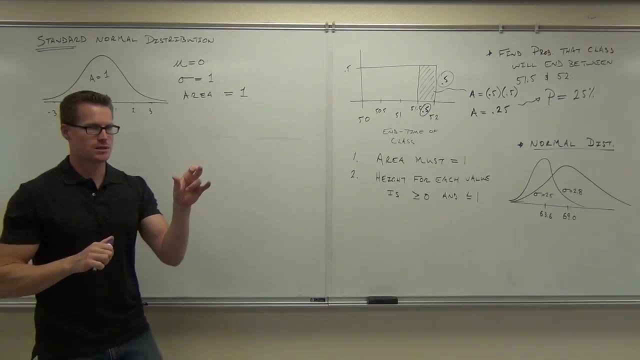 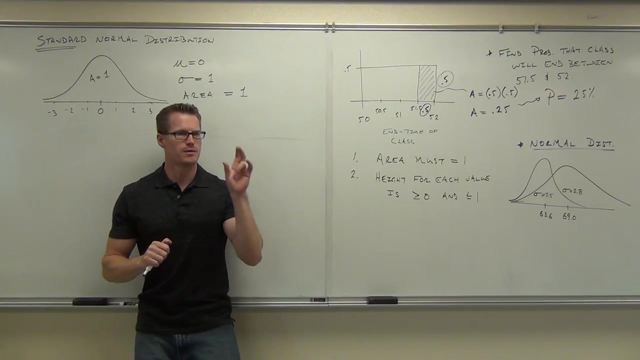 you don't want to see how to do it too bad, here's what I want to do. I want to be able to plug in the mean to some formula and get zero out of it. I want to be able to plug in the mean plus one standard deviation and get one. 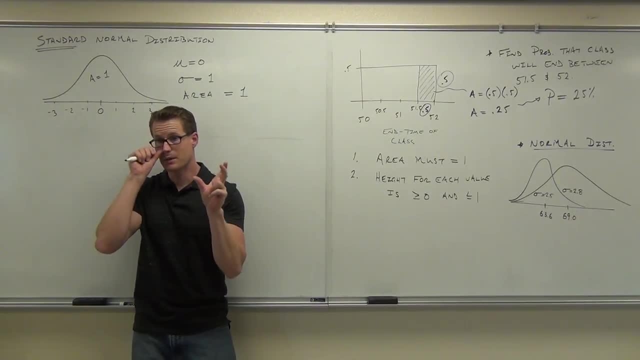 out of it that way: a standard deviation greater than the mean or less than the mean will give me a plus or minus one. two standard deviation is greater than the mean or less than the mean will give you plus or minus two. we only have something that will do that for us. if you think back to this formula just. 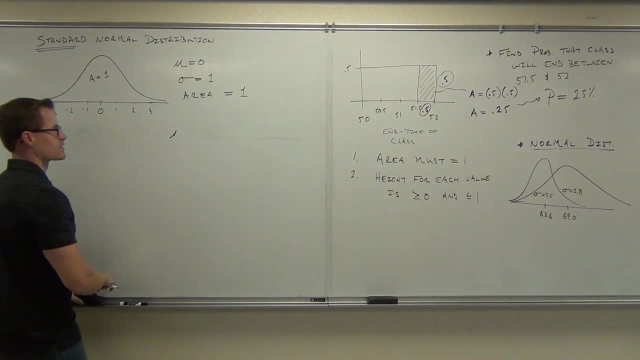 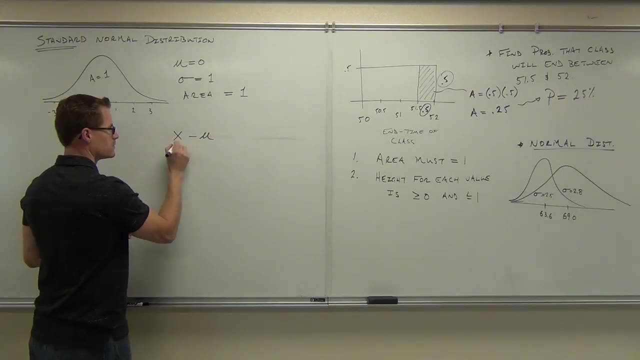 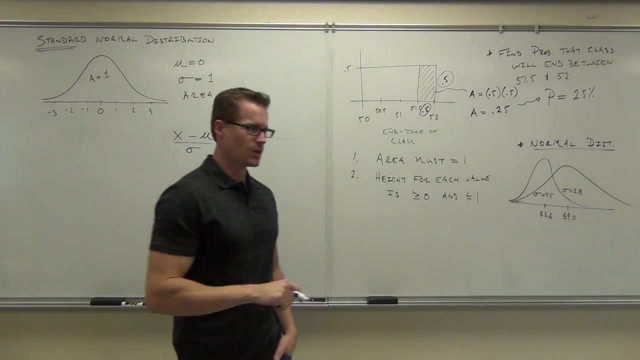 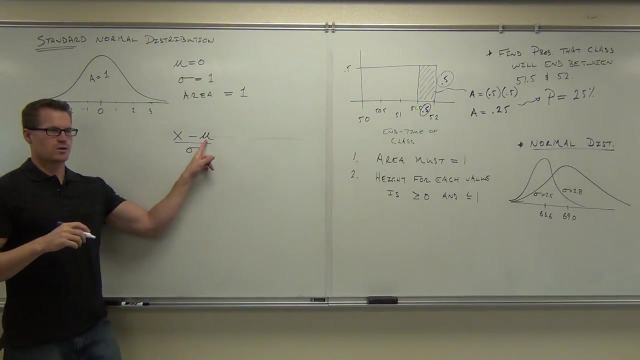 think about this for a second. I'm gonna start off back. so let's draw an X and see what happens. if you think of this formula, which you really should actually know what that formula is right now, check it out. this is your, your, what was that again? you? that's the mean. this is your Sigma, which is standard deviation. 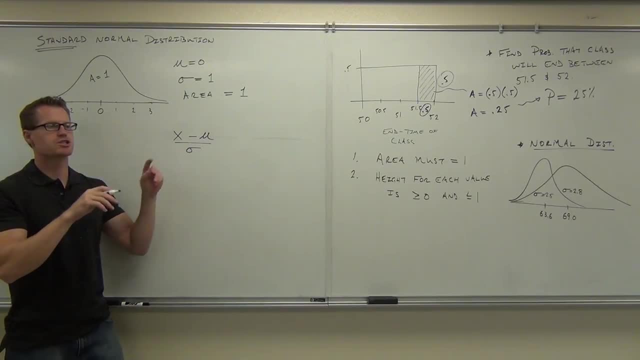 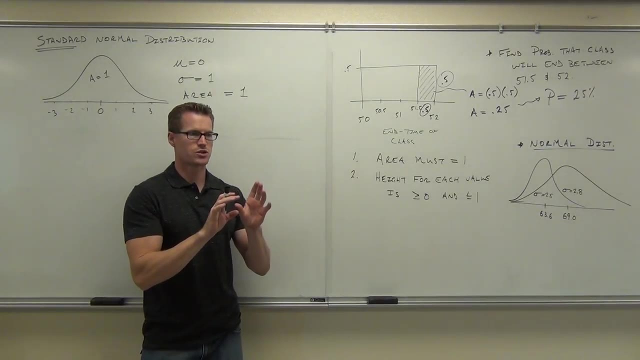 for populations: true, and X would be the value I plug in. just bear with me for a second. if I plug in the mean and I plug in the value of the mean itself, this formula should give me out a zero. true, that would map every mean to zero. you understand that every time you plug in the mean for 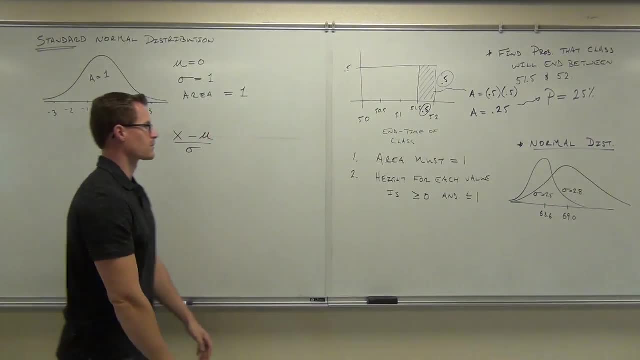 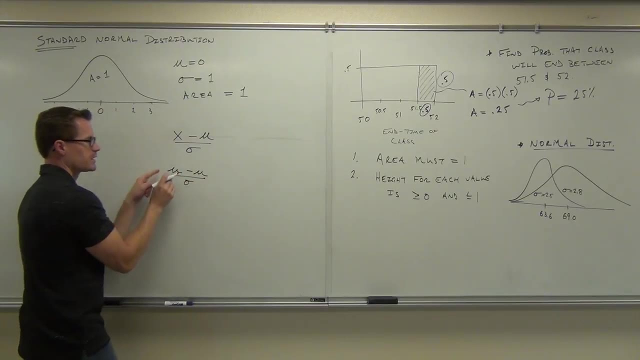 a situation you would get zero out of it if I plug in the mean. now I plug in the mean for my X value. okay, whatever the mean is, I'll show you over there in a second that this works. how much is the mean minus the mean? how much is zero over anything? this maps a mean to zero. now if we check the other, 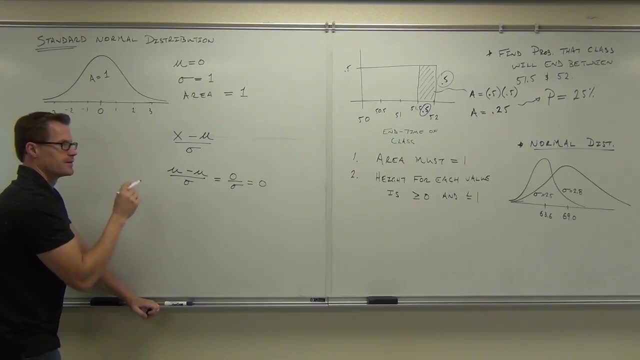 case. we're going to check that. the standard deviation: one standard deviation away from the mean. listen carefully to the wording here. one standard deviation away from the mean maps that's that value to a value of one. two standard deviations away from the mean maps it to two, three standard. 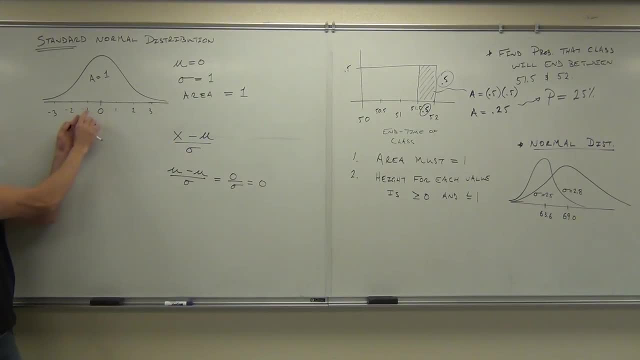 deviations away maps it to three and vice versa. one segregation to left maps it to negative one and negative two and negative three. let's check the first one. if I want one standard deviation away from the mean, well, that's this. that's the mean plus a standard deviation do. 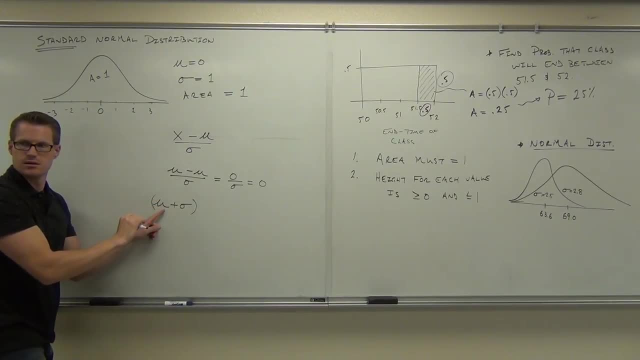 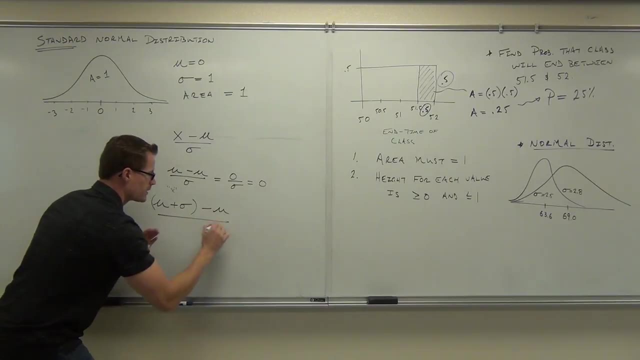 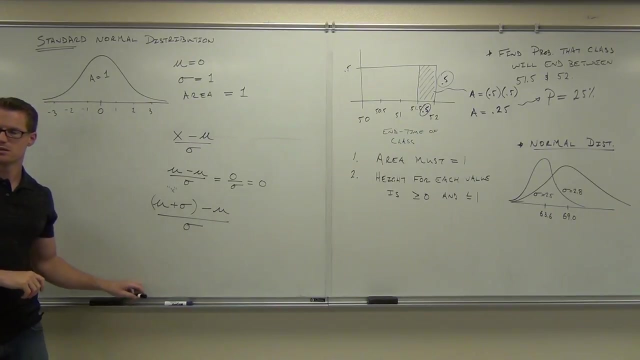 you agree that this is one standard deviation to the right of the mean. okay, if I take this as my X and I plug it into this, do you see what's going to happen mathematically? do you see it? how much is it going to equal? do you think we have a mean plus Sigma minus? 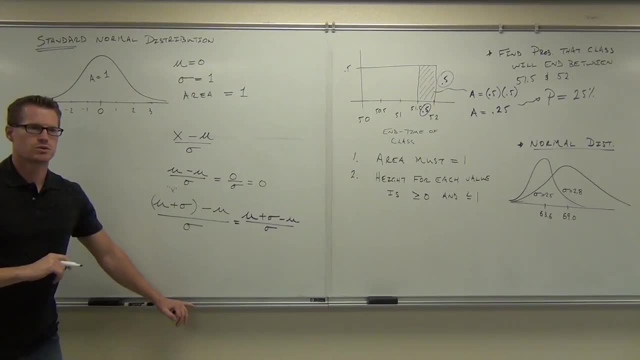 the mean over Sigma. what happens to your muse? these are gone. I get Sigma over Sigma. how much is Sigma over Sigma? okay, whoa cool. look what would happen. I'm not gonna do this every time, but look what happened. if I put in two standard deviations away from the mean, do you see that I would get out of two? put in three. 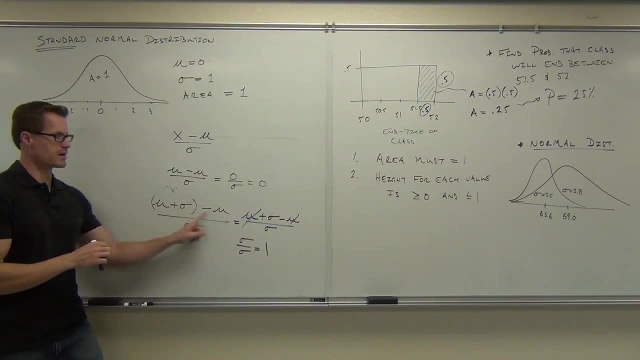 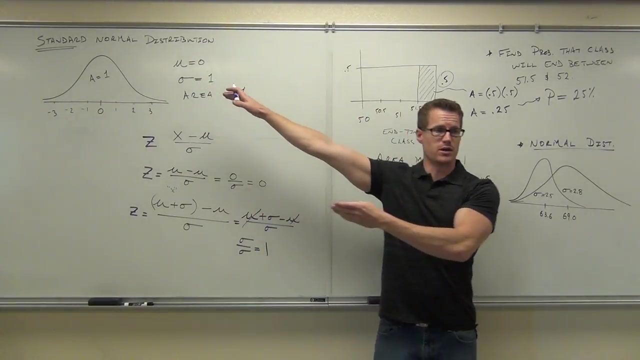 standard deviations, I get out of three. if I put in minus one standard deviations, I get out of negative one. minus two standard deviations, I get out of minus two, and so forth and so on. this, which we've already had, will map every normal distribution into a standard normal distribution for you. isn't that kind of cool. I want you. 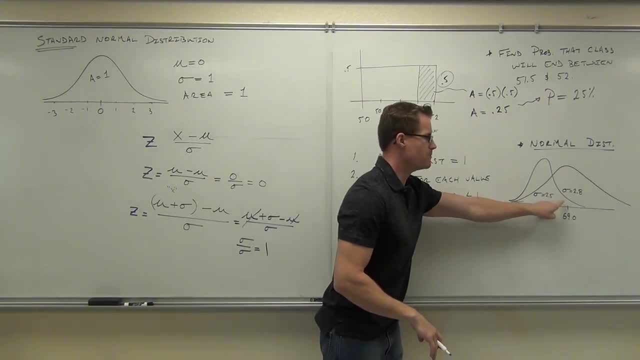 to see it in a real-life example that this actually works. let's take the the men's heights here. I'll take the men's heights here. I'll take the men's heights here. I'll show you that when you plug in the mean to the z-score, you get zero. when you plug. 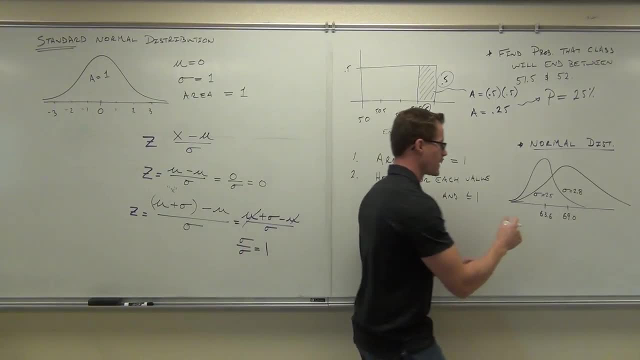 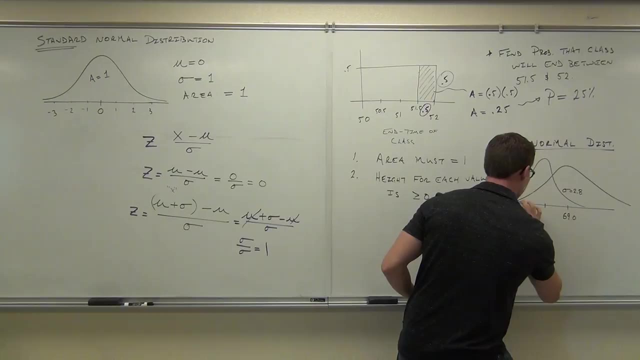 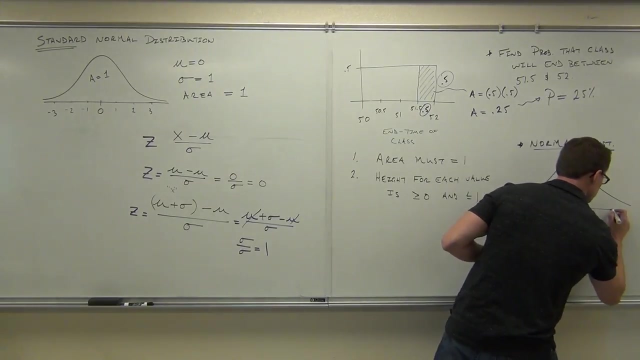 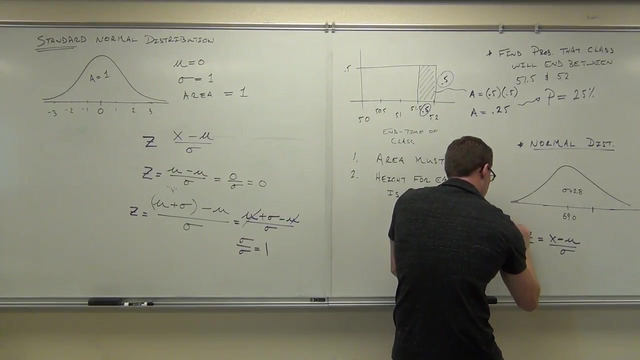 in one standard deviation to the right, you'll get one. okay, check this out. let's erase the women here some. while I'm doing this, can you give me one standard deviation away from the mean, please, and we're going to plug in the z-score. I'll write this over here: 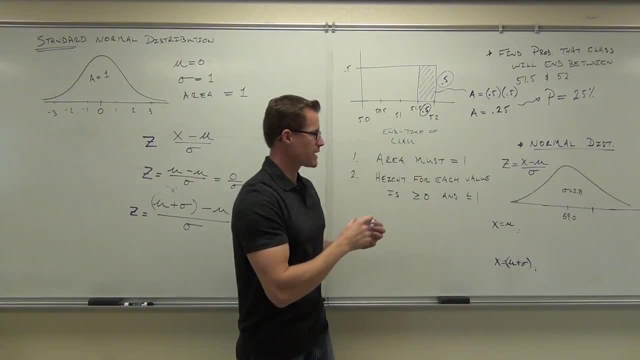 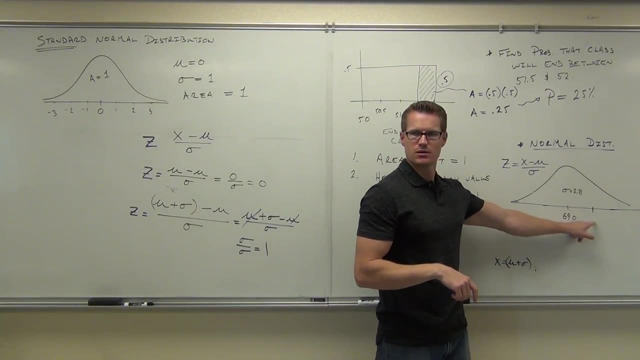 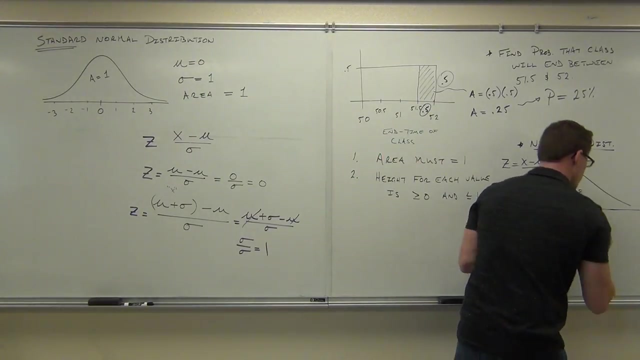 so Z equals X minus mu over sigma. that's the same old z-score that we've always had. how much is this one standard deviation from the now? all I'm showing, all I'm showing to you right now, is that this is actually true for any normal. 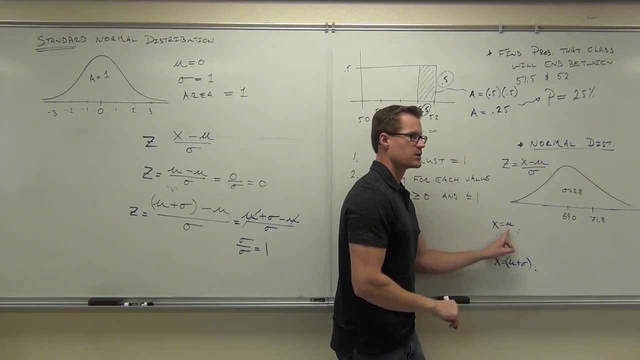 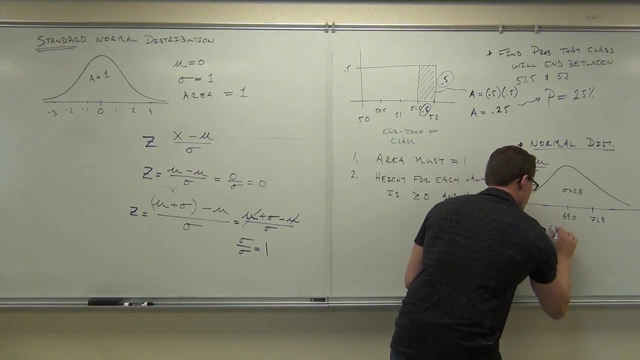 distribution. if I plug in instead of X, if I plug in the mean, which means I'm taking my value right here in the middle, watch what's going to happen. the z-score would be 69.0. that's the X in this case. not sure if you're okay with that, that's. 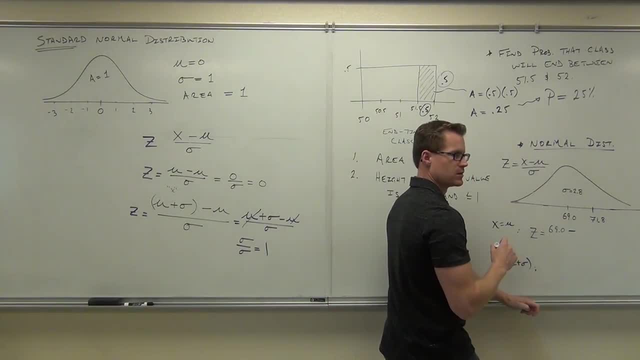 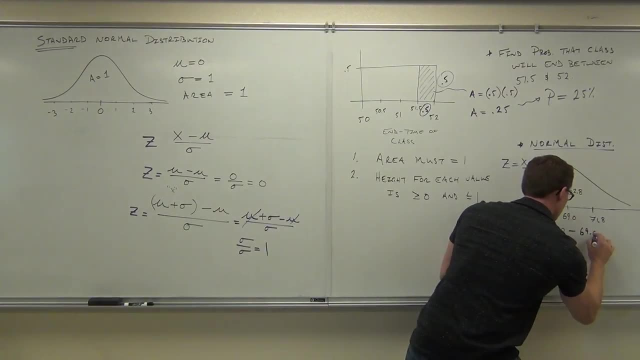 the X minus the mean. what's the mean? okay, over this. what's the standard deviation? okay, come on, quickly, run out of time. yeah, talking here. what's the 69 minus 69 over 2.8? doesn't really matter, because you're going to get zero out of it. what? 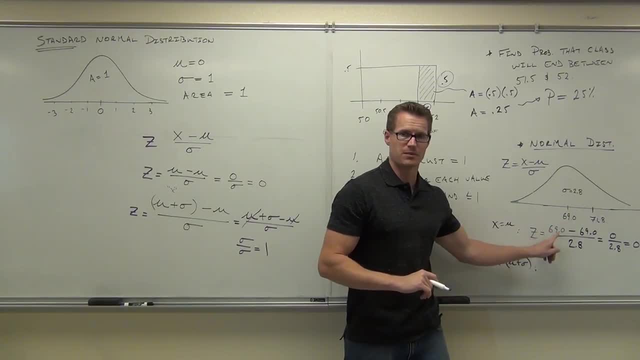 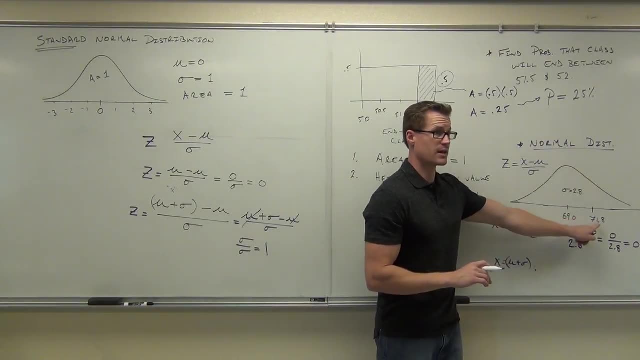 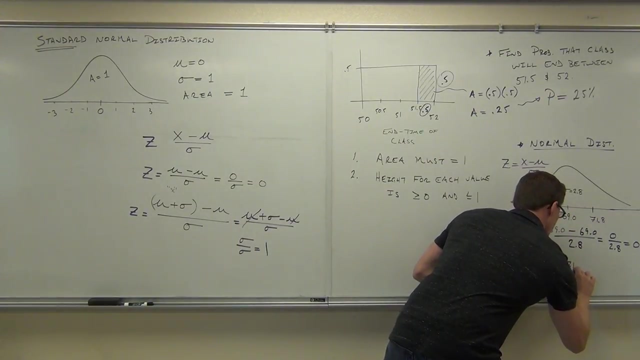 this did, is you plugged in the mean and mapped the mean. the z-score mapped the mean to the value of 0. let's plug in a number. that's one standard deviation. do you understand? that is one standard deviation away from me. plug in one standard deviation away from the mean, so the z-score would be 71.8 minus the mean. 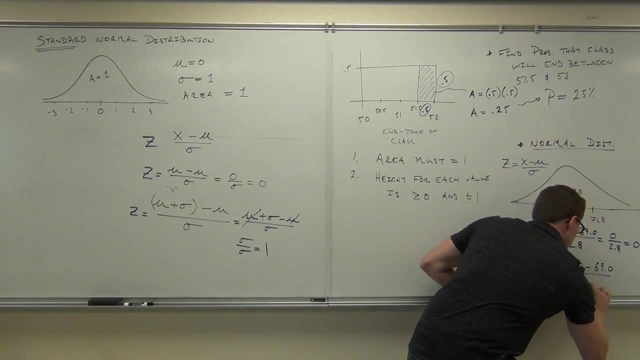 the mean 69. that's not going to change over the standard deviation of 2.8. do the math: what's? It's 71.8 minus 69, sure How much is 2.8 over 2.8?? I think I read it in the room. 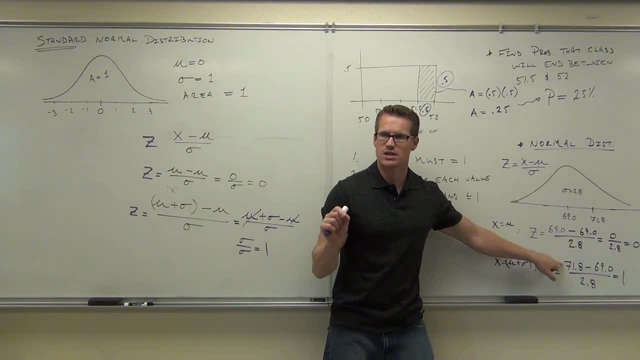 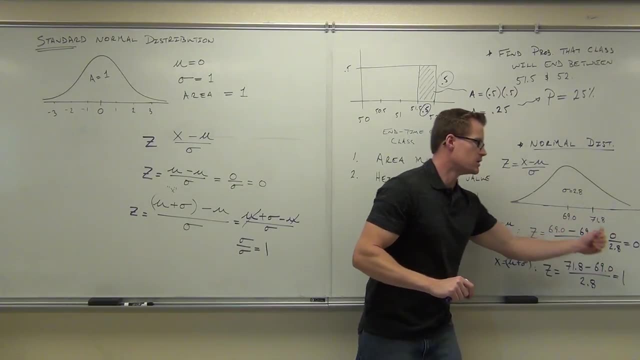 This just mapped a value. that was one standard deviation to the right of our mean to one. If I did two standard deviations away, it would have mapped it to two. Negative three, it would have mapped it to negative three. That's what the z-score does. 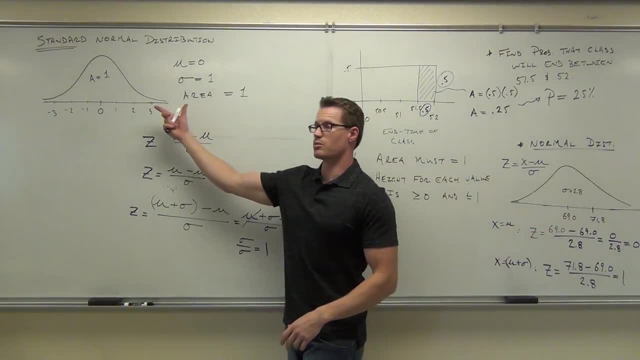 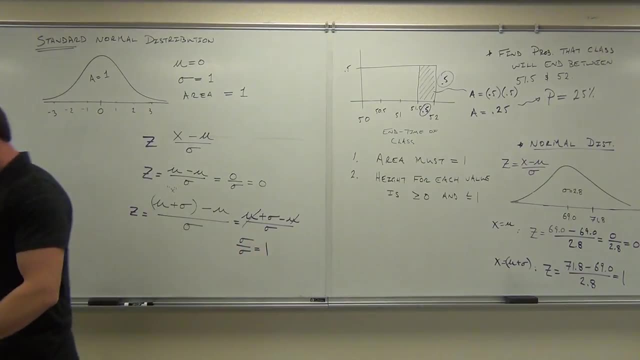 It maps every normal distribution into a standard normal curve, And that's kind of cool, right, because we've all been dealing with this z-score all along. What we're going to learn next time is that we have a table and a calculator that's going to allow us. 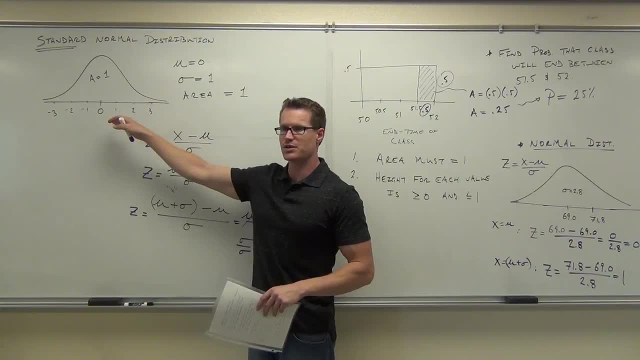 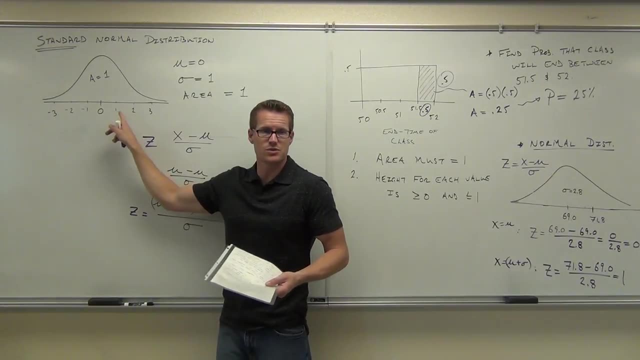 to find the probability of any z-score that you want. So notice that while these are a standard deviation of one, they're also a z-score. Do you guys see it? That's a z-score What? Z-score one? z-score two. z-score three. 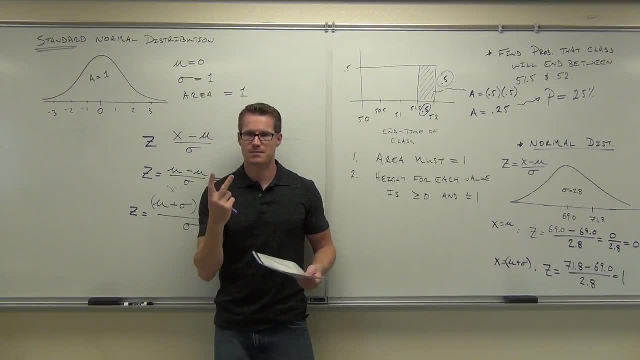 Those are the z-scores. So we're in the business of doing two things. We're in the business of finding z-score first of all. That's what we're going to be doing a lot of. We're going to be in the business of drawing a normal curve. 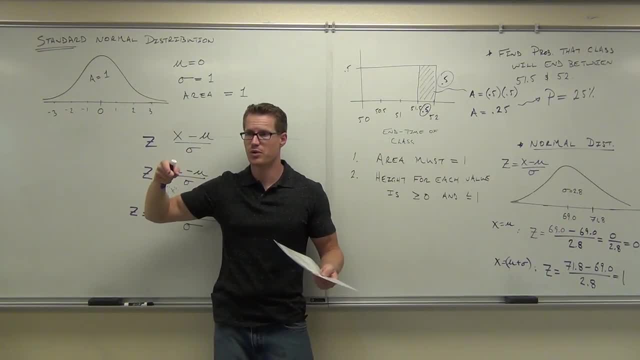 and placing the appropriate z-score on that normal curve. So if we get a z-score of 2.8, we're over here at 2.8.. Then we're going to be in the business of finding an area, And by finding the area you actually find what. 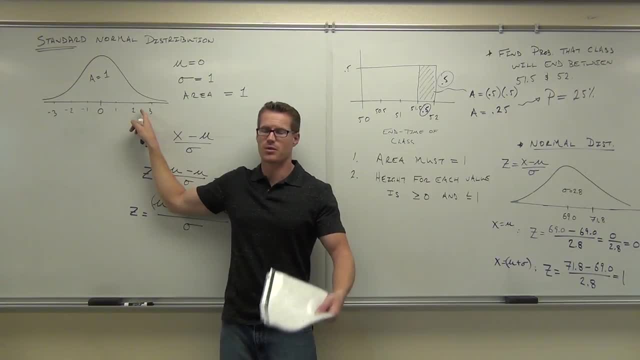 By finding the area, you actually find the z-score, You actually find the probability. that's right. So we're going to be doing three things: Z-score, drawing pictures and finding probabilities. That's what this is all about. How many of you understood today? 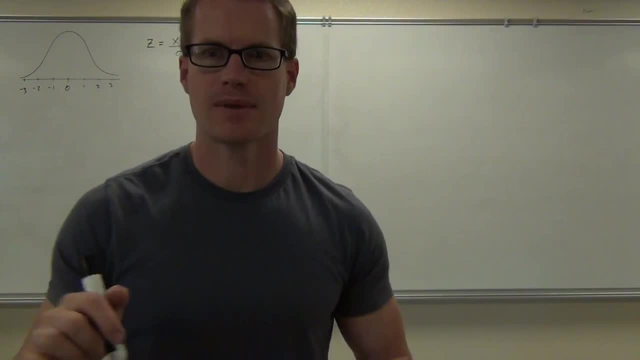 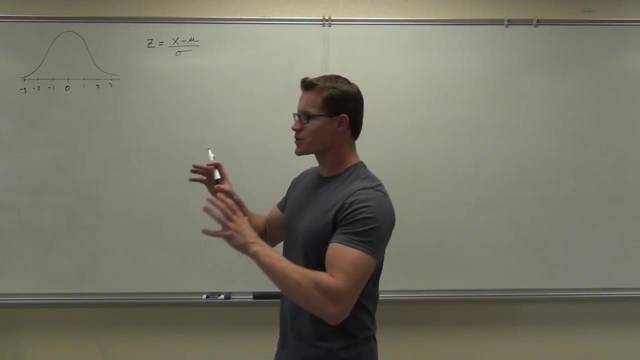 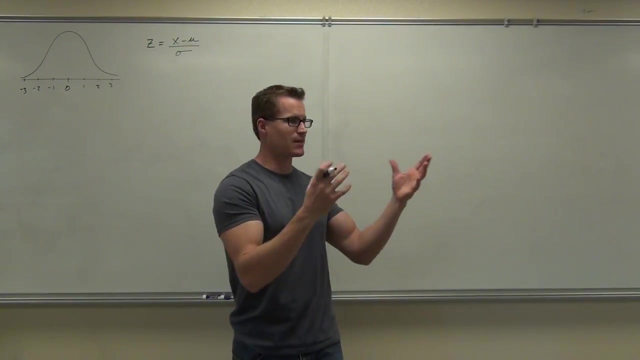 Good deal. So we're talking about this thing called a normal distribution and we realized we did this with continuous random variables and we also understood that there's lots of normal distributions out there for every specific context you're talking about. So, like heights, there'd be lots of different distributions. 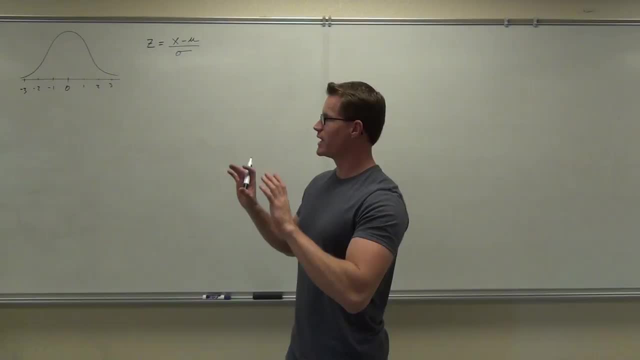 of heights. It's going to depend on your population. What we're doing here is translating any normal distribution into what's called the standard normal distribution. This is where we ended last time, right, The standard normal. What happens was: every mean is mapped to zero. 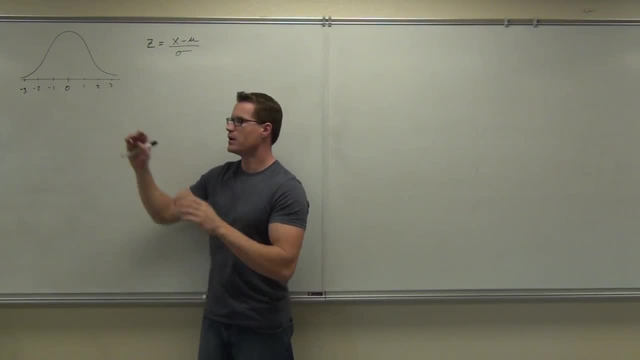 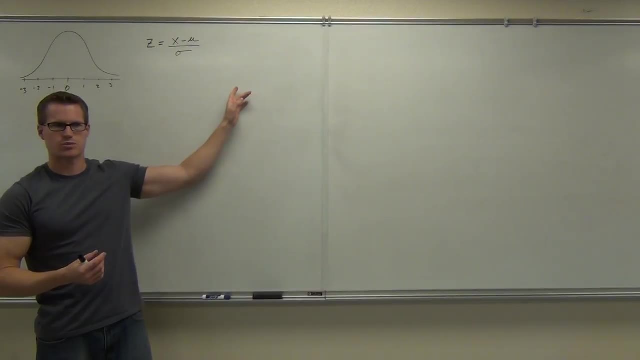 and every value. one standard deviation away from the mean is mapped to one. Two standard deviations away is mapped to two. What let us do? that was our z-score, And remember I showed you that example before for our test, where we actually did that right. 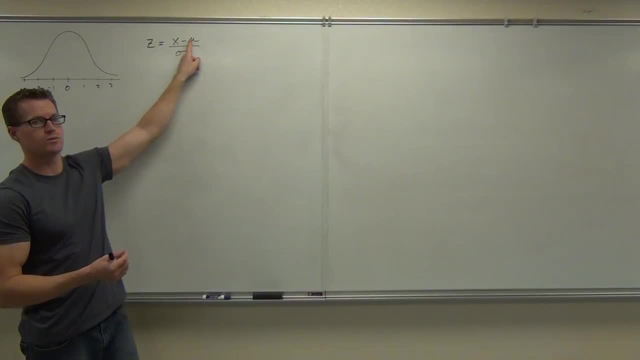 with the mean, that got mapped to zero. If you take the mean minus the mean, well, you get zero. If you take a unit, that's one standard deviation away from the mean, you subtract the mean, you get the standard deviation. Divide that by the standard deviation, you get one. 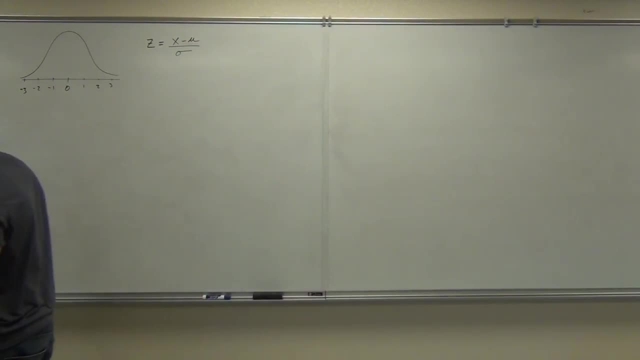 That takes everything and puts it into a standard, normal distribution. Now there's a few things we need to know about this. Firstly, of course, our mean is zero. Standard deviation is always one, no problem, But what's kind of nice is? 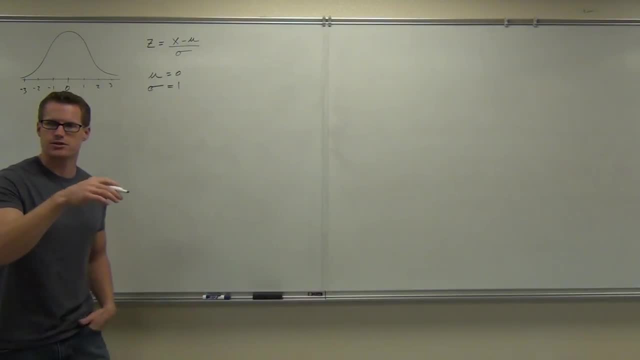 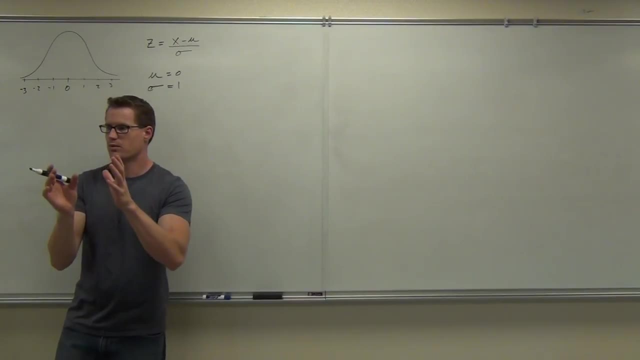 that someone has already done the work for us. Oh yeah, by the way, what's the area under this curve? again One One. yeah, you get one. That has to be it right, because we're associating area. 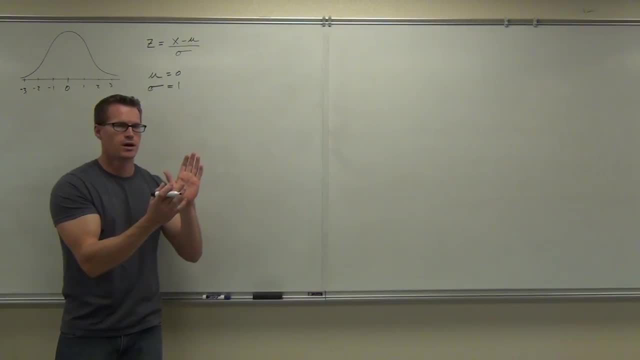 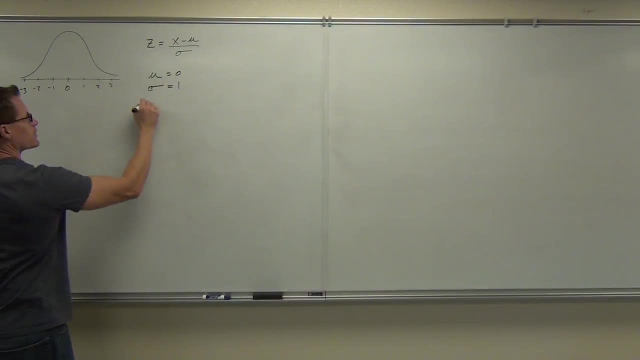 with probability. so if our probabilities have to all add up to one and every probability has to be less than or equal to one, then the area underneath this curve has to also be equal to one, So area equals one. Since that's the case, 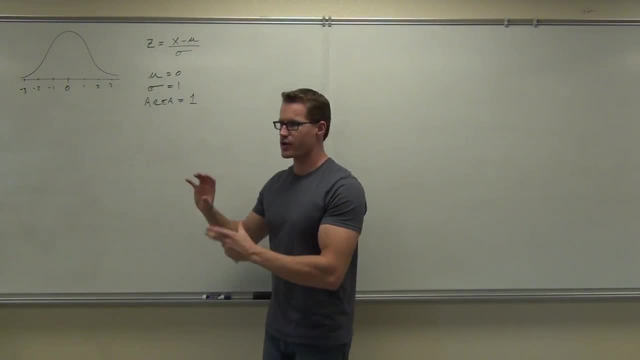 someone's actually already done the work to figure out all the areas, all the probabilities for every one of these cases. As a matter of fact, that's in that pull-out sheet that you guys have. it's the one that looks like this: 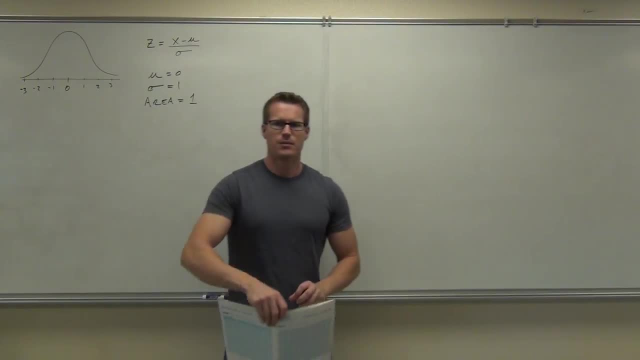 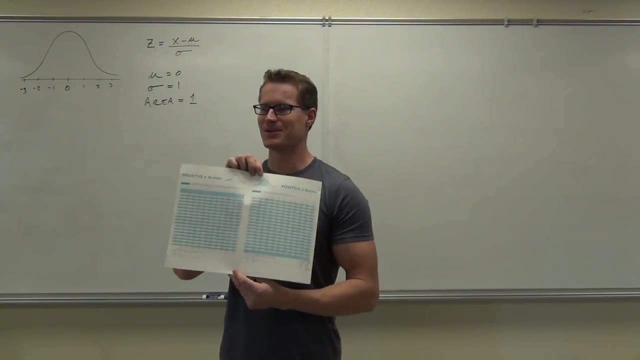 What it says is positive and negative z-scores. Have you seen that one? It's on the back. you're like: what are these tables for? We've never used these. Hey, we get to use them now. The positive and negative z-scores are: 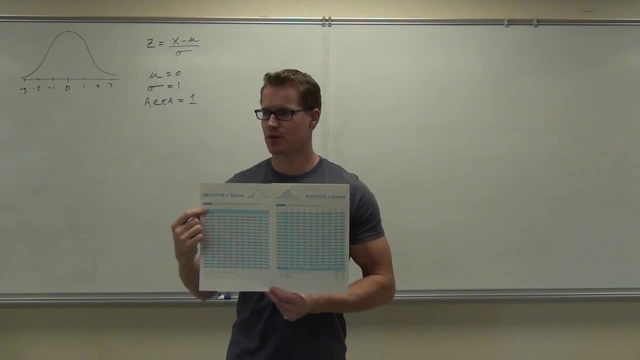 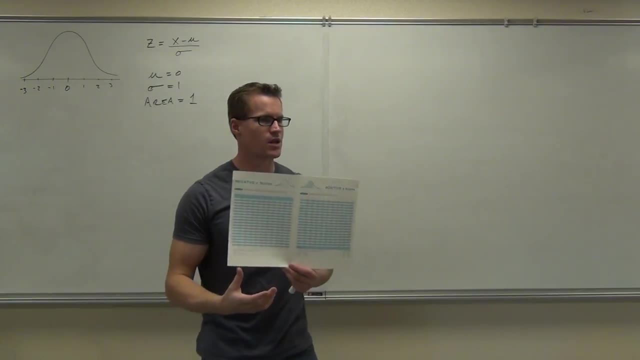 for the standard normal distribution. Notice how it says z-scores. How do we map normal distributions in the standard normal, That's with a z-score. So really all we're going to have to do in this section is be able to find a z-score. 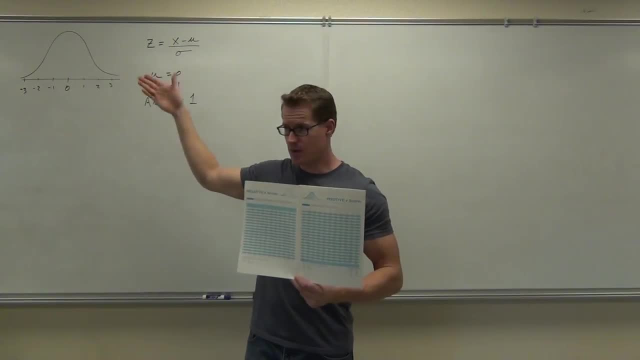 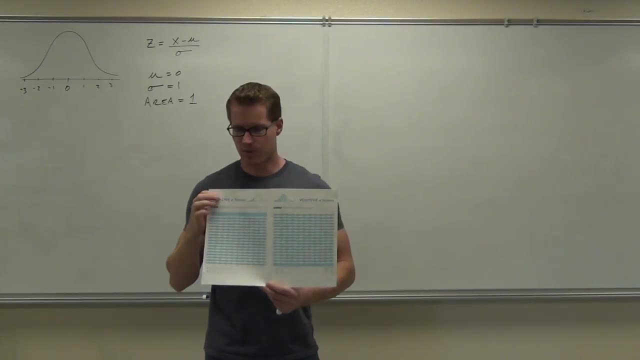 be able to draw a really pretty picture, put the number on there and find out whether we're going to shade to the left or right. I need you to know something about this table though. This table, if you look at the very top. 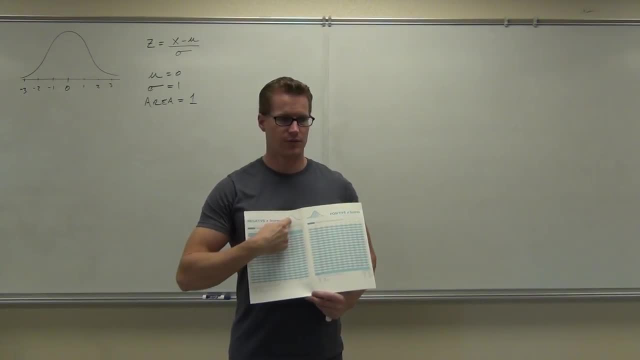 got a curve very much like mine right. It has a zero in the middle. If you guys have yours, pull it out. Then there's a z-score. That z-score is what we're going to be drawing up there, and it's shaded to the left. 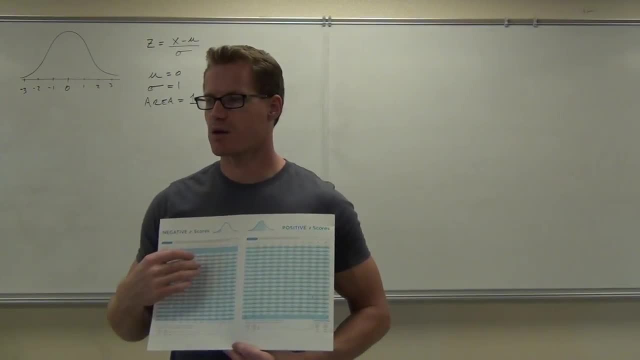 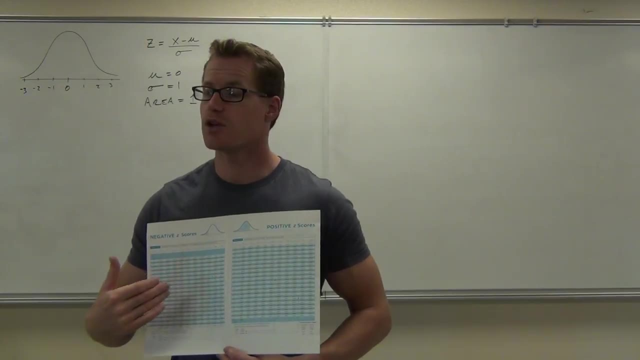 What this means is that this table only gives you the areas to the left of a shade of a value, The area to the left of that value. Now, you're happy with me on that? All it gives you. Your calculator will calculate this for you. 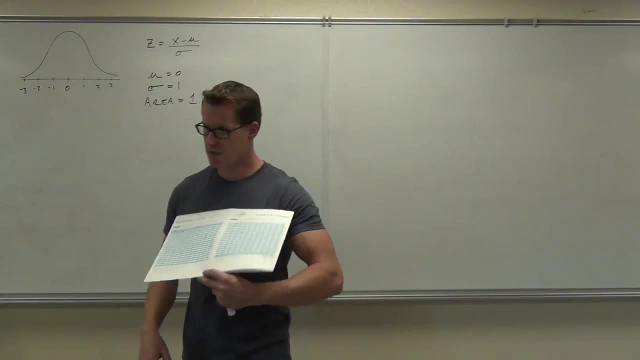 I'll probably show you that next time, But for right now, let's do an example using this table to see if we can figure out our area or our probability. Are you ready for it? Yes, Okay, Did you know that every thermometer is not completely accurate? 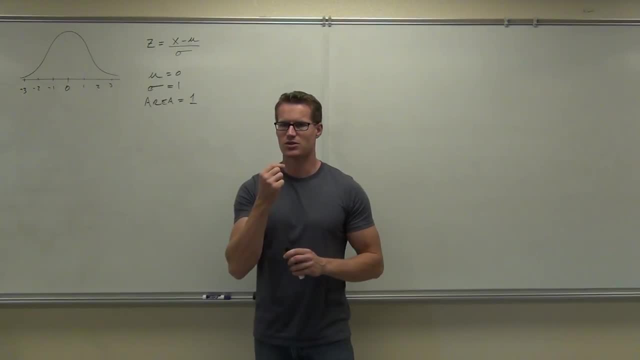 If you think about that- I mean, no one ever thinks about that- Someone thinks that when you take your temperature it's always perfect, right? Well, haven't you ever got like a bag of chips that seems like it has less chips or a little bit more chips. 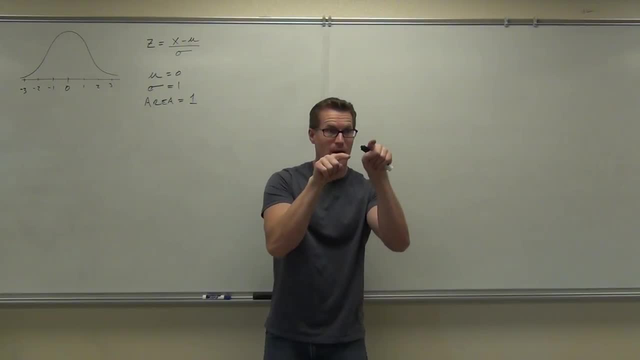 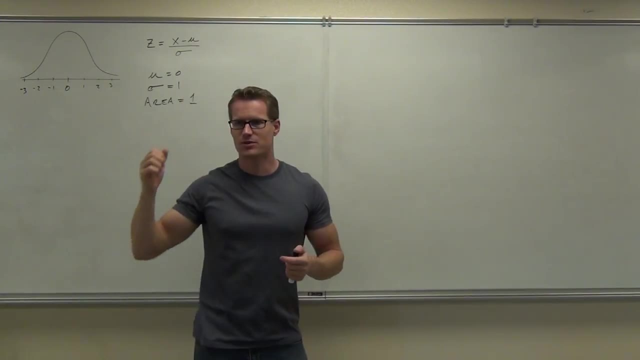 Or a soda that has more soda. You're like, I want that one, that one, But you always do that. Well, the same thing happens with thermometers. I said thermometers right the first time. Yes, Thermometers are a little bit off, not like a whole bunch. 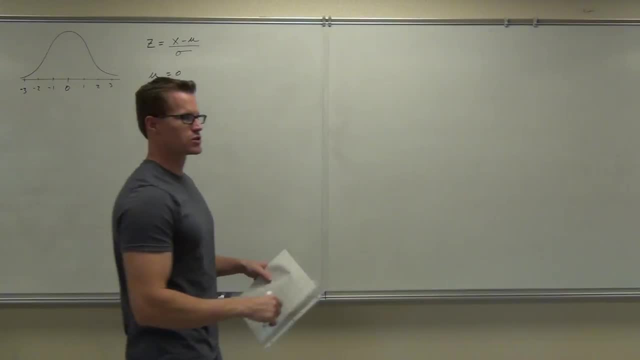 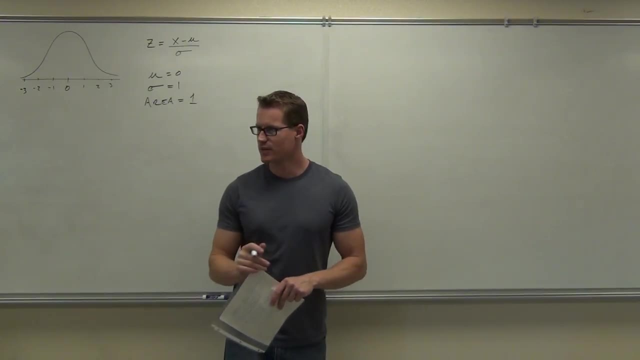 but a little bit off, A little teeny bit, As one company wanted to determine the probability of getting a reading that's less than a certain amount. You see, what they didn't want was that a thermometer gave too high of a reading, because that would give like a false positive. 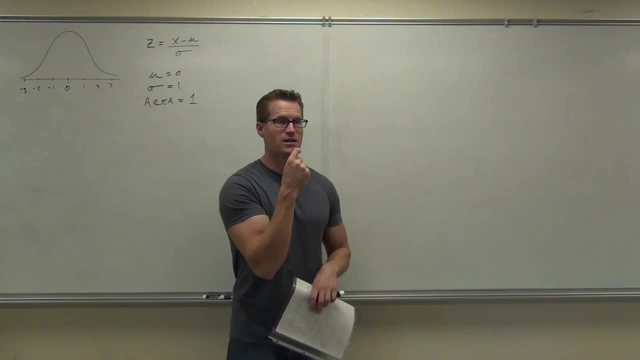 for a temperature, right, Because if you took a temperature of 108, oh my gosh, I'm going to die. actually you'd already be dead. But like if your thermometer said you have a temperature of 108, you're like, but I feel fine. Your mom's like rushing you to the hospital or whatever, or you're rushing yourself to the hospital. Don't do that. if you have a temperature of 108,, by the way, Just get in the ice bath. I think that's the best thing you can do. 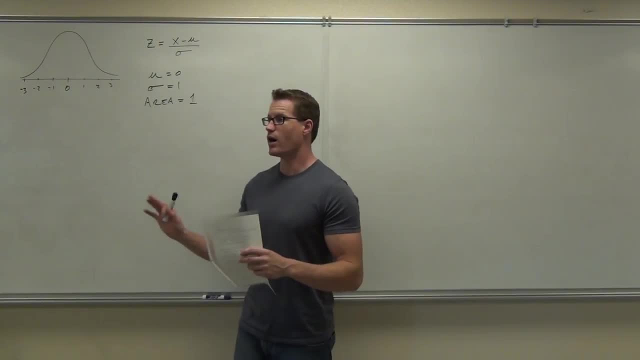 But anyhow, they don't want to send out these thermometers that are way, way off, do they Probably not? They don't want to send them where they're too low or they're too high, because they're giving you a false reading. 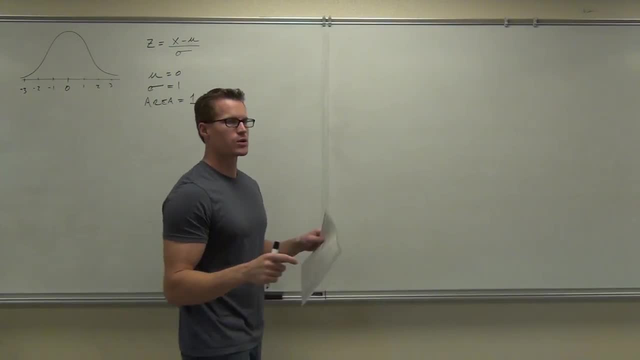 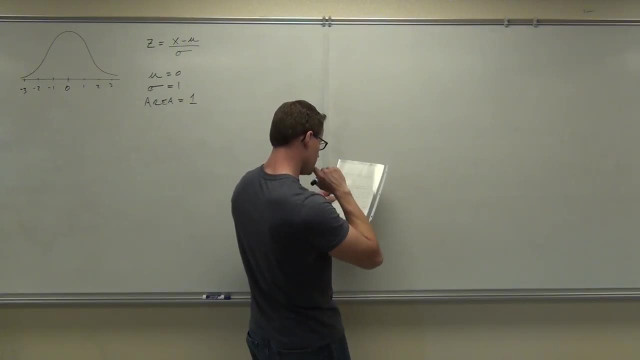 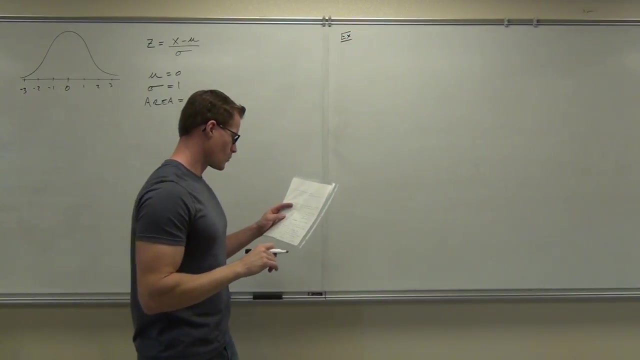 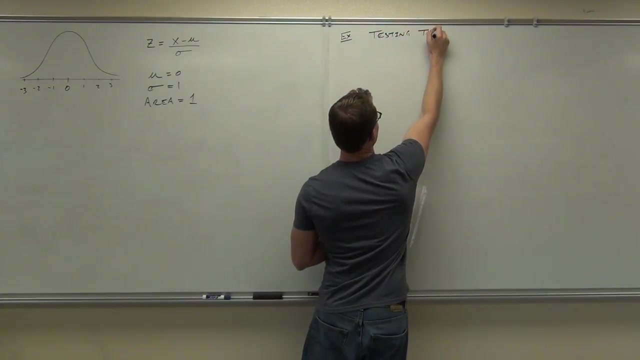 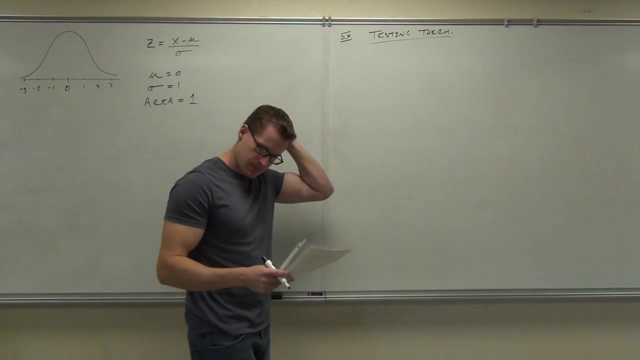 So what this company said, or what this company did, I'm sorry, was took a large, large sample, close enough to be a population for us. So this company tested thermometers. What they found out was that the mean, the mean of these thermometers was zero. 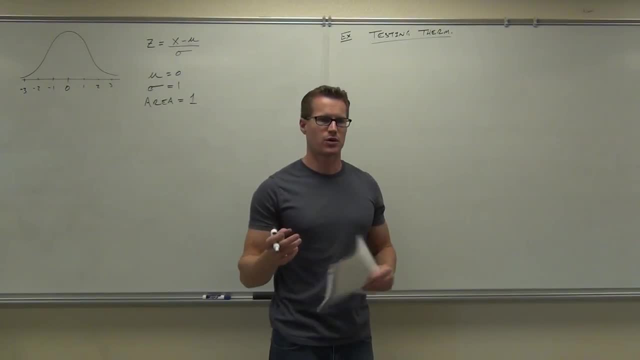 Why was it zero? Well, these particular thermometers are based on the freezing point of water, saying that if you stuck this in the ice bath, you're going to die. If you stuck this in frozen water, well, ice that it's going to read zero for you, okay. 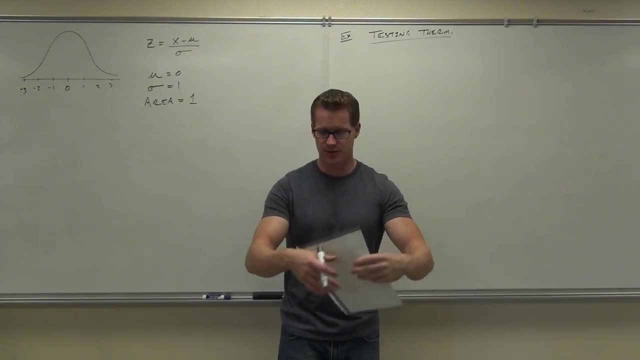 And so what they did was they found out, they averaged all the readings, So they stuck them all on the same ice and they read their readings, And some of them were a little bit high. some of them were a little bit low because the thermometers are not completely accurate. 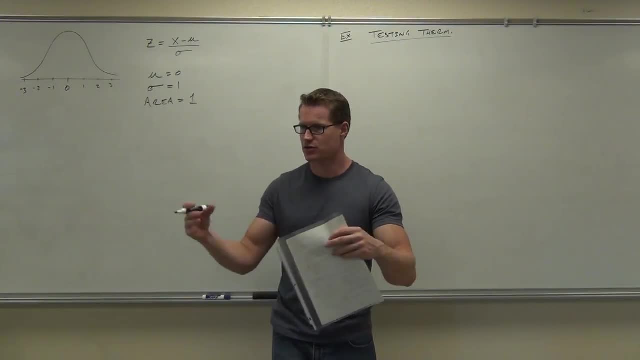 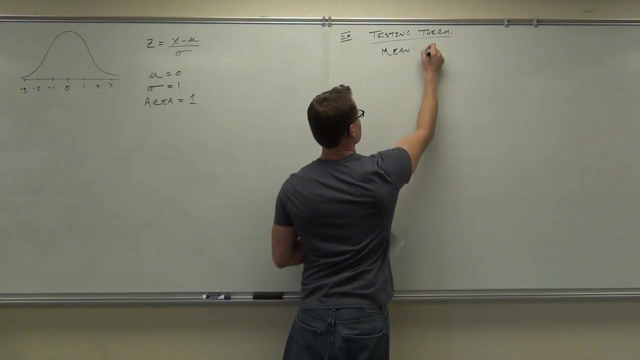 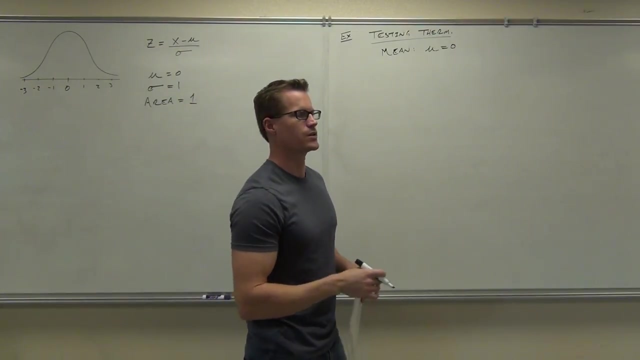 You understand that right. But most of them, when they averaged them, they averaged all of them together. they read zero like on average. So their mean was zero And just to make things easy for right now, their standard deviation was one. 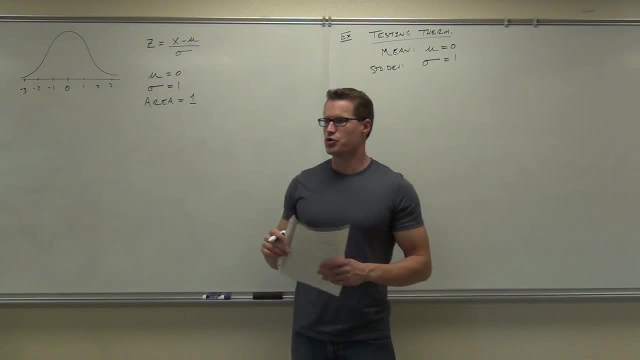 Also one more important piece of information. The readings were normally distributed. Is that important for us? Is that an important piece of information? Or why is it an important piece of information? Why? What type of distribution are we working with? A what distribution? 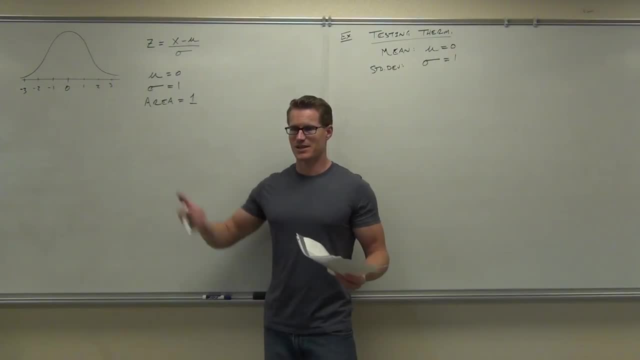 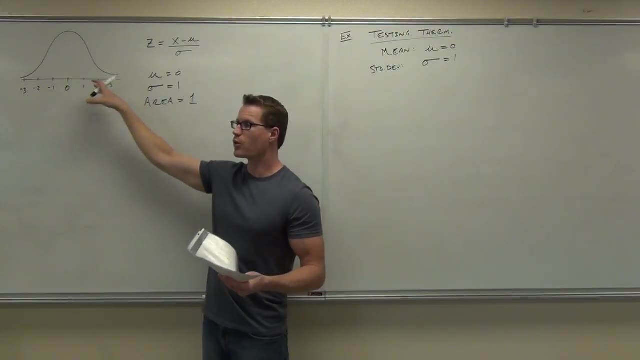 Normal distribution, Normal distribution If it's not normal, does that work? No, No, If you don't have a normally distributed data, this doesn't work, because this is only for normally distributed data. So this had a mean of zero standard deviation of one. 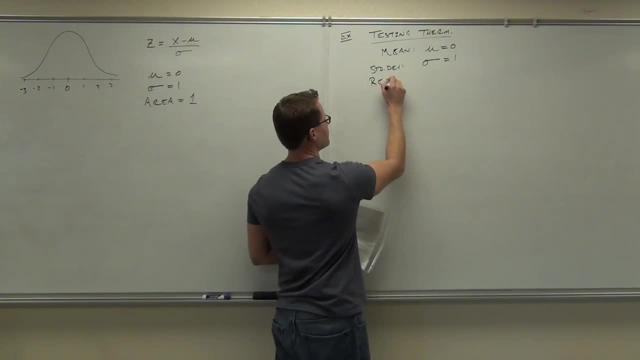 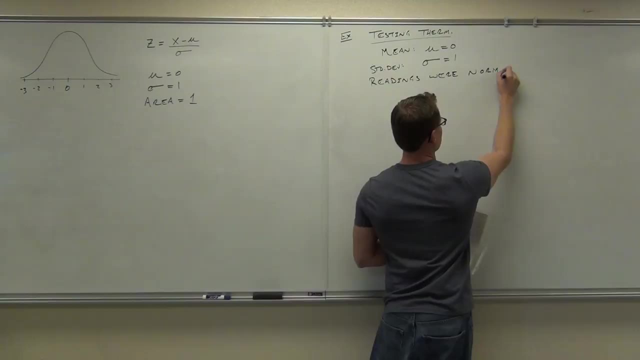 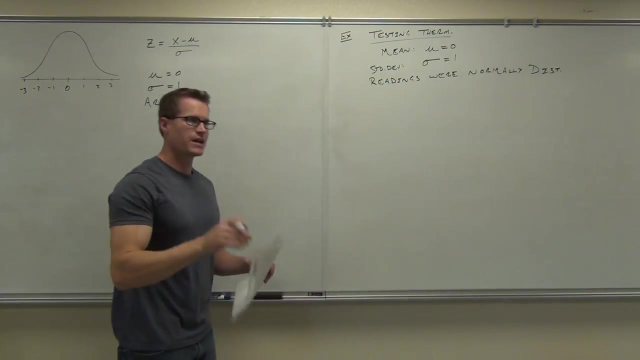 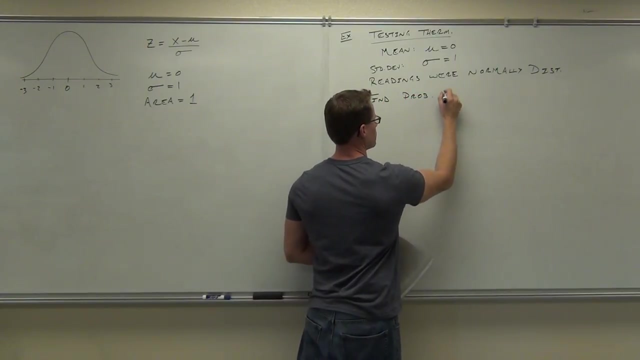 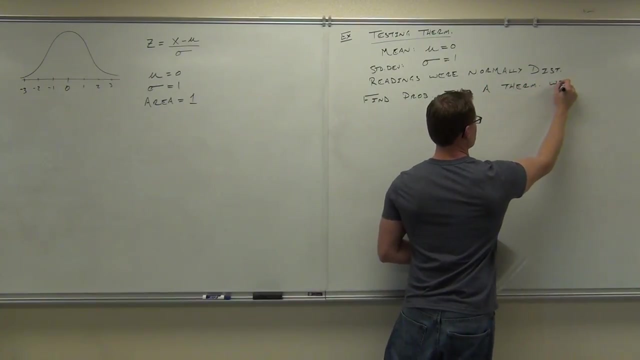 and the readings were normally distributed. So what we're going to do is we're going to do a little bit of a math test. Here's what we want to find out: We're going to find the probability that a thermometer will have a reading. 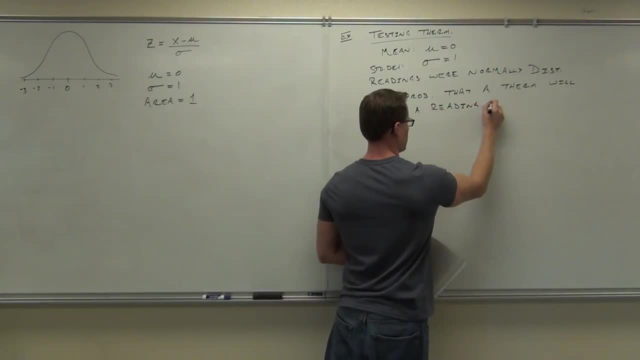 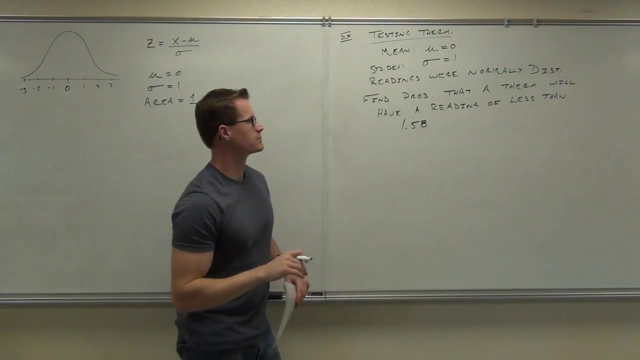 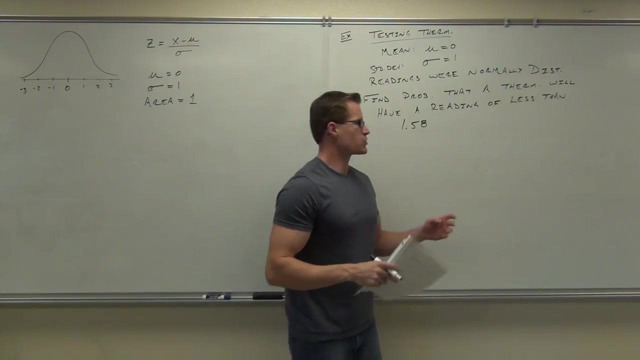 that a thermometer will have a reading, that a thermometer will have a reading of less than 1.58.. Let me give you the idea for this and we'll call it a day. okay, Here's the idea. What we're going to do here is we're going to translate this score of. I'm sorry. 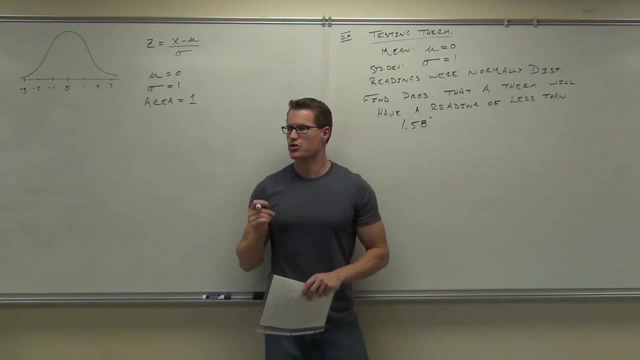 this value, this data value of 1.58 degrees. we're going to translate that into a z score. Now, that's going to be very easy, because this information is very easy to work with. In general, it's not that hard. 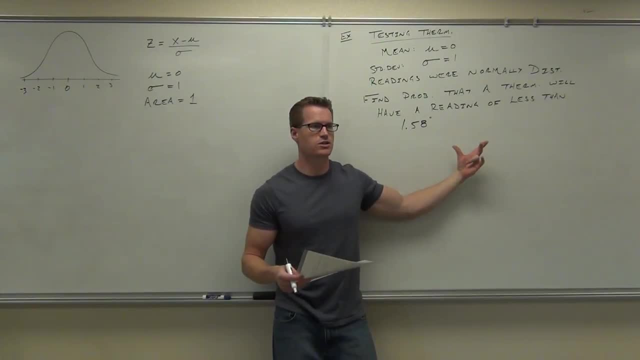 You can calculate this very fast. We're going to translate this into a z score. Ladies and gentlemen, why are we translating this into a z score? do you think? What was that table based on that? I just showed you Z-scores. 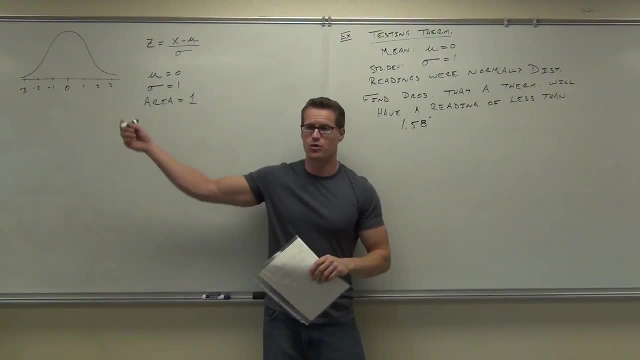 That's why we're going to translate z-scores. It's based on z-scores, right? It's based on the standard normal distribution, which has z-scores on it. We're going to translate this value into a z-score. 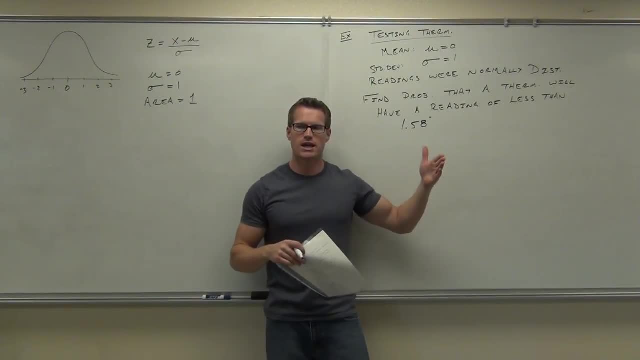 After we do that, we're going to draw a picture and we're going to shade one side of that line. What we're going to find out is an area under a curve That's going to associate itself with probability and will give us a probability. 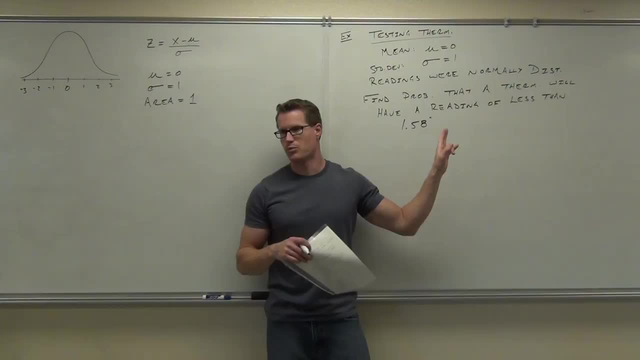 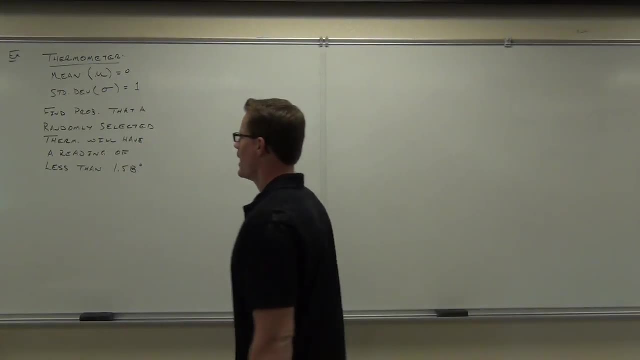 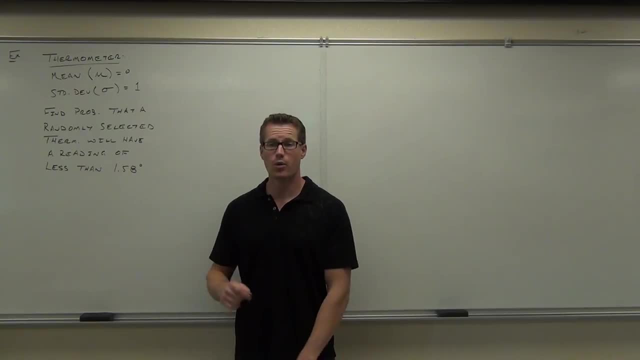 I want it to be pretty accurate within a couple degrees. So we're going to go ahead and see how you would find the probability of randomly selecting one of those thermometers, and it has a reading of less than 1.58.. Are you guys ready to do this? 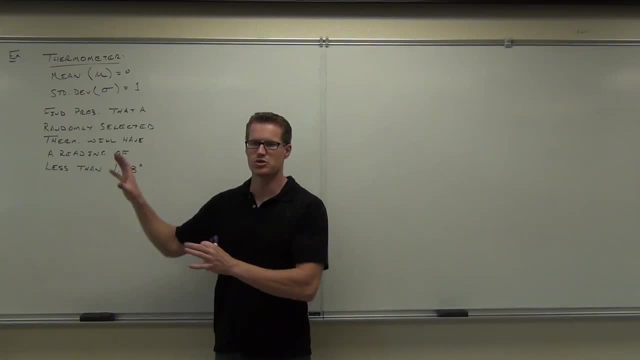 Yes, Good. Last time we talked that a normal distribution can be translated to a standard value of 1.58 degrees, standard normal distribution by simply using the z-score. It maps the mean to zero. it maps a unit, that's one standard deviation away from the mean. 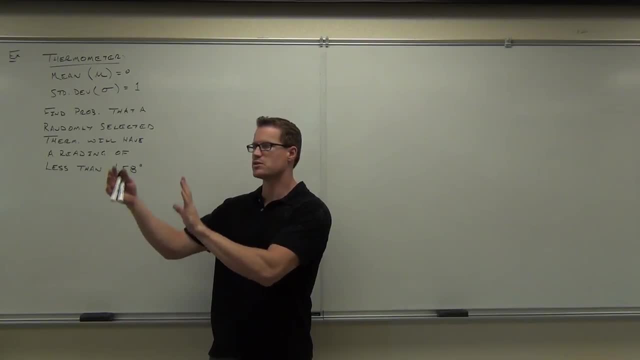 to the value of one and negative one, standard deviations away to negative one. So it maps any normal distribution to a standard normal and the reason why we wanna do that, all of the computations that your calculator and then the table I told you about last time is based on. 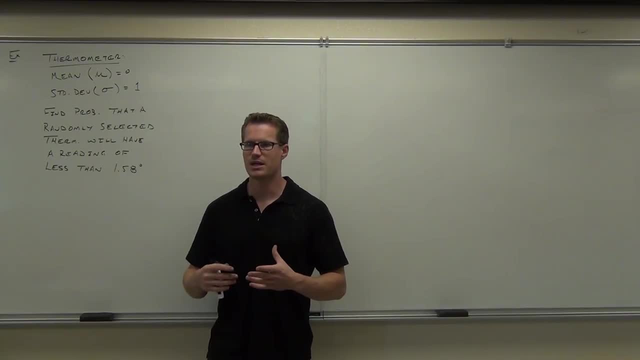 is a standard normal distribution. You see, there are infinitely many normal distributions, but only one standard normal. It takes all those normal distributions and translate them to the same picture. Are you with me on that? That's why we have such a thing called a z-score. 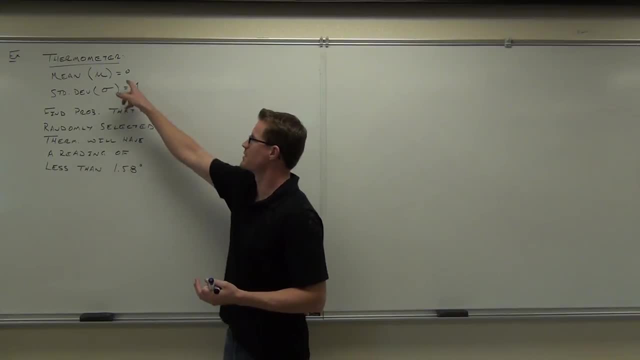 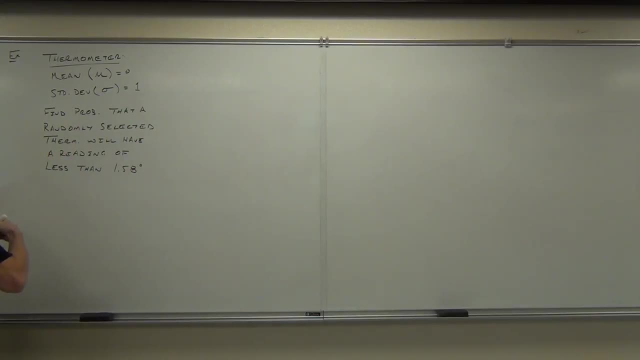 So, in order to translate this problem, which is gonna be pretty basic because of our situation here, into a standard, normal distribution, we're gonna use a z-score. So the first thing we're doing is somehow we gotta calculate this, The z-score, if you don't remember it. 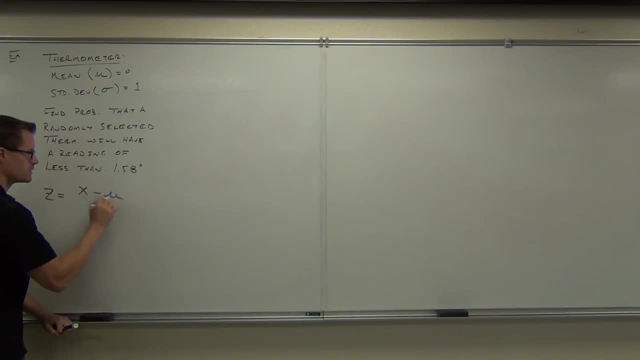 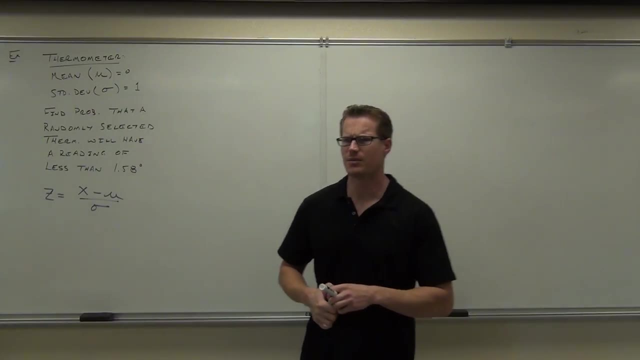 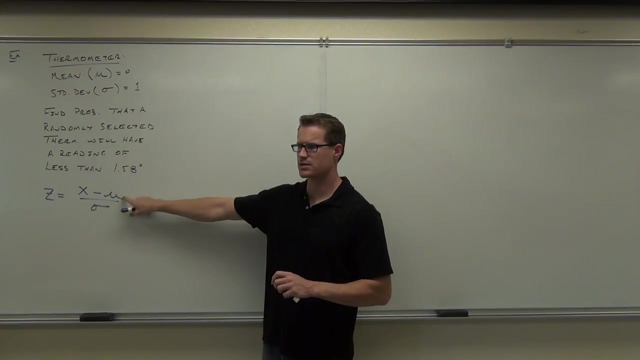 you're gonna wanna memorize this is x minus the mean over the standard deviation, Or x minus mu over sigma. Hey again, by the way, what does the mu stand for? That's a mean for a. that's not a sample. 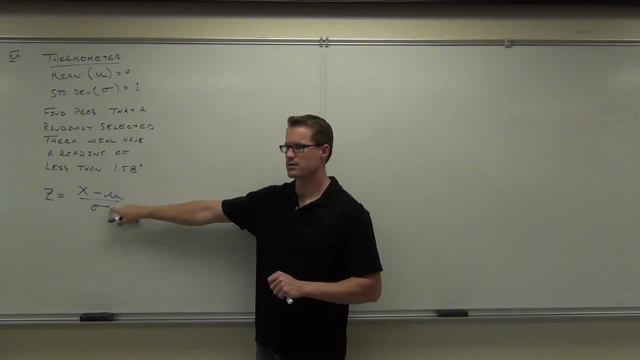 that would be x-bar. this is a- And this is a Good standard deviation for a population as well. What is x? I'll bet you could tell me x in this case? I'll bet you could, but what's x in general? 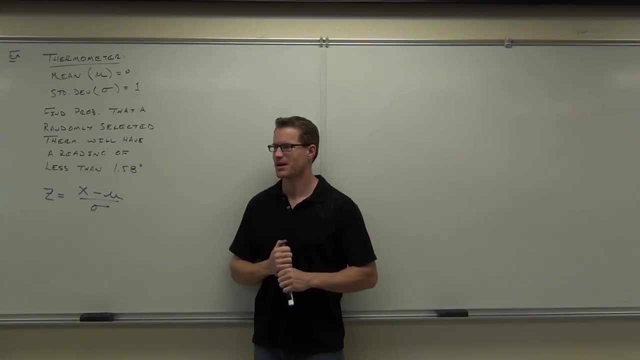 Ooh, stumped y'all, Stumped y'all. What is x in this case? Yeah, you're right. Yeah, it's the value. So in this case, x is 1.58.. If I said less than two degrees, x would be two. 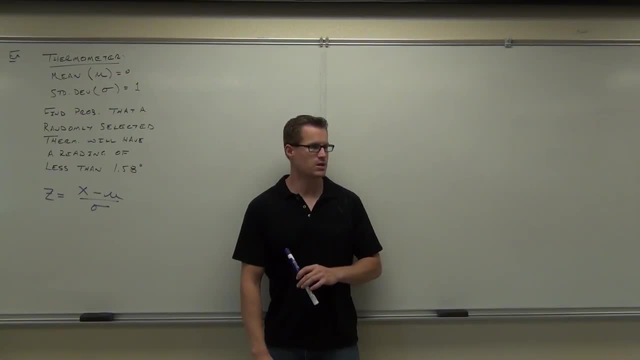 If I said more than negative three degrees, x would be negative three. Are you with me on that? X is the value that you're checking. In other words, it's the continuous random variable. It's the variable. It's what can change here. 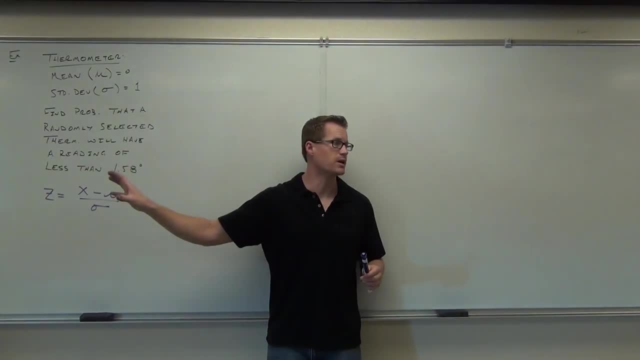 Your mean and your sigma. those aren't gonna change. Those are set for your population. However, your x- that's the value that you're checking. In this case it's 1.58.. Remember, we're continuous because we're typically dealing with measurements. 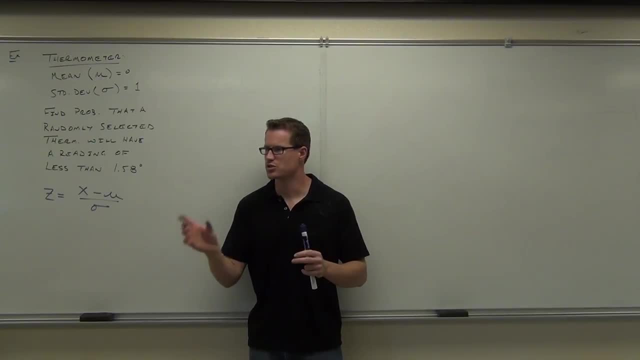 and those have an infinite number of possible values. Remember the difference between discrete and continuous. Discrete was like rolling a die: You only get one through six. Continuous was like a measurement: You get 1.58.. You get 1.5823.. 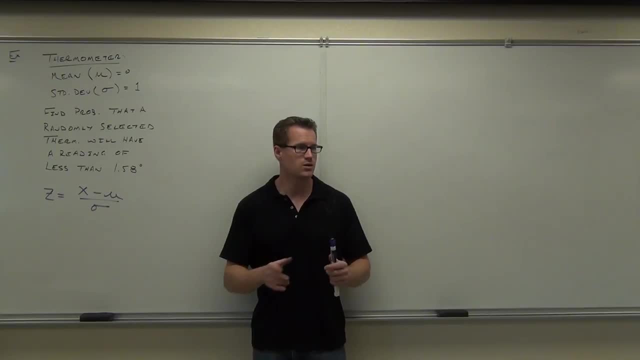 You get 1.5810.. You know, you get all sorts of different values in there and infinite numbers. That's why we have a continuous situation here. That's why we're in chapter six talking about continuous random variables, and that's what x stands for. 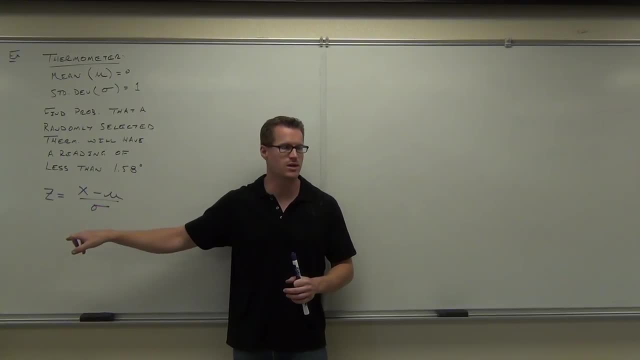 Do you understand that? So when I ask you what x stands for, you're gonna tell me that x stands for the value of what. Wow, that didn't sink in, did it? I don't? You better know it. We just talked about it. 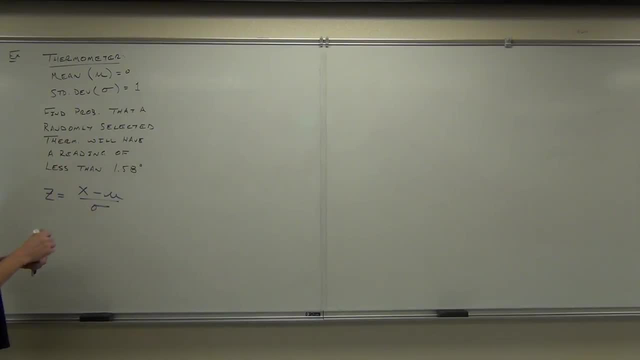 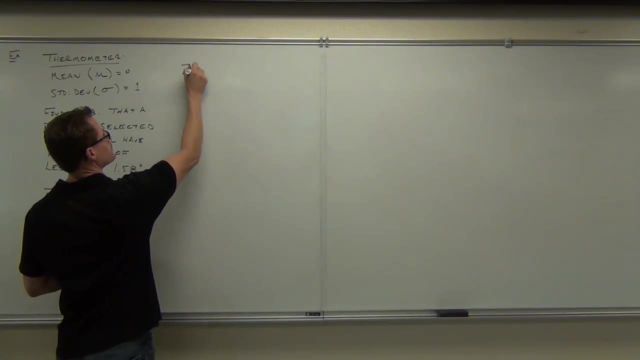 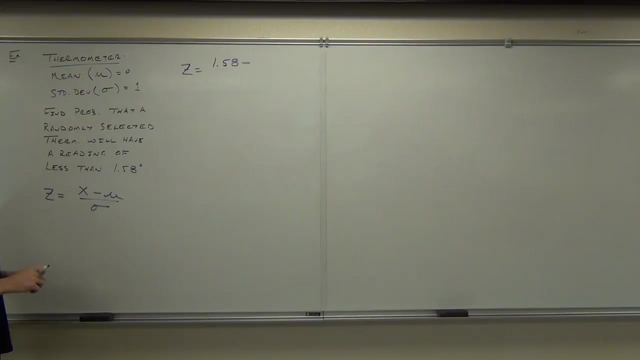 Figure it out, Okay, so in our case, x is how much? Yeah, good, It's the value we're talking about. It's the value we're talking about. Watch that video again, if you didn't catch on what we were talking about. 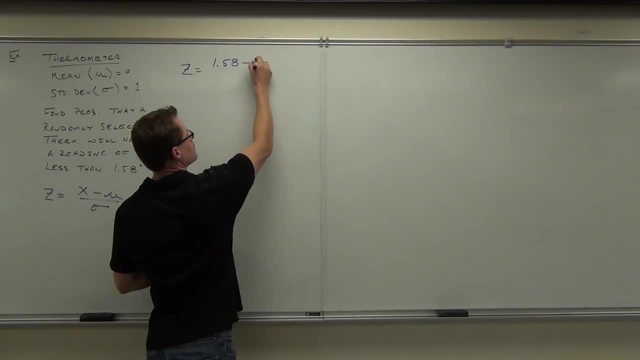 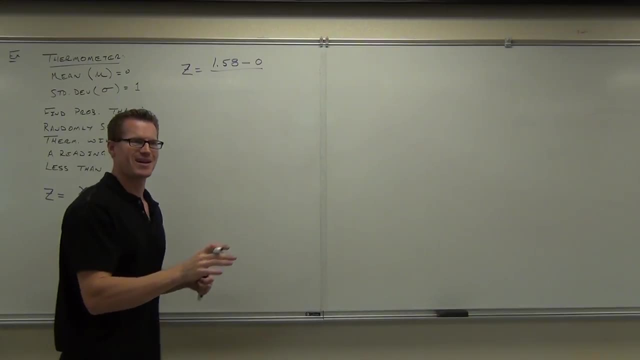 What's our mean in this case? So we're gonna subtract zero and we're gonna divide. What's our standard deviation here? One: Okay, you're pretty good at finding the formulas out. You just don't know what any of these values mean, right? 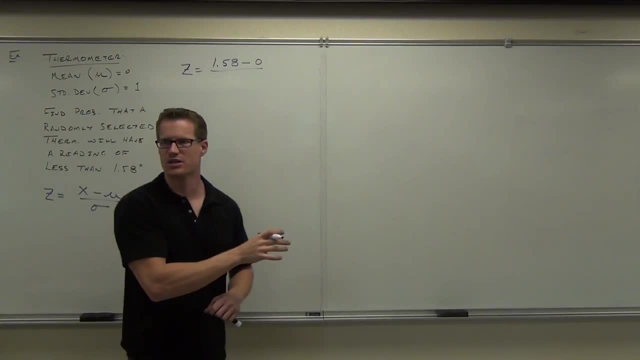 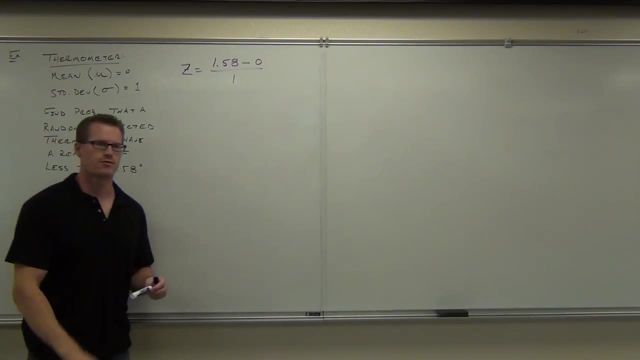 You know what the mean is. You know what the standard deviation is. We've been doing that for a while. X is your continuous random variable, Just like x was your discrete random variable in the last chapter. It's the variable. X is a variable right. 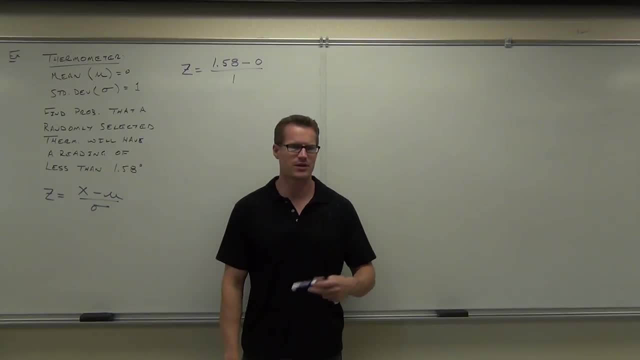 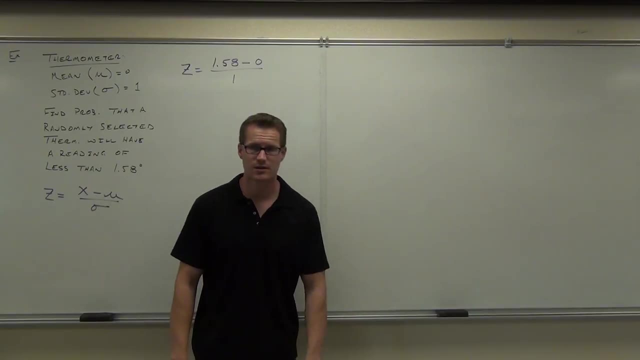 It's the only thing up here that's even possibly changing, So the only thing that can be changing. you call that a variable. In this case we're talking about continuous variables. That's why that's a continuous random variable. So what is x? 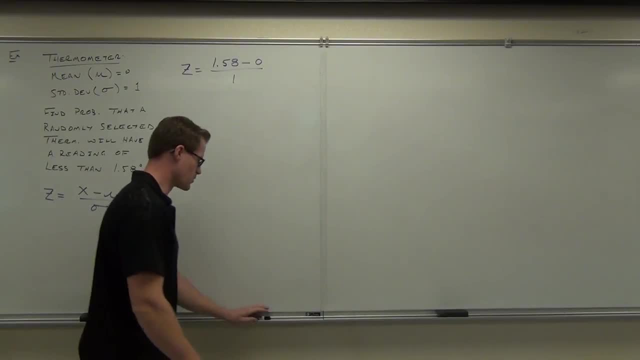 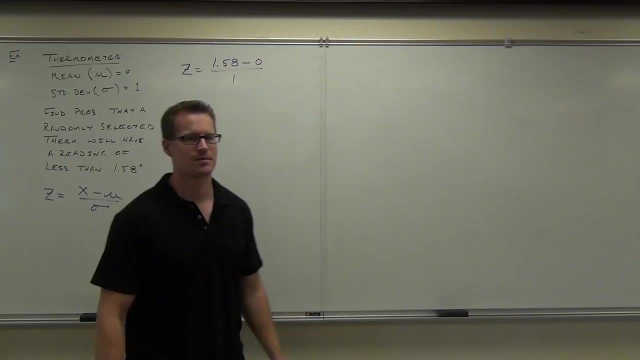 Continuous random variable. There we go, There we go. Continuous random variable. Hey, can we figure out the z-score for that? Yeah, this situation's gonna be pretty easy. What's the 1.58 minus zero? And then we divide by 1, we get how much. 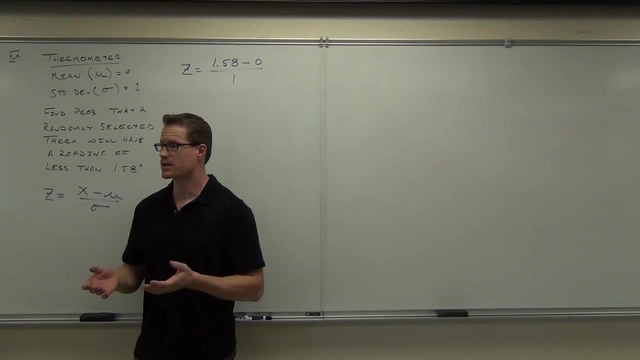 This is the most basic example we have, because with this thermometer situation it's already a picture of a standard normal distribution, so it's not changing anything. But I want to go through the process here to show you that this is what you would do in any case. 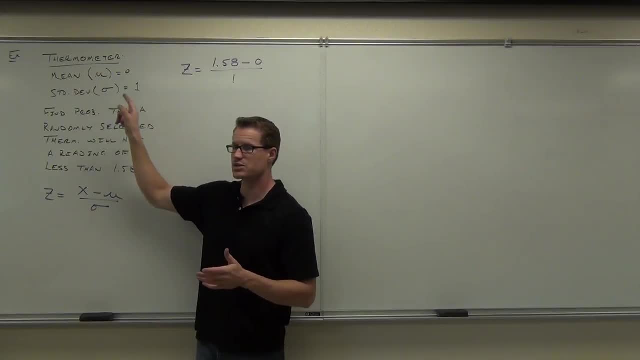 If you had a mean that was different than zero and a standard deviation that was different from one, you would still find the z-score here. The reason why the z-score doesn't change for us is because we know standard normal distributions are supposed to have a mean of zero. 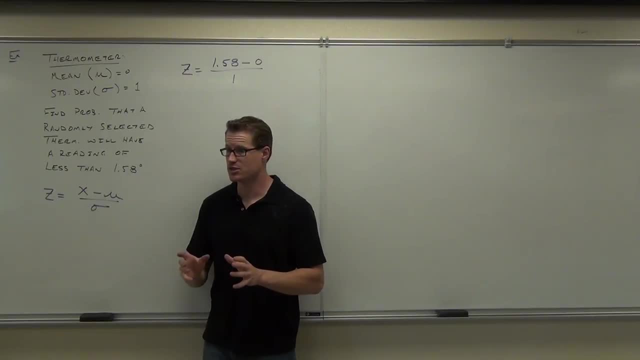 and are supposed to have a standard deviation of one. If they don't, the z-score works. for us to change that value. If they do, the z-score confirms that this is a standard normal distribution and in this case, the value is the z-score itself. 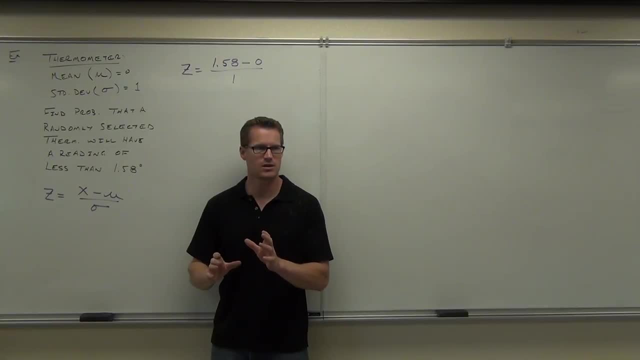 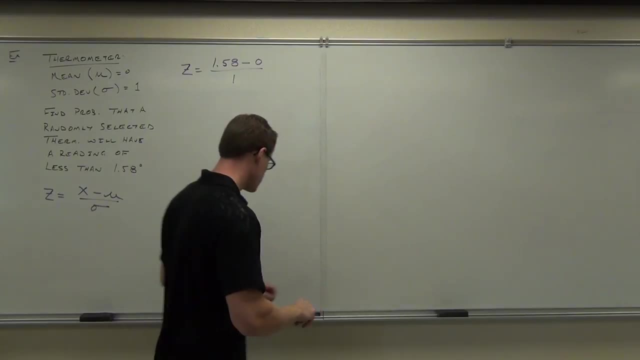 Did that make sense to you? Did you follow that? So this is a very special case. Most of the times our mean isn't zero. Most of the time our standard deviation isn't one. We have to change it using the z-score. 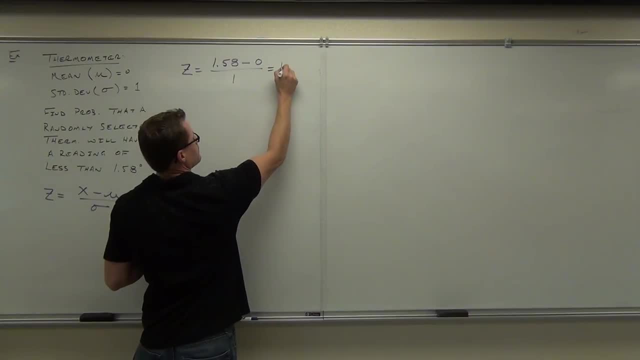 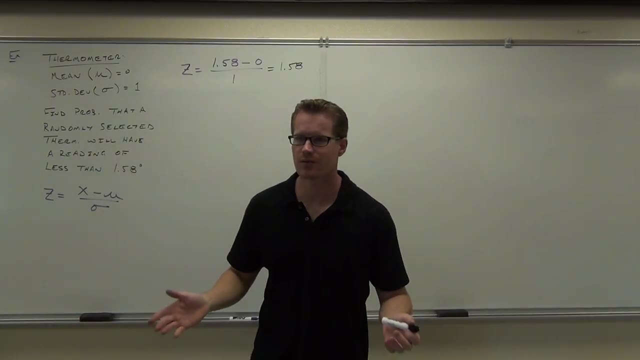 Here, of course, our z-score is 1.58.. Now here's the important part: Everybody in here is going to be able to find a z-score. That's not a hard thing, right? It's not a hard thing. 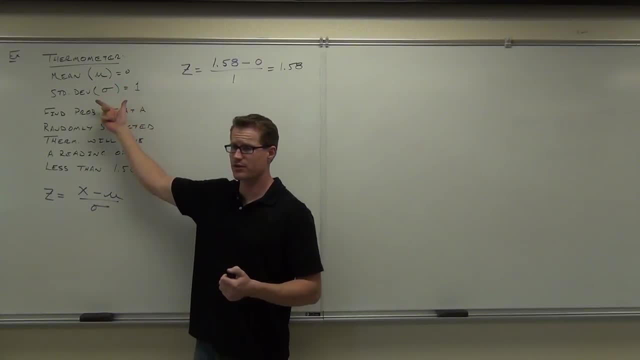 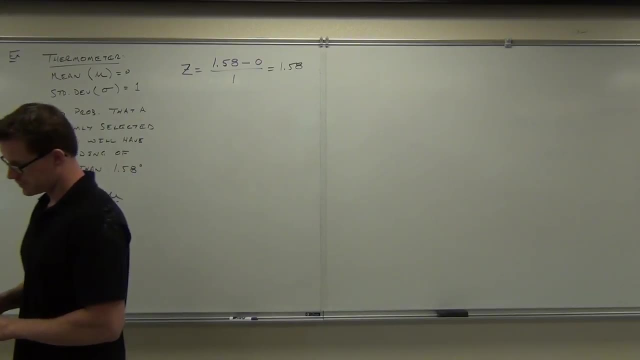 You just take your value, subtract whatever mean I give you, divide by whatever standard deviation I give you, and you get a number out of that. True, The next part that you have to do after you find your z-score. So step number one: 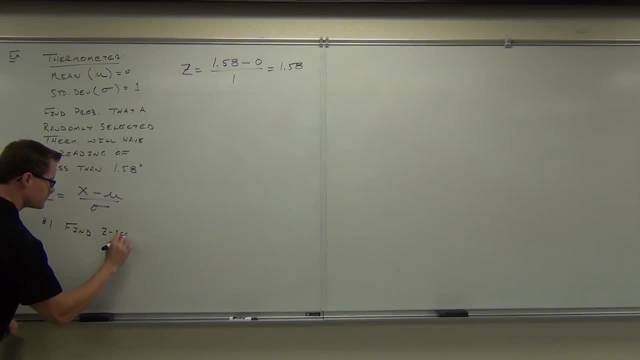 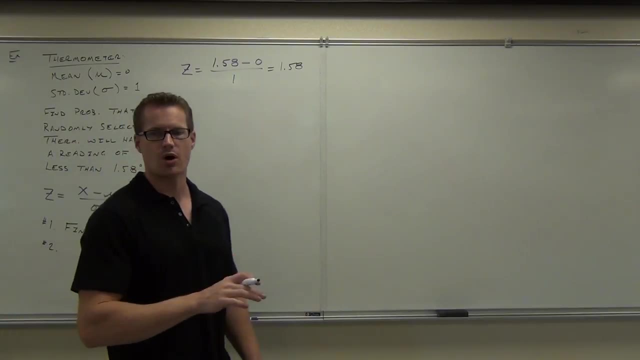 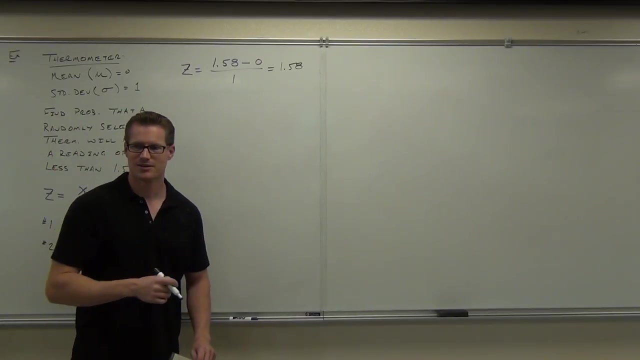 find z-score. Step number two: after you find that z-score, you are going to draw a picture. I don't mean like a kitty, cat or a horsey, I mean like a picture of a distribution. Let's say, Mr Leonard said 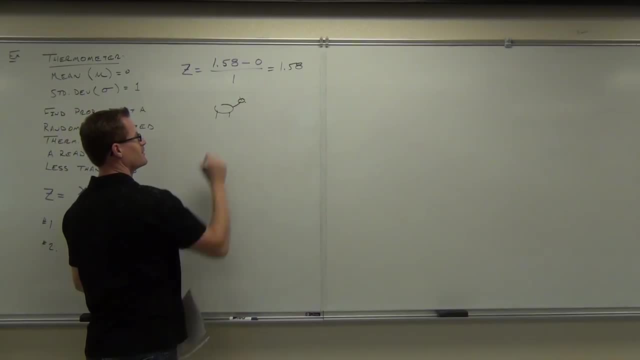 draw a picture of a little kitty cat. Meow, That's my cat. It's a giraffe. I beat him up. I don't even have a cat- Actually I do. It's a stray cat. It comes around. 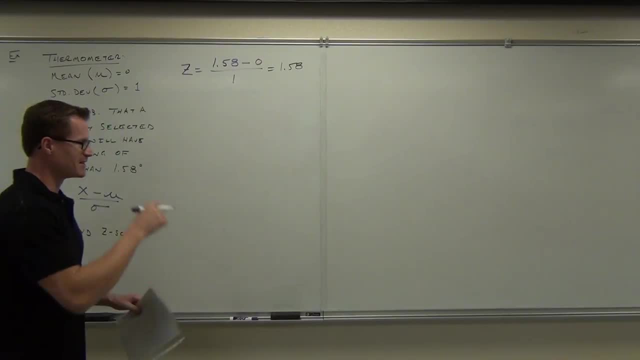 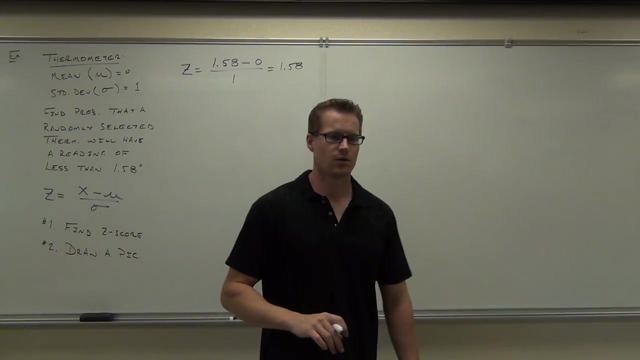 I was stupid. I fed it once and the thing keeps coming back. It keeps beating. That was my first mistake. Yeah, Absolutely. Find a z-score, then draw a picture. Here's the picture I want to see for you. 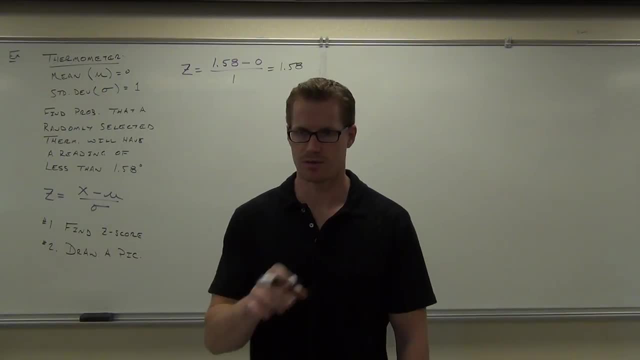 You kind of got to know these things, But again, I'm going to kind of refresh your memory on them from time to time. X stands for what particular chapter, Good, And the z-score translates a normal distribution into what. That you got to know as well. 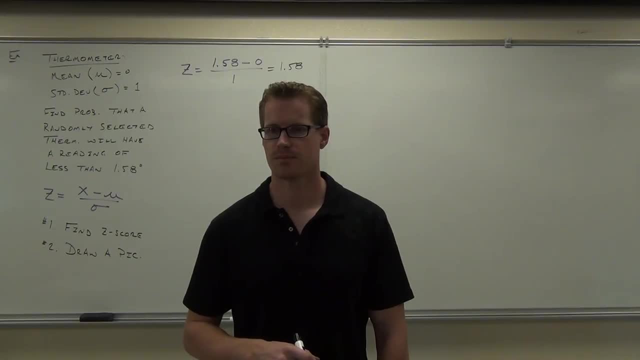 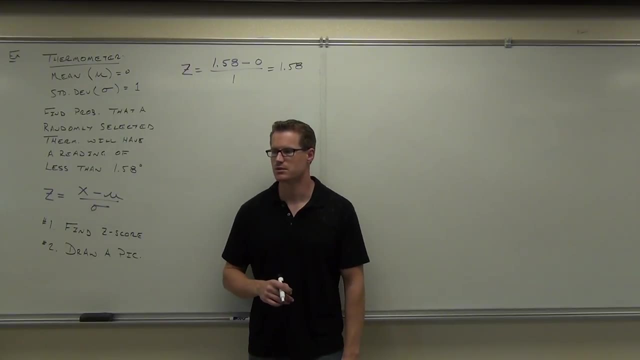 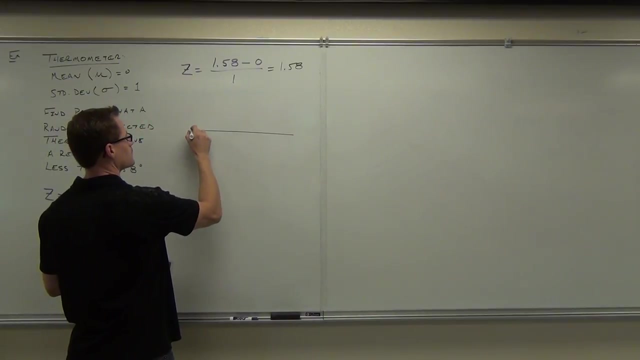 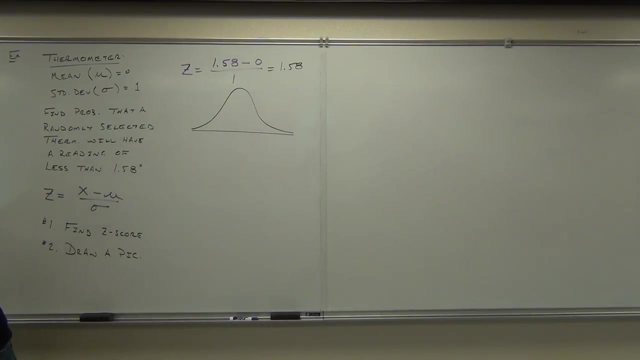 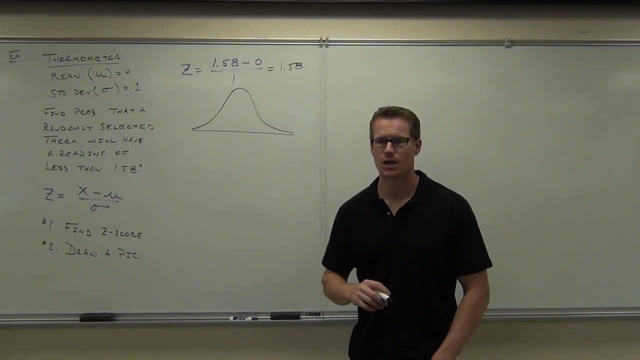 The z-score translates a normal distribution into What's the z-score you work with. Read through your notes if you have to. I don't care what you do. Figure that one out, Talk about it several times. so far You have an infinite number of normal distributions. 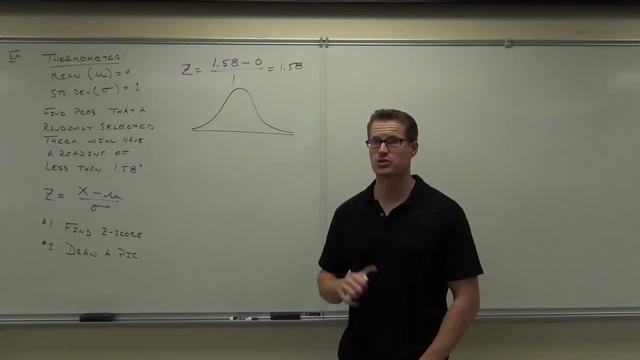 You use a z-score to translate those infinite number of normal distributions into one Standard Standard normal distribution. That's what a z-score does. You got to get this stuff. This class isn't just about doing simple mathematics. That's very simple. 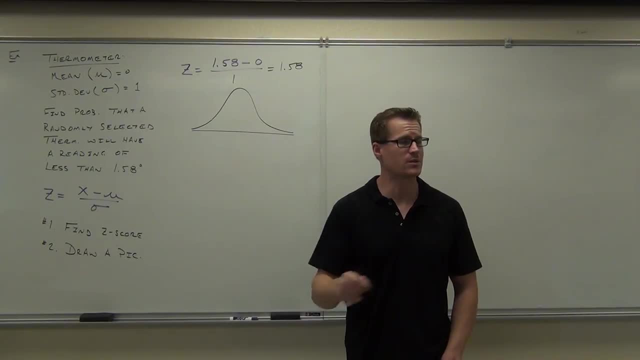 You have to have the understanding about what's happening here, Otherwise, when you get to chapter seven and eight, you're going to be lost. You're not going to know what to do. You have to understand it in this class. That's why this class is different. 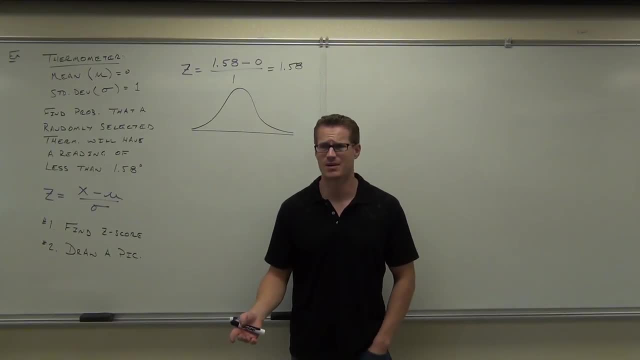 than like a Math C. Math C is pretty easy. I mean, really it's pretty easy. There's formulas, You plug numbers in, You figure it out. There's a set number of ways to do things. Statistics is different. That's why this is not a pure mathematics class. 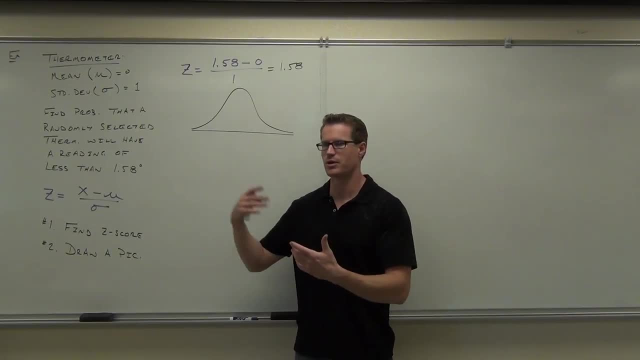 It's like sociology mixed with mathematics, mixed with critical thinking, So those three things pretty much combine. And so when you're doing this, you can't, just, It's not just good enough that Mr Leonard says: do this, then 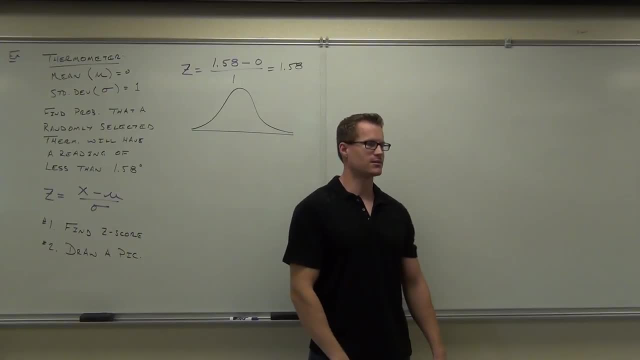 do this, then do this, then There's my answer. Yay, That's not good enough. You got to really understand what's going on. The x in this case is a continuous random variable. The x in the previous case was a discrete random variable. 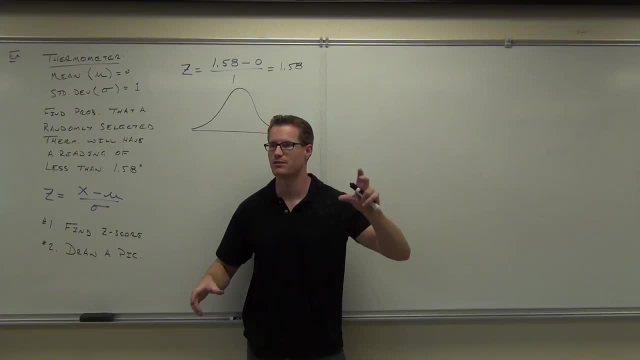 The reason why you have two different situations is because in one case you only have a set number of items. Here you have an infinite number of items. That's why we can't just find a direct probability for one value. I can't say: 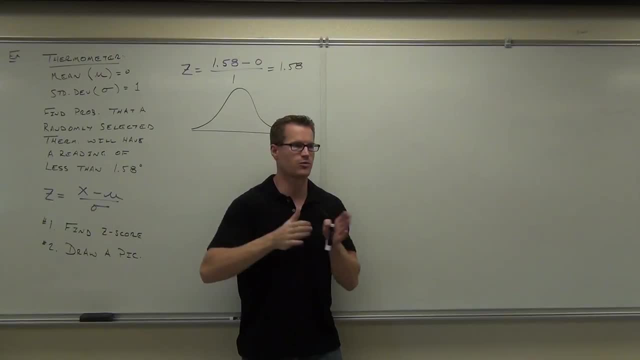 what's the probability of finding 1.58?? Because there's an infinite number of possible values. The probability of finding one in that infinite number is a needle in an infinite haystack. You're never going to find it. The probability would be zero. 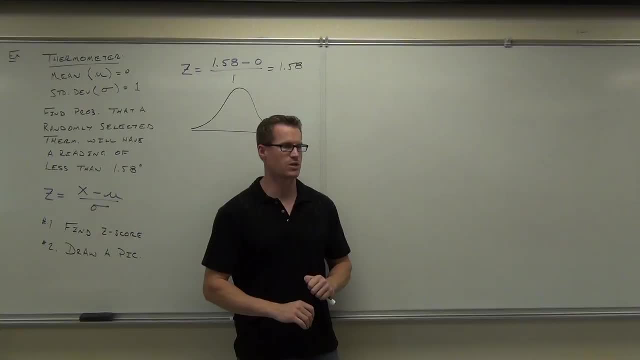 That's a different story than last chapter where I said: what's the probability of rolling exactly five threes or pulling out exactly one part out of a deck of cards? You could do that right, And we'll only find a number of choices. 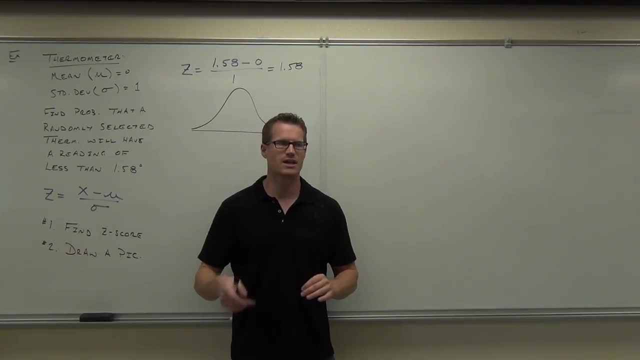 We're in a different story here. You can do that if you want, But you also need to know that we have an infinite number of possible normal distributions For every case that you can think of the distribution of age in a normally distributed population. 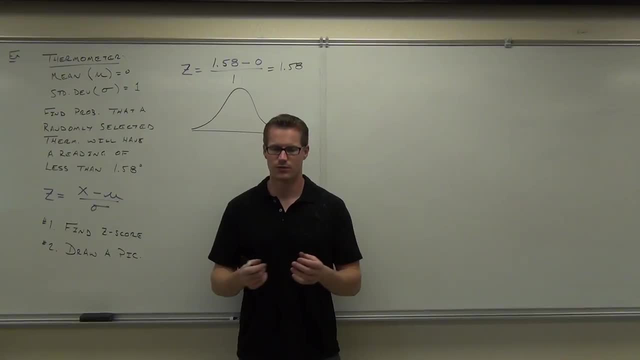 the distribution of heights or volumes of soda cans is normally distributed. There's an infinite number of those situations. We need a way to translate those things into something we can work with. You're not going to want to do an infinite number of problems, are you? 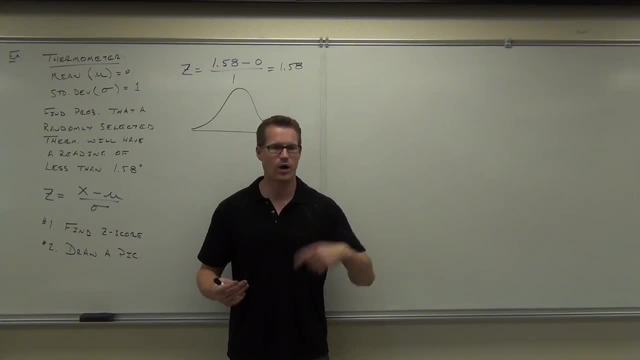 No, You want a way to do a problem, one way all at once. so you create something that's reasonable, so you don't have to invent something new every time. The way you do that is: you deal with a standard, normal distribution, The way you get. 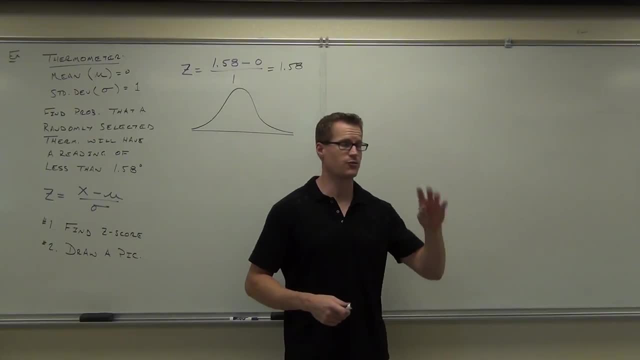 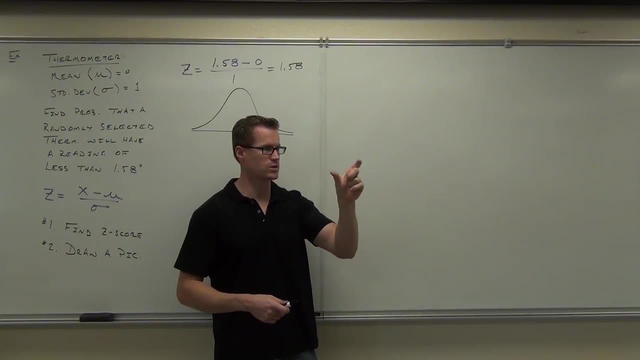 from a normal distribution to a standard normal distribution. I've shown this to you three times now. is you use a z-score? The z-score maps the mean to zero. It maps the standard one unit standard deviation away to one and two and three. 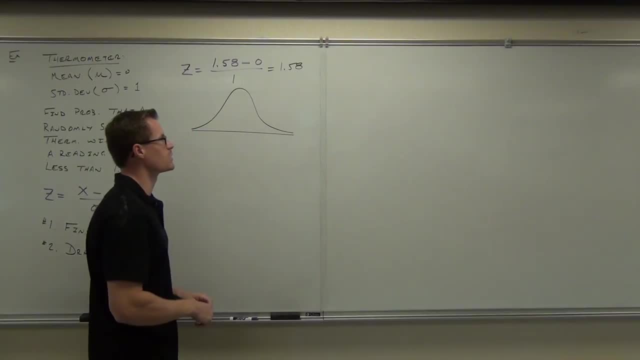 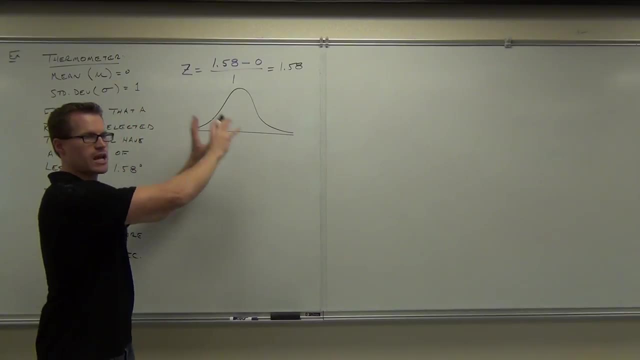 for those values that are two and three standard deviations away. So now that we've talked about it, we're mapping a normal distribution, any normal distribution, into a standard normal distribution. That's what the z-score does. If you haven't written that down, 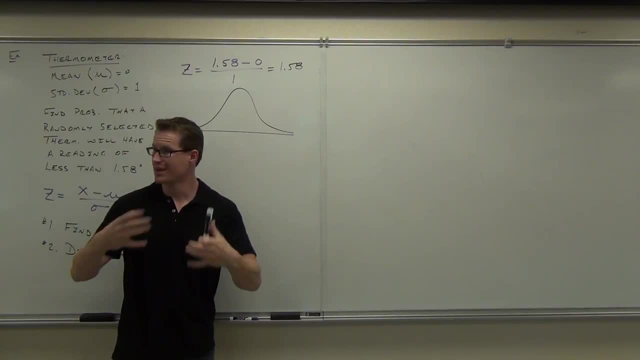 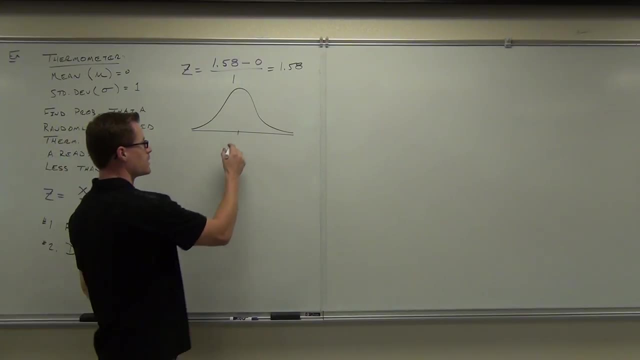 write that down. I mean, shoot, I'm not going to write everything on the board. We kind of need to pick that up. What is the center value for a standard normal distribution? Zero, Good, All right, Now here's what we do. 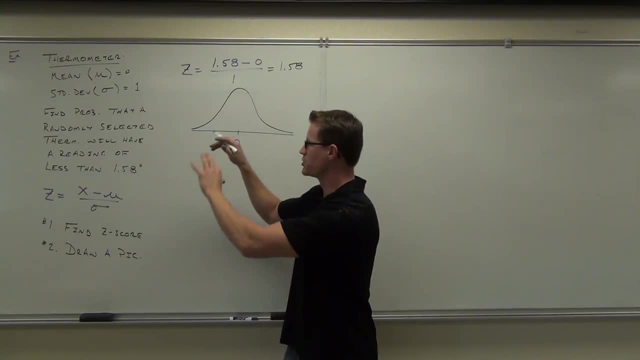 Since the z-score maps the normal distribution to a standard normal, we just have to draw one picture of standard normal distribution. You see, the cool thing about a z-score is it takes whatever value you have and it translates it into a z-score. 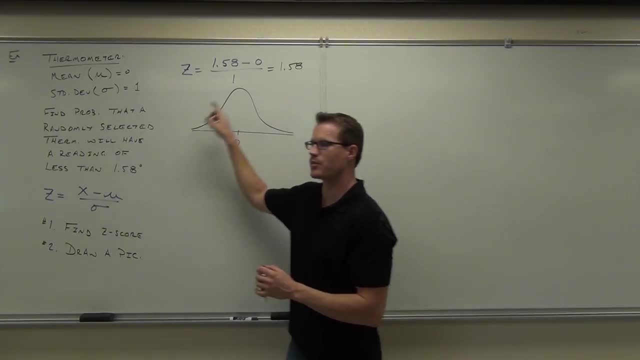 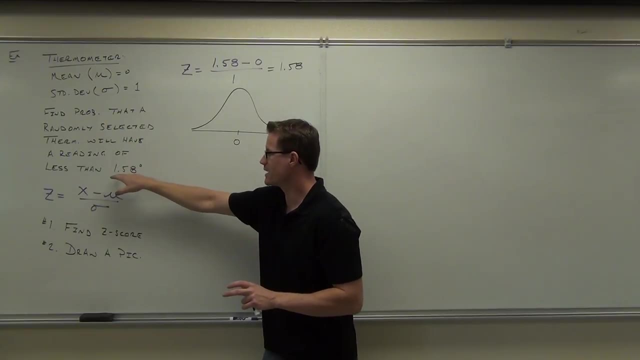 Now, in this very specific case it's the same number, because I chose these ones for you. I chose zero and one to make it easy, so you don't have to do a whole lot of math right now. But in this case it maps a number of degree. 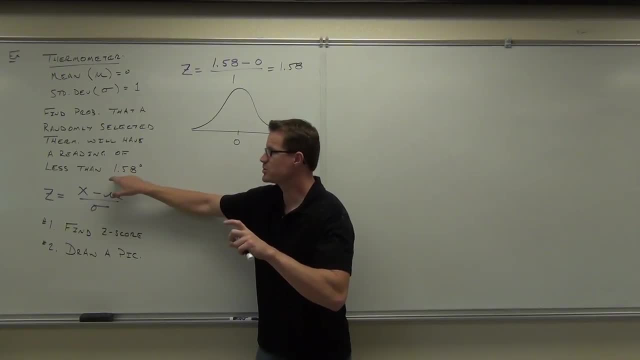 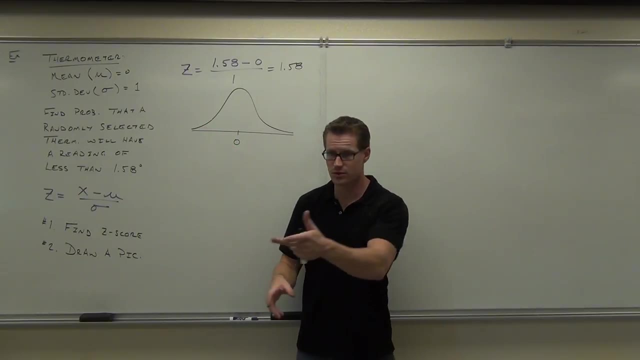 This is like 1.58 degrees right on the thermometer. It maps that to a z-score that we can put on the standard normal distribution, because that is just a listing of z-scores And I'm not taking a table and in your calculator. 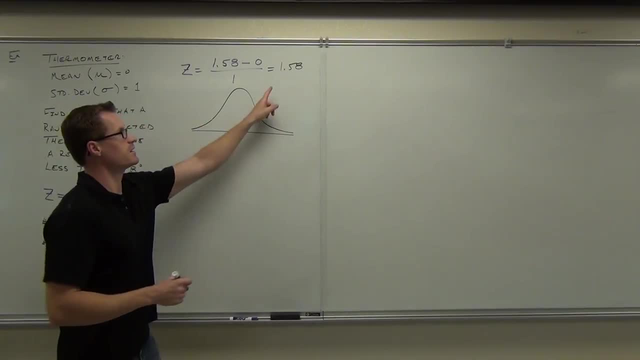 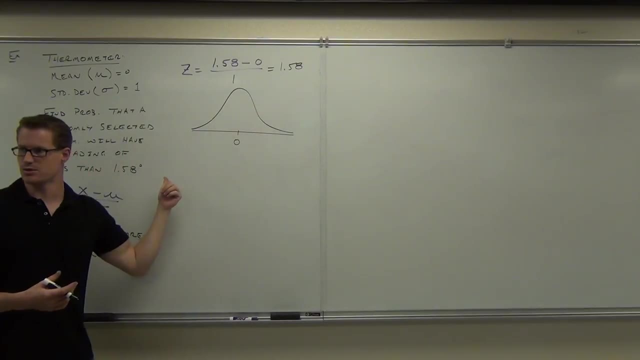 I'm just talking about z-scores there. So what we're going to do is we're going to place 1.58,, the z-score that represents my value, the z-score that represents my x. Are you understanding that? The z-score? 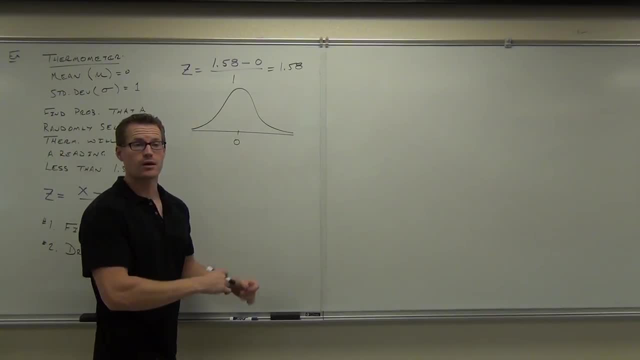 that represents that number somewhere on this chart. Where do you think it goes To? the left of zero or right of zero? Right, Sure, it's a number right Right Z-score is the problem About how far One and a half. 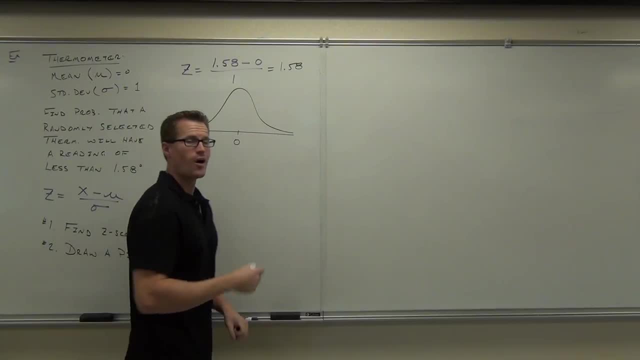 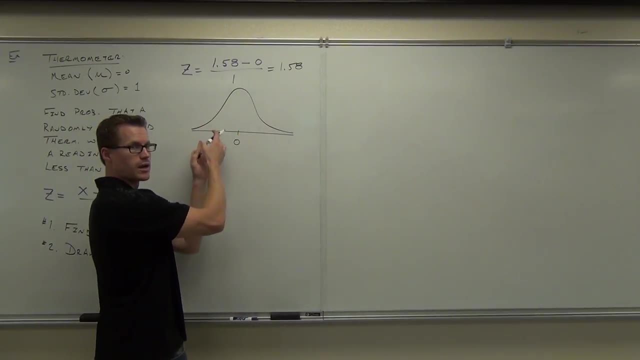 About one and a half. Yeah, if you want to do one and a half, honestly, it doesn't really matter all that much. This doesn't have to be to scale, It doesn't have to be perfect, I just need to know. 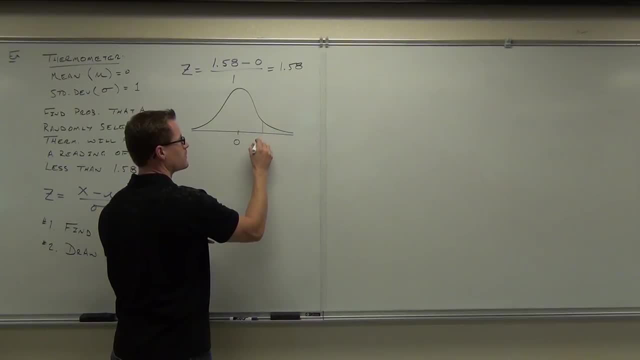 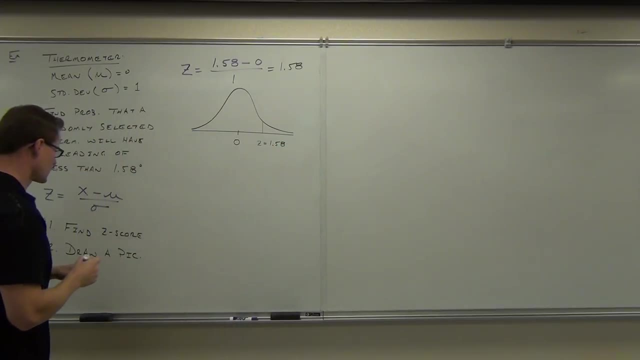 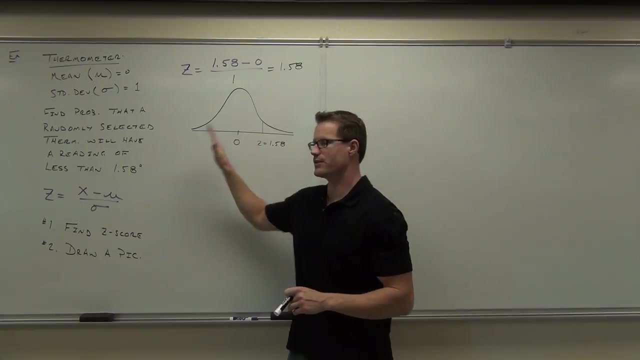 basically to the left or to the right. Positive is to the right and negative is to the left, So we're going to put 1.58 right here, And then what you're going to do is you're going to shade one side of this graph. 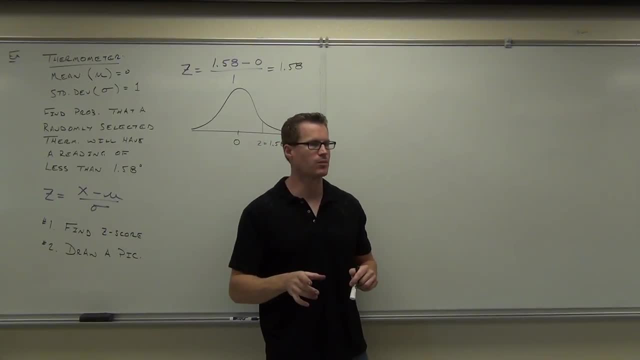 And here's the reason why We just spoke about this a second ago. I can't ever ask you to find the probability of selecting a thermometer that has exactly a reading of 1.58 degrees. That was the needle in an infinite haystack concept. 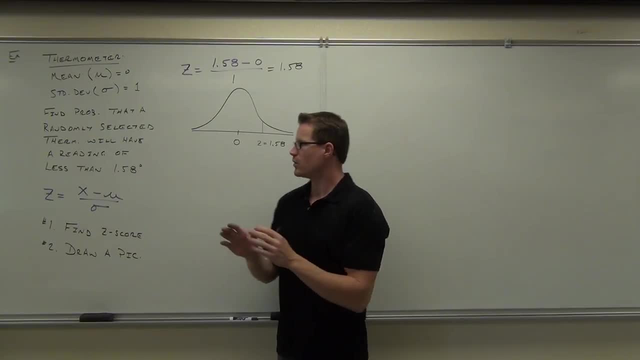 that we talked about a couple of times. Also, the area under this. you have to know this one. what's the area under this whole curve? 1. Good, That lets you associate area with probabilities. You with me, I can explain this. 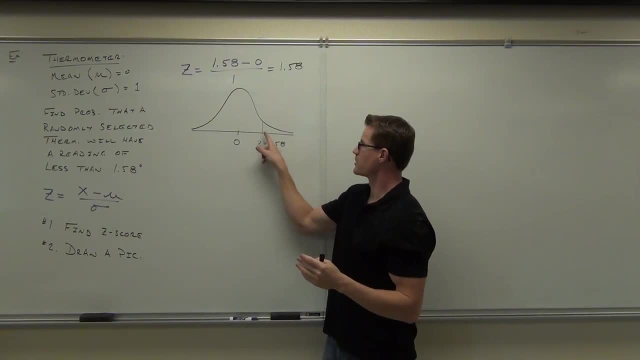 in a different way. now, What's the area under a single line? What's the area of a line? What's the area of a line? Can you find the area It's got? a height area is height times width right. 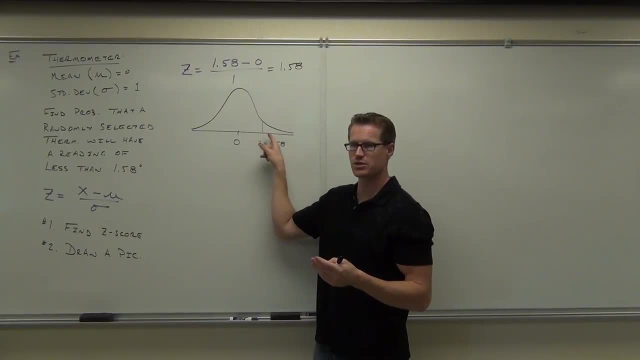 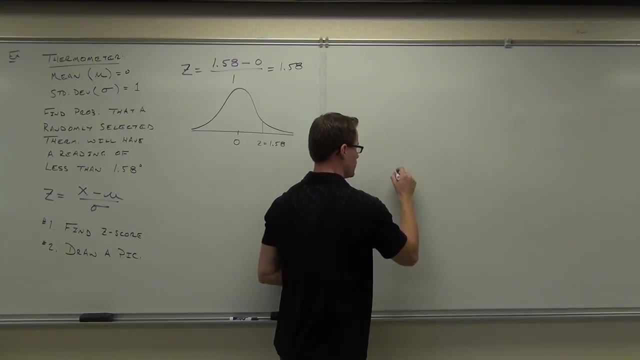 The height is. who cares? the width is how much? What's the width of a line, basically, is what I'm asking you: 1. The width of a line is 1? 0. This would be like a width of 1, right. 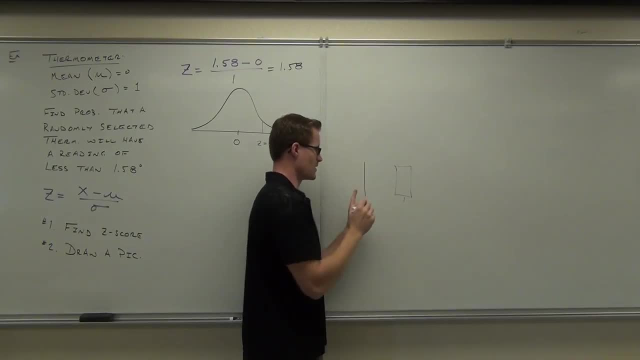 What I'm asking you is: what's the area of that? It doesn't have any, Because a line is supposed to have no breadth right? A line is only 1, dimensional, It just goes up, It doesn't spread out. 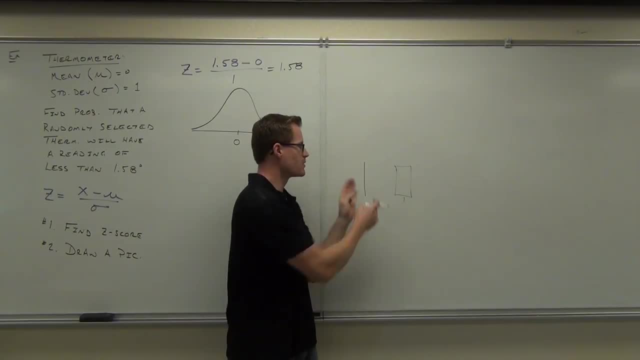 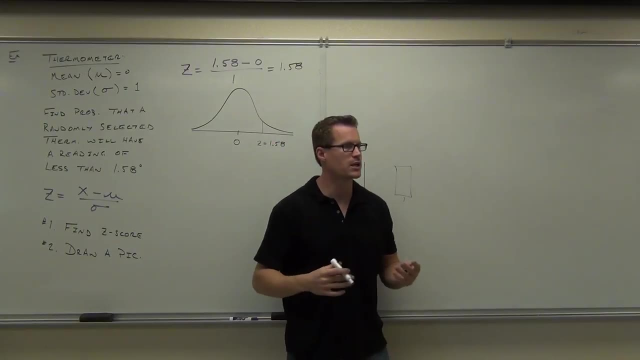 Even though we draw it on paper, it has a little teeny bit of width. There's actually no area here. So if you're trying to find the area of a line, is there any area there? No, So the probability of this value 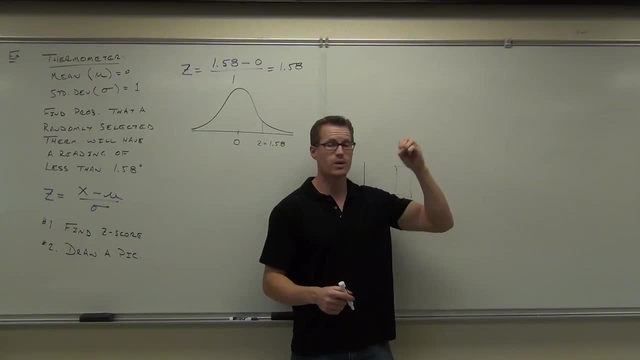 finding exactly that value is 0.. It's 0.. That's two ways I've explained it now: The area concept and the picking out one value out of an infinite number of possible values. You just can't do it because the probability is 0.. 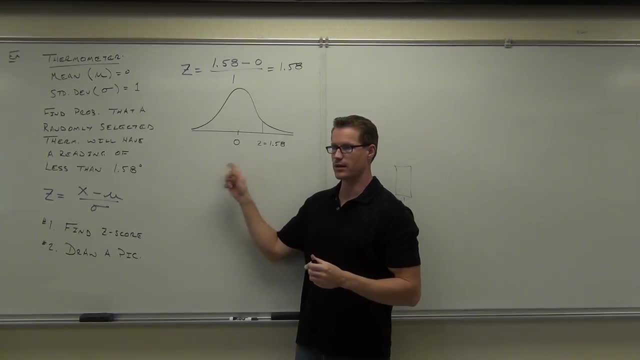 You can't find the exact value of a number like this in chapter 6 in continuous random variables? No, Discrete. Yes, We just talked about discrete chapter 5.. Chapter 6?? No, Not so much, We can't do it. 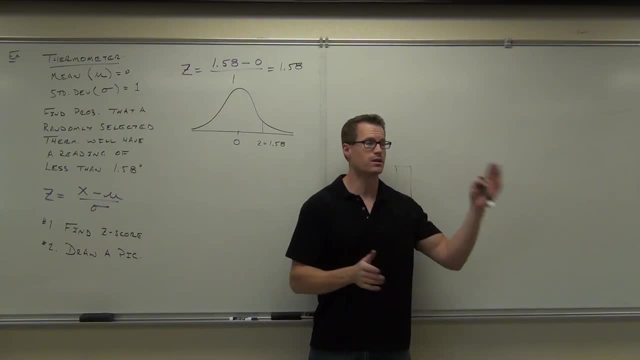 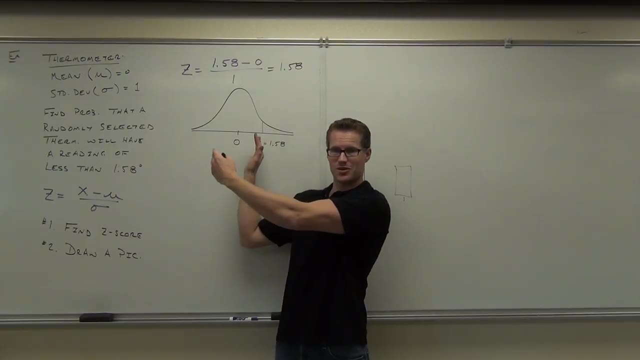 So it's always going to be this situation. What's the probability of finding a thermometer that has a reading less than something or greater than something, or between two numbers? That's the only things you're going to get. You can either do less than 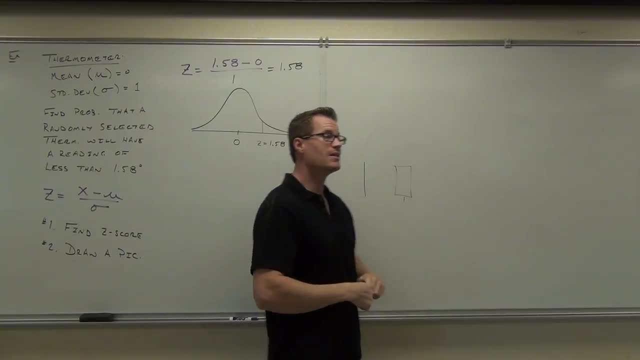 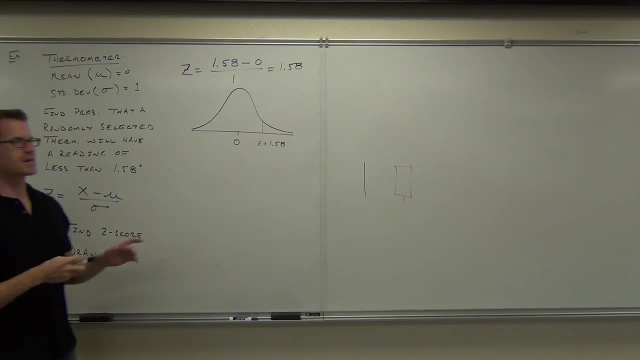 greater than or between. There's only three situations In this case. what am I asking you for? Am I asking for values greater than, less than or between? What do you think? Let's read through it. Where would less than be? 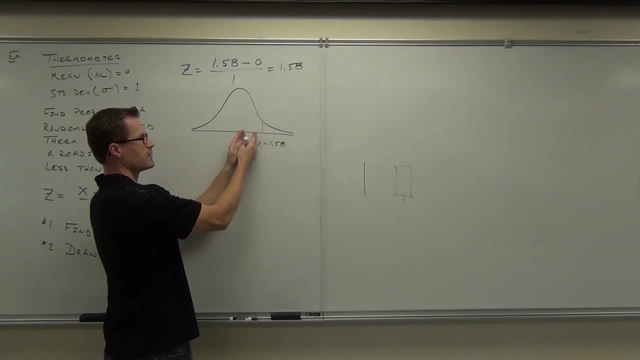 To the right or to the left, To the left? Yeah, These are the readings of z-scores that have 1.58 and less. Here's 0.. Here's some negative z-scores. This would be greater. So what I'm asking you is: 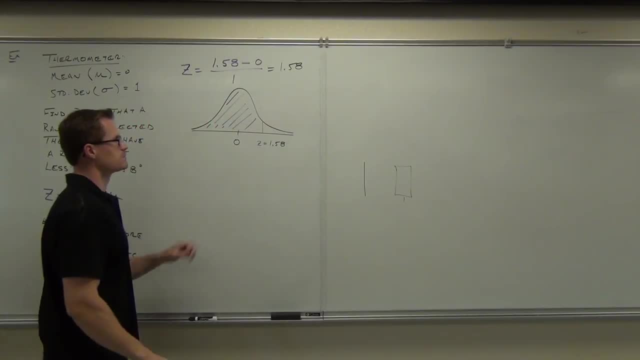 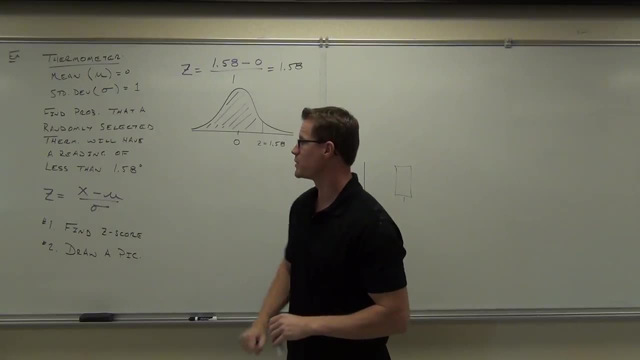 what's the probability that you're going to randomly select a thermometer and it has a reading that's over here on the screen. Okay, So let me kind of recap our situation. We're dealing with continuous random variables To translate a normal distribution into a standard. 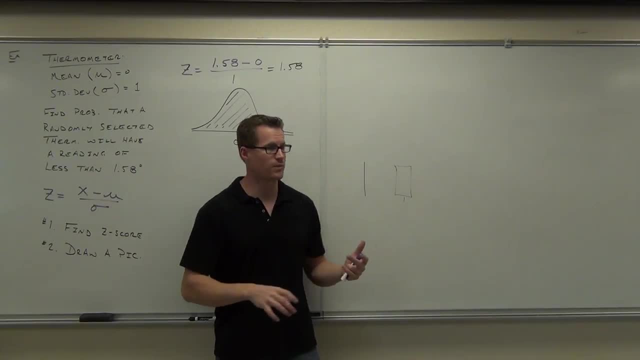 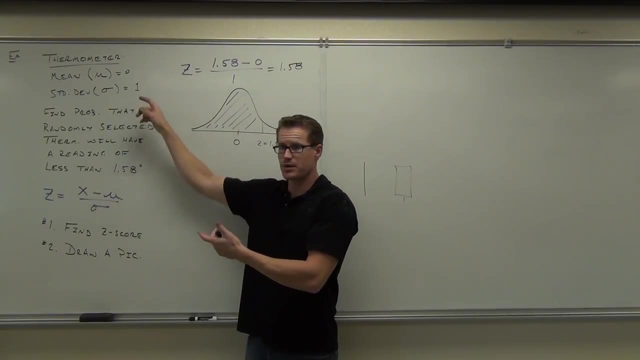 normal distribution. we've got to use the z-score. That's what we're going to do. We plug in our x, which is our continuous random variable. We're going to be given a mean and a standard deviation per population. We use that. 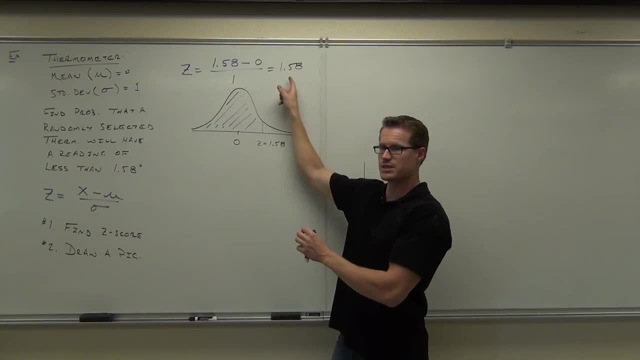 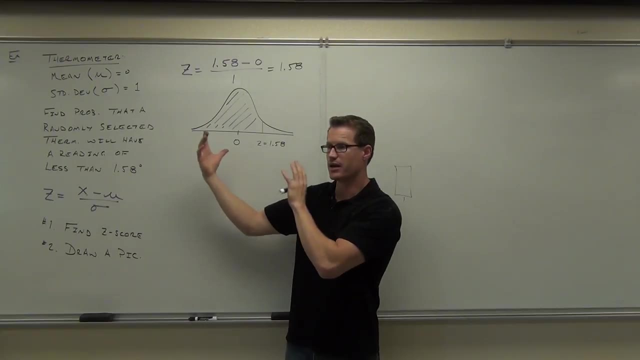 to get a point, that's a point, value the z-score. That z-score gets placed on our standard normal distribution and now we can find the area that's associated with our picture. So important steps here: Find z-score, draw a picture. 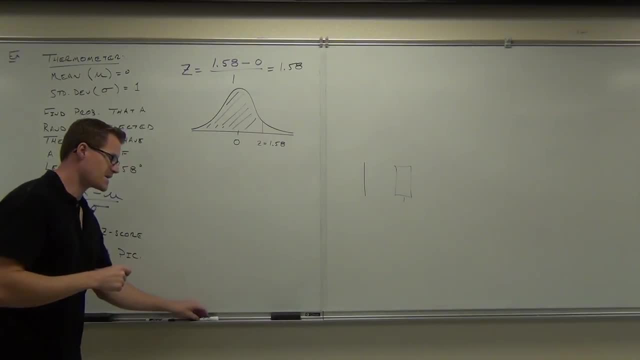 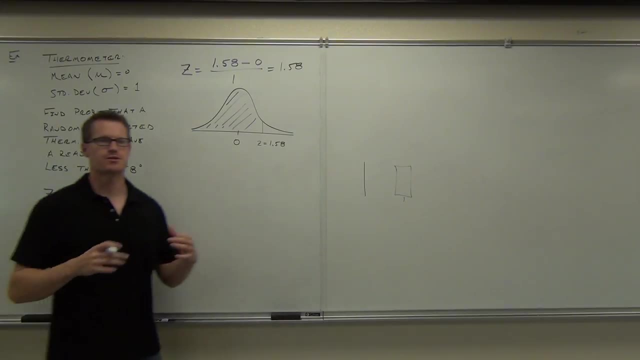 Now we're going to calculate or look up the area, or find the area, And by finding the area we actually find the probability. Now there's two ways to do it. You can use a table, or you can use a calculator, or you can use 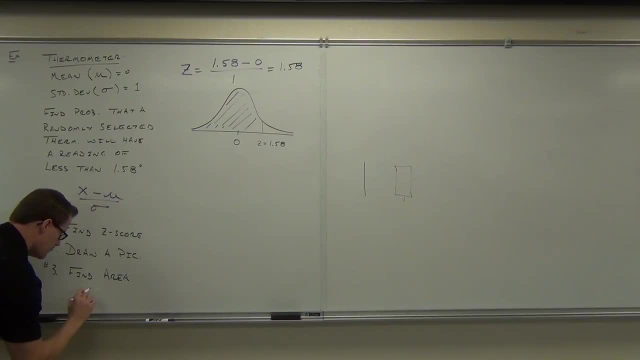 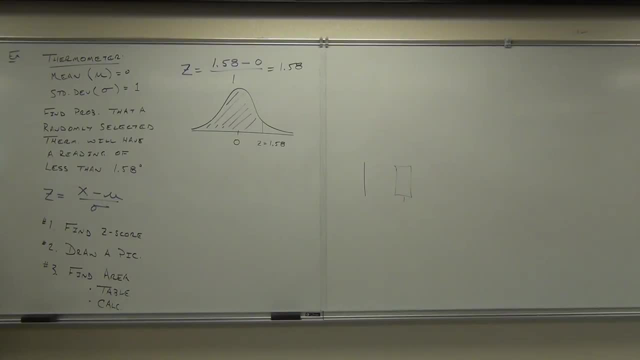 I'm sorry about that. The table you're going to be using is table A2.. Maybe I'll move it up here so you can see it. So you're going to be using table A2.. So you're going to be using? 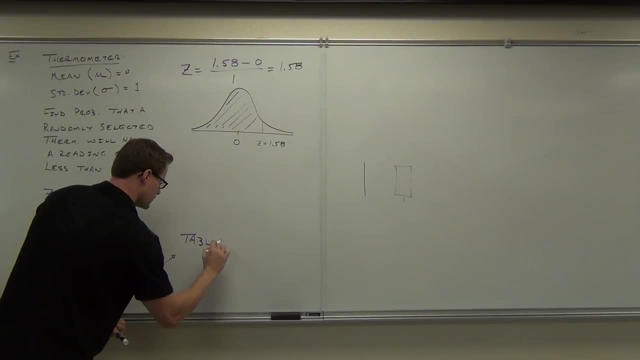 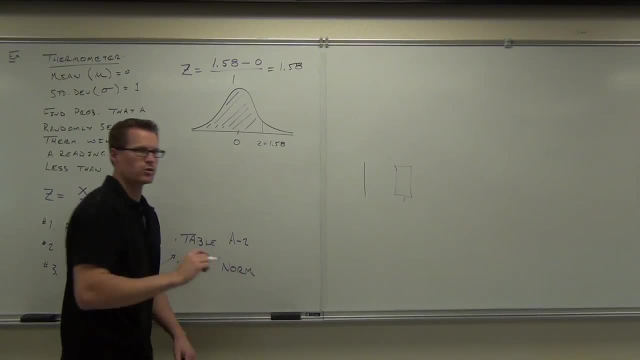 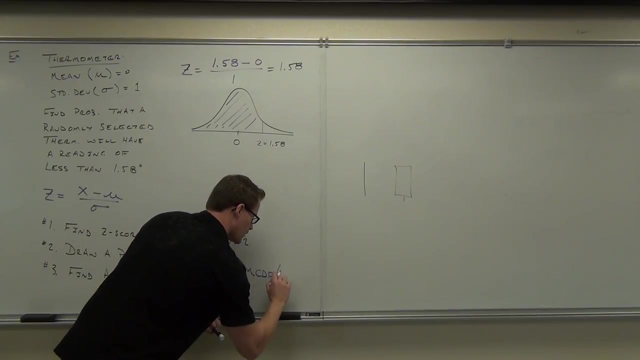 I'll show you how to get there, but you're going to be using something called normal, Normal. Why normal? Why normal? Hey, we're in a normal distribution: Normal, c, d, f, cumulative, cumulative, Cumulative. That's what the 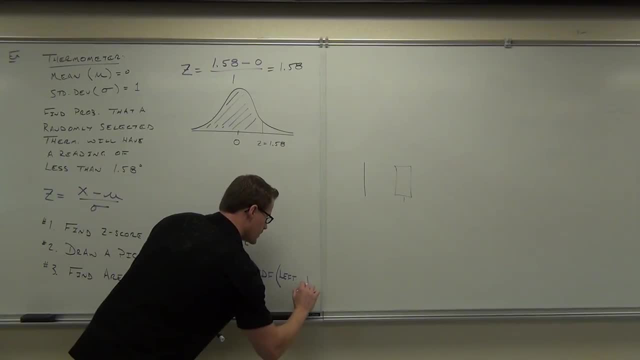 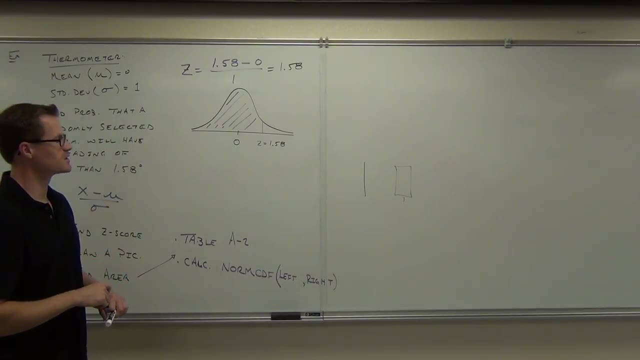 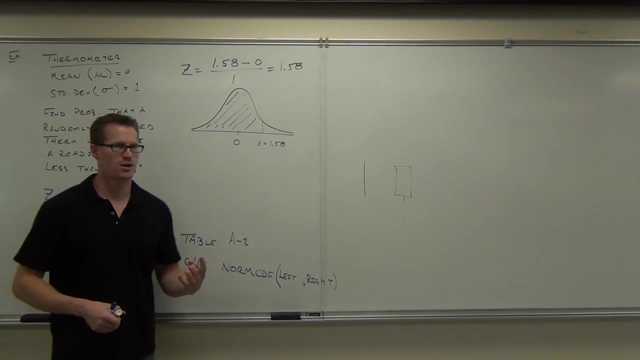 c means And you're going to put in your left. I'm not supposed to write on that. we'll see if it comes off, but it's right there. So we've got two options here if you don't have a calculator, a graphing calculator. 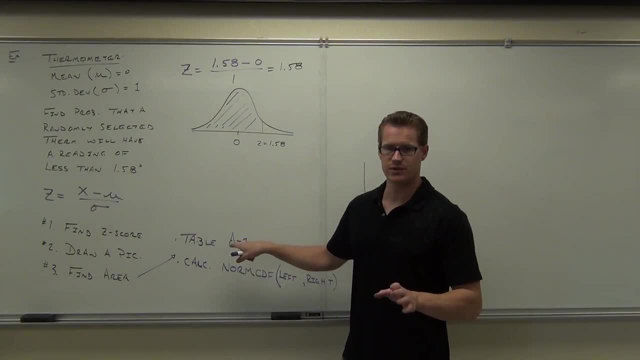 a statistics calculator. use your table. it's there for you. you can use it every time If you have a calculator. it's easier. this class is way easier with one of those calculators. you just plug in the left z-score and the right z-score. we're going to talk about that. 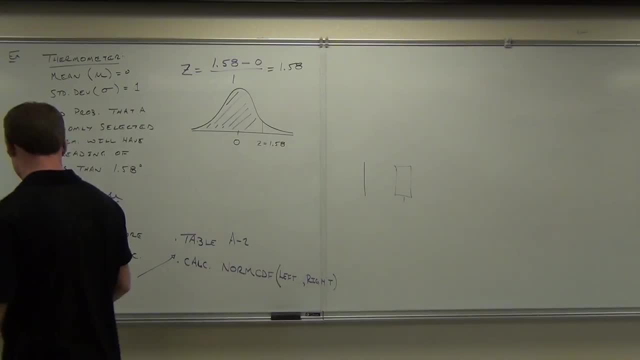 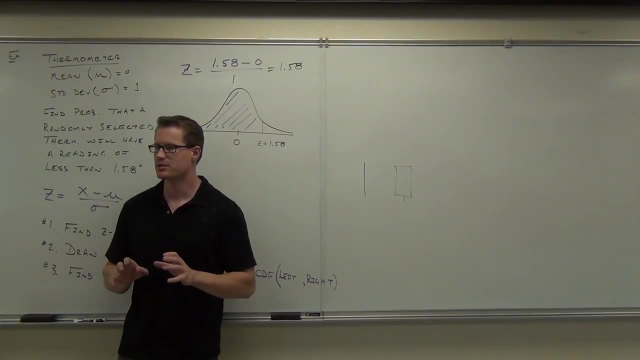 in just a second. the left z-score and the right z-score. just talk about it right now. For those of you who have a calculator, I'm going to show you on your calculator in just a second. but I need to explain something first. 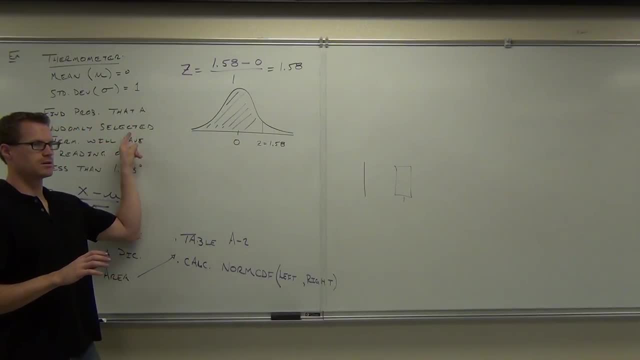 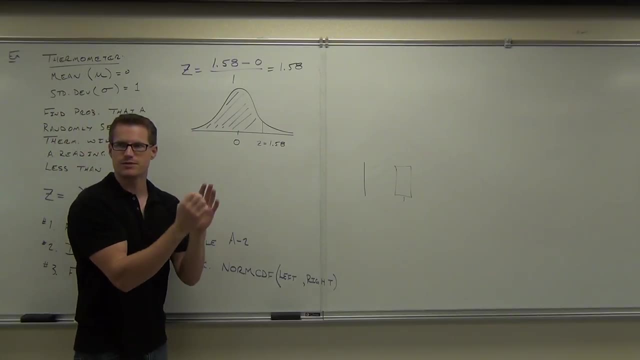 Does this ever end? No, Okay. so if I want a starting spot for this area, I know the ending spot. look up here at the board, please, if you have a calculator, the ending spot. my right z-score for this area is 1.58,. do you agree? 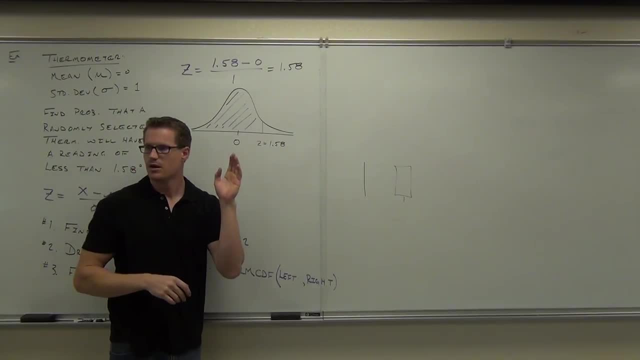 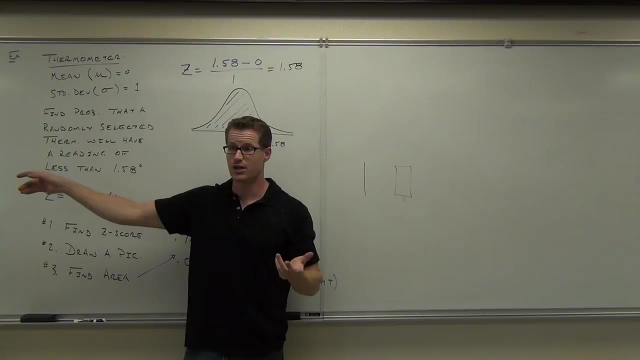 No, The question is, where do you start? I mean, basically this goes to negative infinity. that's where that thing goes. you can't plug in negative infinity on your calculator. So when you have a situation where you want to find an area from where it's like negative, 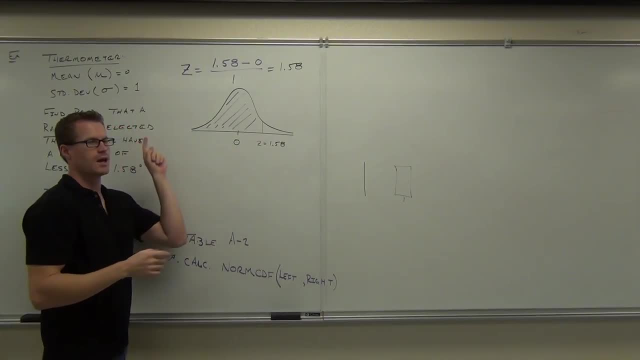 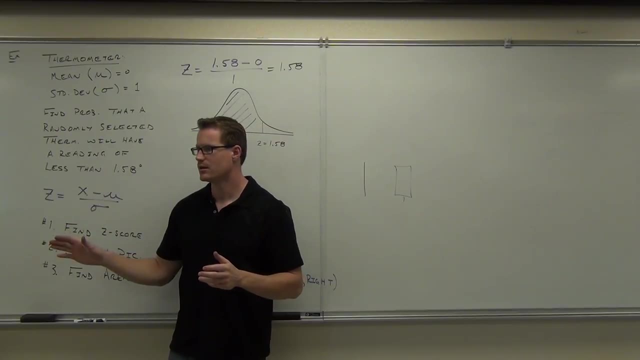 infinity to a number. you can go far enough to the left where it makes no difference really, and that number is something beyond like negative 5 or negative 6, I always plug in negative 10. Because if you go past, I mean the probability of it being negative 10, it's going to be. 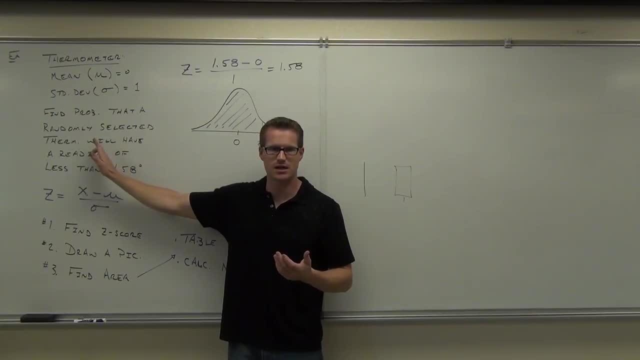 negative 10.. The probability of getting a value less than negative 10 standard deviations away from your mean is so small it doesn't even make a difference anymore. It's so close to zero it might as well be zero. does that make sense? 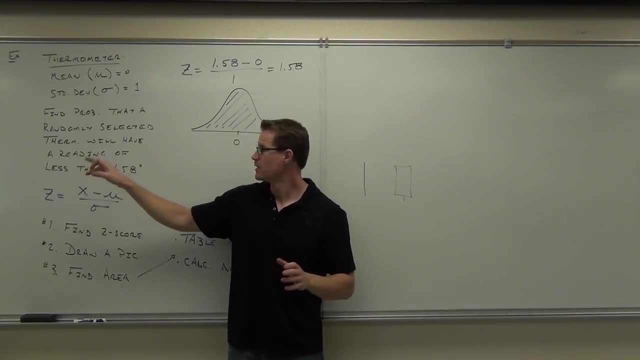 So if you have a calculator where you start from the left is negative 10, just put in negative 10.. I know that's not negative infinity, this thing actually doesn't stop at negative 10, but that will give you a precise approximation up to at least 6 or 7 decimal places. you. 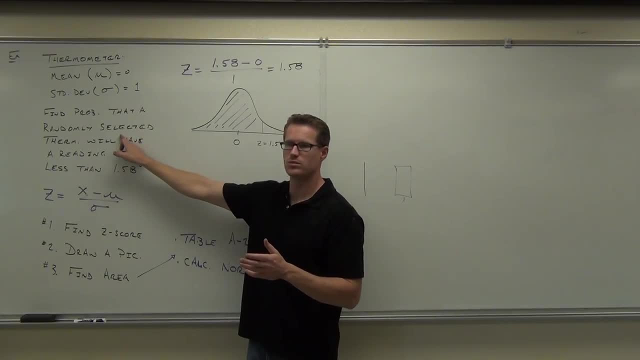 okay with that. So does it actually start at negative 10? No, no, But the area doesn't ever end. we're just picking some ending spot where our calculation is not going to be off tremendously. Are you with me? Are you sure? 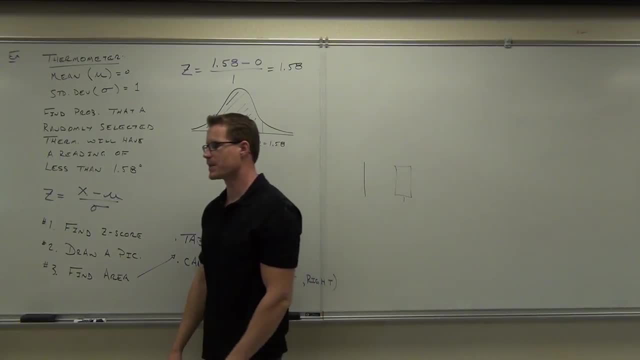 Okay, let's try this on a calculator. So what we're going to do right now we're going to look at that table, the z-score table. I'm going to show you how to do this with a table. then, right after that, I'm going to 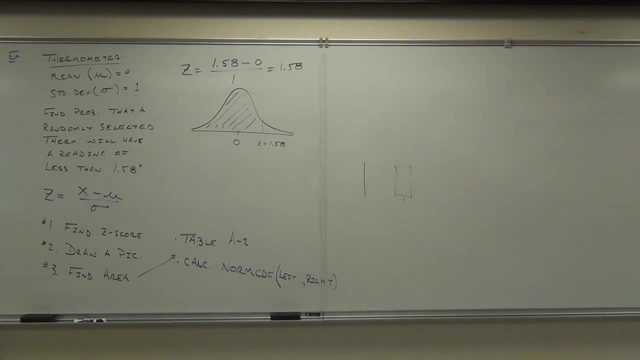 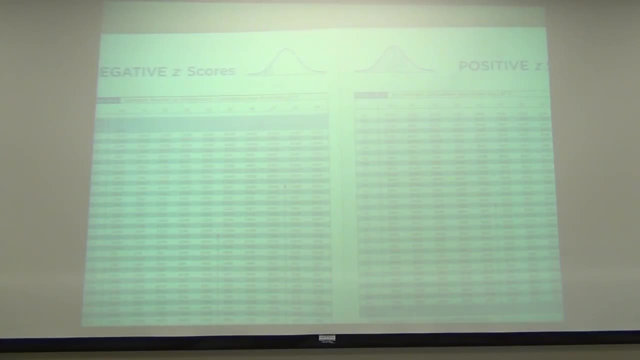 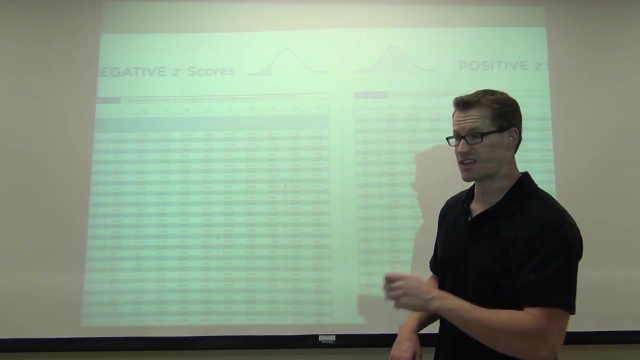 show you how to do this with a calculador. Did I say that right? Calculador, Calculador, All right, so you shouldn't have your table A2, hopefully you have that thing with you and have that out, because you need to play along with this, because you know how to use. 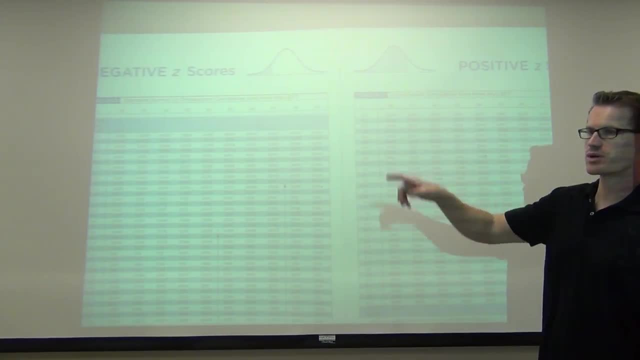 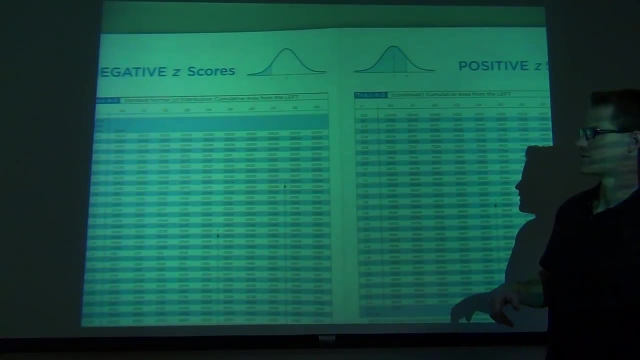 this thing When you look at your table A2, you're going to notice at the very top of your screen. by the way, can you turn off one of those, one or two of those lights? That works, That's fine. don't take a nap on me now. 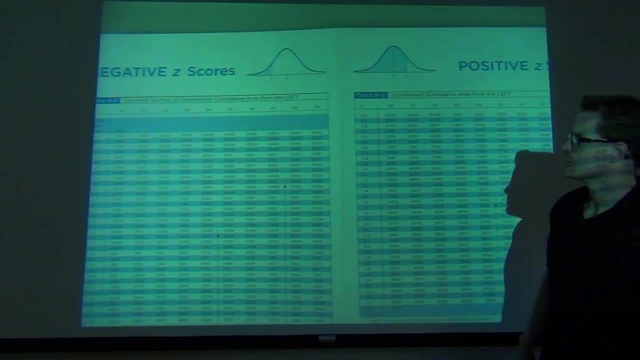 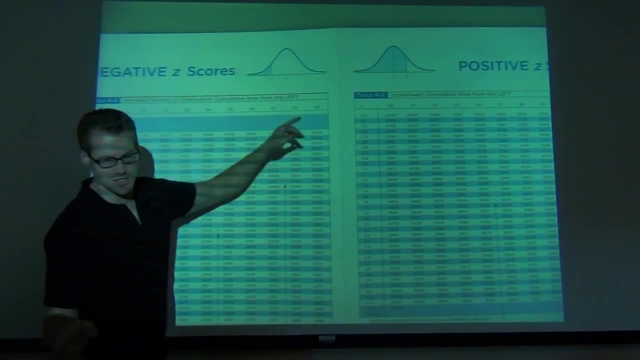 If you look at the top, we've got two different situations here. We have something that says it's not negative. actually it's negative, so there's a little end there. that's not on the screen, but you should see that on yours. 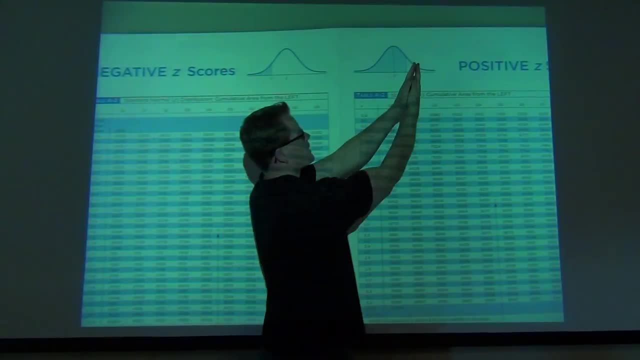 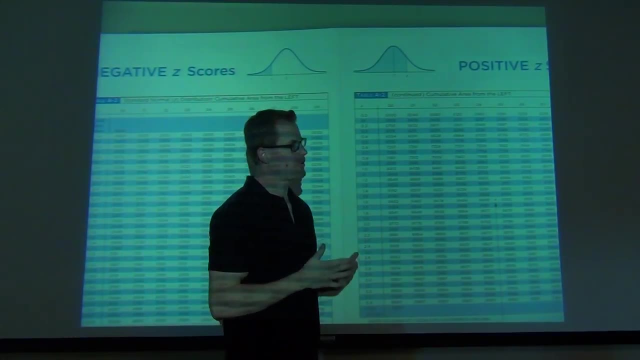 or positive z-scores, But you're gonna notice that every situation it's shaded to the left. You see what I'm talking about. So that shading that says that whatever value you look up, it's just gonna give you the area to the left. 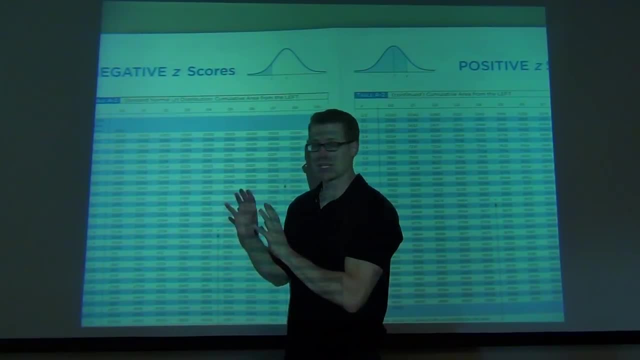 of whatever you're telling it. Does that make sense? So in this case that's gonna work great, because I'm looking for something that's less than 1.58.. If I was looking for something that was greater than well, then that's another story. 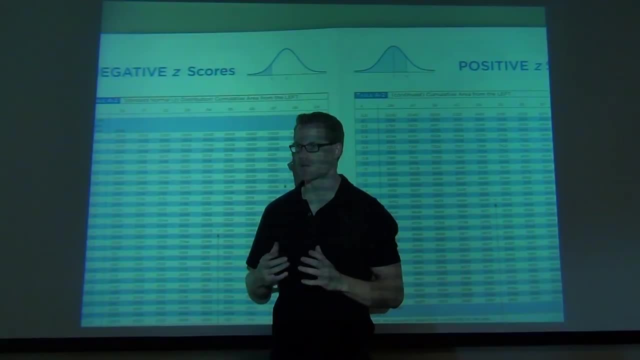 This is not gonna give you this. This is not smarter than you are. It's not smarter than your problem is. You have to know how to manipulate this thing to get what you want out of it. This only does one thing. This gives you the areas to the left. 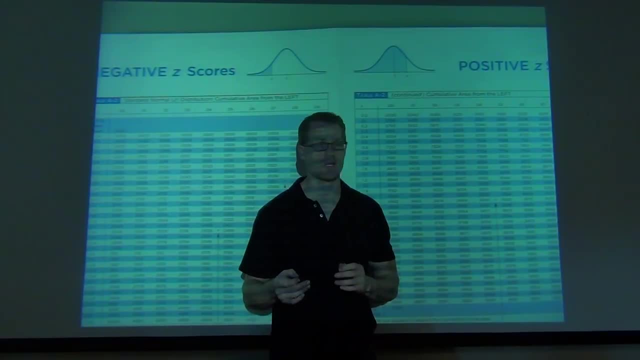 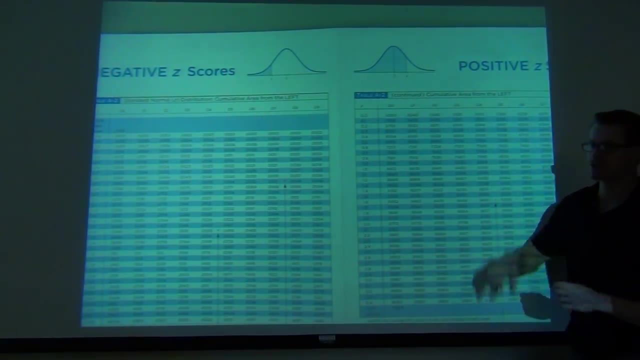 of whatever value you look up- Not sure if you're okay with that- It's always to the left. That's why this is shaded to the left and it says right here: cumulative area from the left and from the left. So let's go ahead and see if we can do this. 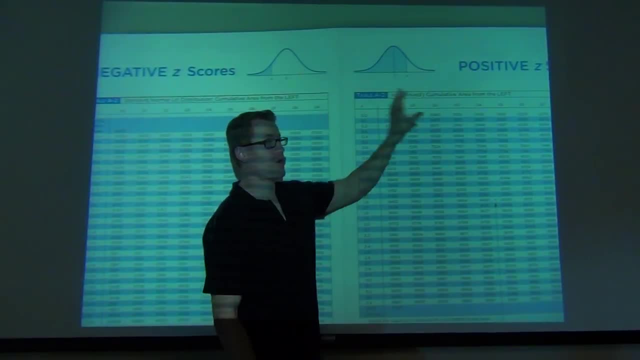 Should we be looking, do you think, in our negative z-scores or our positive z-scores? What do you think? Positive? Yeah, definitely, because we have a positive z-score. So let's look at that positive z-score. 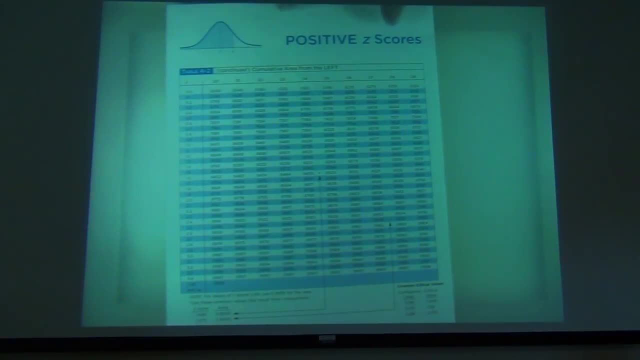 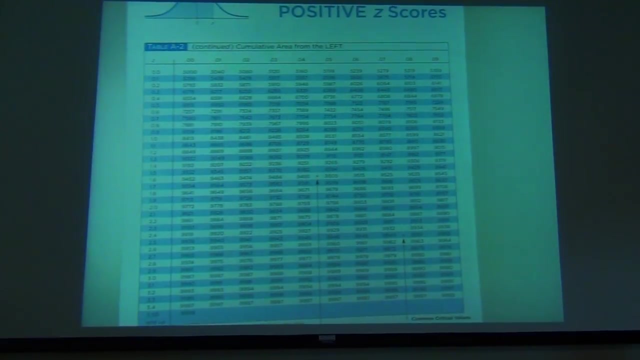 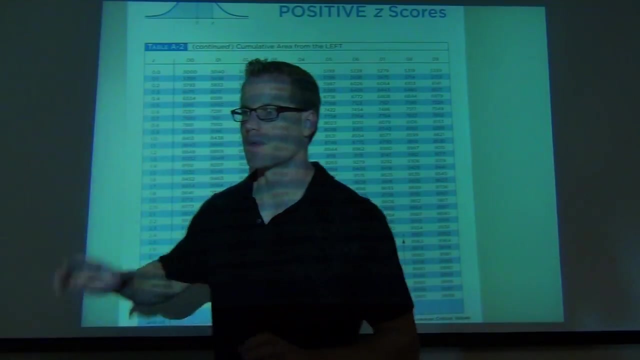 If we're looking just at the positive z-scores here, Can you read that? okay, Here's how you use it. Your z-score is always going to be one point, something, something. You're going to round to two decimal places because that's what your table gives you. 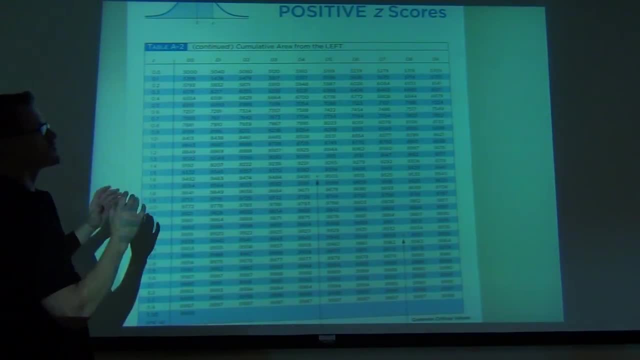 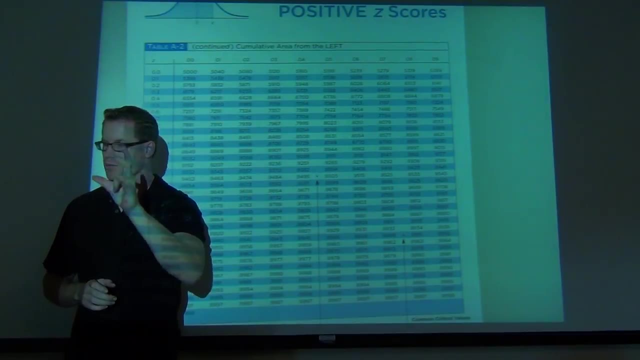 So when you round to two decimal places, ours was 1.58.. How you use your table, this will give you the one point to the tenth, This will give you the one point to the tenth, or two point to the tenth and then the hundredth value. 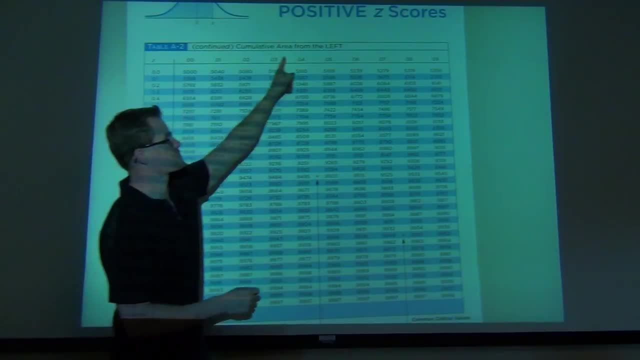 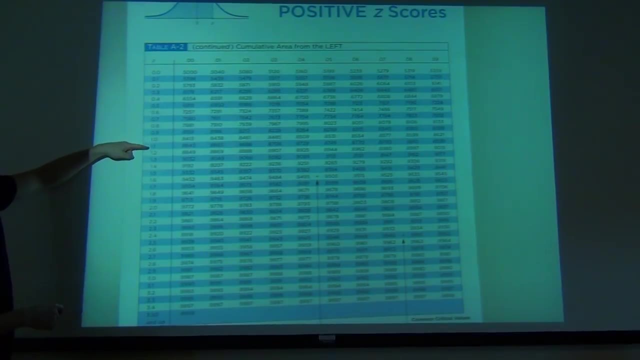 which is like our eight in our case. so we have 1.58, will be given by this column. So here we go. Z-score is one. Where's 1.5? 1.5,, that gives you the 1.5.. 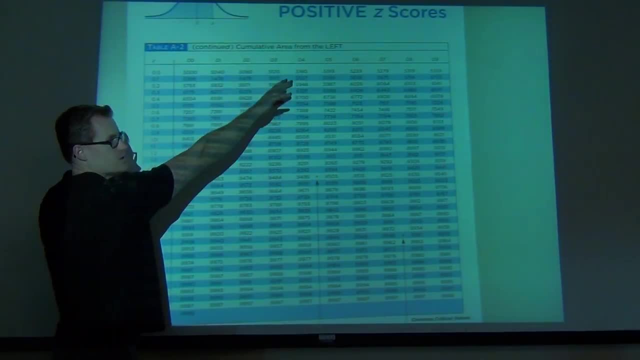 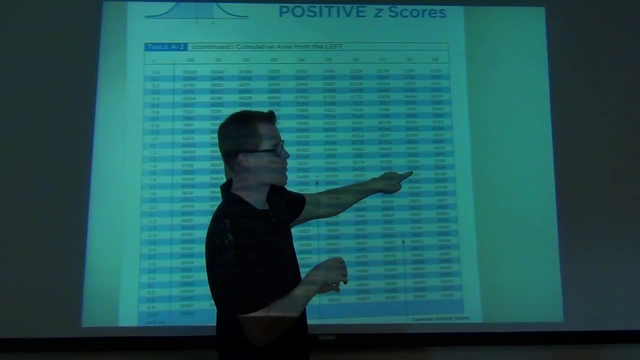 To get the. this is why it says 0.0,, 0.0.. To get the 0.08, you're going to go 1.5 all the way over there, 1.58.. If you look on your table, you should be looking at 0.9429. 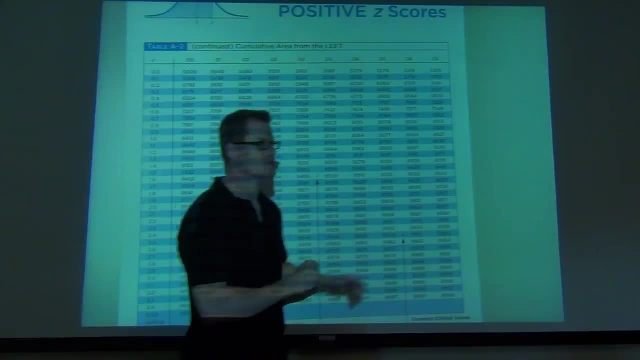 Was everyone able to find that Awesome? Okay, so that's how we look up z-scores. Any z-score can be done the same way If I wanted 0.429.. 0.429. 0.429. 0.429.. 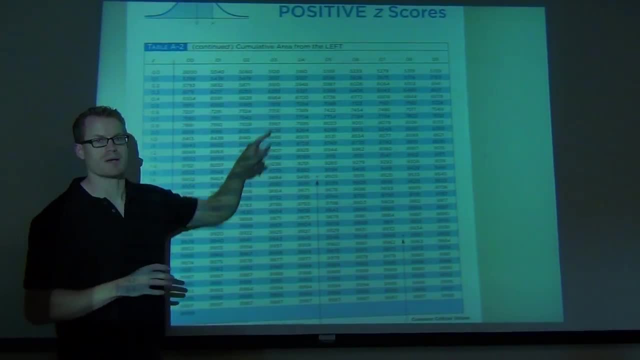 0.429.. 0.429.. I'd go to 0.4 over the 3, that would be my z-score. What this is giving you is an area to the left of that number, to the left of that z-score. 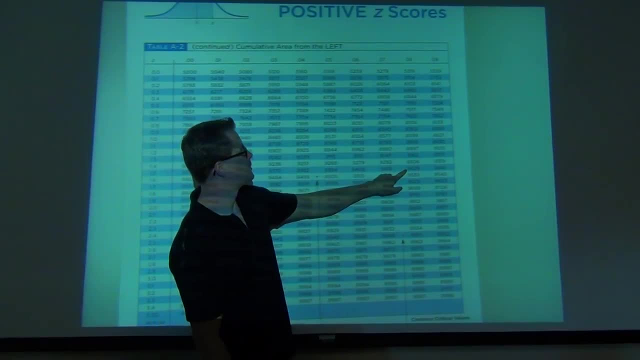 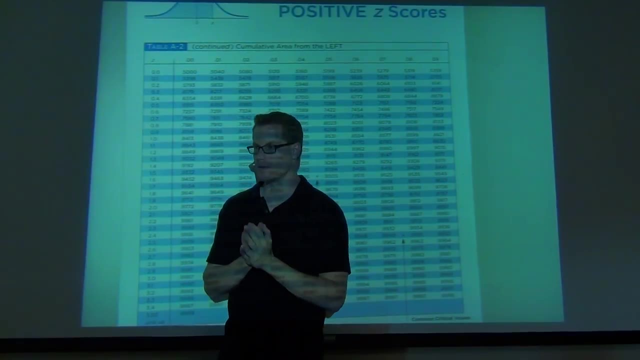 So in our case, our area- let me look it up again- 0.9429,. that's 0.9429, or 94.29% of the area, is to the left. That's what this is saying, And in a moment we're going to translate that area. 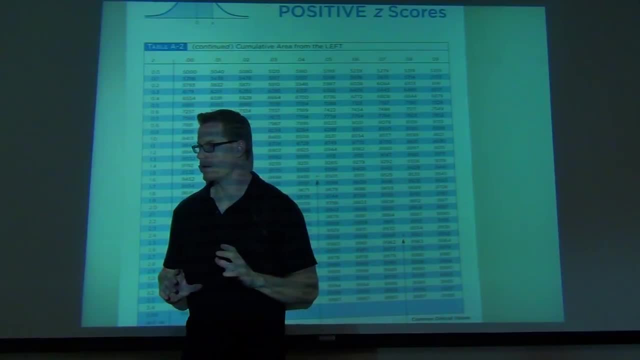 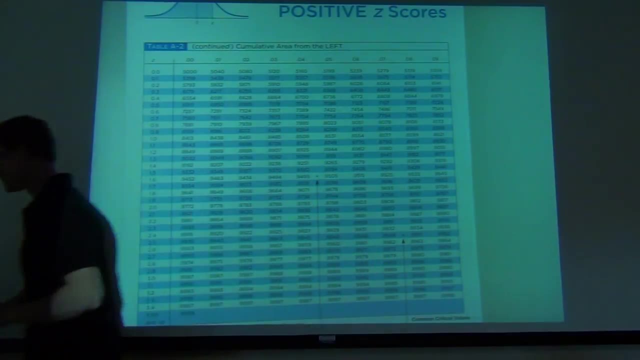 into a probability and realize that we're talking about the same thing. Now for the calculator. would you like to see how to do it? Okay, you're sure You ready for it, So take out your calculators, Here we go. 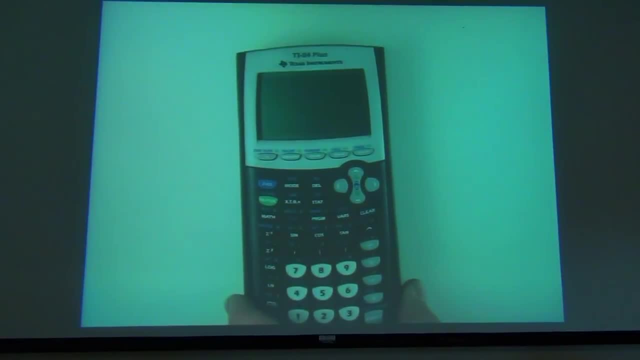 So let's turn that thing on. Do you remember how to get to the binomial distribution? Yes, If you do, it was a distribution right. So you're going to go to your distribution button that second and then the VARS button. that's right here. 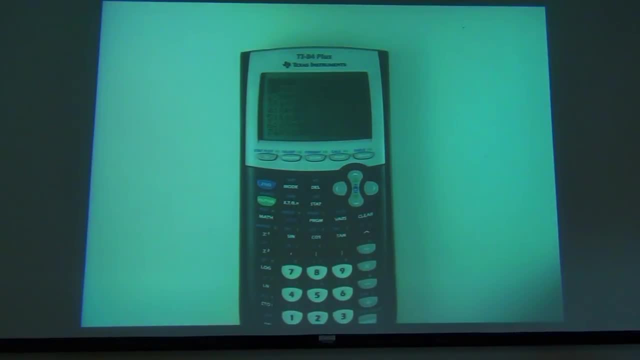 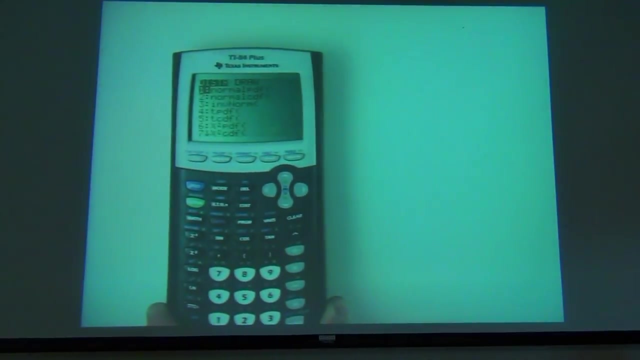 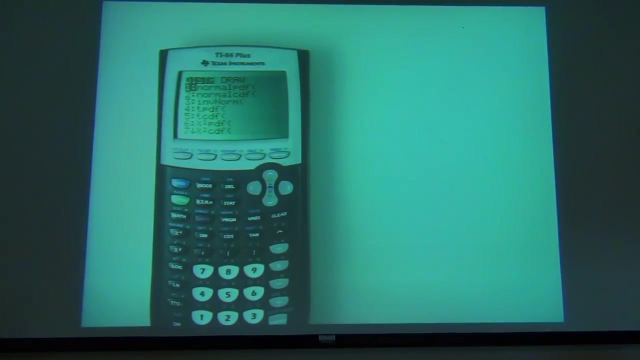 That's going to give you your distributions. Can you read that? okay? Can you read that screen? Not really, huh Better. Yes, All right, And right up at the very top, you've got yourself normal PDF and normal CDF. 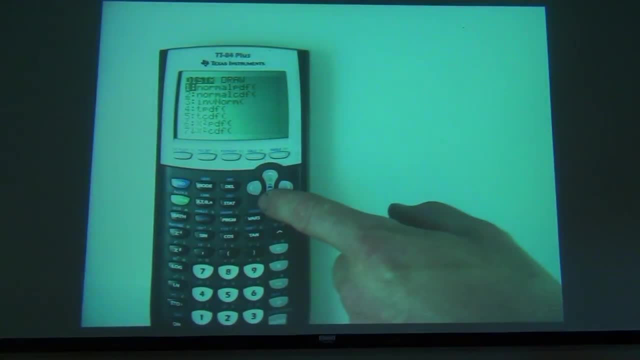 You're going to go to the CDF. You want a cumulative distribution. It's going to give you everything from the left over. We press Enter. It says normal CDF. All you've got to do is put in the left the starting z-score. 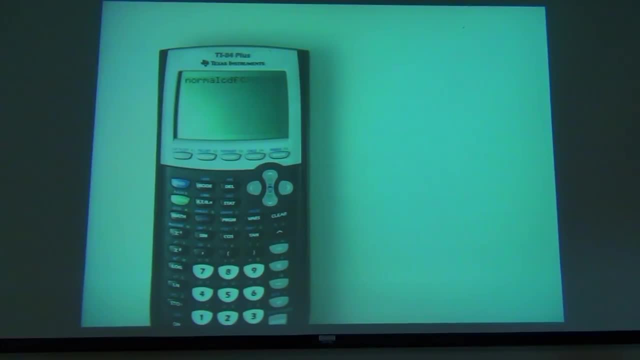 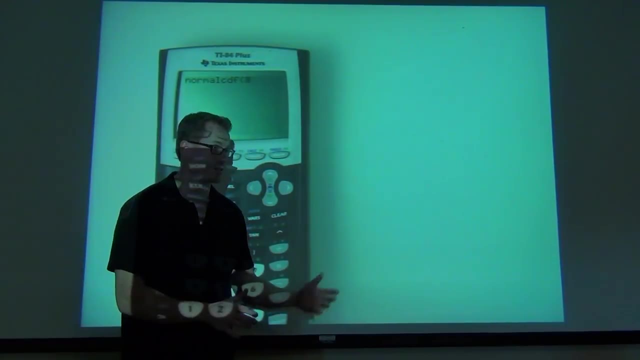 and the right ending z-score. So in our case, where are we starting actually? on our picture that you have on your paper, Yeah, Technically you can never start anywhere, right, It starts at negative infinity. It goes all the way up to 1.58.. 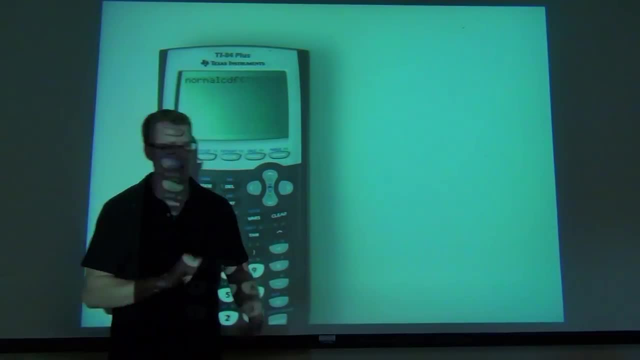 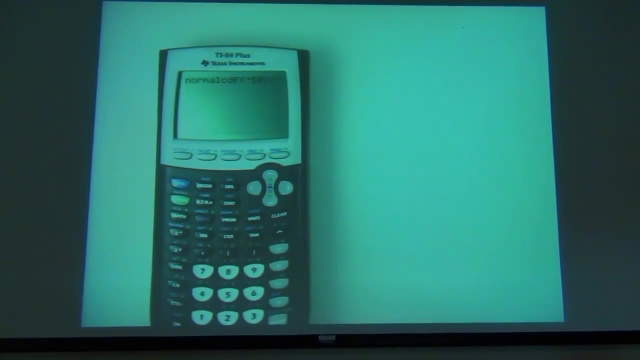 But we're going to put negative 10 because it's not going to make any difference after a certain point. So we put in negative 10.. It makes you do negative 10.. Then we put a comma And you put the ending z-score as well. 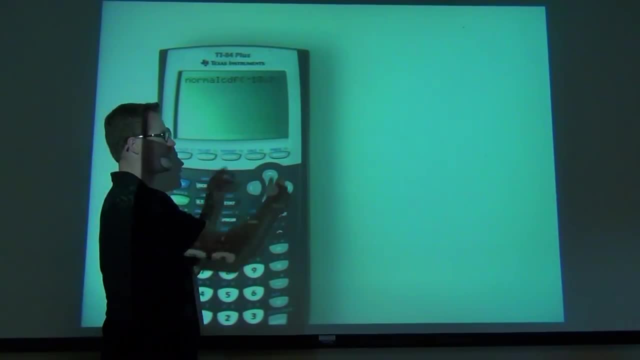 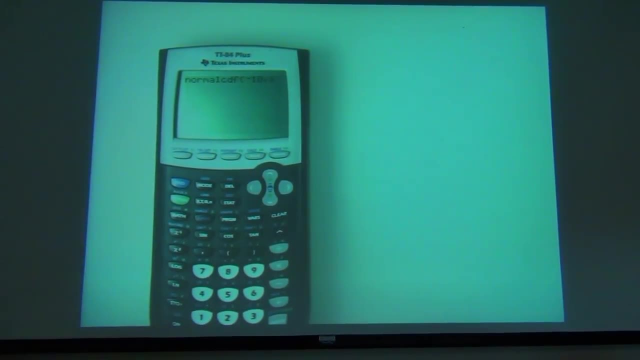 So we have our negative 10 comma. Then we're going to put our ending spot. Remember our curve was negative 10 all the way up to 1.58.. So we're going to put that 1.58 in there. 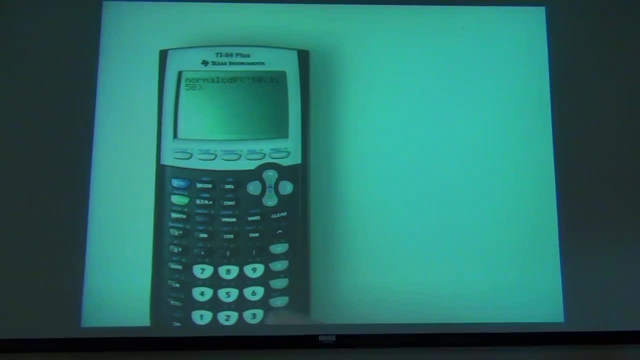 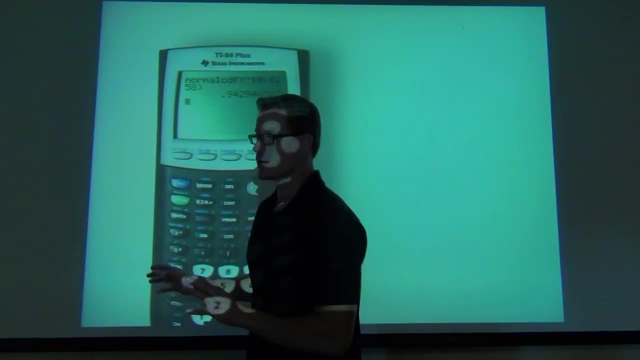 Close it with parentheses if you'd like. Press Enter And you get exactly what your table gave you to four decimal places. Now, after that, you're a little bit more exact, right? Because you get yourself a calculator that knows how to do this table. 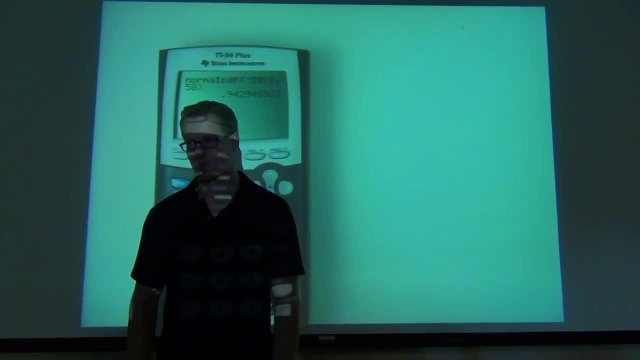 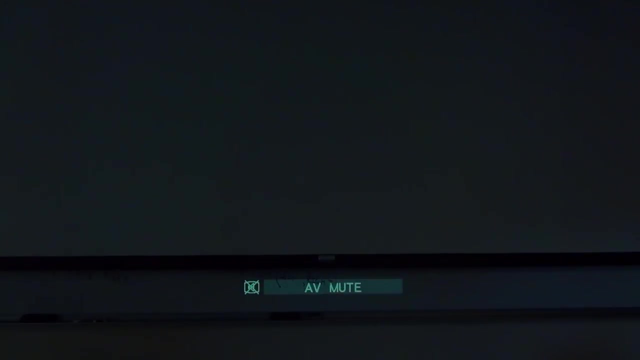 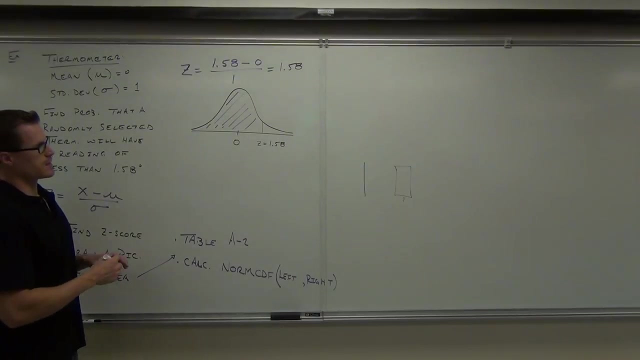 precisely to as many decimal places as it shows on your calculator screen, which is kind of cool, But in each case you get the same number. How many people feel okay with using the table and the calculator? Good, All right. So what we've done is we've figured out that this area, right here, 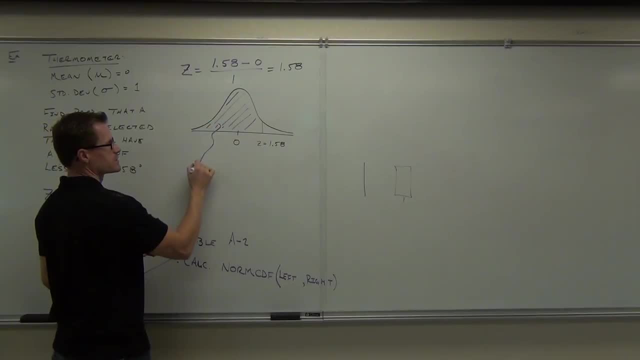 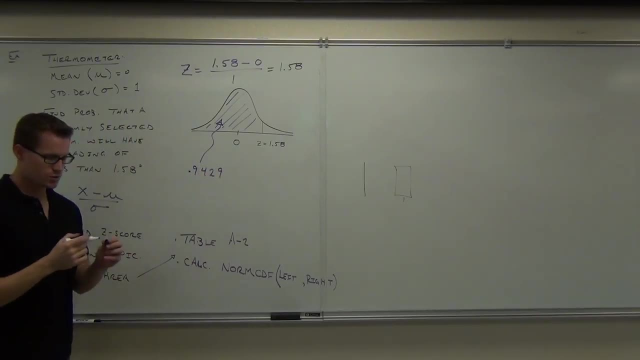 the area to the left of our z-score. Can you read that to me again? What was it? 0.9429.. 0.9429.. Right there, that thing stands for a proportion of the area that's underneath our curve. 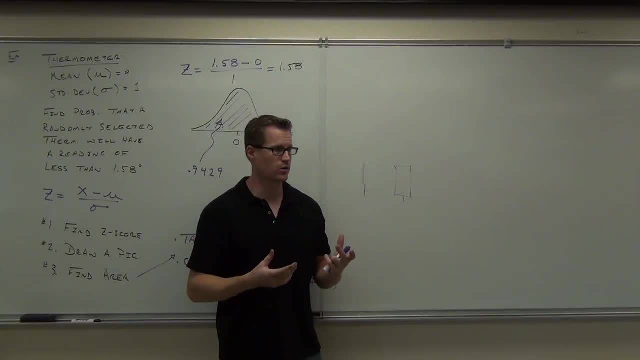 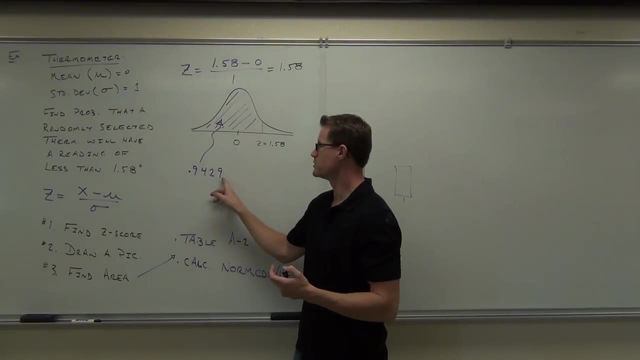 Now can you tell me how much area in total is under our curve? 1.. 1 total. We just took 0.9429 as a proportion of our area. What this means is, since the area is equal to 1 and a probability has to all equal to 1,, 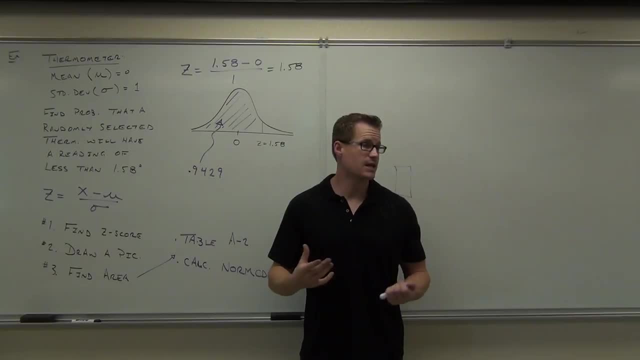 that thing is also a probability. So not only does that stand for an area, that stands for the probability. So here's what this says: The probability of randomly selecting a thermometer that has a reading of less than 1.58 is 0.9429.. 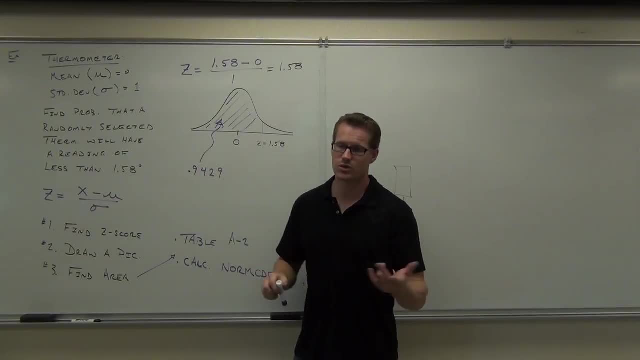 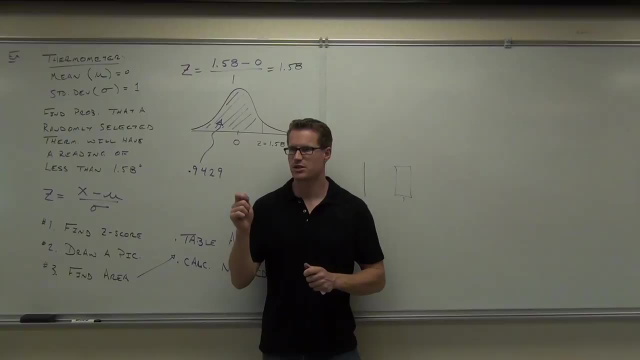 0.9429, or 94.29%. So in other words, here's what the company just figured out. They said: if I go randomly select one of my thermometers, there's a 94% chance- 94.3,. 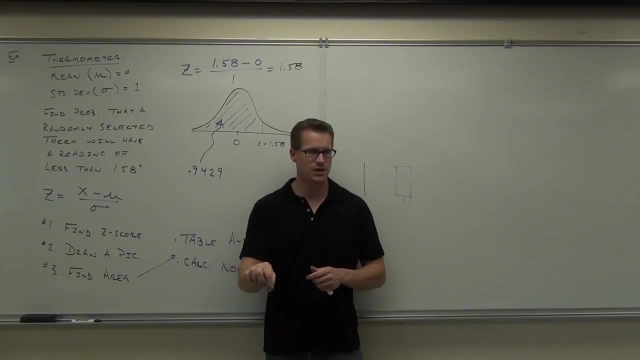 94.3% chance that if I stick it in ice water it's going to have a reading of less than 1.58.. I don't understand the interpretation. See, now we're in the business of interpreting, interpreting, interpreting. 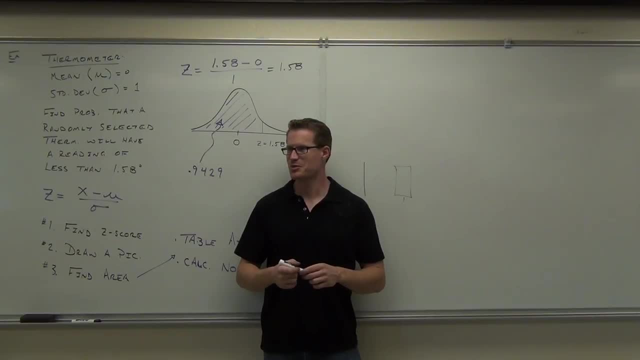 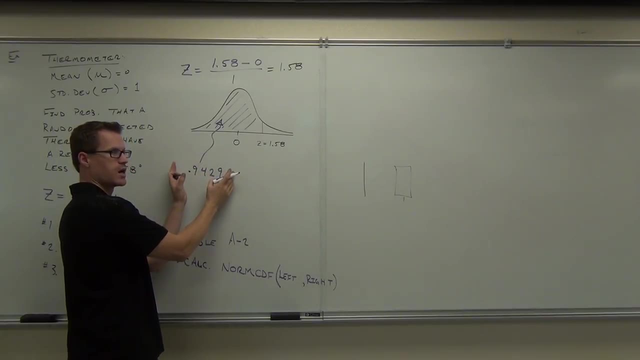 It's not even a word. Interpreting, Interpreting these things as well, We're going to have to know what they mean. So we'd say all right. the probability of the area is 0.9429.. Therefore, because the area in total equals 1,, 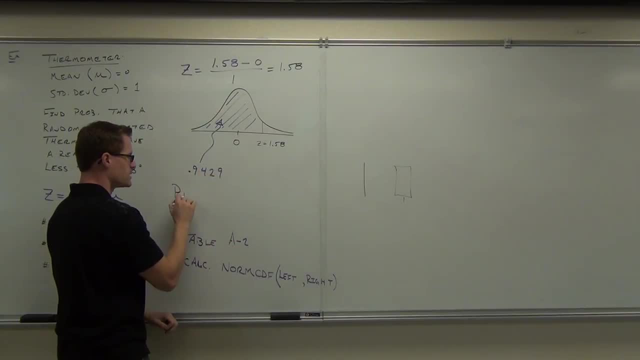 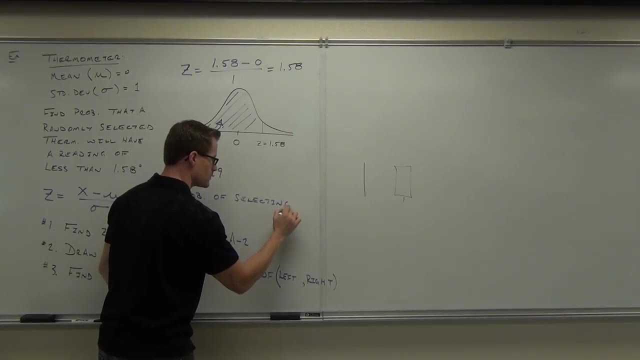 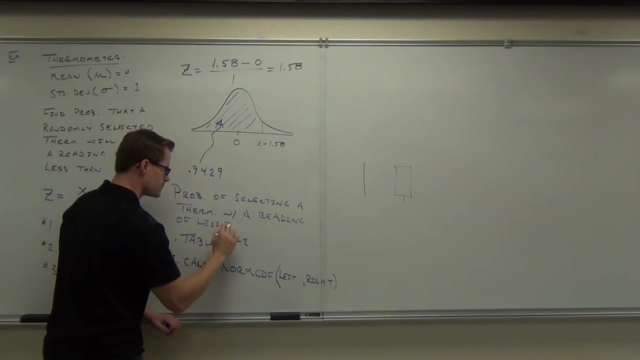 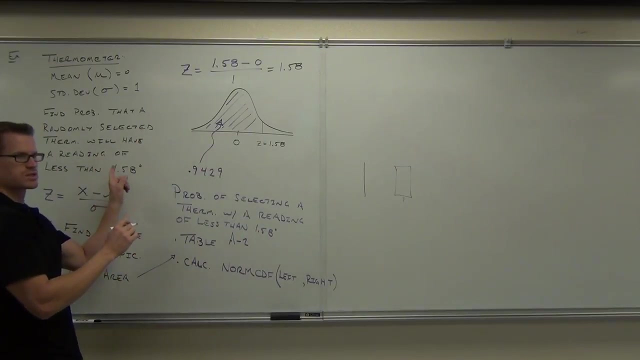 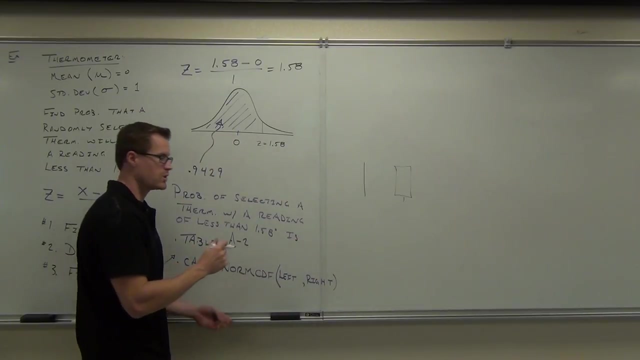 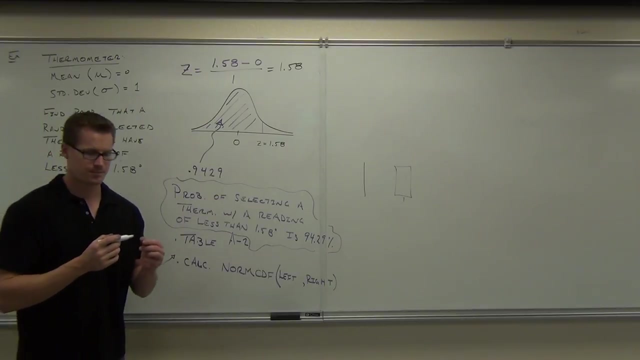 I know the probability of selecting a thermometer with a reading other than 1.58 degrees. Notice how I'm going back to my original statement here. You can either put 0.9429, or you can translate that into a percentage. That's what we just figured out. 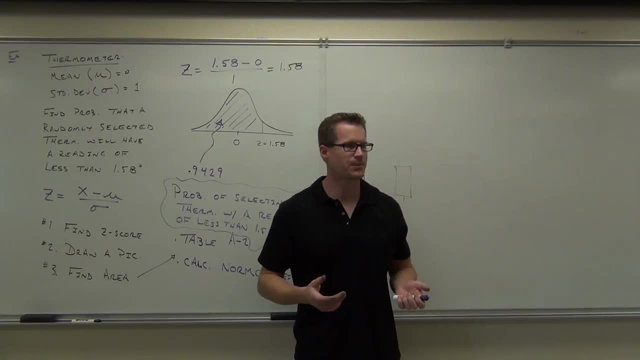 By using this, we can now calculate probabilities of things that really are quite interesting If you think about that. I mean, that's actually a lot of math going on, really, when you think about it. How many possible values are less than 1.58?? 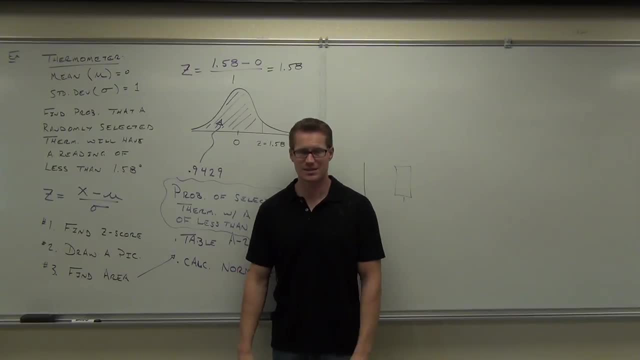 Infinite, Yet we're able to calculate the probability. you're going to select a value that is less than a certain thing. That's kind of cool. That is normally distributed And a z-score. we can translate those things. Use your table or your calculator to calculate it. 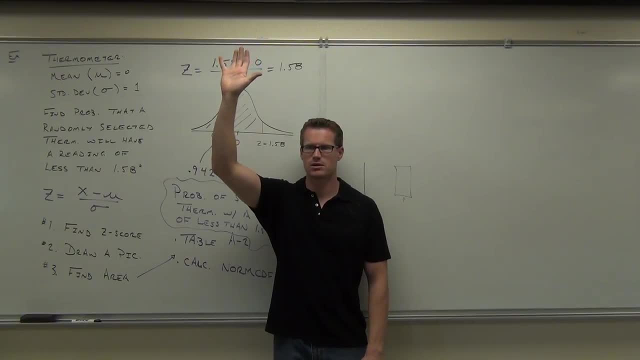 How can we be able to follow that? We'll take a few more examples. I have a question on it. Does that mean that the probability that if you select a random thermometer, that the reading is going to be off by less than 1.58?? 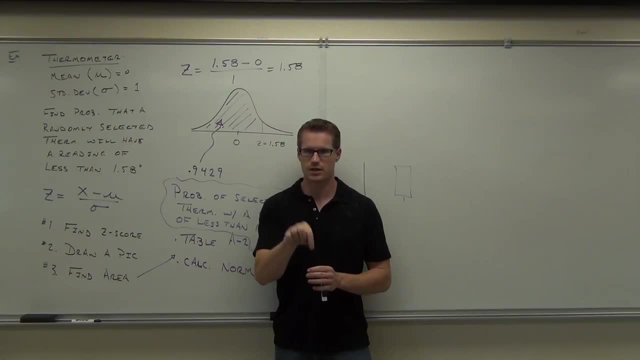 No, what that means is that your reading's here for a thermometer that you're dunking in ice water. That's what this company's doing right now. They're taking the same bucket of water, They're taking all their thermometers and they're dunking them in. 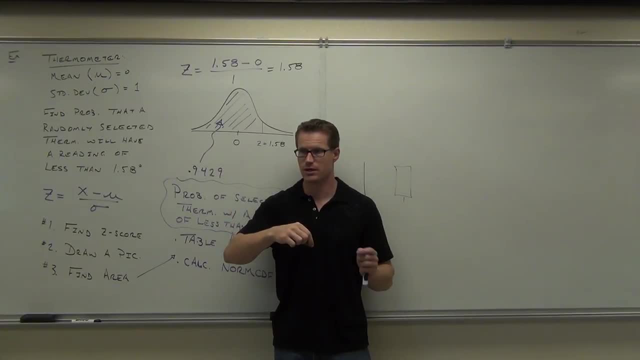 and reading it Now. it should read zero. It should read exactly zero. Are they all going to read zero? No, because everything we make we're not perfect. They're going to be off a little bit, So they all should read zero. 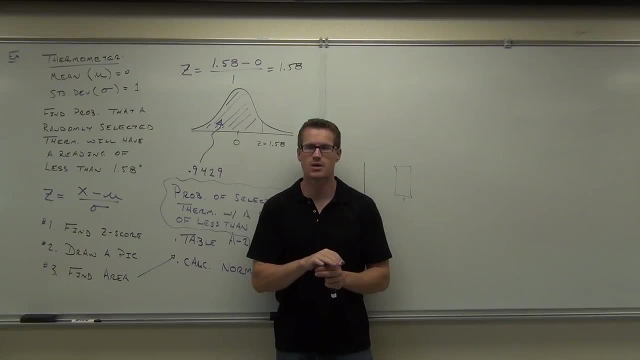 They're not all going to read zero, Some are going to read a little higher, some are going to read a little lower, But the company has realized over their vast number of years creating thermometers that the average is zero And divided by the number that you added. 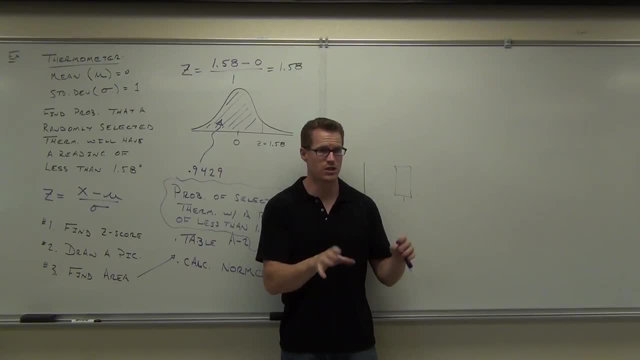 you're going to get zero And the standard deviation amongst those readings after doing the standard deviation that you know how to do. right, We've done standard deviation. here was one. Now what they're asking you is this: What's the probability that I'm going to dunk? 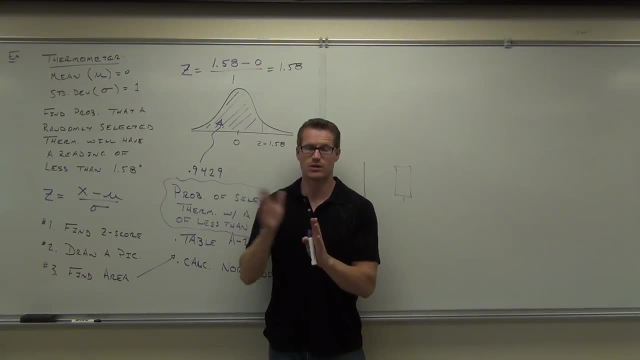 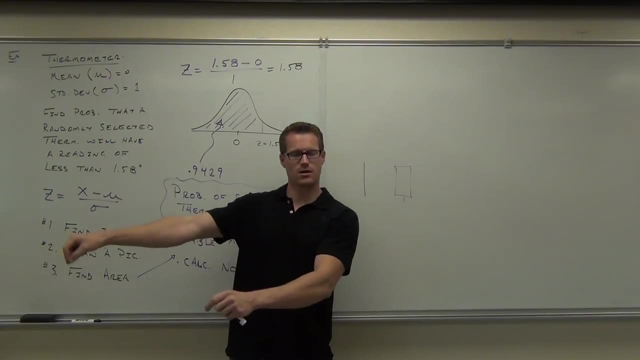 a random thermometer in that bucket of water and that reading is going to be less than 1.58? That's what they're asking you. Does that make sense? Okay, let's pick one random, Dunk it in there. 94% chance it's going to read less than 1.58.. 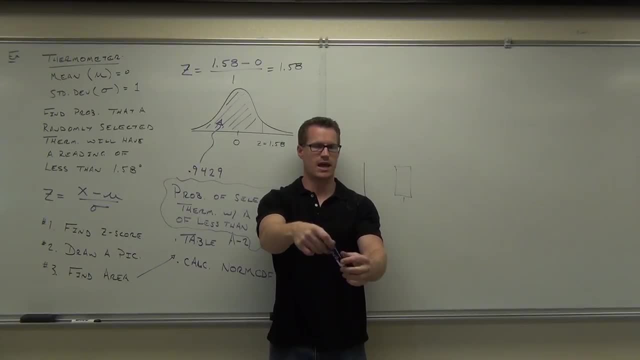 Make sense. That means that when you hand this to somebody that they're not going to get a reading 94%, certain that they're not going to get a reading more than 1.58.. That they're not going to overestimate your temperature. 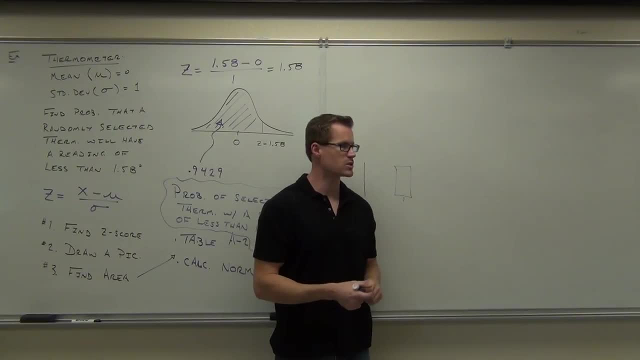 So that might be useful piece of information if you're dealing with certain situations. Does that clear things up for you, You sure? Well, I'm thinking also. I mean, if you're dealing with something that's zero, but then we would. 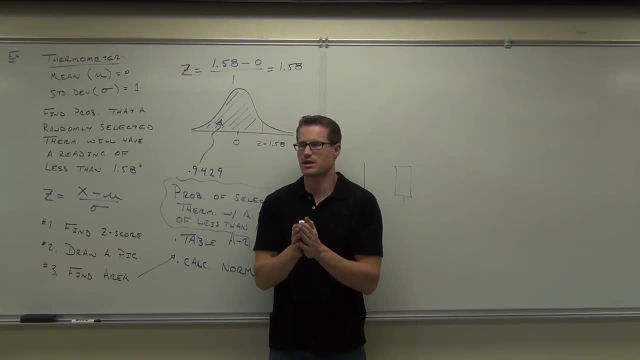 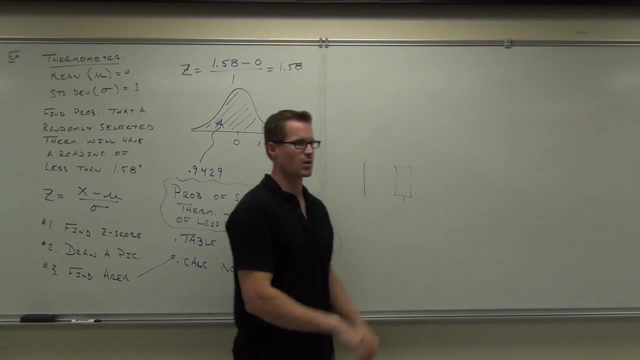 The z-score makes everything zero. That's what's so cool about the z-score, right? Because you can use a table for every situation In our case. yes, It was kind of trivial to do the z-score. I just wanted to make it easy so you could see. 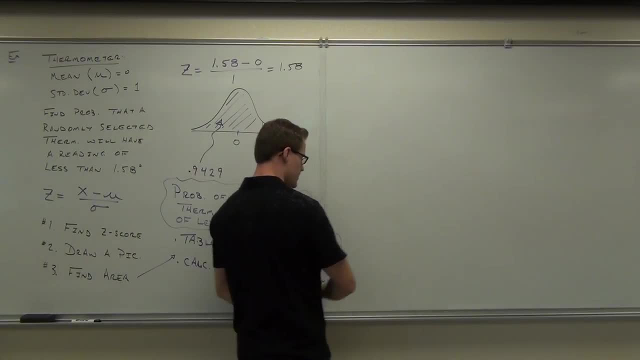 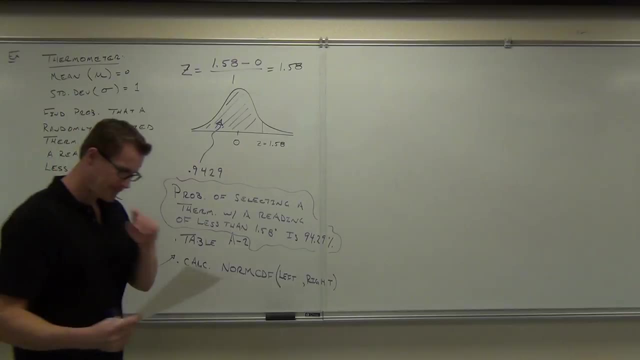 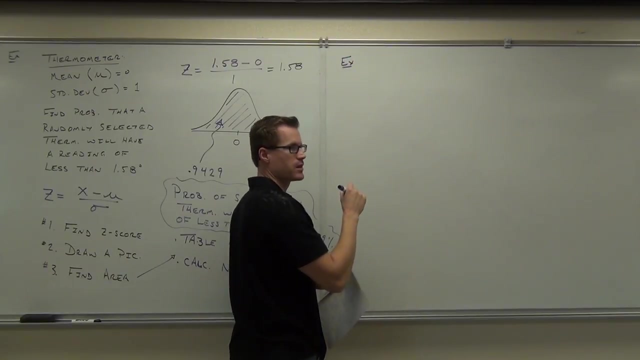 a couple things about it. Let's try a few more examples. Specifically, we'll try two of them and our day-to-day Okay same question: Find the probability, with the same information, that a thermometer is going to have a reading less than. 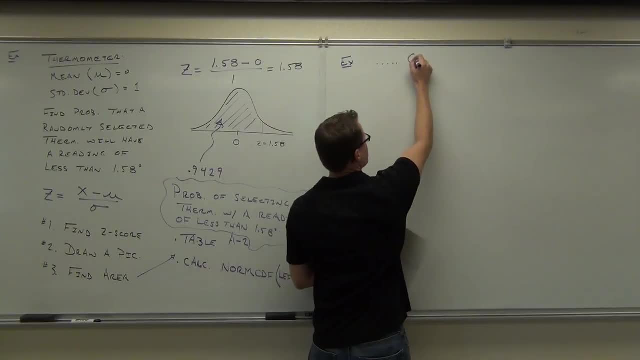 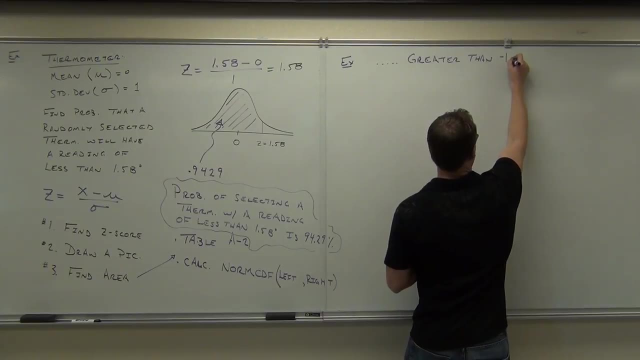 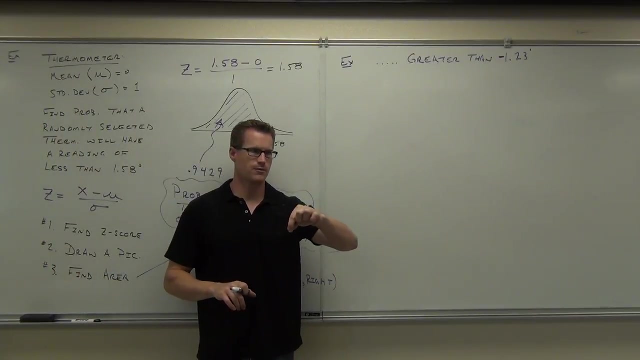 Oh yeah, let's do greater than Let's try that one. Greater than negative 1.23 degrees. Greater than negative 1.23 degrees. Notice that when you put a reading that you dumped a thermometer in a bucket of water. 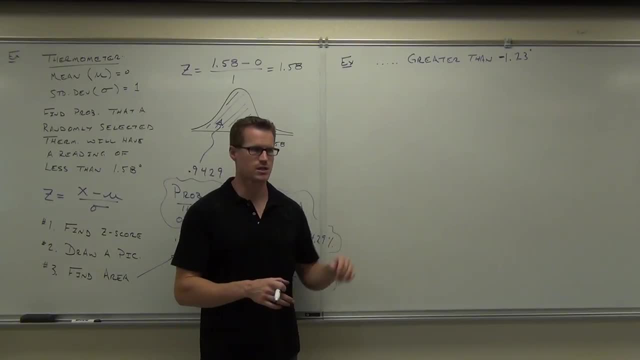 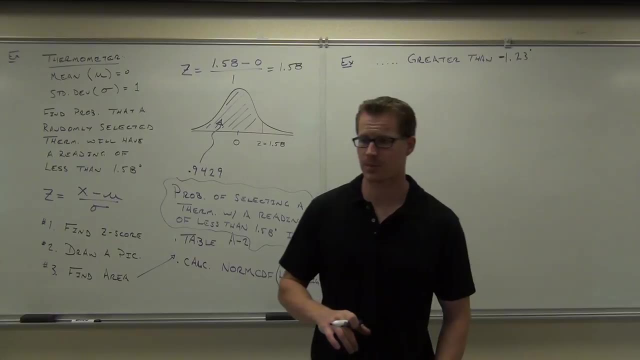 you know, below freezing, below zero would be negative. so that's the same. Let's go through the whole process. alright, What's the first thing we should do? if I give you this type of problem, What are you doing? Great z-score. 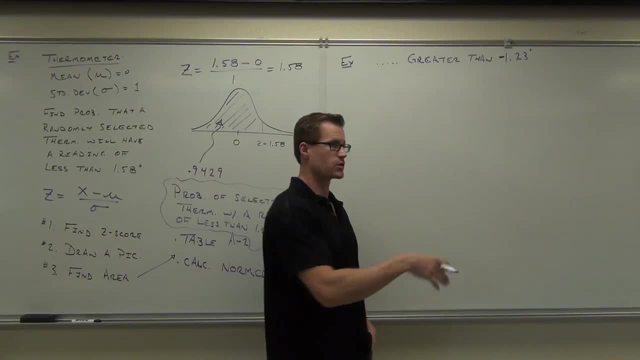 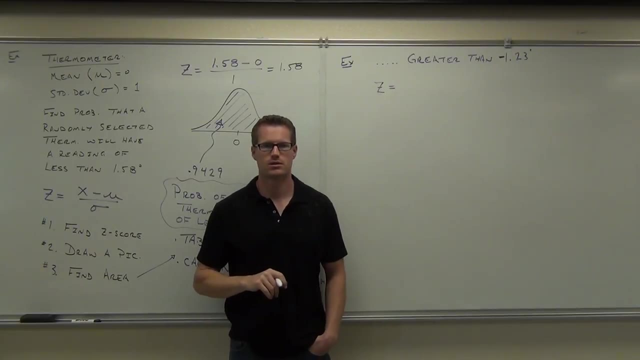 Because that's going to translate a normal distribution into awhat's it called Very good, so let's do a z-score. Can you tell me what is my x in this situation? Wait, somebody said, is it 1.28? 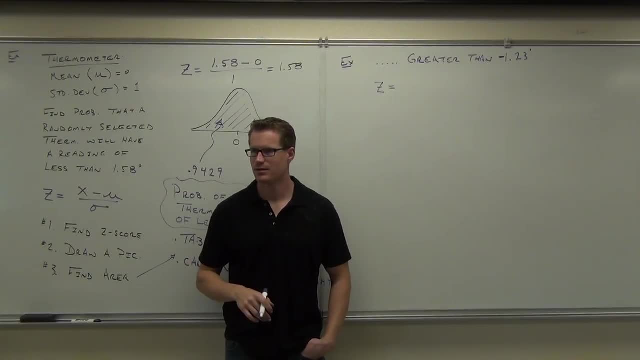 or negative 1.28? Does it matter Absolutely, Because a negative will be to the left of zero. a positive will be to the right of zero, right? If you screw that up, mess your sign up, you're going to have a completely different probability. 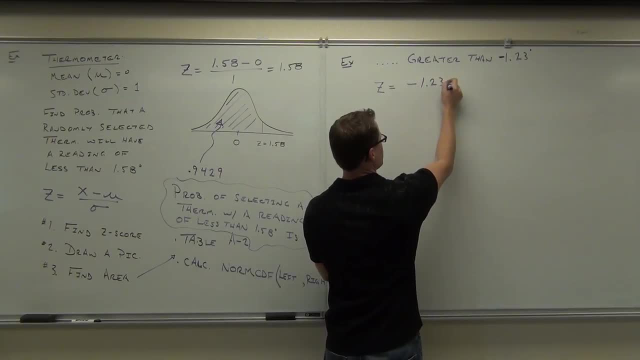 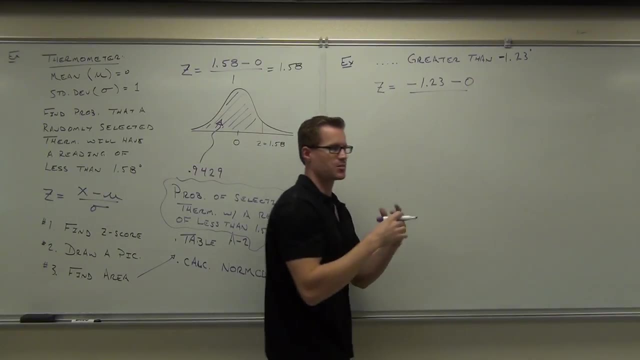 that will be off significantly. So yeah, this is negative 1.23.. We would subtract the mean. How much is the mean here? ladies and gentlemen, That's kind of nice. We're dealing with this nice and easy example that has a mean of zero and a standard deviation of one. 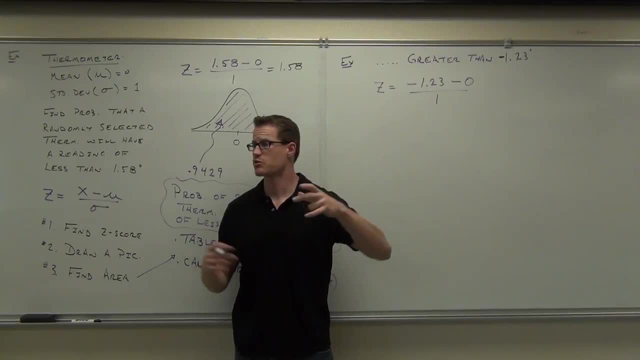 I'm just going through this so that when we get to the next section, you're comfortable with doing this manipulation. Yeah, are you with me on that? Okay, so negative 1.23 minus zero. of course, that's going to give you how much. 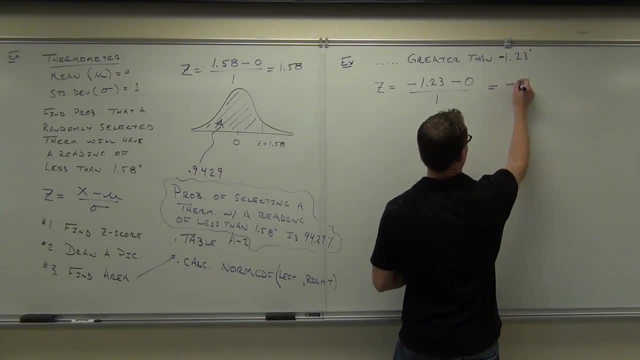 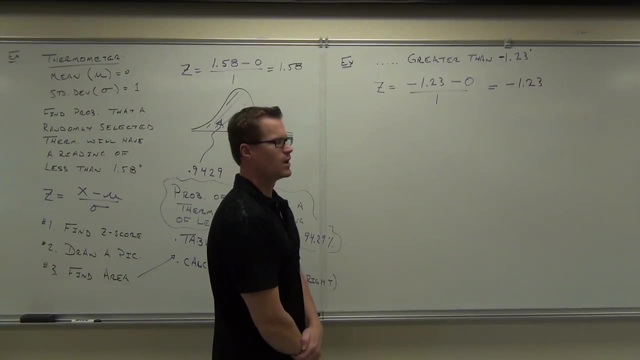 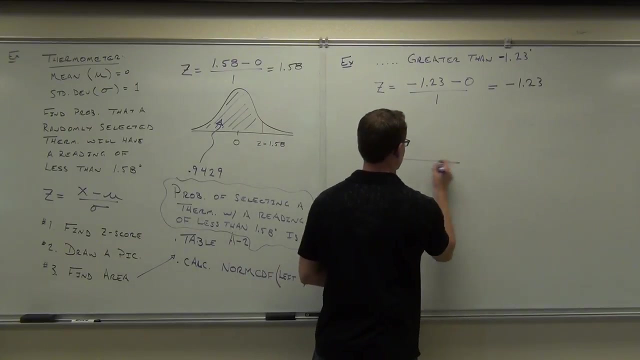 And then we divide it by one. it still doesn't change. so we get negative 1.23 as our z-score. What's the next thing you do after you calculate your z-score? What do you think? Hey, what number is in the middle of this picture? 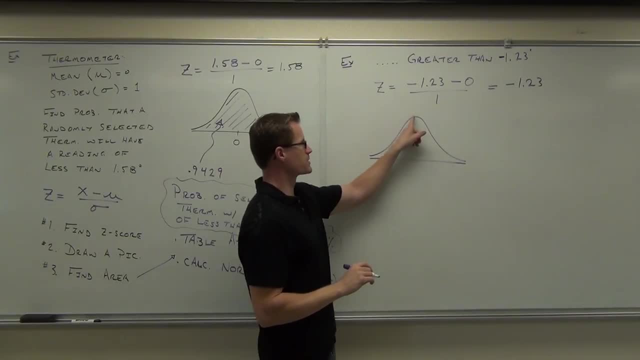 Zero. Where is our z-score going to lie? Notice how now we're talking about a z-score. We're not talking about the degree anymore. We've translated that to a z-score. Everything is translated to a z-score. That way, you can use this table. 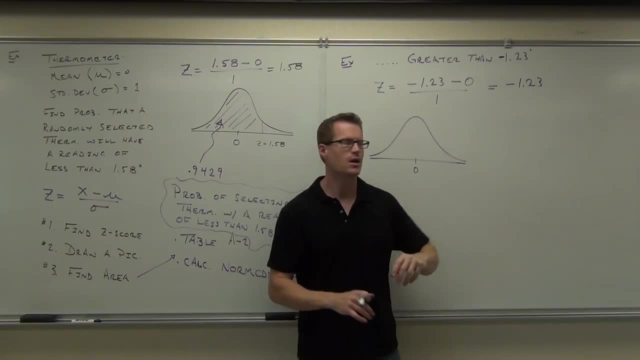 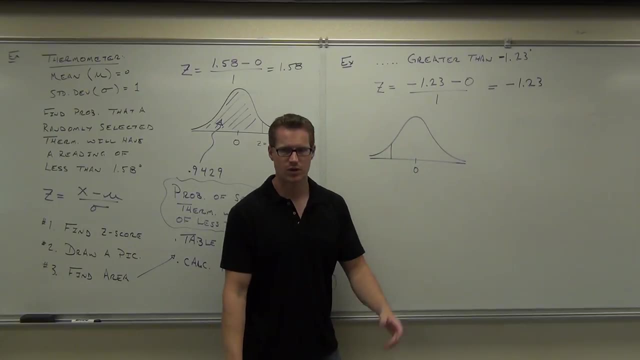 So this negative 1.23, where is it? at right or left, Left, We don't have to be exact, Just go to the left of zero, put a line somewhere and make sure you know it's a z-score of negative 1.23.. 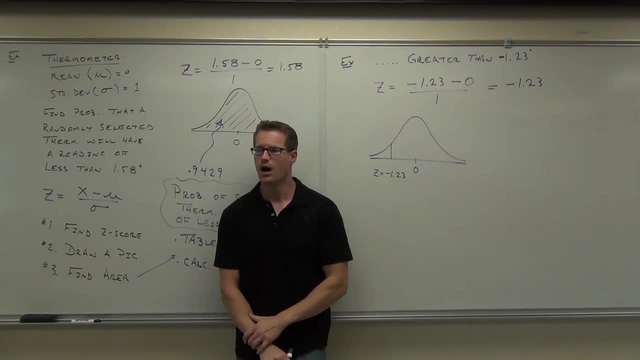 Now here's a question. This is kind of an important question: Are we going to shade to the left or to the right of that negative 1.23?? What do you think? Where's less than, Where's greater than? Where are we shading? 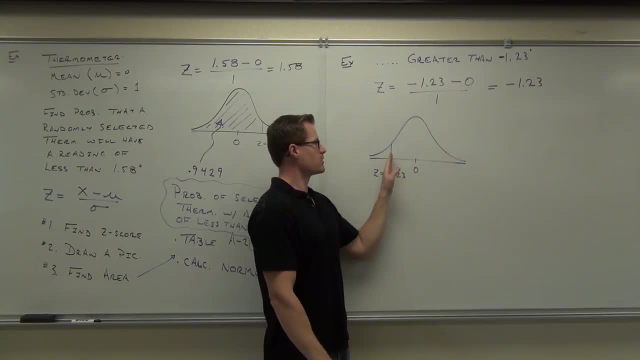 We want more than that, right. We want greater than The greater than stuff. what's bigger than negative 1?? Is negative 2 bigger than negative 1.3? That one makes sense. That's why we have to cover number lines. 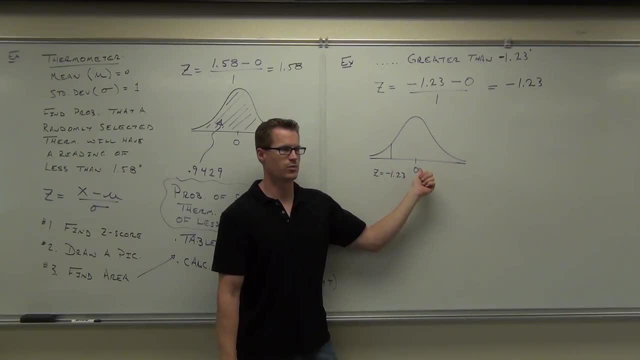 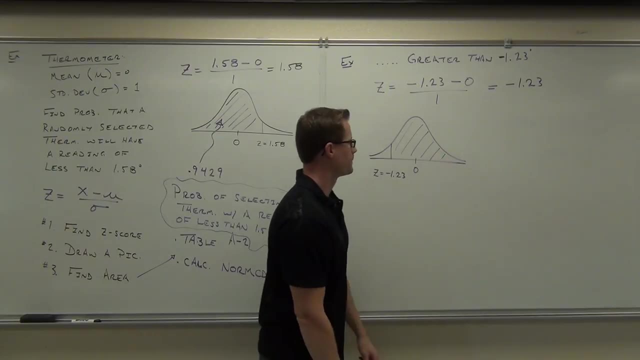 to be in here, right? So we know where greater and less than is Is zero. greater than negative, 1.23? Well, that should tell you what side you're shading right there. So we're shading this side Right there. 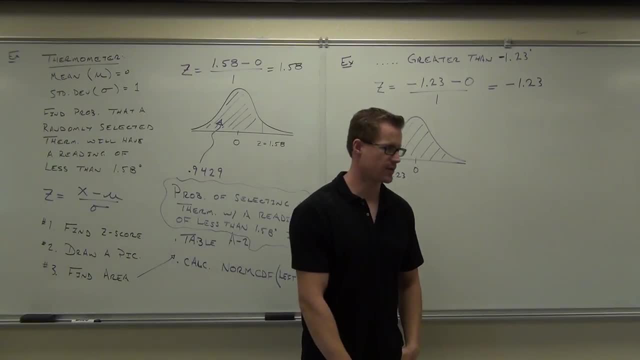 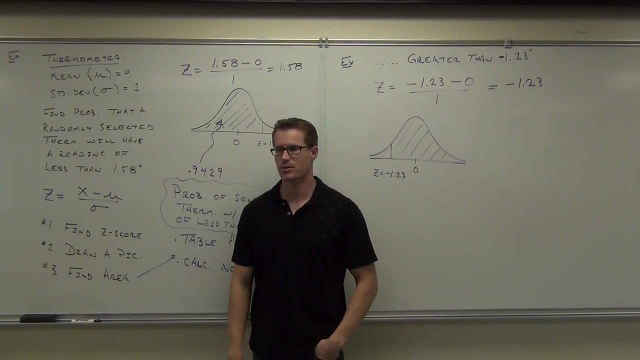 Okay, what I'd like you to do right now is practice the table stuff, and you have a calculator. Do this for me: Find your negative z-score right now on your table or your calculator. Actually, I'd like you to use the table first, if you can. 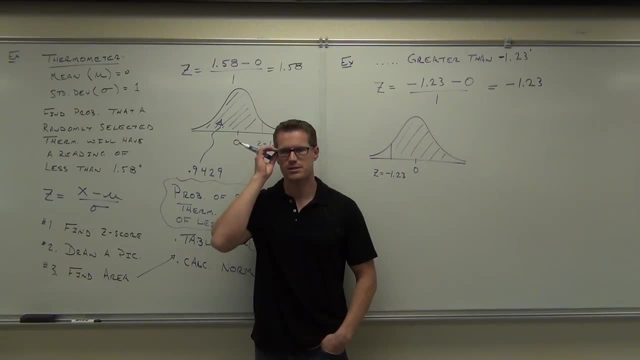 You all should have a table. Use the table. Find the z-score negative 1.23.. Look up when you found it. so I know you're all done, okay. Look up when you found the z-score of negative 1.23.. 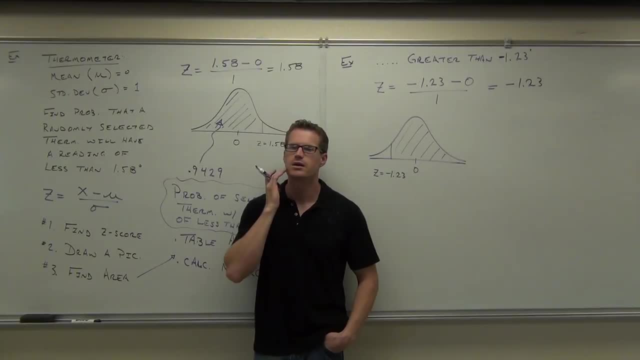 Good, good, good. Did you all get it? Here's the question: The area that you just found. please watch your paper for a while. The area that you just found. is that this area? or is that this area? What do you think? 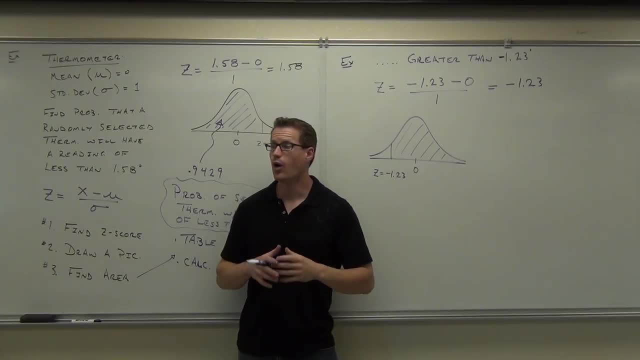 Is it the area to the right or to the left, The table? always it's not smarter than your problem is. It's not smarter than you are. It's always going to give you the area to the left, Even if you want the area to the right. 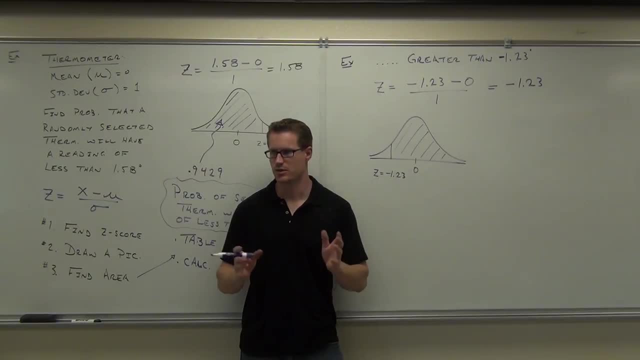 it always gives you the area to the left. Are you understanding that It doesn't change depending on the problem you're doing? That is a piece of paper. It cannot change. It's already written on. It always gives you the area to the left. 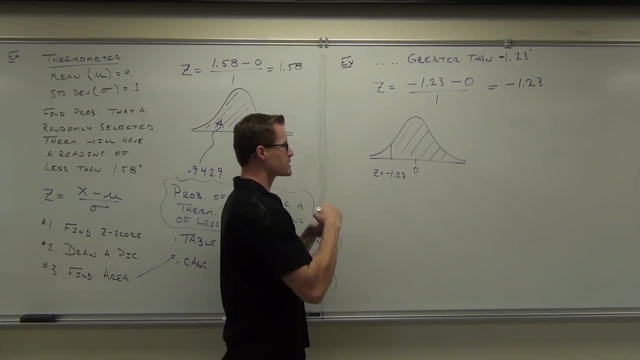 So here's what this does. This says, if I looked up negative 1.23 in my little chart there in my table A2, it's not going to give me this area. It's actually going to give me this area, which is why we draw a picture of this thing. 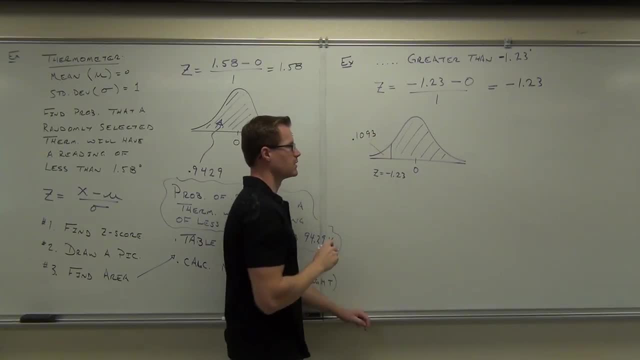 How much did it give you for this? Yeah, How many people were able to find that Good? okay, You just have to be smarter than the problem now. Now, we weren't actually looking for this area. We wanted stuff bigger than this number. 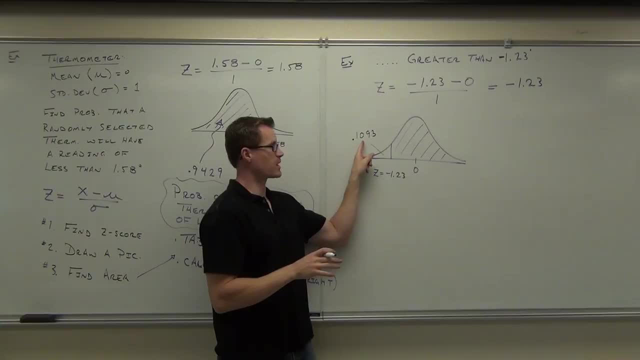 We're not looking for this. So if you put this as your answer, is that your answer? No, that would be wrong. That would be finding the area or the probability of selecting a thermometer that's less than negative 1.23.. 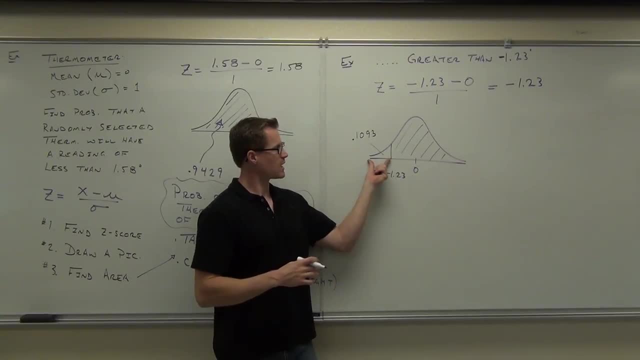 So the question is: if I know this area is 0.1093, how can I find this area? Explain, subtract that from 1.. Why? That's the whole reason why we set that equal to 1. So that we knew if this whole area is equal to 1,. 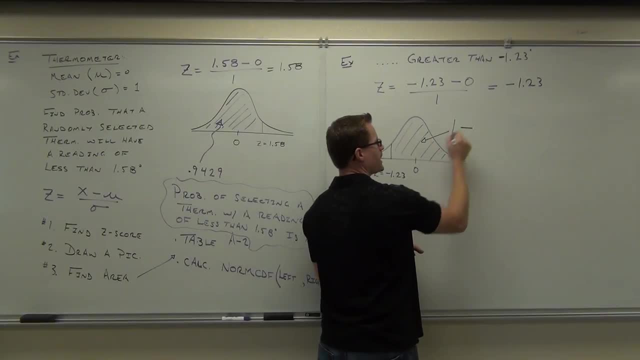 then this area, the area that we want, is 1 minus. They're complementary areas. They have to add up to 1.. If this is a little bit of 1, this is the rest of it. Or in other words, 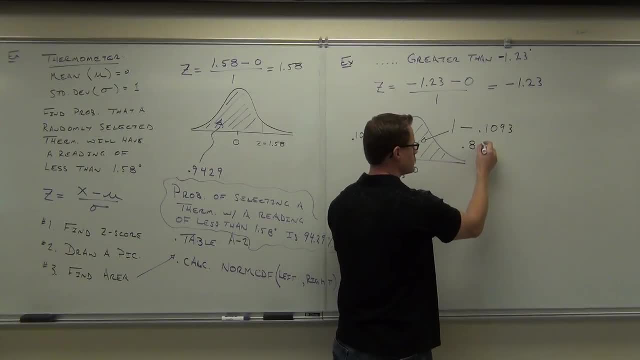 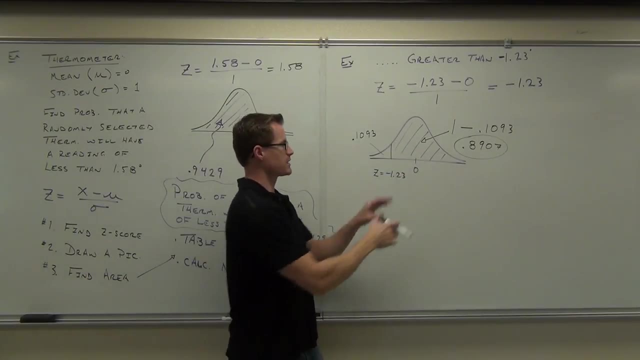 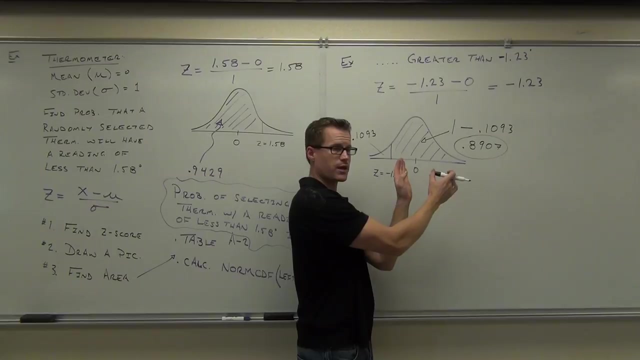 you're going to get 0.8907.. That's your area. That's your probability. Notice how this is the area I wanted. It wasn't to the left. Your table will only give you the area to the left. That's all it will do. 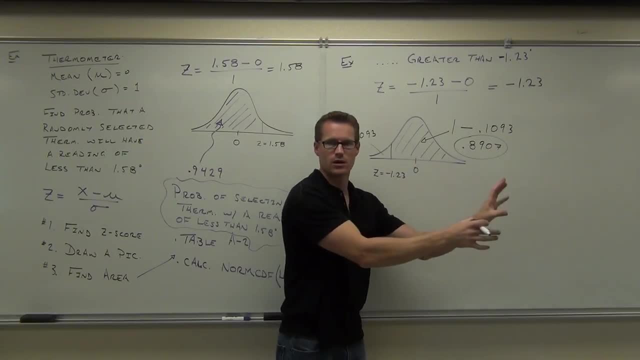 If you're not looking for the area to the left, you have to subtract it from 1.. Subtract it from 1.. That's going to give you the area to the right. Your table will never give you the area to the right. 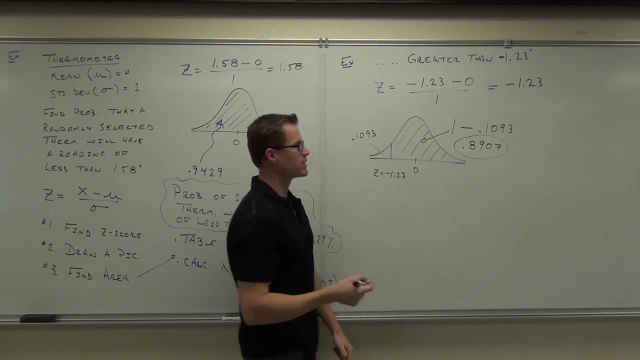 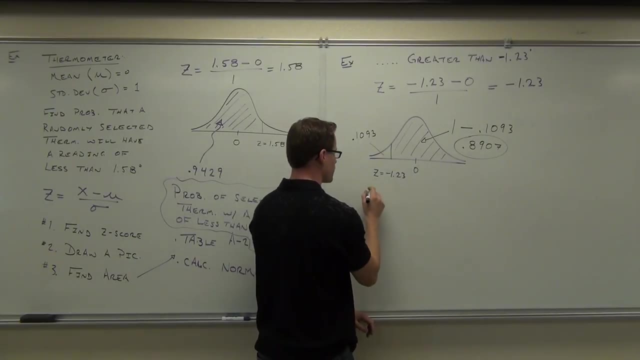 Good. The way you answer this question is: there's an 89.07% chance that you're going to randomly select a thermometer and it will have a reading greater than negative 1.23.. So with these you always want us to answer, 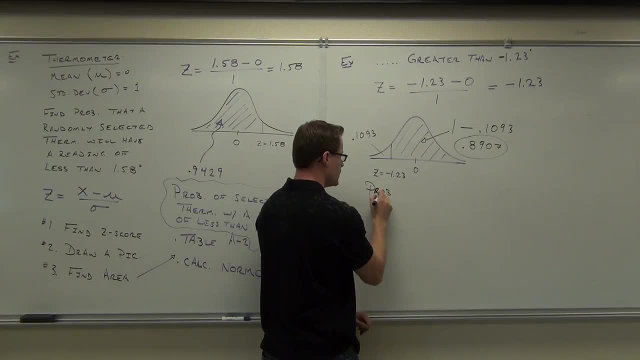 in a complete sentence. I would, yeah, Get in the habit of that, because in chapter 7, 8, you're going to be interpreting, I'm going to invent it. Just put it in the dictionary, That way I'm not wrong. 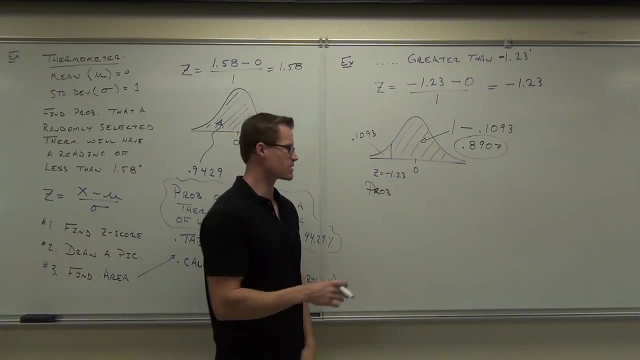 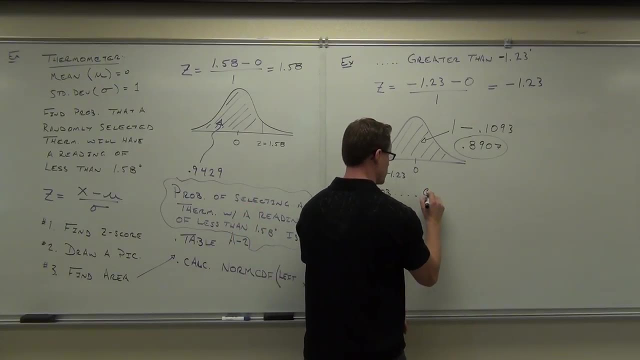 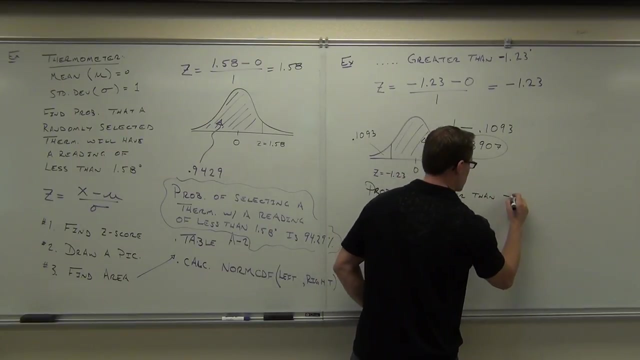 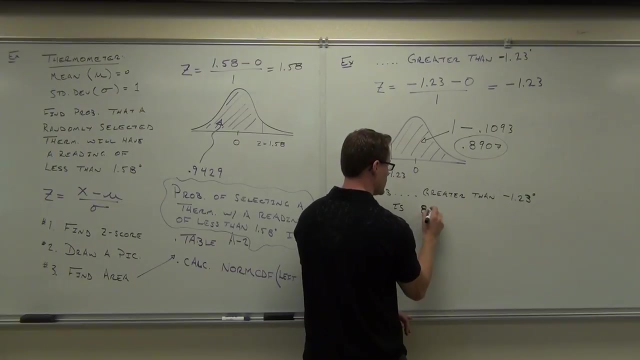 Interpreting these things and you are going to have to write out sentences, So I'm going to be lazy. I'm going to say: probability of selecting a thermometer with a reading greater than negative 1.23 degrees is 89.07%. 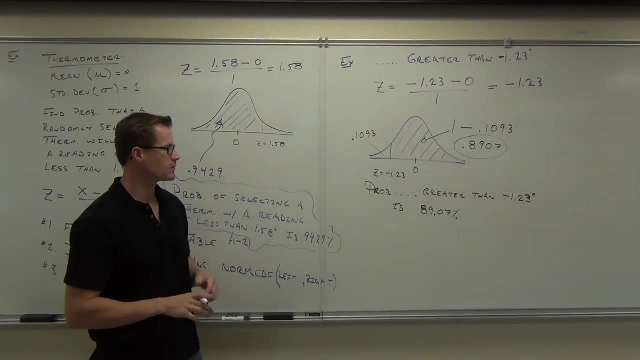 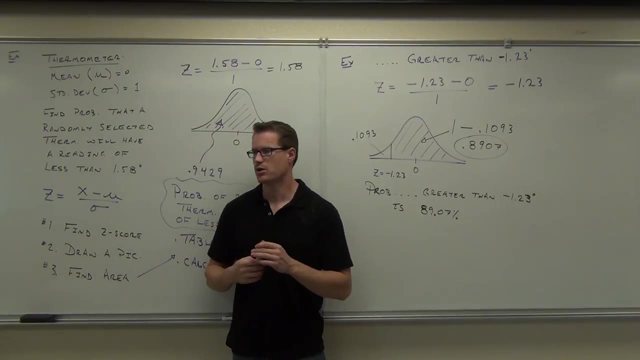 89.07% Now. calculator people- Calculator people. If you want to not use a table, you don't have to use a table. You've got to calculate it, But you need to know how to punch these numbers in correctly If you're going to do your area. 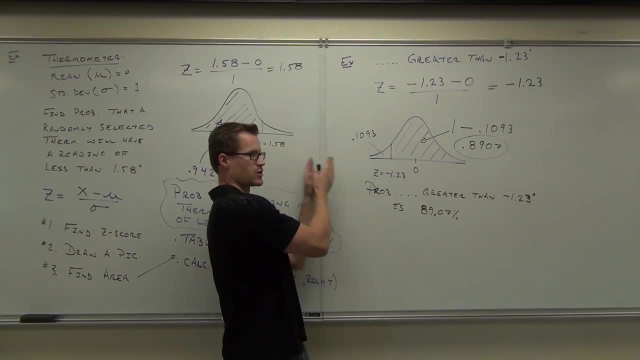 from the left to right. does this area start at negative 10?? No, this area actually starts at negative 1.23.. Do you follow So on your calculator, do this right now. if you have one, Go back to your normal CDF. 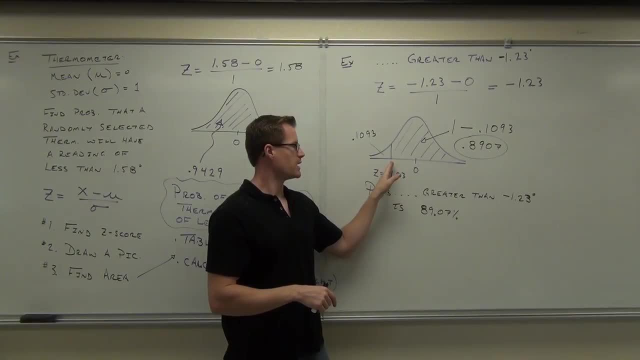 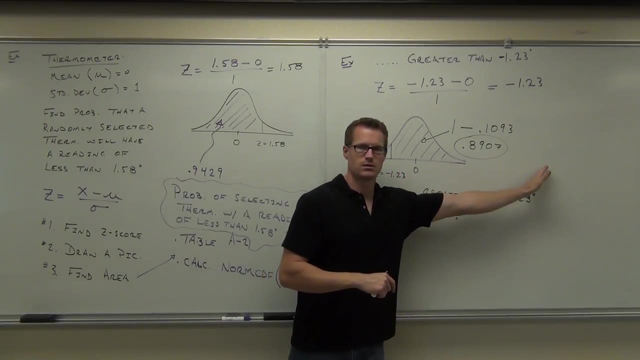 Plug in your negative 1.23.. Press your comma. Where does it end? Yeah, let's just use 10.. It doesn't really matter, right? It doesn't end, actually It doesn't end, But we're going to use 10. 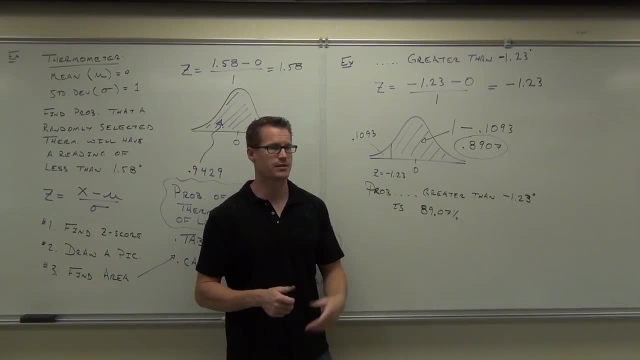 because it doesn't make a difference. after that Did it give you .8907 and some numbers after that, .89065? What .06?? Wait, how come it's .065 on yours and it's .07 here? That table rounded it. 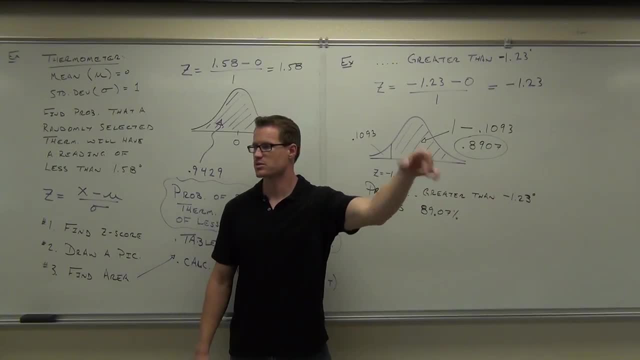 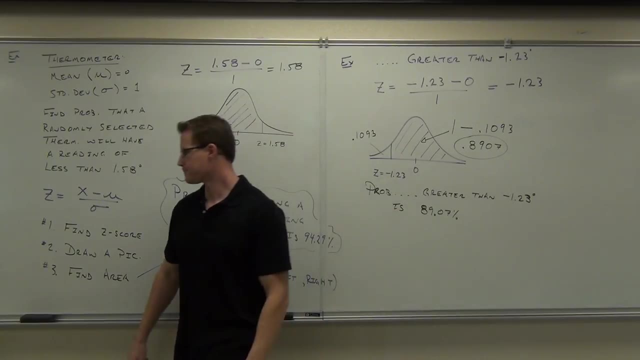 Yeah, for sure. So you got .065 and so so, so. So it's a little bit more accurate than your table's going to be, And that's the case because it's always rounded. Let's try one more. We'll just talk about it. 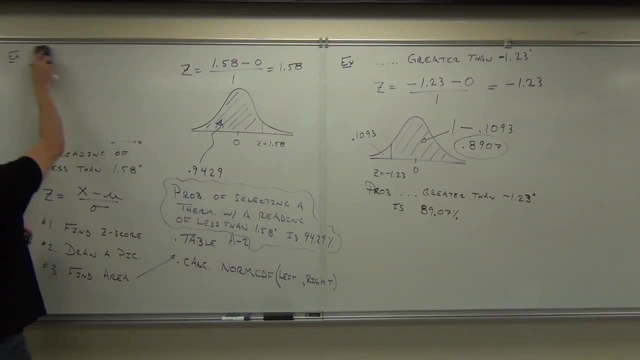 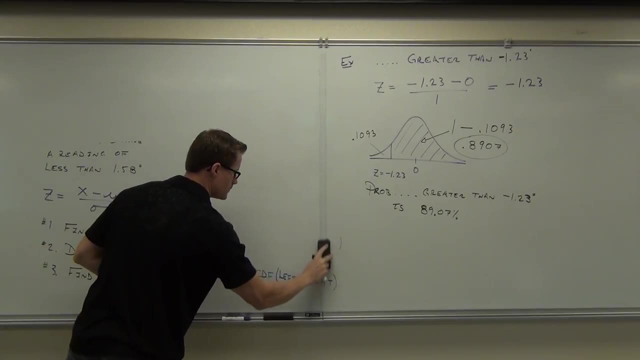 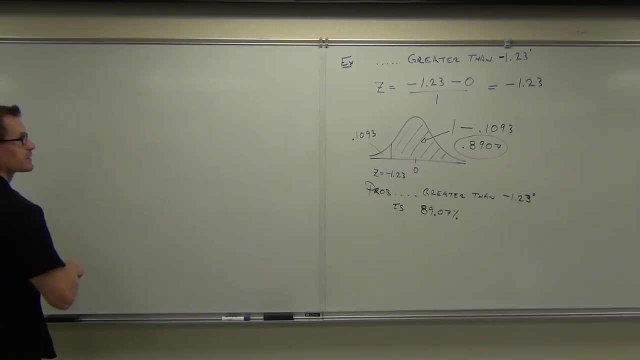 We're not going to actually do it. I don't think we'll have time, But at least we can talk about it. Okay, So same question, Same information: Probability of selecting a thermometer between negative 2 degrees and 1.50 degrees. 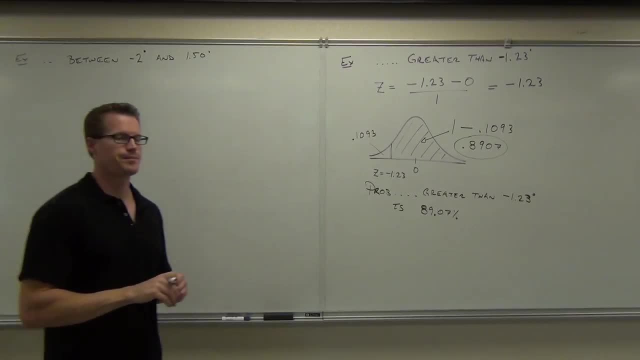 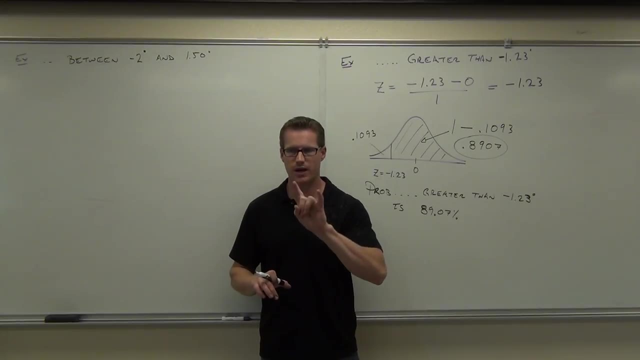 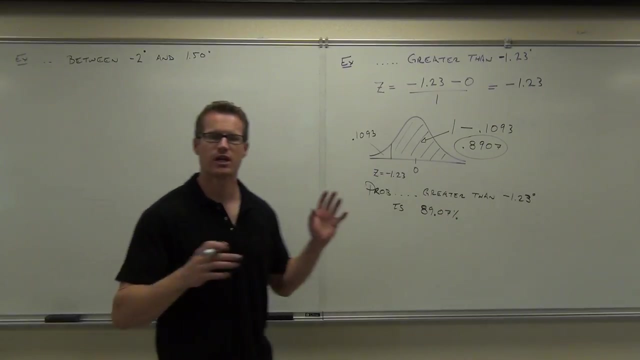 Negative 2 degrees and 1.50 degrees. Hey, we have two values. now We have two x's, not just one. What are you going to do? first, Z-score, Z-score, of course. Yeah, that's how we change from a normal to a standard normal. 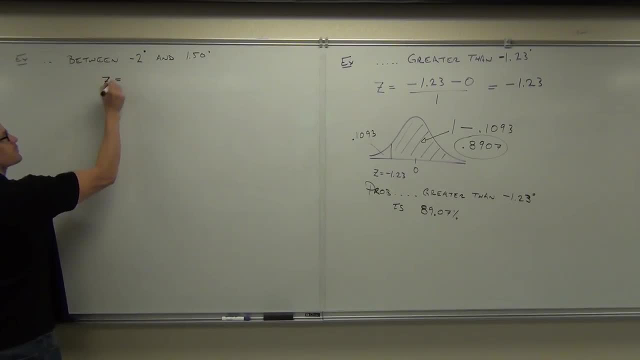 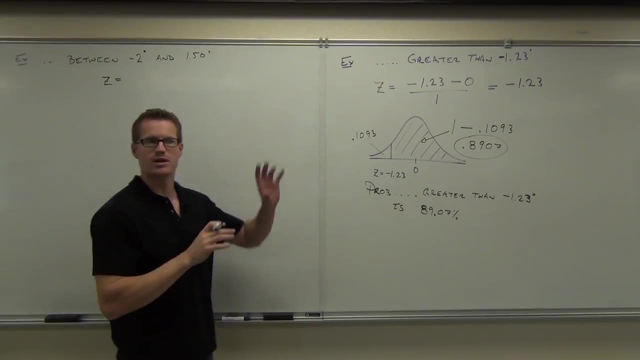 So we're going to do a z-score for negative 2.. You know what, If you do a z-score for negative 2, do you know how much you're going to get out of that? I'm going to give you a visual example. 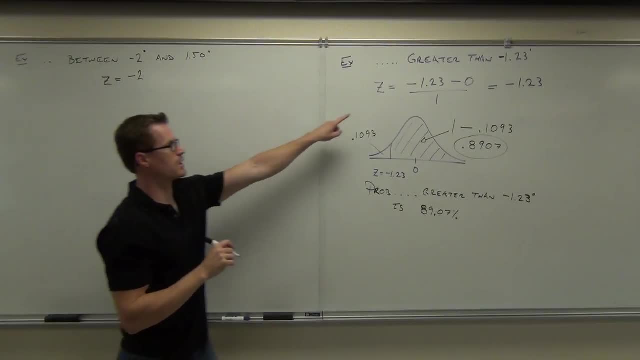 because our mean is 0 and our derivation is 0. You're going to get negative 2.. Do this work again and you're going to get negative 2.. You with me? What are you going to get for 1.5?? 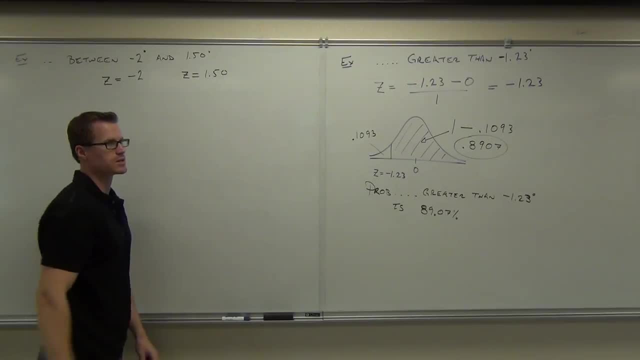 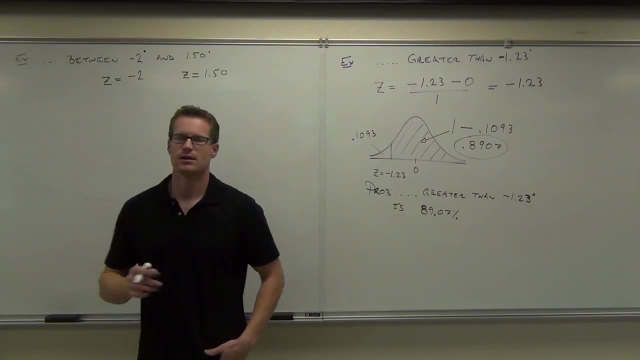 Eh, you're 1.5.. Again, this is a very special case. It doesn't happen all the time like that. okay, After you find your z-score, what are you going to do next? So here's your picture. 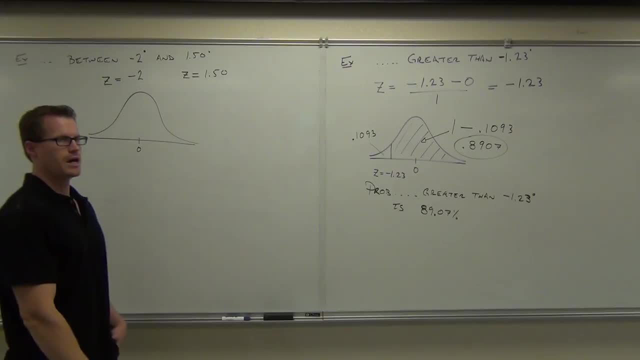 Of course negative 2 is in the middle. Now we have two z-scores to place, We've got negative 2.. Negative 2 is to the left of 0.. 1.5 is to the right of 0.. 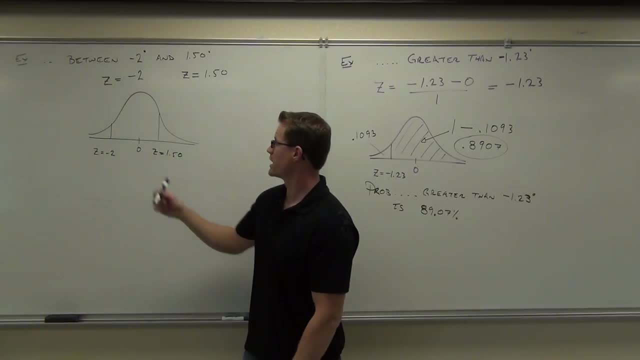 You've just got to tell me where we need to shade. Do we need to shade to the left, to the right, to the middle or all of it? We want between those two values, Between this value and this value is represented by the area. 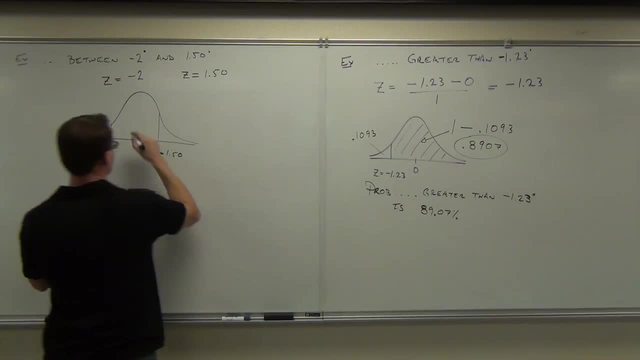 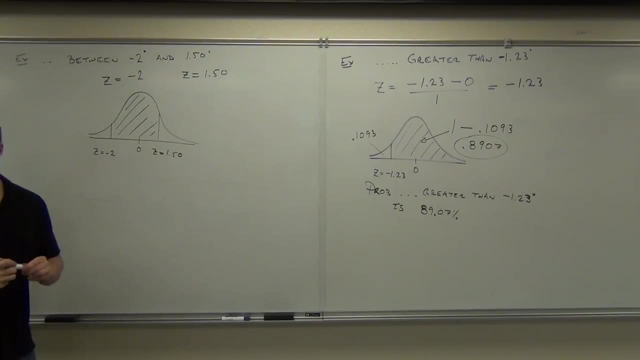 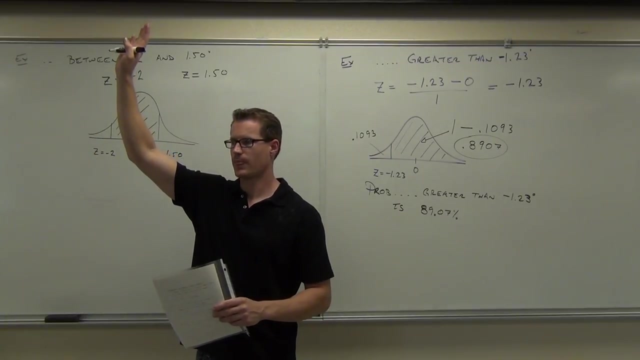 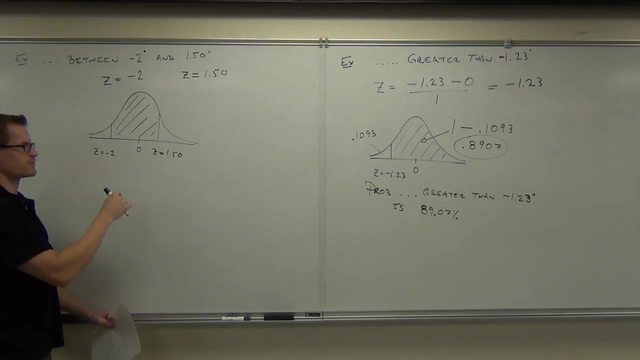 between this z-score and this z-score. So in other words, this stuff right here. Hey, how many people feel okay looking up numbers in the table? How many people feel okay doing this on a calculator? Here's your two ways If you look up this z-score. 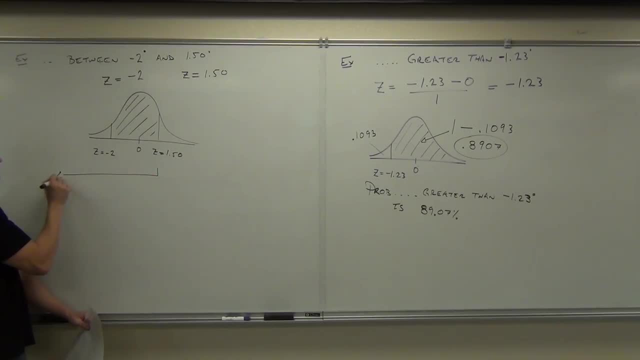 it's going to give you all of this area. Double-check this for me if you'd like, but this is going to be 0.9332.. This area is 0.9332.. Do I want all of this area? No, 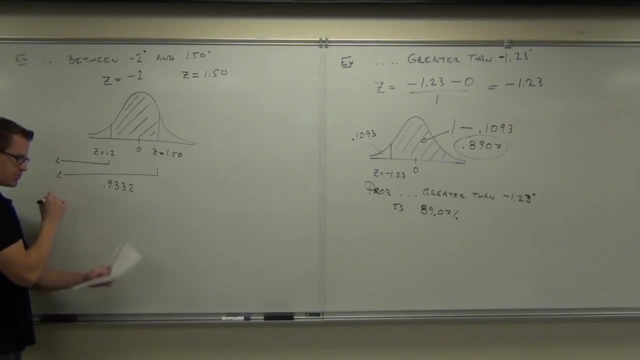 See, I don't want this area. This area is 0.0228.. Double-check that on your own if you'd like. How can I find this? If I have all of this and I don't want this subtract, then 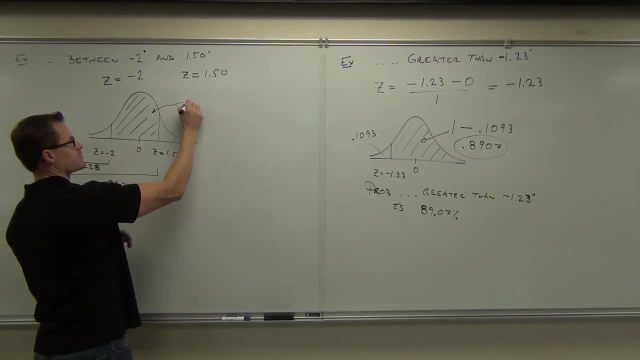 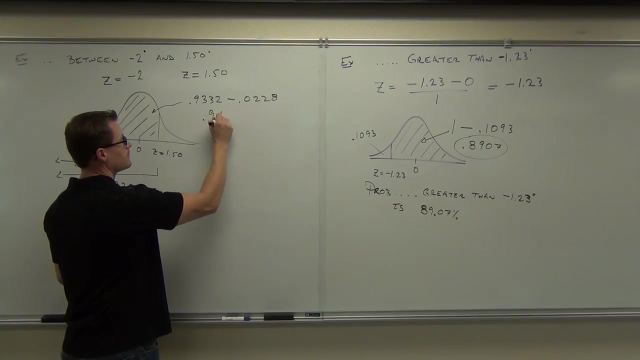 So our area, or in other words, our probability, is 0.9332 minus 0.0228.. How much is that going to give you? What is it? 11? 91104.. 91104? Yeah, That says you have a 91% chance. 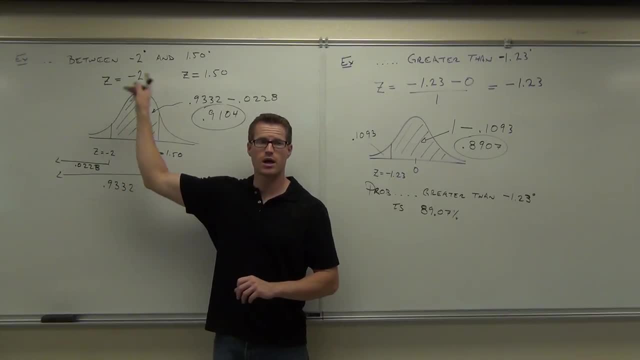 of selecting a thermometer that's between these two readings, 2 degrees and 1.5 degrees, On your calculator. it's even easier. You don't even have to look up two things. You just put normal CDF negative 2, 1.5, enter. 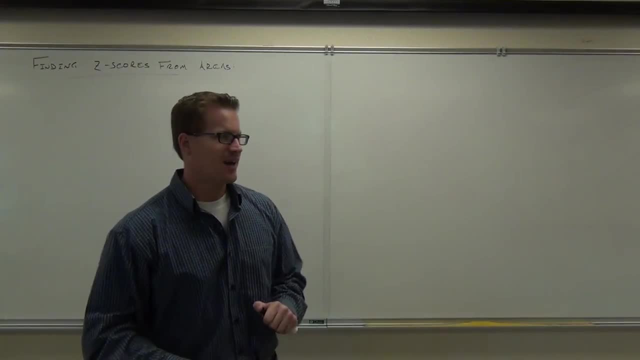 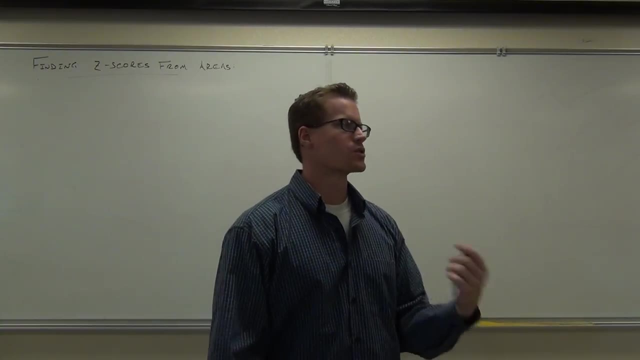 you get the same exact value. Feel pretty good about this. Okay, Let me show you some statistics to you. So we're going to do one thing today: We're going to go backwards of what we've been doing, You see, lately in this class. 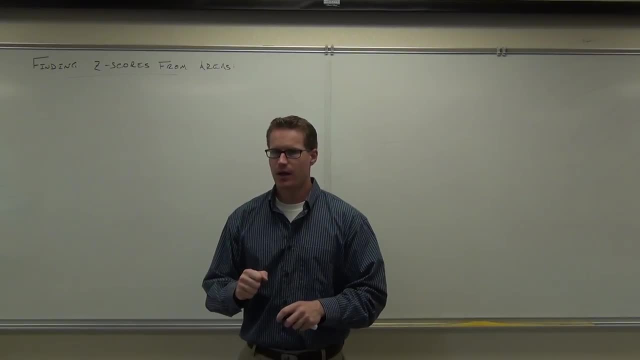 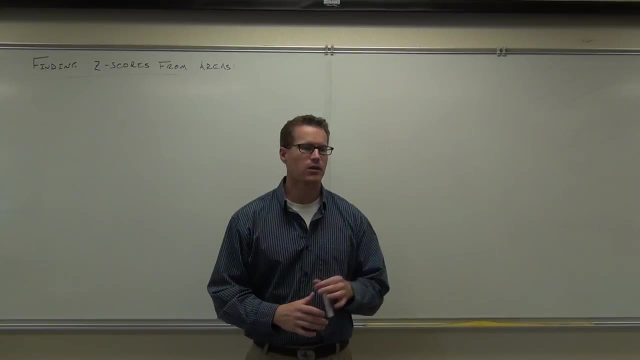 we've been looking up z-scores with your table, with your calculator, and finding out areas. You remember that from last time, right, We spent quite a bit of time doing that. There is another thing that we can do with this table and with your calculators. 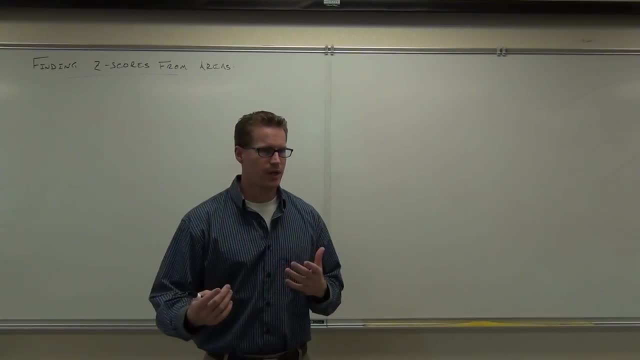 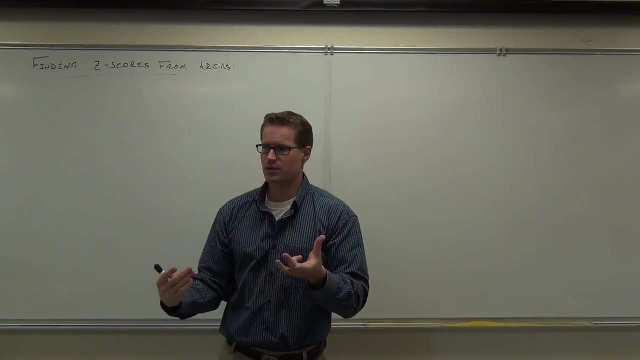 We can look up an area, or in other words a probability, and find a z-score from that. That table works both ways. So not only remember how you can find a z-score, but we can look up an area and therefore give you a z-score. 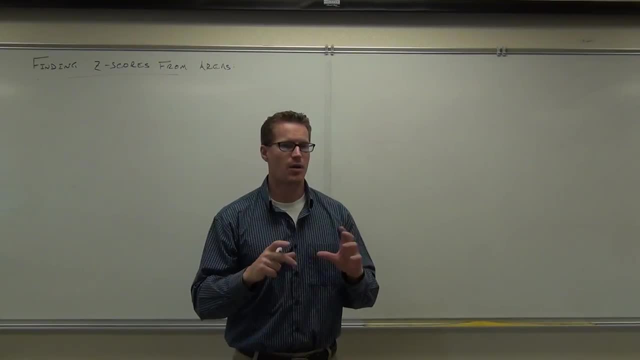 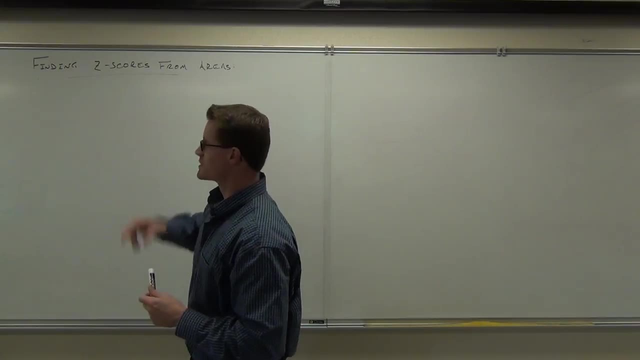 Does that make sense to you? We're going to learn how to do that today. I'll show you that sometimes we can find probabilities of having a certain value over, under, or a certain value over or between two values by doing this. So we're going to be finding z-scores from area. 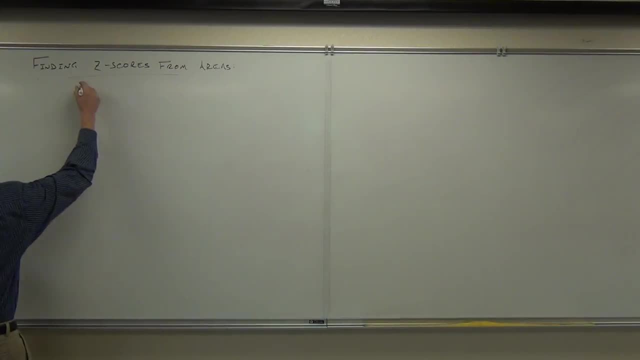 We're going to be using the area or a probability to find the z-score. We'll be working backwards. So we're going to work backwards By using an area, or, in other words, probability, to find the distance from the mean. 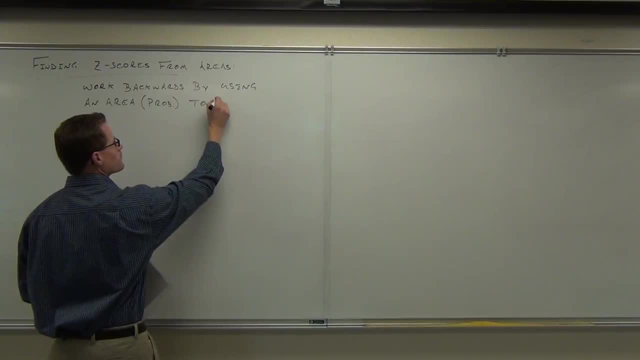 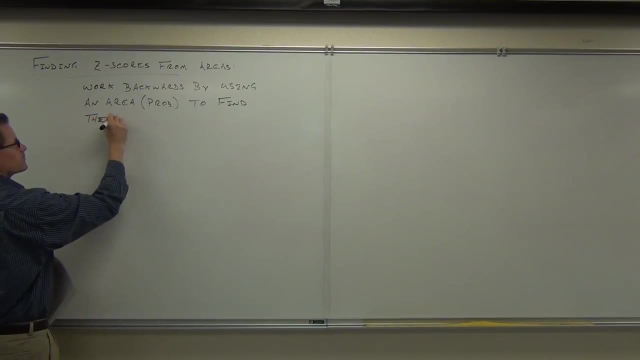 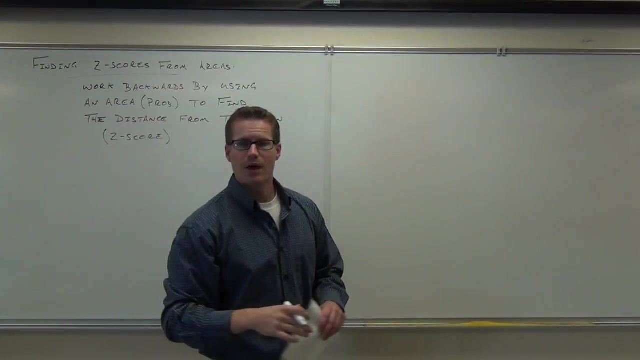 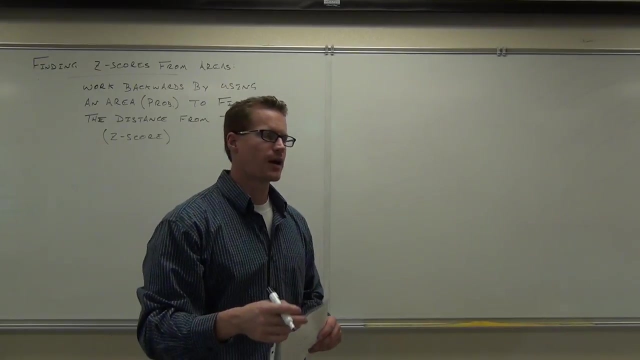 or in other words, a z-score. Now there's only really two things we need to do. The first thing we need to do is be able to draw an appropriate picture for this thing. So we've got to draw a picture, and then we're also going to have to find. 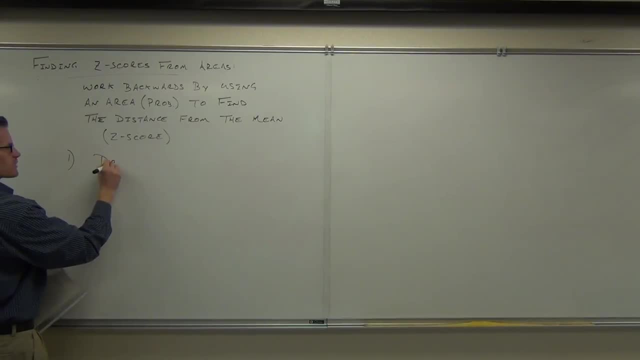 the z-score from an area. You're going to be drawing a picture, just like we've been doing every single time. Step two: we're going to learn how to use the table in reverse or your calculator. I can show you that too. 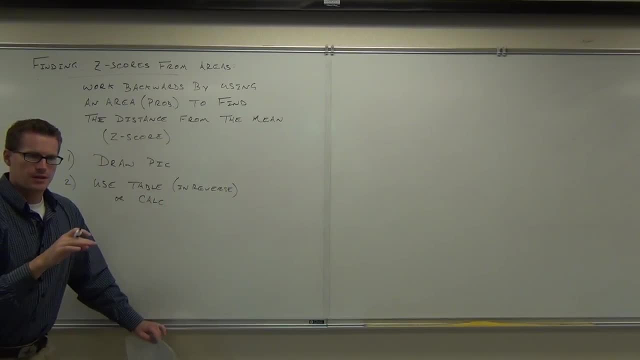 On your calculator you're going to find something- I think it's number three. Number three: on your distribution You're going to have something that says inverse normal. Inverse normal means backwards of normal. So when you do inverse of something, 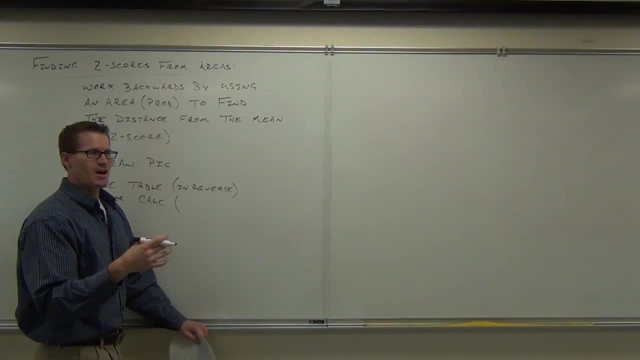 it undoes it. It undoes the operation. So inverse normal will be the opposite of looking up a z-score. It'll tell you a z-score from the area. So you're going to be looking for inverse norm If you have a calculator. 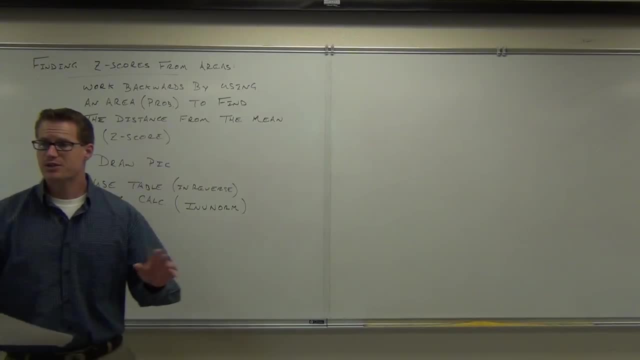 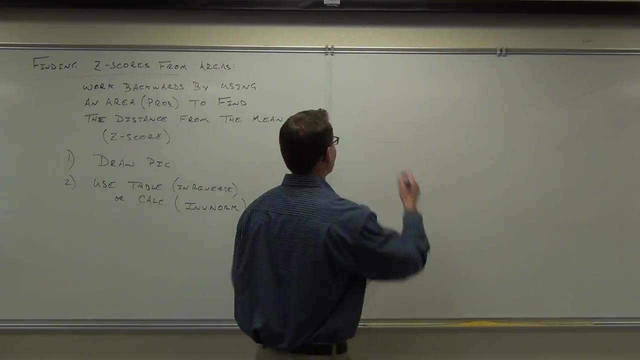 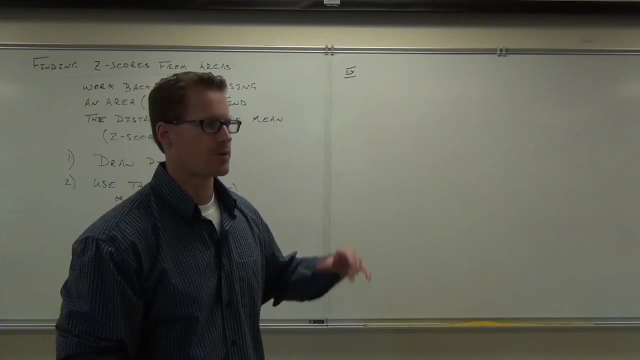 you might want to find that. Are you ready to do an example? Yeah, You seem super stoked about that. Alright, cool. Here's how your examples for this type of problem are going to look. Now we're going to use the thermometer example again. 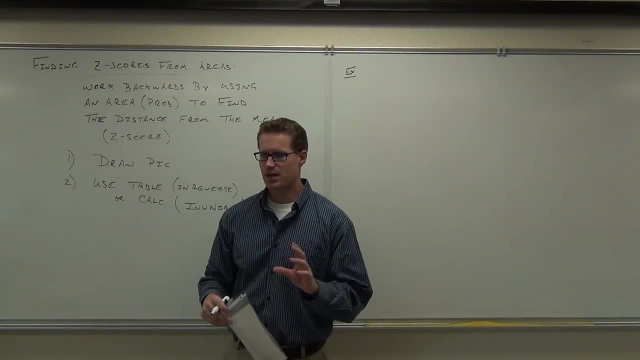 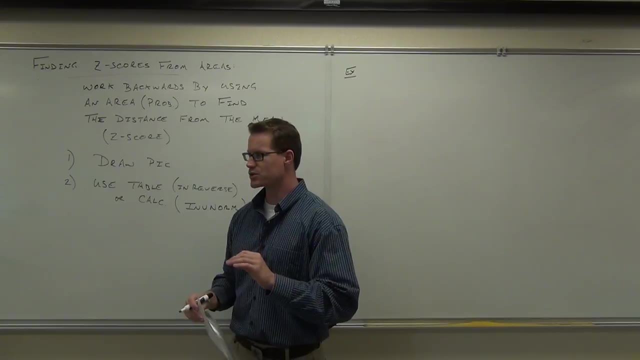 The thermometer criteria, which means a mean of zero and a standard deviation of one. I'm not going away from that yet. That's for the next section, But right now we're going to keep it very, very simple as far as the mean and standard deviation goes. 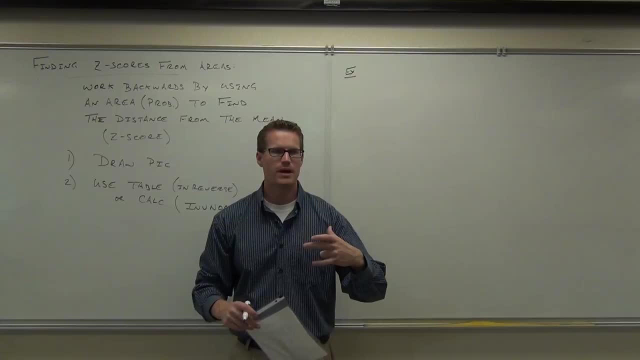 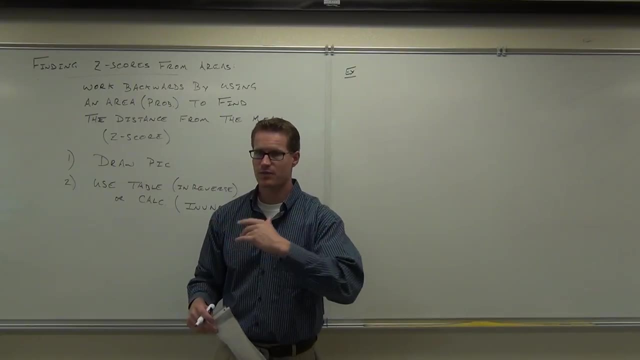 That way, our distribution is always standard normal. I'd love to hear if you're with me on that. Just remember, on what a standard normal distribution is, What the variable is for this particular section, chapter, which is a continuous random variable, and that a z-score will translate a normal distribution. 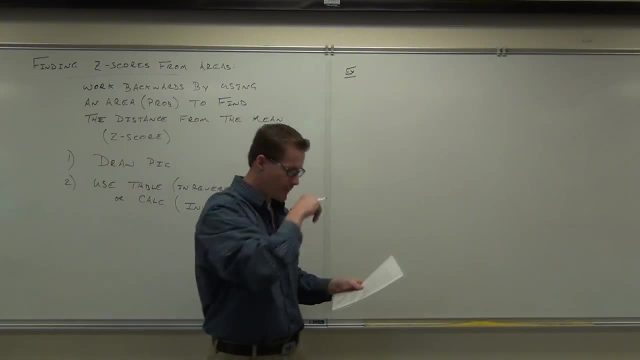 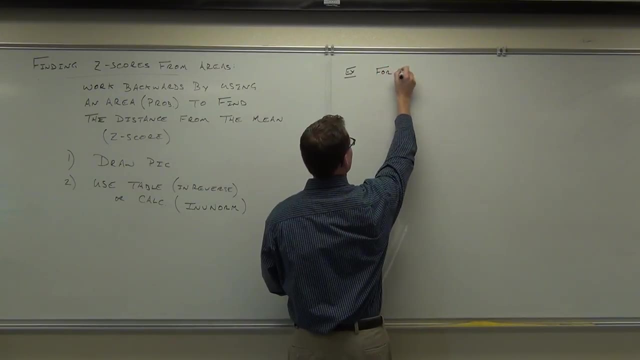 into standard. normal. That should always be in your head for this stuff. That's what we're doing In our example for the thermometers. what I want to do is find the z-score that represents the bottom 95% of the data. 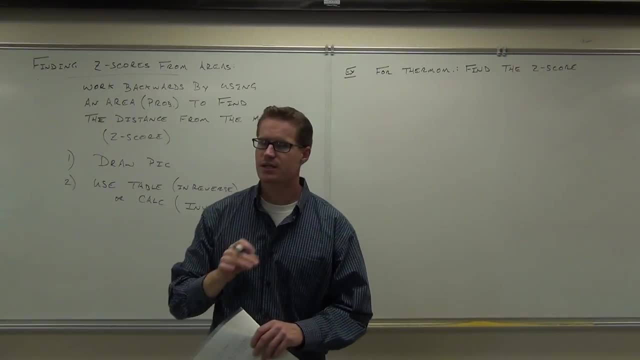 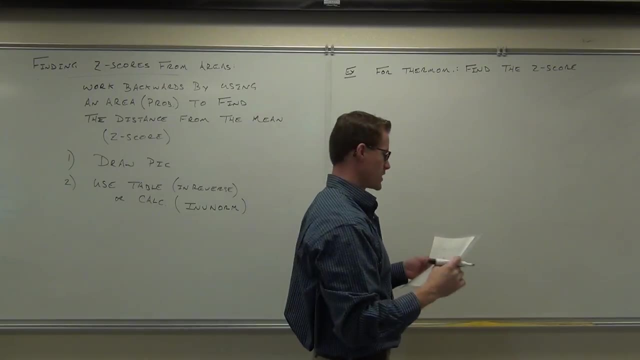 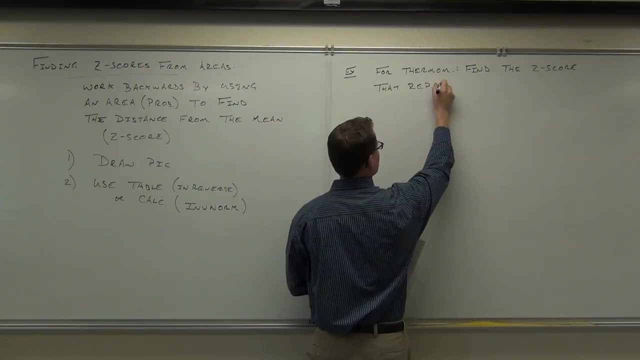 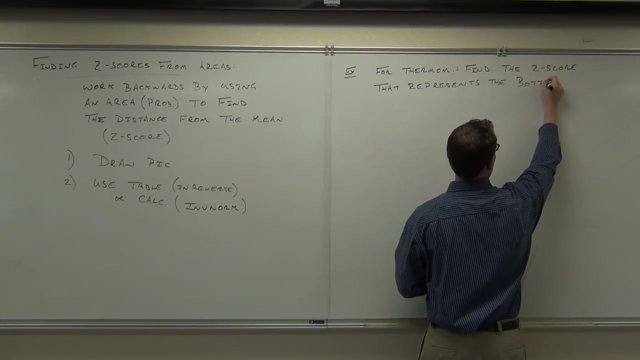 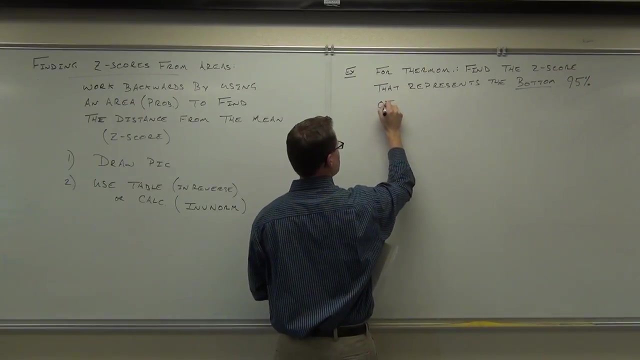 That's how a lot of these problems are going to be worded. Find the z-score that represents the bottom or top or middle, in this case the bottom 95% of the data. Before we go any further, I need to refresh and remember. 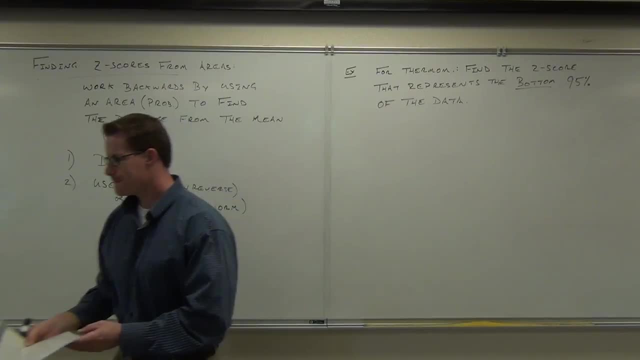 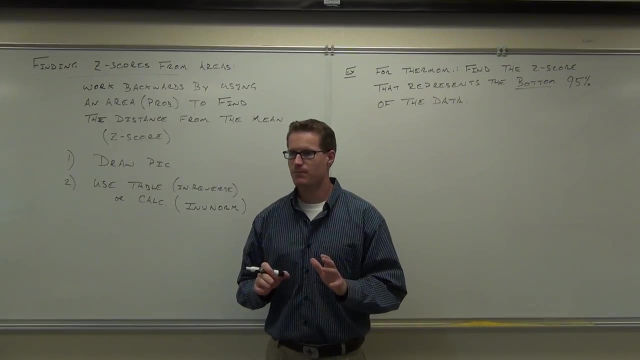 on this thermometer stuff. If you recall, the thermometers had a mean of 0 and a standard deviation of 1, which automatically mapped the thermometer reading to its own z-score. Do you remember that Like a thermometer reading of 1.38? 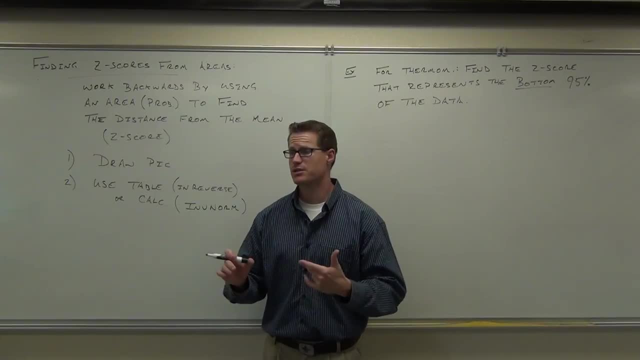 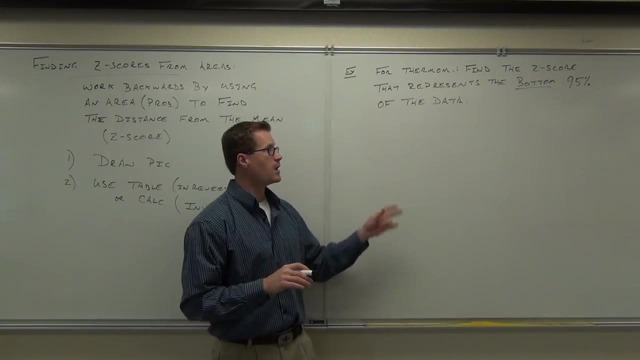 was a z-score of 1.38.. That's why this works so nicely for us. So what that means is, when we find a z-score for this, for this particular example, because the mean was 0 and the standard deviation was 1,. 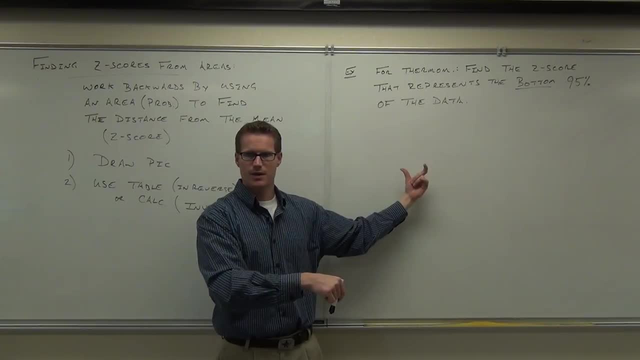 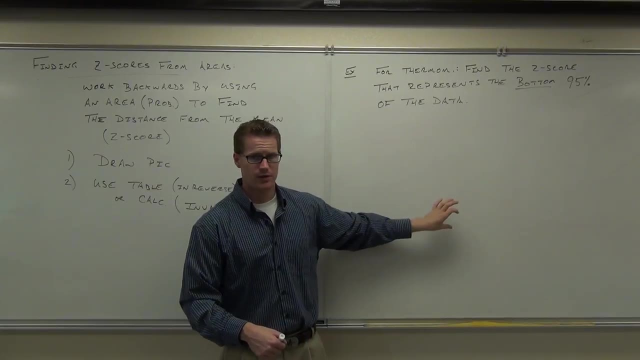 the z-score we find will be in the thermometer reading. Are you with me on that? Otherwise, we have to do a little bit more work and I'll teach that to you in section 6.3, how to go from a z-score to a value. 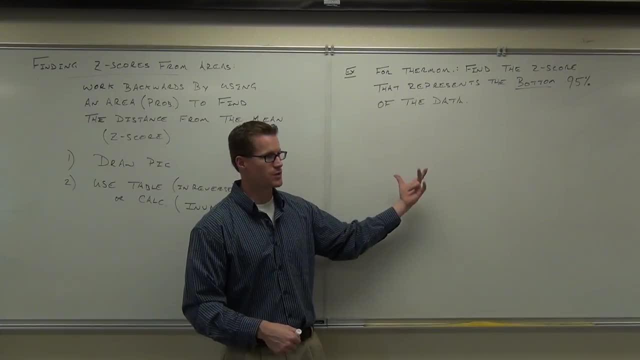 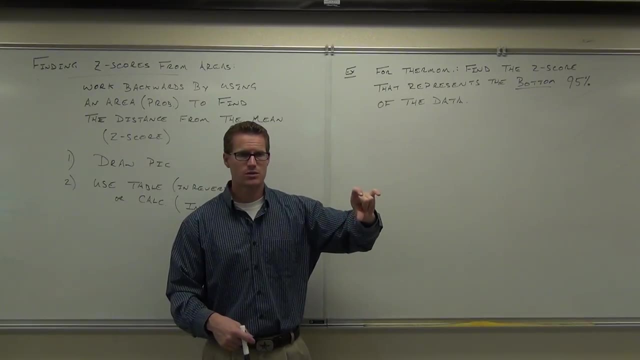 I'll teach you how to do that. It's not hard, but I'll teach you that. So, for right now, because the mean is 0 for the situation and the standard deviation is 1, the z-score is the value. is the thermometer temperature in degrees. 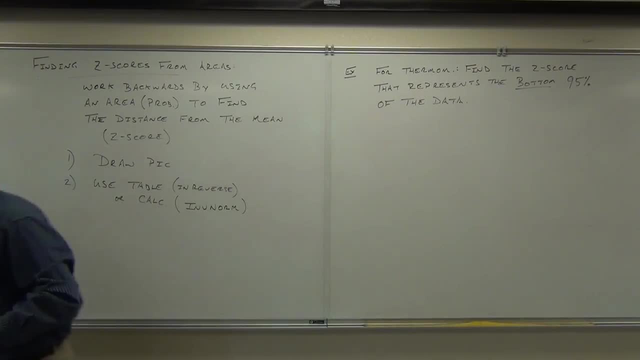 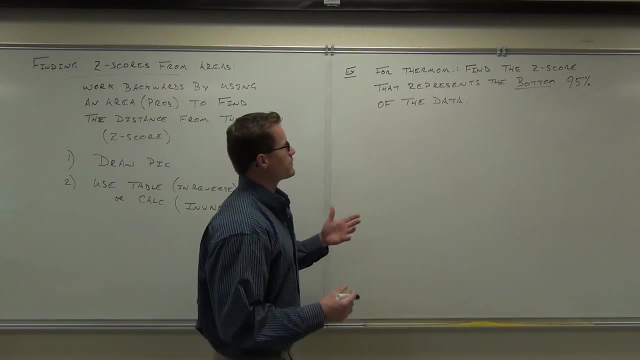 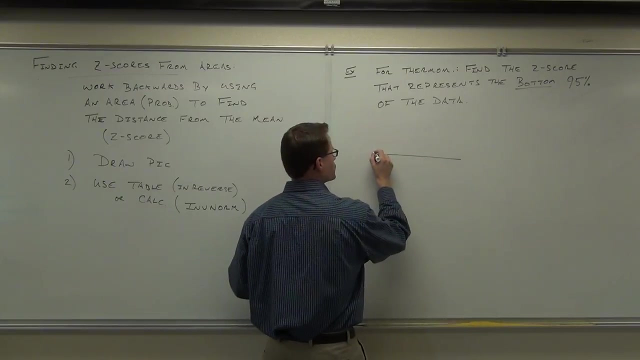 is the z-score. They're one and the same thing for this one example. Okay, so the first thing we've got to do, we've got to draw a picture. That's why I told you, in every single case, we are going to be drawing pictures in this section. 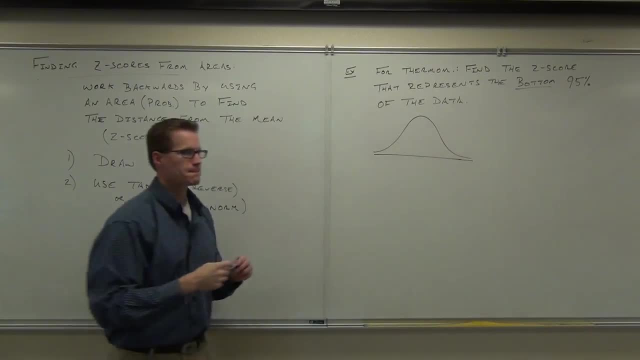 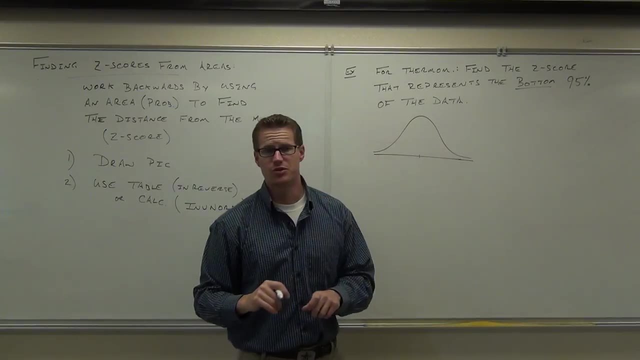 So we'll draw a picture here. Now. what you've got to know is a couple things. Firstly, what value is always in the middle distribution? 0, because our mean is 0 for every case. Okay, that's great. 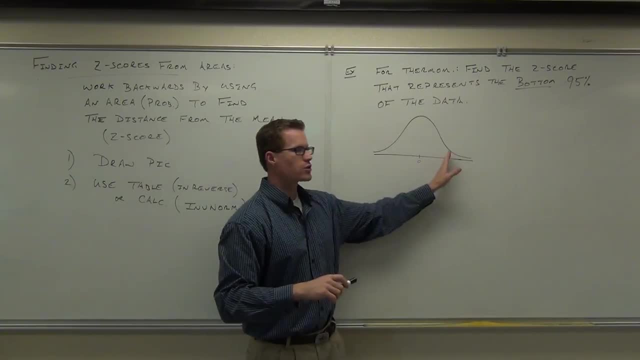 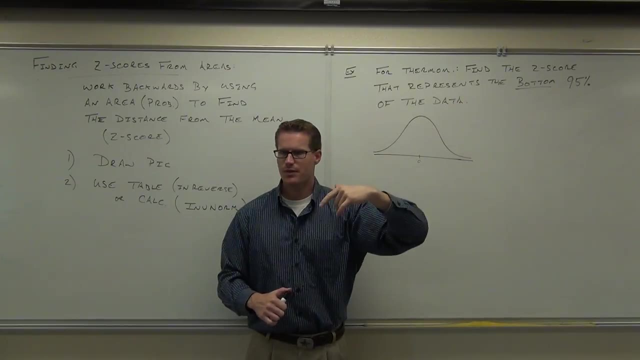 Now what we want to do. instead of looking for a z-score to a probability, which is what we've been doing this whole time, we're going to be going from a probability or an area to a z-score. Are you with me on that? 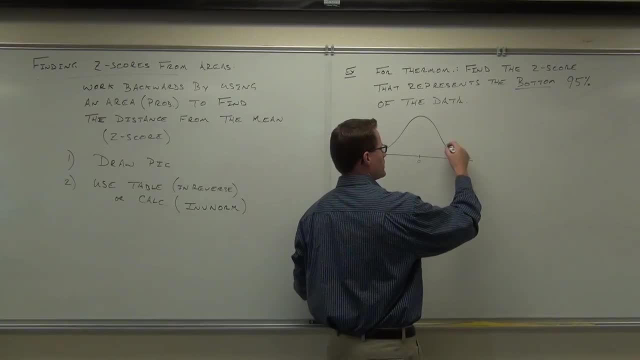 So normally this is what we would have happen here. We'd go: okay, I would be drawing a line, putting a z-score and shading one side of this. I'd be looking up that area in my table or in my calculator. 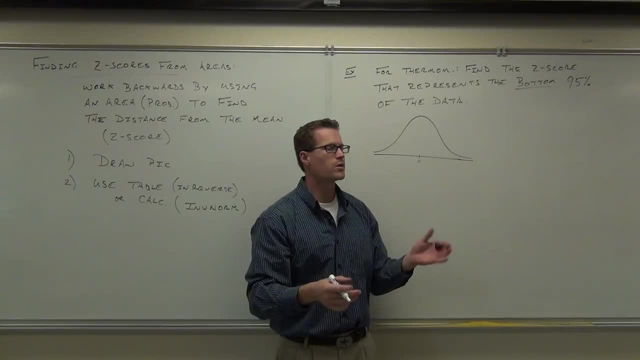 and that would be the probability. Now do you have your own z-score? Okay, Now we're going backwards. now, Instead of looking up a z-score, what I'm doing is reading this problem real careful. this says: find the z-score. 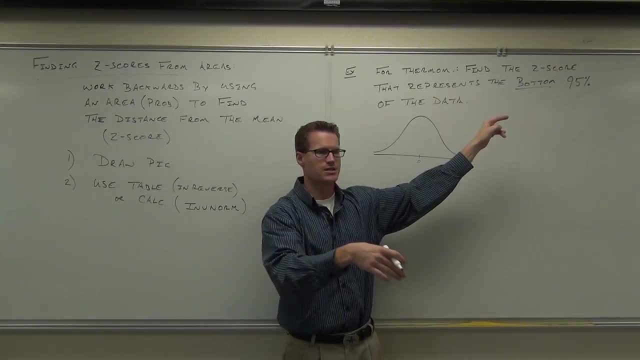 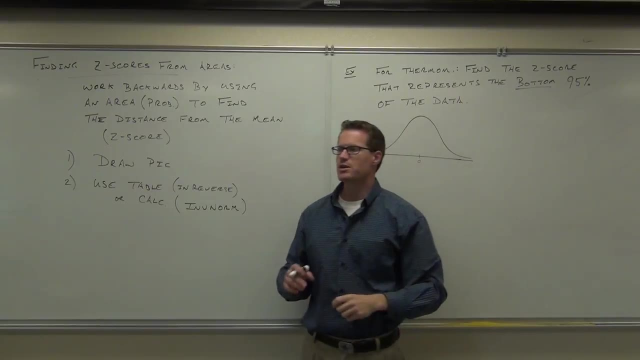 Oh wait, wait, wait. Before I was given a z-score, or before I had a z-score, I looked at the area. Now I want to find the z-score when I'm already given an area. You just have to be good about what the bottom. 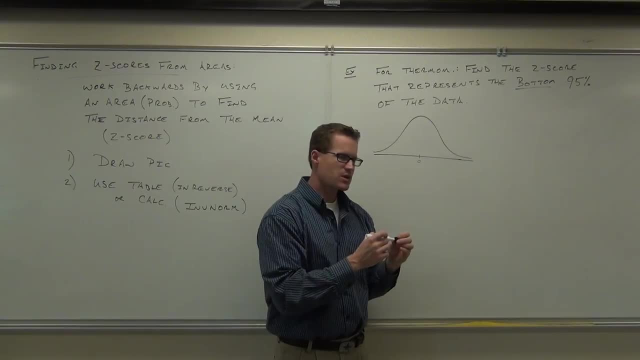 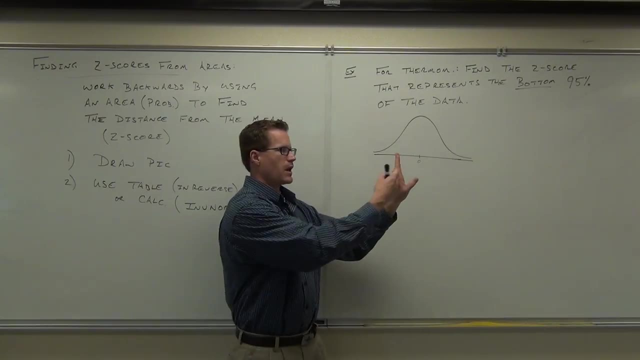 what the top and what the middle means according to this picture. If I'm talking about the bottom 95% of the data, the bottom 95%, that would be a value and 95% of it would be lower than that. Does that make sense to you? 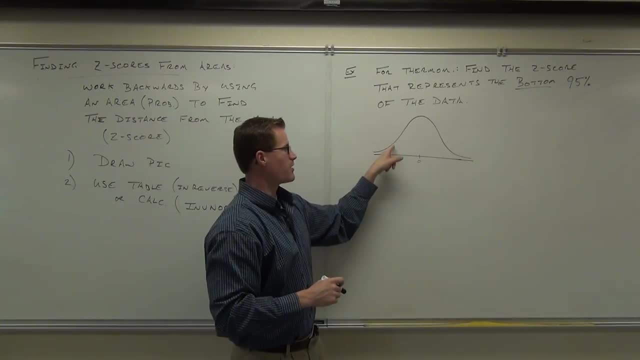 So where are we going to draw our line for our area? Is our bottom 95% over here? This would be the bottom, like 0%. Does that make sense? The way you can think about this, Locate 50% first. 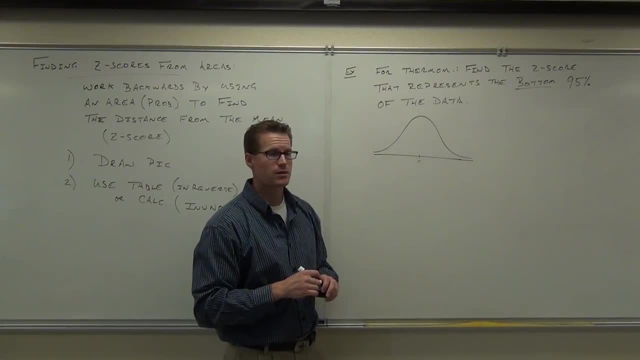 Locate 50% on your table. Where's 50%? Where's 50% Middle, Right in the middle. This is symmetrical right. I hope so. Would 50% be over here? Would that be half of it? We're certainly. 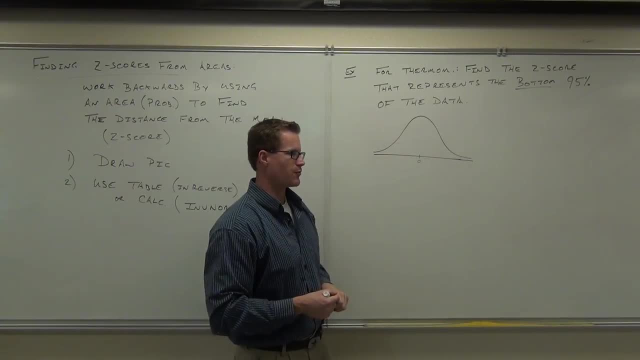 not going this way. We're going this way. So where's half your graph? Hopefully it'd be right in the middle, right? Would you agree that this is look up here at the board, please, that this is the bottom 50%. 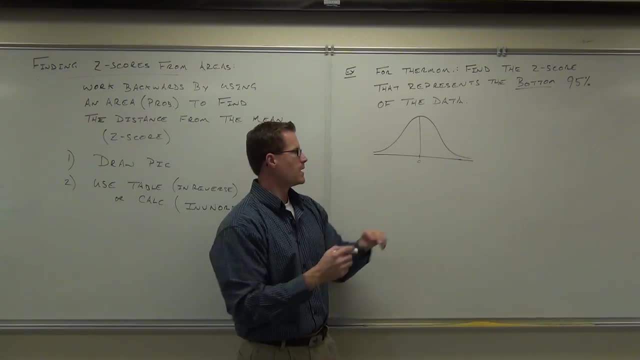 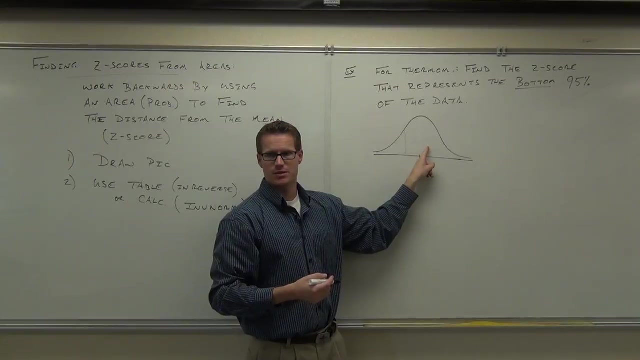 and this is the top 50%. Would you agree? Yes, Now, okay, If I draw a line over here, let's pretend that this is like 40%. Would you agree that this is the bottom 40% and this is the top 60%? 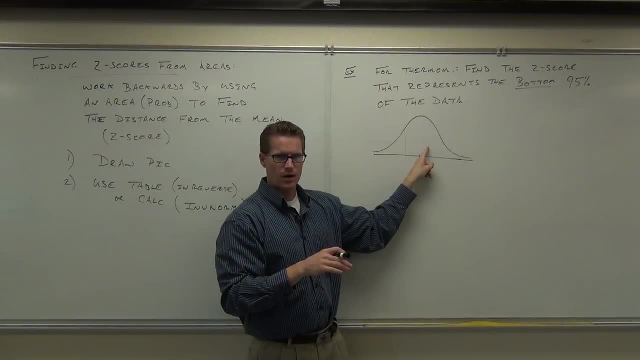 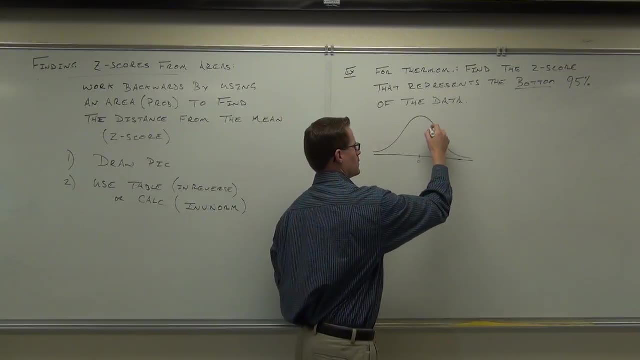 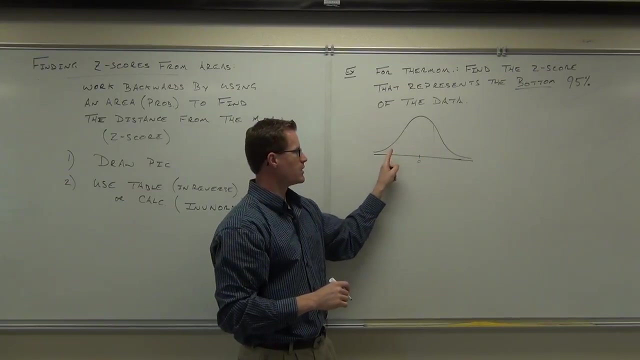 So if I say bottom 40% or I say top 60%, do you see I'm saying the same thing? Would you say that this is the bottom 60% and the top 40%, Is that okay? This is the bottom 60%. Notice that this. 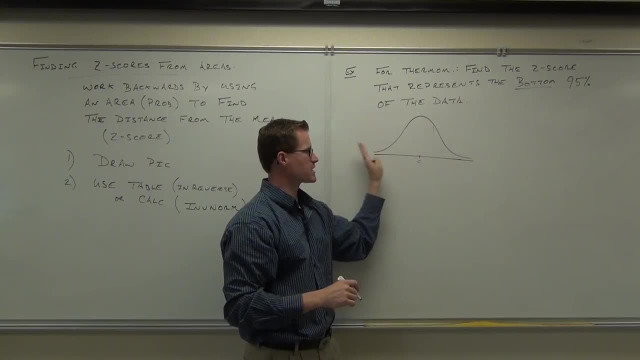 would be like the bottom 10%. This is the bottom 50%, This is the bottom 60%. Where's the bottom 95%? Am I going to draw my line over here to the left or over here to the right? 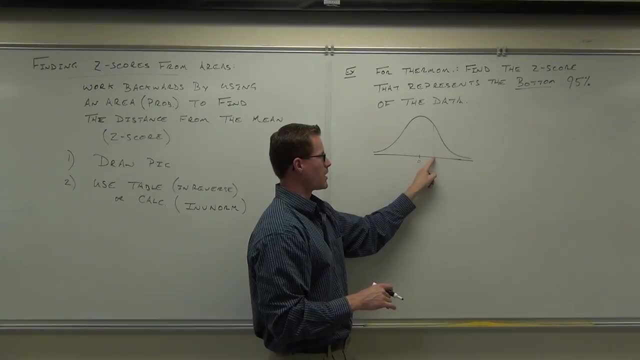 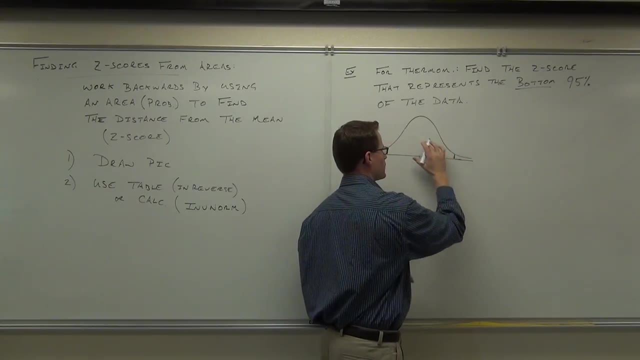 To the right. This would be the bottom 50%, the bottom 60%, the bottom 70%, the bottom 8.. This is like the bottom 95% Shade, what you were talking about. If I want to find the bottom 95%, 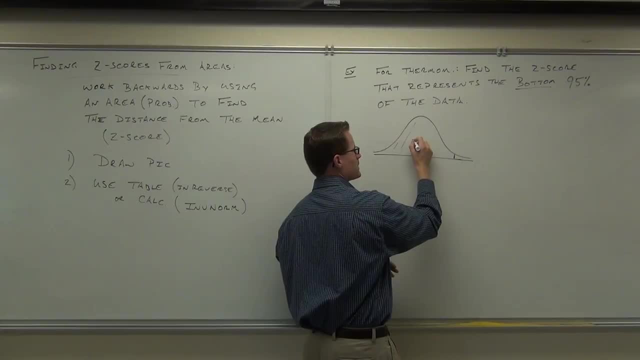 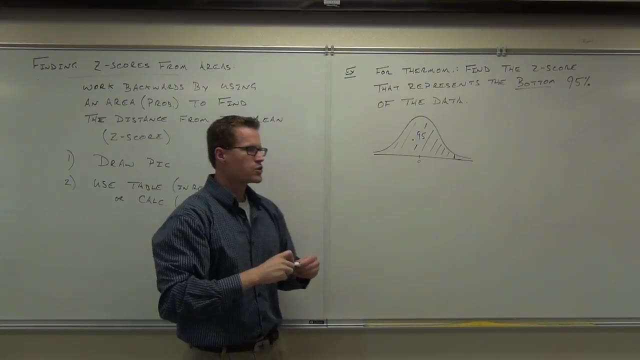 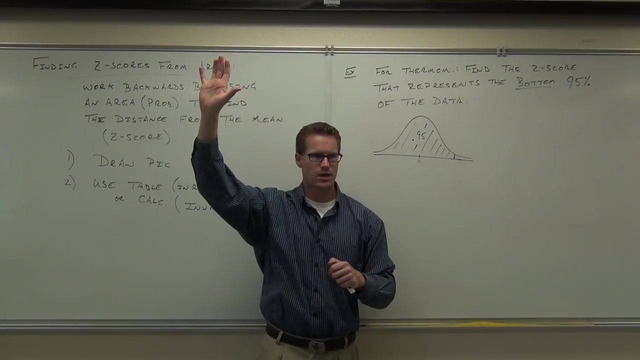 it's. 95% of the data is below that number. Would you raise your hand if you feel okay with that? An honest raising of hands if you're alright with that. Okay, some people didn't. I can't move on unless you do. Are you guys okay with this or not? 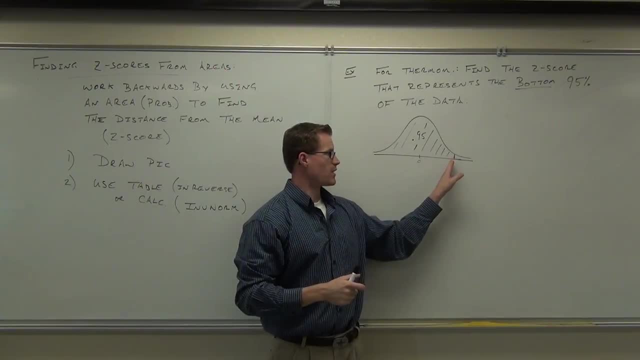 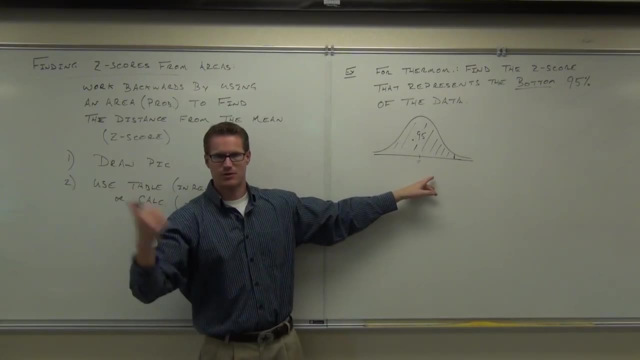 Yes, That this is the bottom 95%, or this value is going to represent the bottom 95%? yes, Now what I'd like to do. did you have this picture drawn? Okay, so I'm going to have to lower that screen over there. 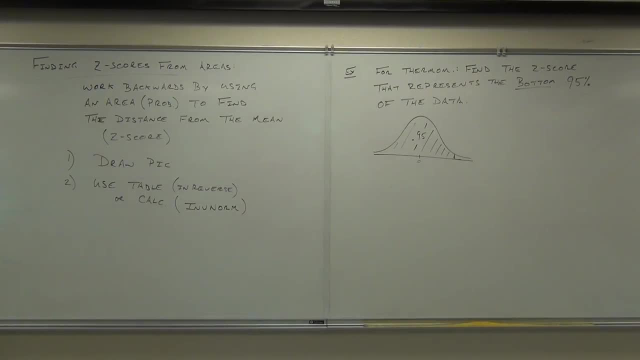 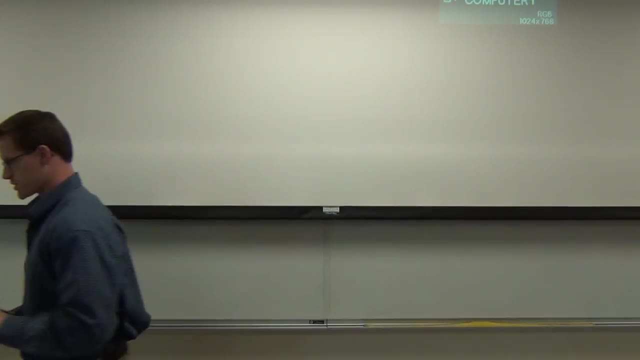 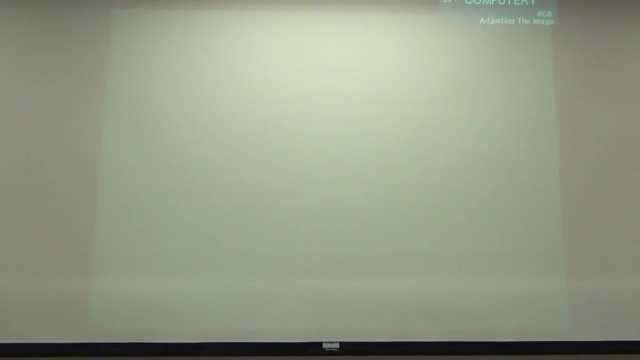 What we're going to do now is I'm going to show you how to use your table so that we can find the bottom 95%. Okay now, I've asked you to bring this to every class from now on. Take out your table. 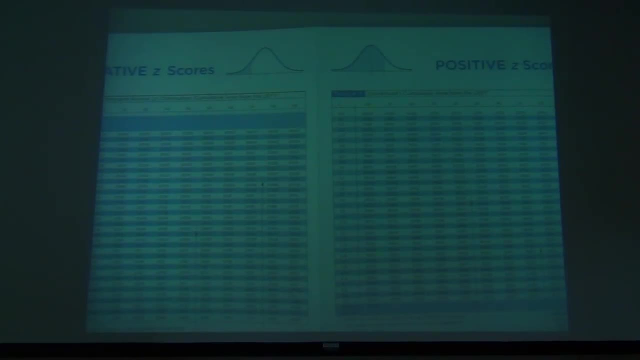 Okay, Hey, folks, thinking back to that picture we just had on the board, do you think that we're going to be in this situation with a negative z-score or this situation with a positive z-score? What do you think? Where was the line drawn? 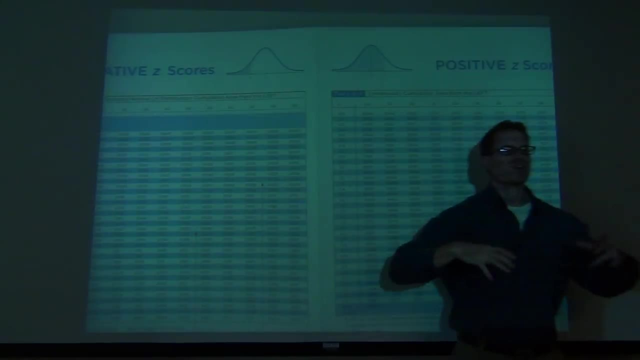 Was it to the right of zero or left of zero? Definitely the right. That's why you have to be very good at knowing the bottom 95%, the bottom 10%, the top 30%. You've got to be very good at that. It's like the more 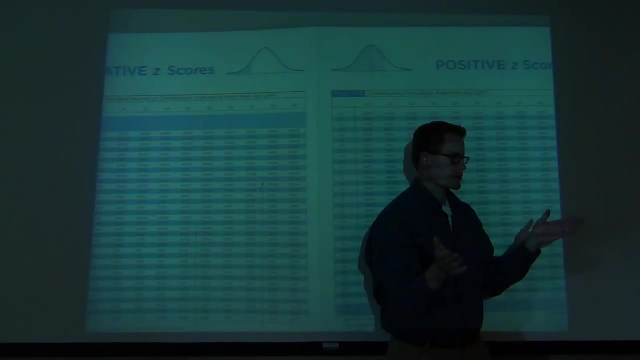 than less than thing. Remember that If you didn't know more than less than you were stuck on those problems on your test. Here you're going to be stuck if you don't know how to draw a picture of the top 5%. 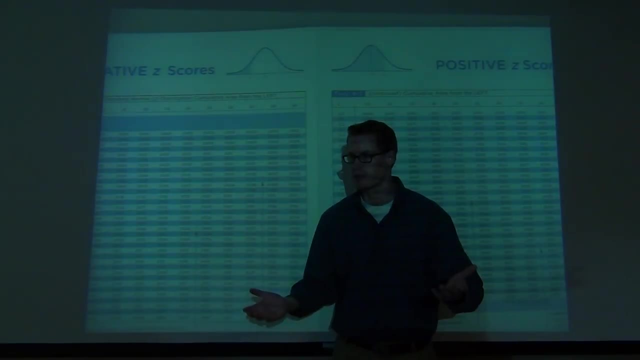 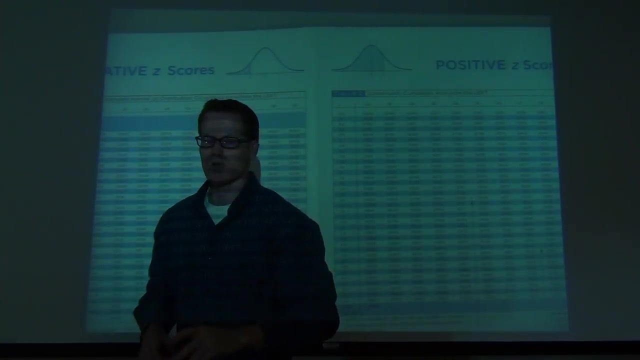 Which, coincidentally, is the same thing as the bottom 95%. That's the same exact thing. So here we're dealing with the bottom 95%. Our picture looked like that. That's why we draw a picture, So we're over here in this situation. 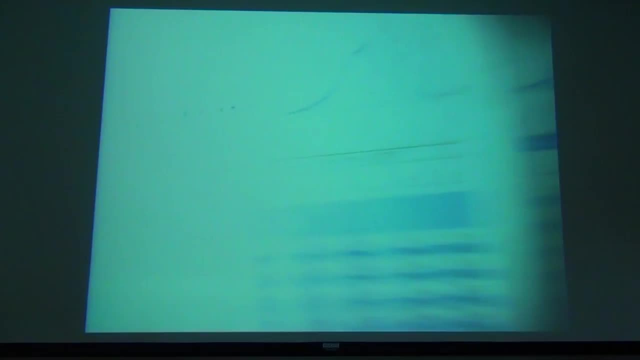 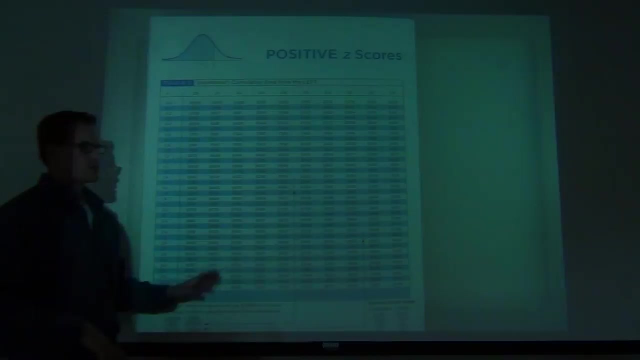 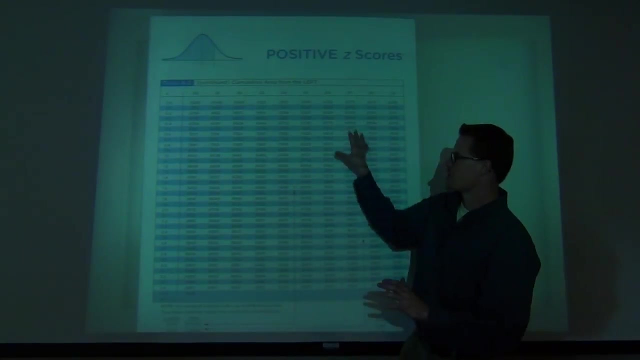 So I'm going to ignore the negative z-scores. Go over here to the positive z-scores And let's think about what this table actually means. Can you tell me which are the z-scores? Are the numbers? let's call this the bottom 95%. 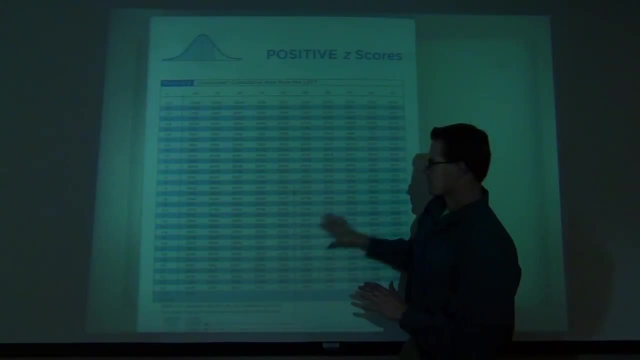 or the body? Are the numbers in the body of our graphic here. are these z-scores, Or are these z-scores Which one? The body or the size? The size of the z-scores Good, What are these? 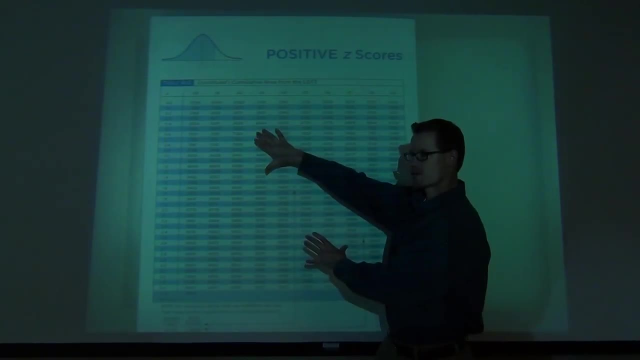 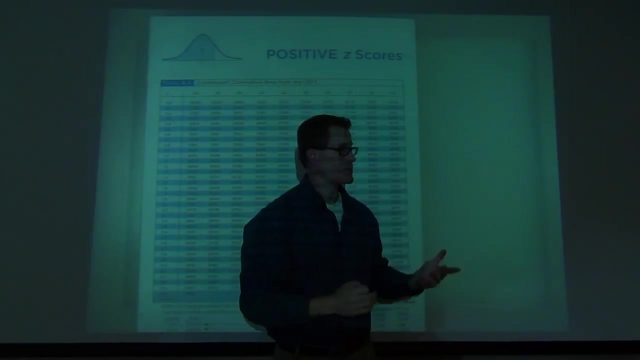 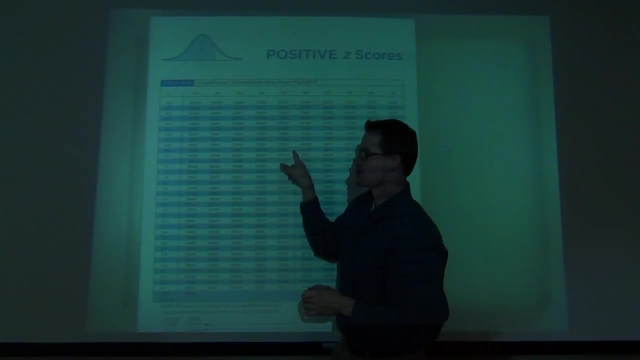 Areas. These are areas, These are z-scores. True, You can't confuse that. You can't confuse that Because if you go right now and you look up 0.95, you can find it. 0.95 is right here. 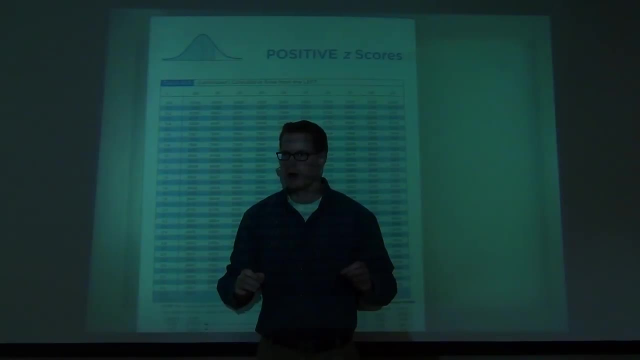 However, you'd be looking at a z-score Right. We're trying to find a z-score right now. I've actually given you the area, So you need to know the difference between a z-score and an area. The z-score is the distance. 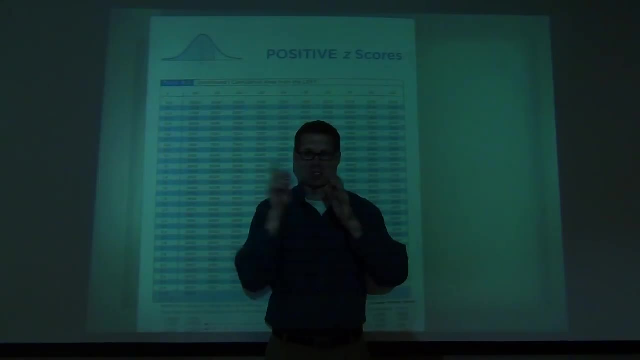 from the center, from the mean, The area is the shaded region. We're going to be going two ways on this graph. If you have a z-score and you're looking for an area, you look up the z-score. these are your areas. 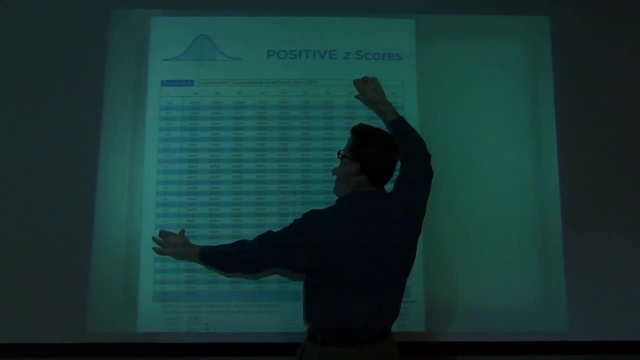 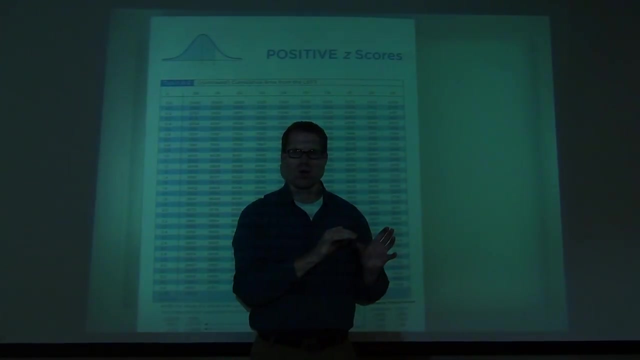 We have areas here. We've got z-scores on the sides. What have I given you here for this example you have on your paper right now? Have I given you a z-score to look up, Or have I given you an area to look up? 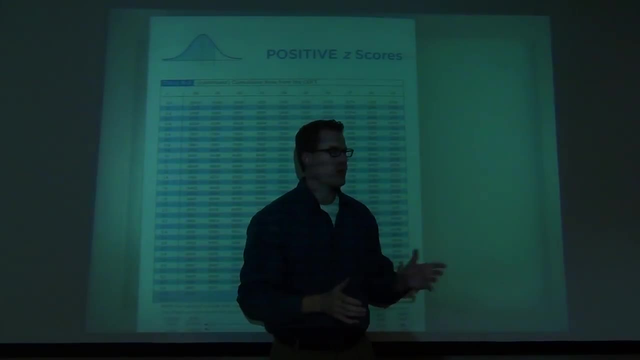 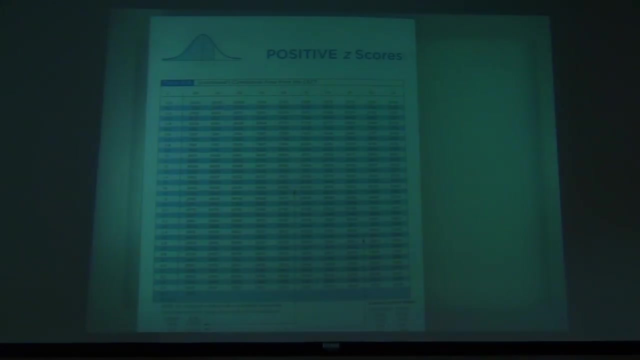 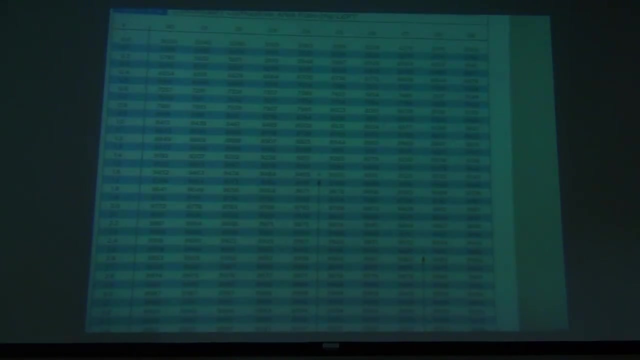 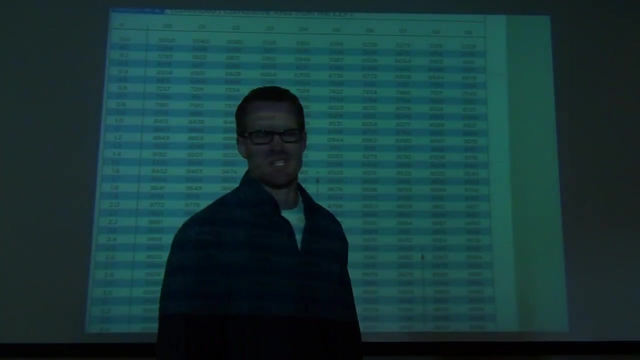 Area? Definitely an area. Let's see if we can find it. Let's go down here. I need to zoom in a bit. We're looking for 95 percent. How much is 95 percent? 0.95.. Can you find 0.95?? 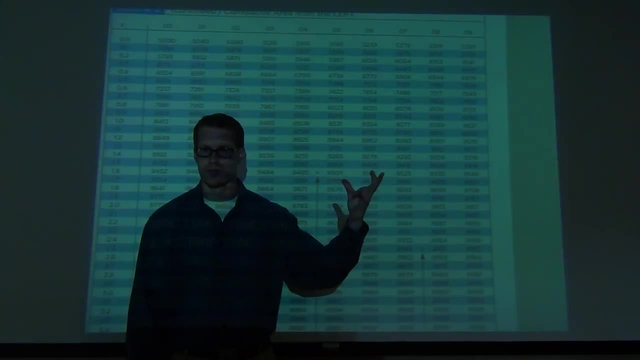 Notice, these are all four decimal places, That's 0.9500.. What we're doing right now, if you're not with it- we're looking up an area and we're going to find the corresponding z-score to that area. I've given you an area. 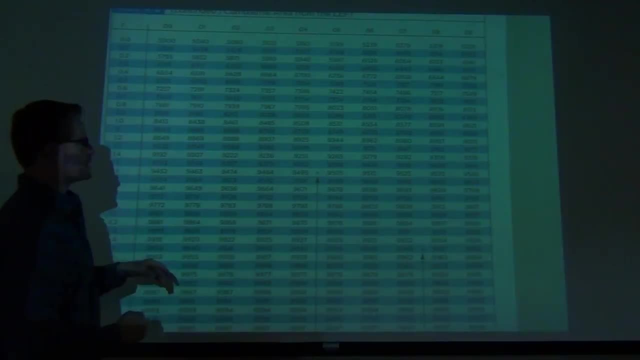 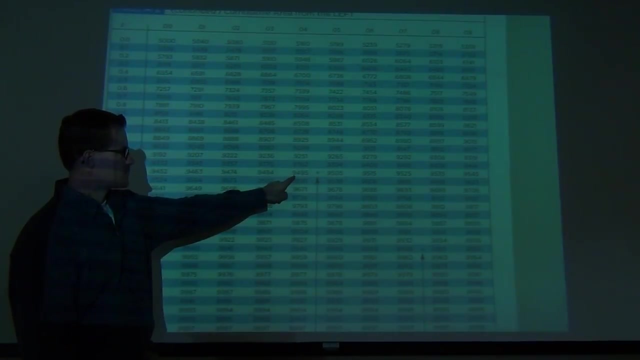 That's why you shaded it. The area was 0.9500.. Let's find it. Here's 0.93.. Wait a minute, That's 0.9495.. That's 0.9505.. It's right in between there. 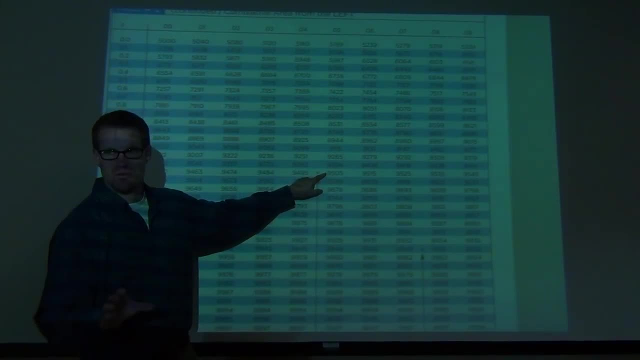 Right now it says: here's how you do this. for normal, Let's say: this was exactly here. By the way, you're not always going to get the exact value. It's in between here, These jump. There's not every single value. 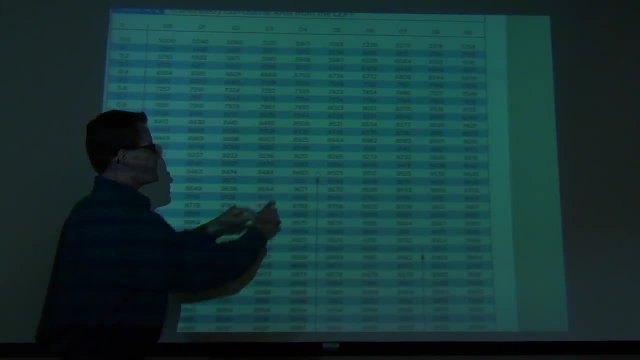 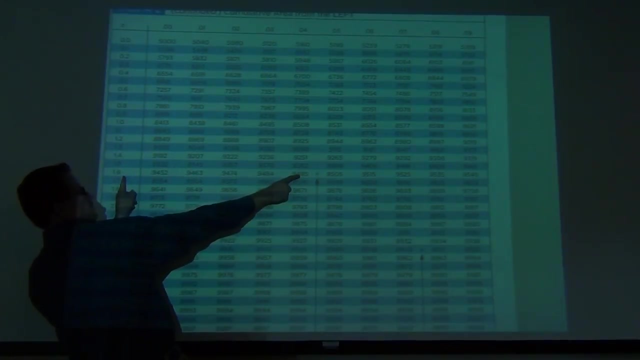 Your calculator will give you the exact value. It's not right there. Let's say it had been that one. Could you find the z-score that correlates with this 0.9495?? You would have 1.6. what 1.64.. 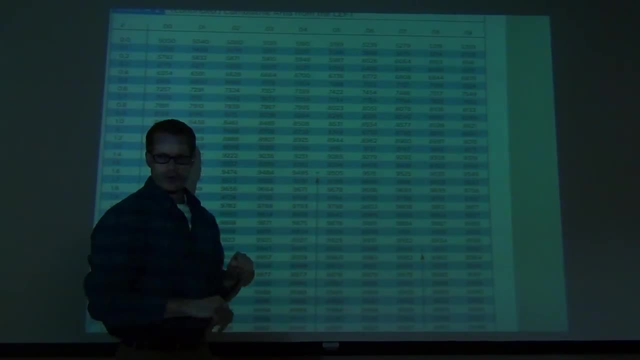 This one would be 1.65.. Are you with me on that? There's a few special numbers here, Like the 0.95.. You're going to notice there's a little asterisk right there. What in the world is that asterisk doing? 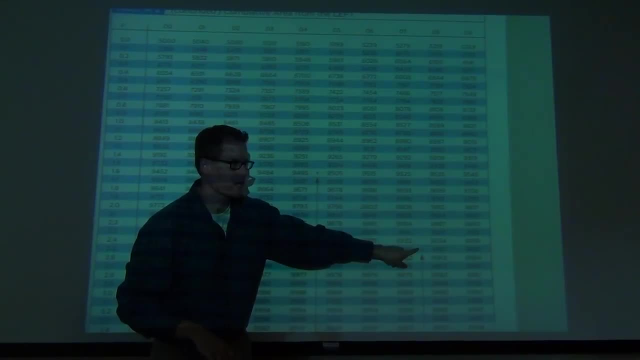 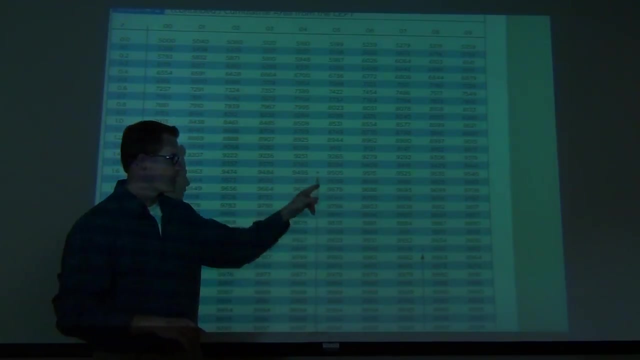 They've actually calculated this one special. They've calculated that one special for you: 0.995, because we use those all the time. You're going to find that in chapter 7.. We use those a lot. This has a special little value. 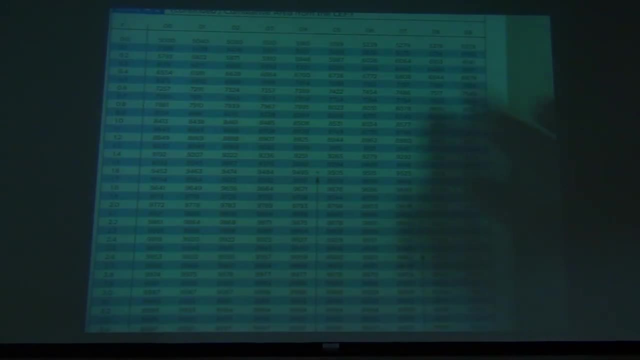 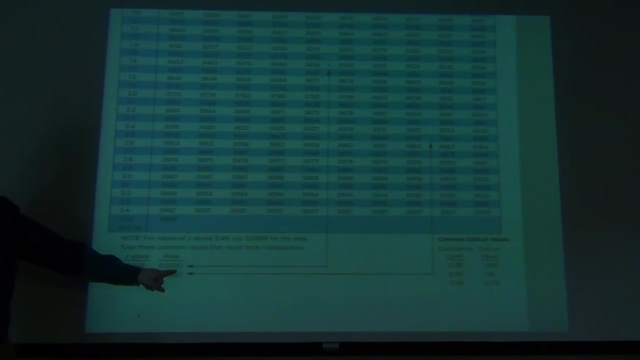 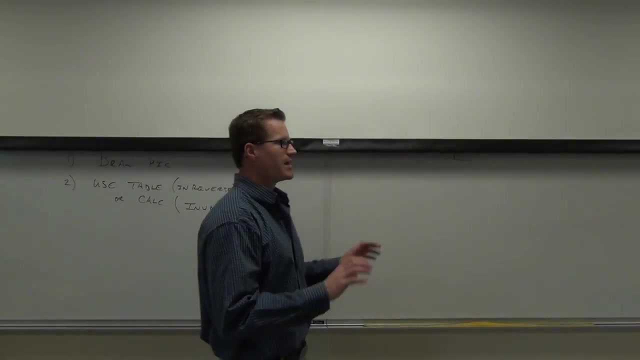 On your table. Follow that down, See where it goes. What's the z-score that's associated with an area of 0.9500? 0.9500.. Here's what you just did on your table. Hopefully you all had your table out. 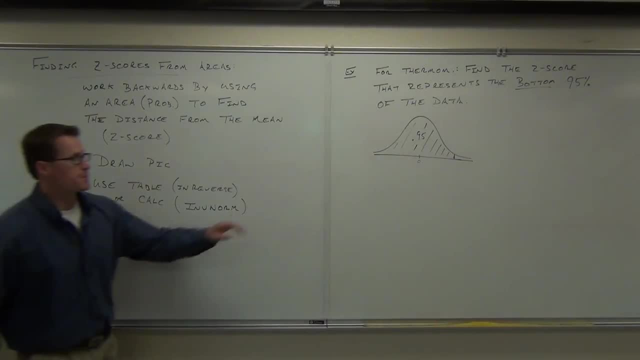 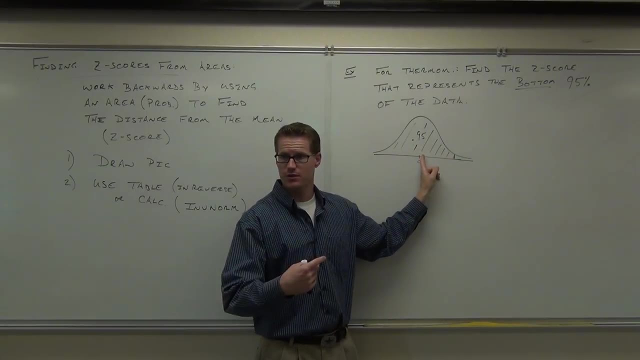 I'm requiring you to bring that from now on. We just looked up this area. We noted that we looked up an area to the left that was 0.95.. Remember, it was always an area to the left, Correct. This worked for us because all the area we wanted 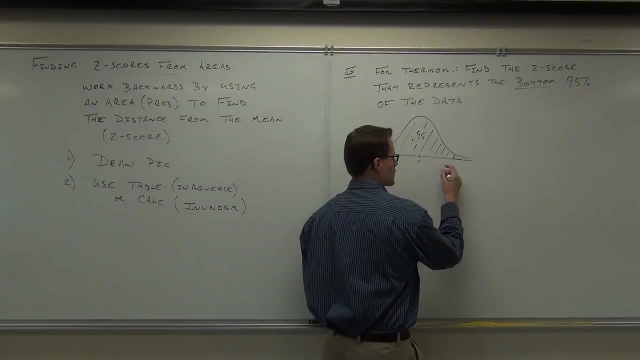 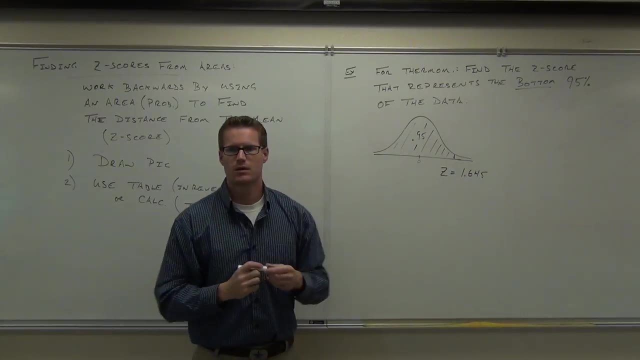 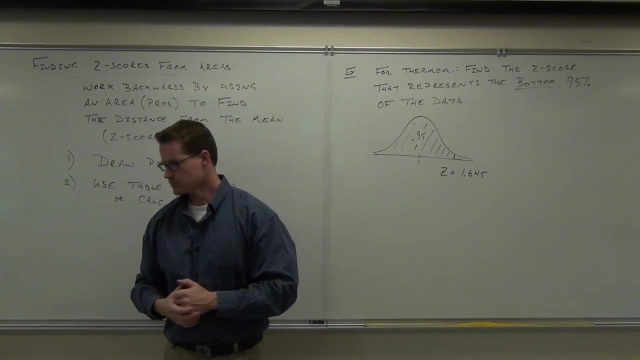 was to the left of that score. We looked up that area and it gave us a z-score of 1.645.. Are you with me? You'll feel okay about doing that Now. the interpretation is important. The interpretation says area and probability. 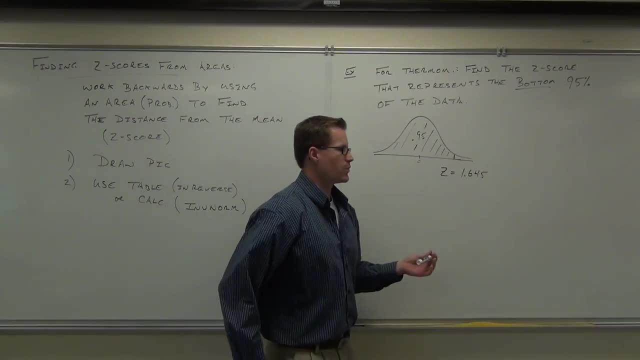 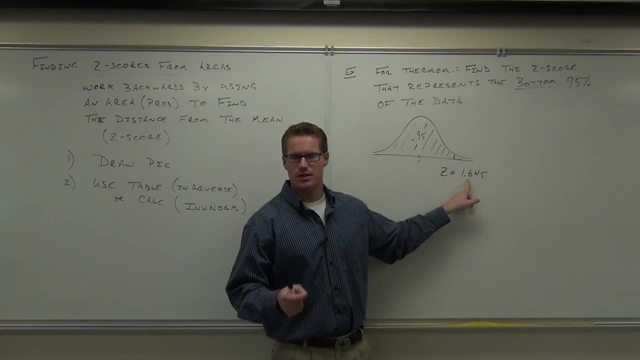 are the same thing. Here's what. and proportion is the same thing. What we said was 95% of the thermometers. in this case, 95% will have a reading of less than 1.645 degrees when dunked in cold water. 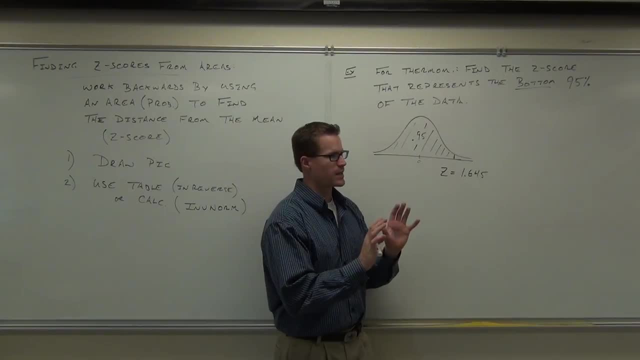 That's what that says. Remember, the one reason why I can say 1.645 degrees is because the mean was 0 and the deviation was 1.. So a z-score is a degree in this case, In this one case, And a degree is a z-score. 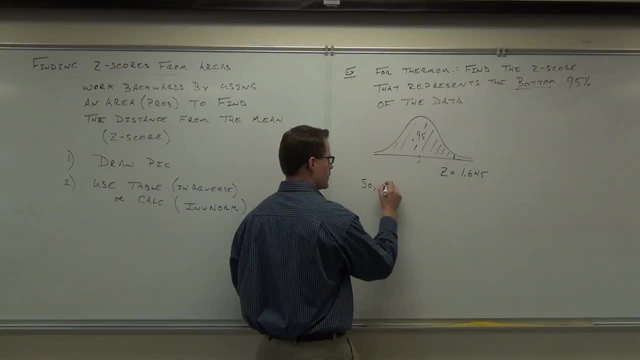 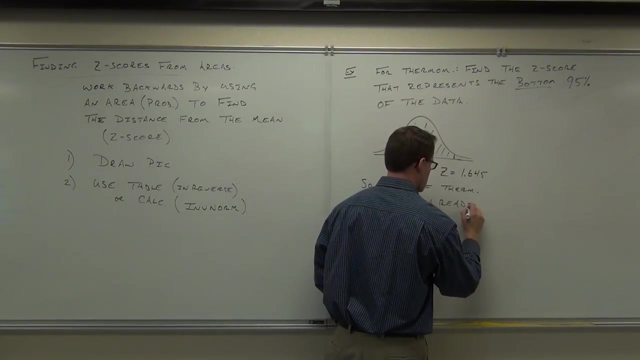 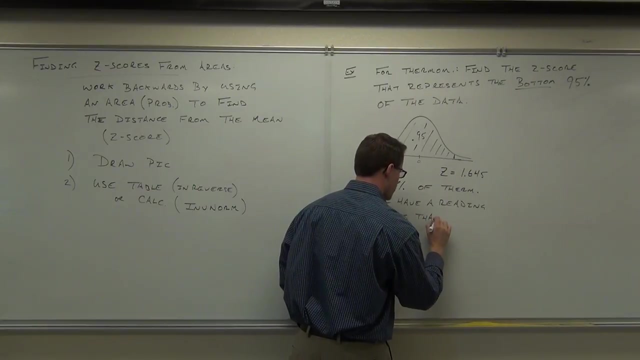 So this interpretation says this. So 95% of the thermometers will have a reading of less than 1.645 degrees, And this, of course, is when it's dunked in water that's free like 0 degrees. That's what that means. 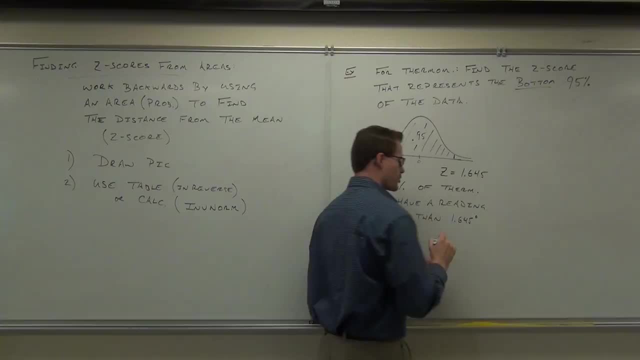 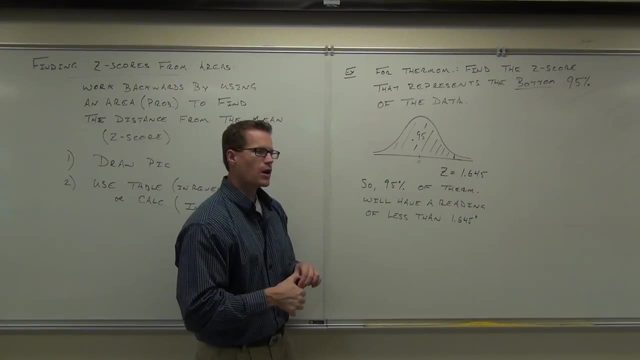 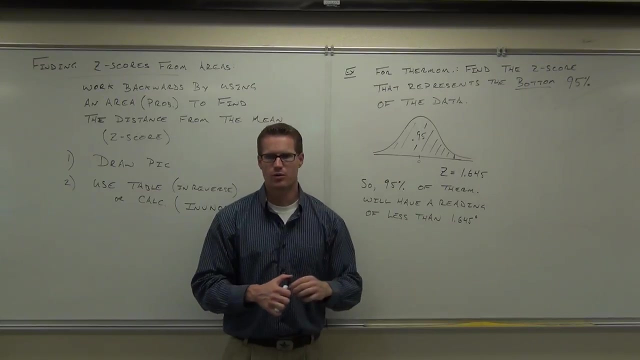 Also, you could do this interpretation: There's a 95% chance that if you randomly select a thermometer, it will have a reading of less than 1.645 degrees. The same exact interpretation right there. So 95% of the thermometers will have a reading of less than. 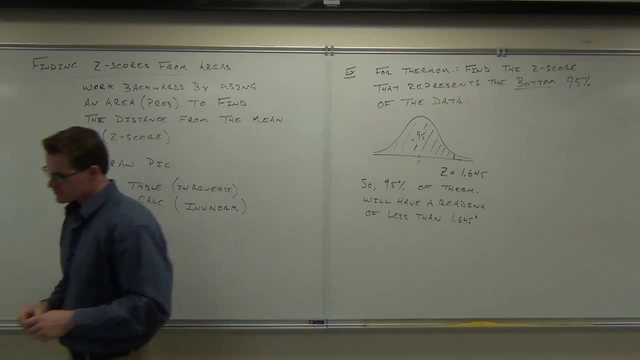 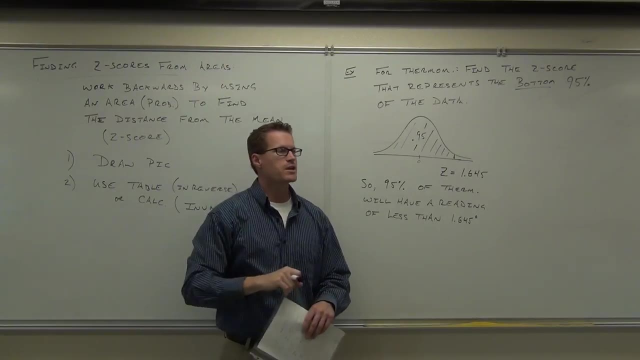 1.645 degrees. So how many people feel OK with this so far? How many people feel OK with this so far? I want you to try something with your calculators right now. I want you to try something with your calculators right now. 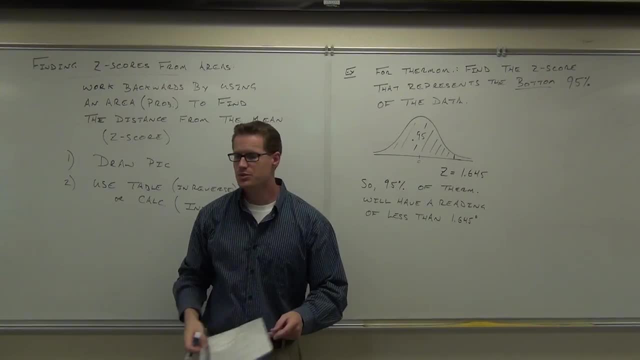 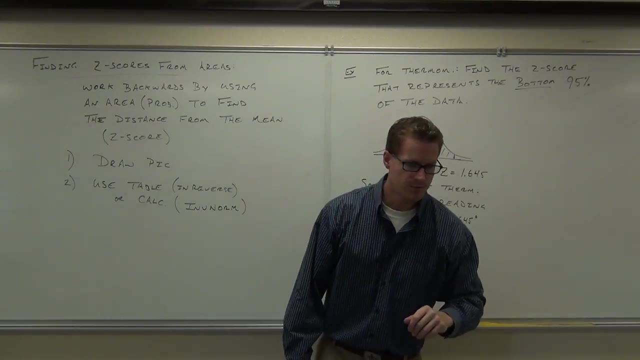 If you have your calculator do this. I want you to go to your distribution button. I want you to go to your distribution button, like we've been doing in the past chapter. so, second Vars button, Go down number 3.. It should be inverse, normal. 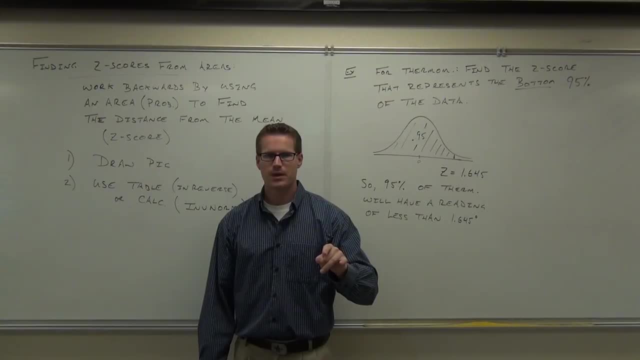 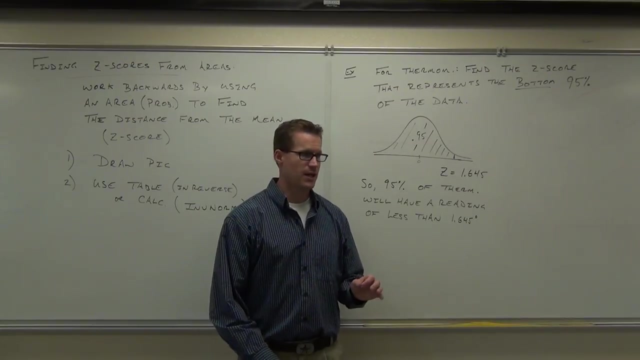 Do you see it? Press that button. You just have to be careful on this. Your calculator does not know you're actually asking for. You always have to give it, just like your table, the area to the left, The area to the left. You have to do that. You have to give it that. We'll. 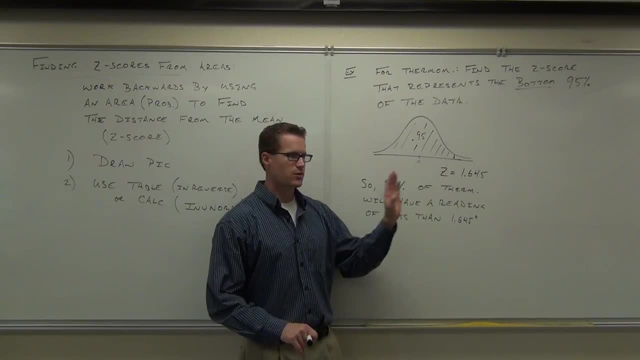 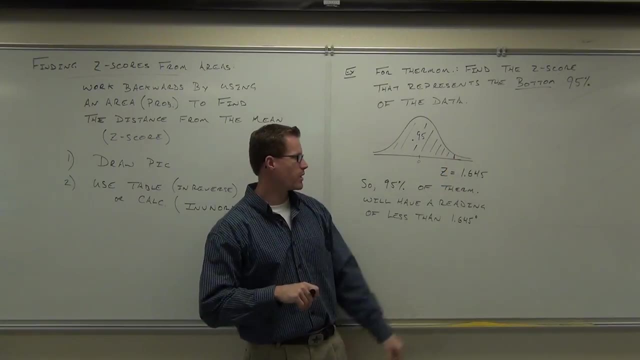 talk about some examples in just a little bit. You have to give it the area to the left of whatever you're looking at Here. I have to plug in .95.. Try that on your calculator. Plug in .95,, press enter. You should get .16446 or something like that. 1.44, is it six? 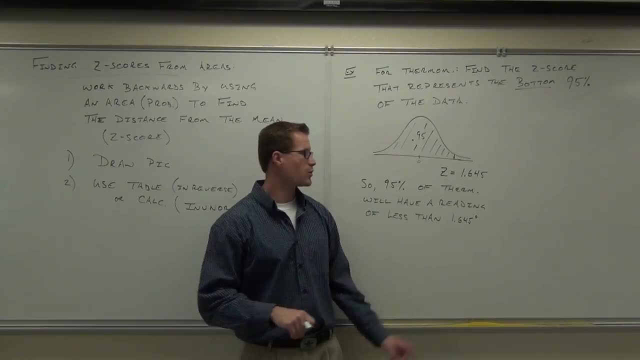 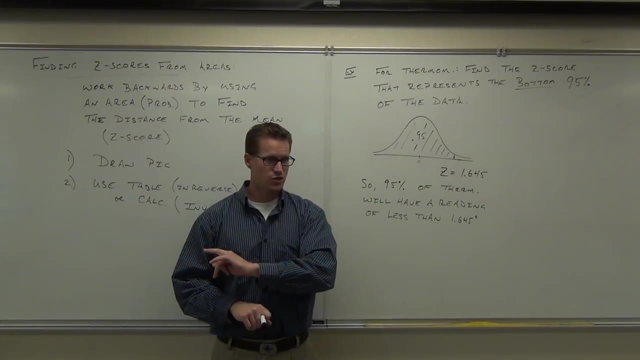 1.6, 448.. 448, okay, 1.6, 448.. That rounds to the 1.645, which is how they got it on their table. See how you can use your calculator or the table. either one It's fine, Let's. 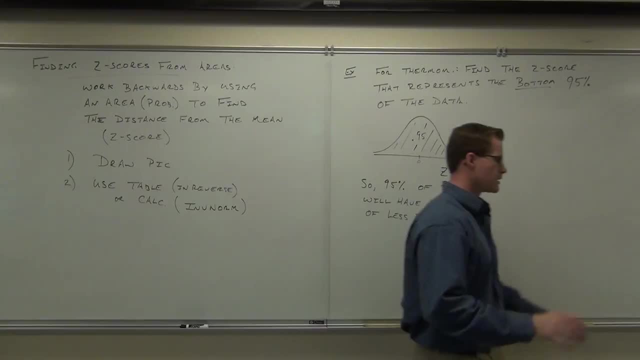 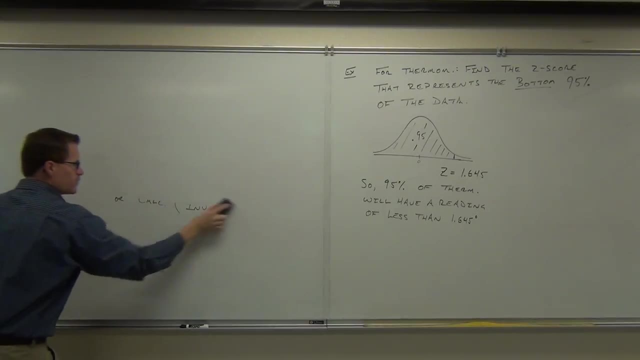 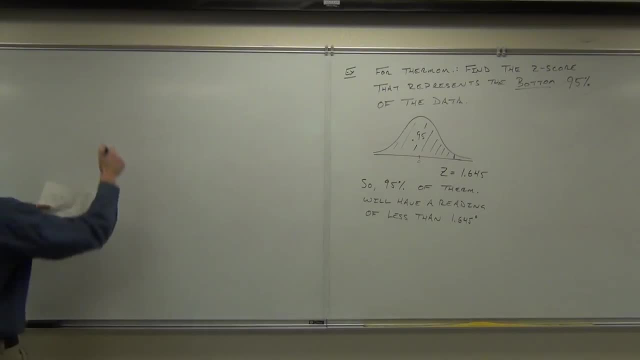 just going to talk about them and drop pictures from them. I need you to be able to draw pictures for something like the top 30 percent, The bottom 10 percent, The top 80 percent, Bottom 10%, the top 80%. 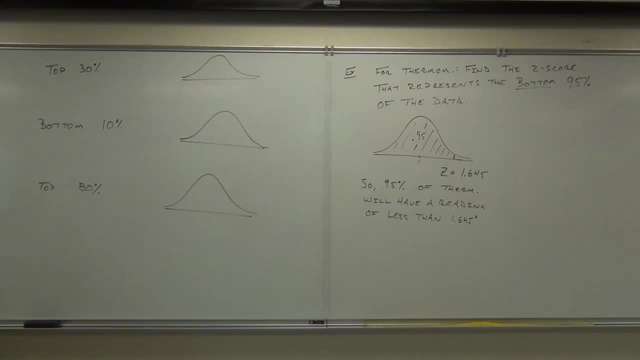 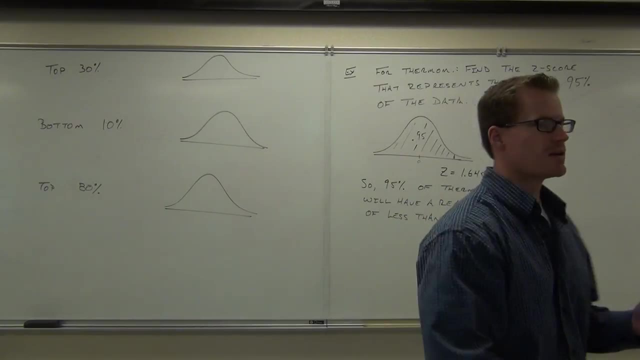 Okay, the first thing we want to do is be able to identify what these pictures look like. We're going to go through right now. We're going to do all of our pictures at once. Then we'll talk about how to compute them in just a bit. 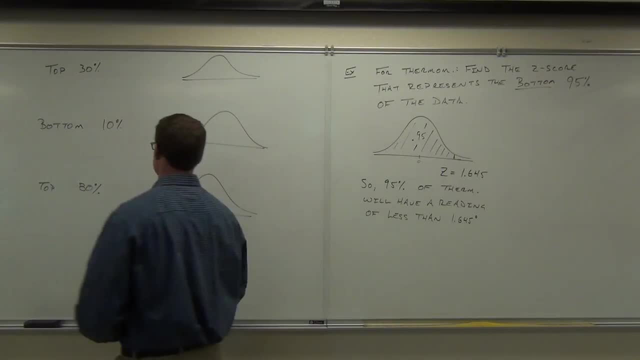 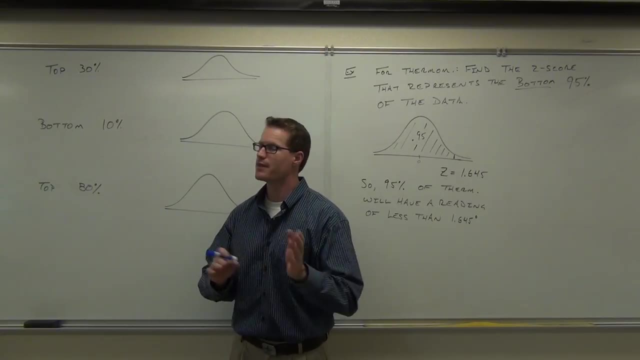 Are you ready for it? Yeah, Okay, watch on the board. You're with me. If you talk about the top 30%, honestly, the best thing you can do is locate the top 50% and the bottom 50% first and then work from there. 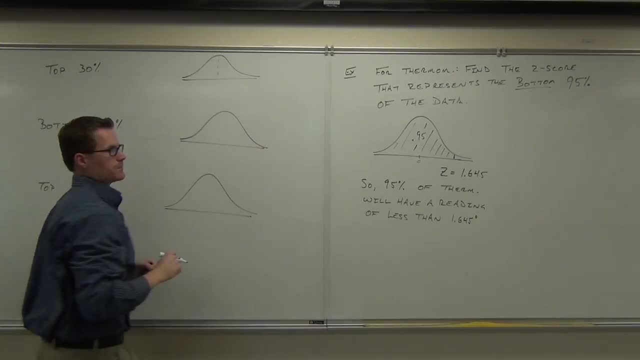 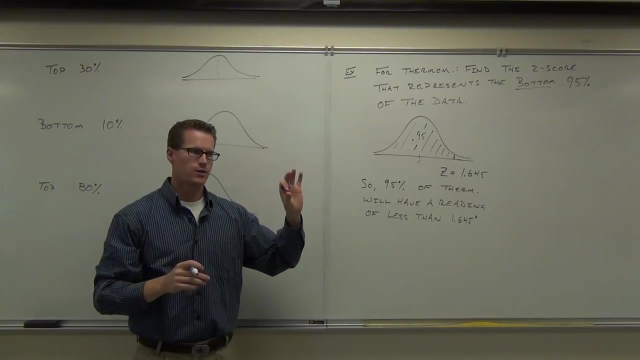 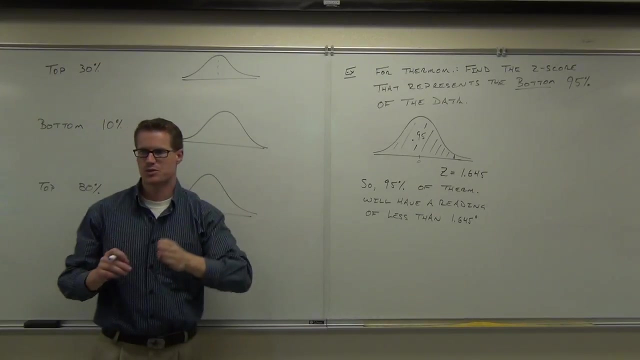 So the 50% range that's right in the middle. This separates your bottom 50% and your top 50%. You with me on that. What we want to do? listen carefully. we want to find the number that separates the top 30% from the bottom. how much percent? 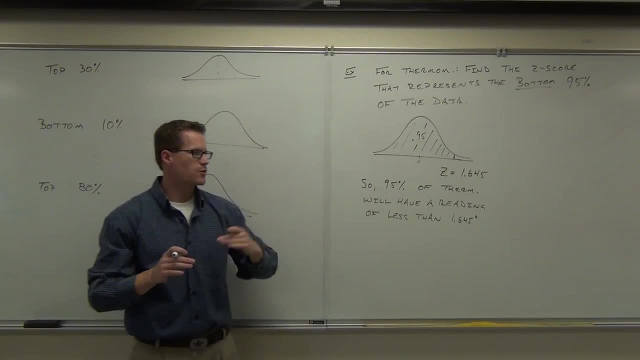 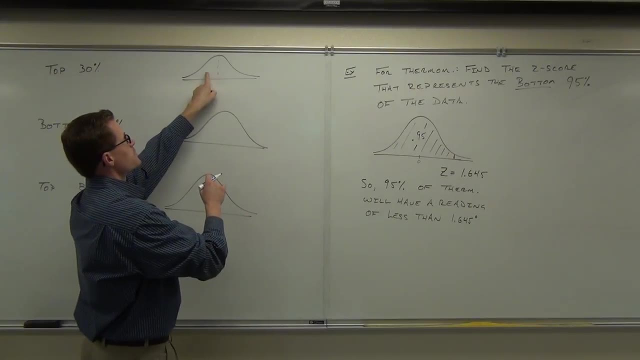 70%. These things have to add to 100%. So asking for the bottom 70% and asking for the top 30% is one and the same thing. If this is the bottom 50% and this is the top 50%. 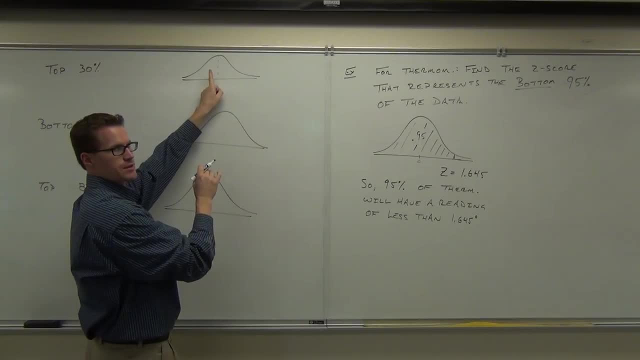 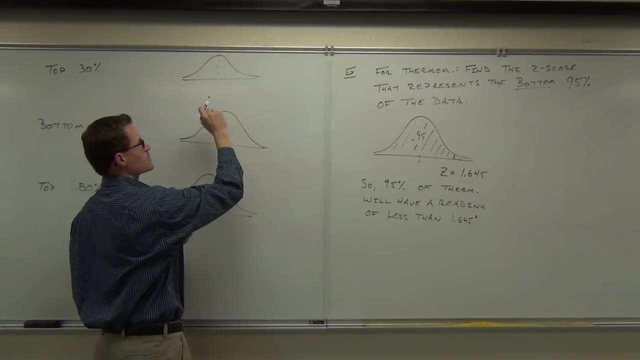 I want to change it to make it the bottom 70% and the top 30%. Are you with me? Where does it have to go? left or right, It has to go. I want the bottom 70%, I want the top 30%. 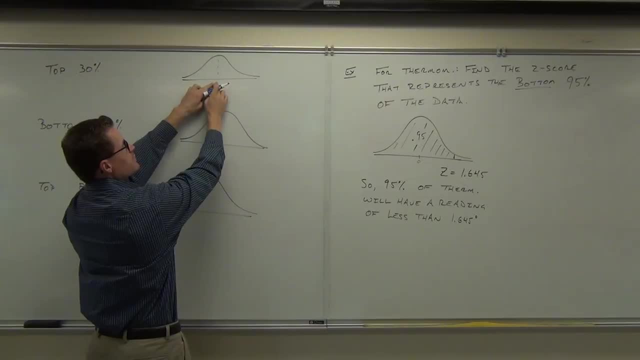 Right now it's 50-50.. If I move it this way, it's going to be the bottom 40%, the bottom 30% and the top 70%. If I move it this way, it's going to be the bottom 60% and the top 40%, the bottom 70% and the top 30%. 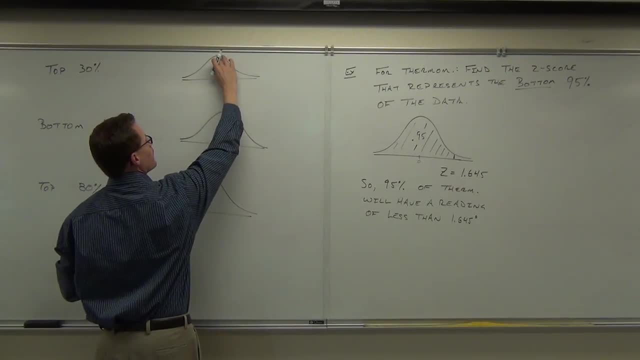 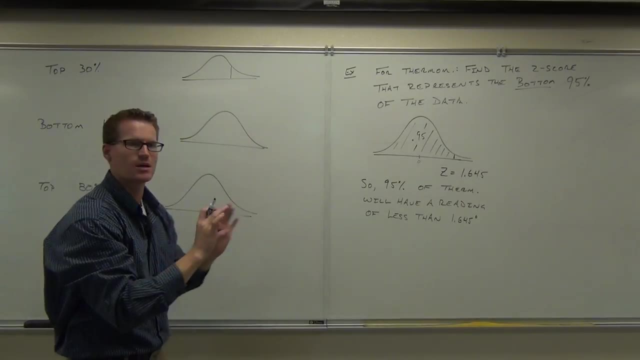 Which one do I want? Let's see Left or right. Right, I want right. So not here, but maybe there. You don't have to be exact, but you do have to draw the picture at least somewhat representative. So this is the top 30%. 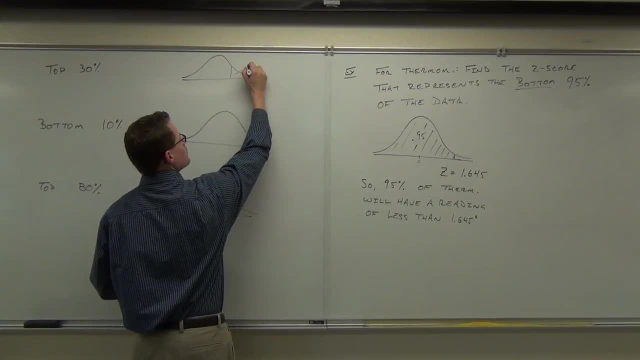 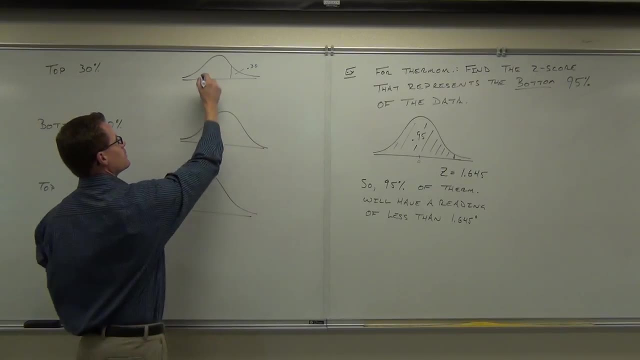 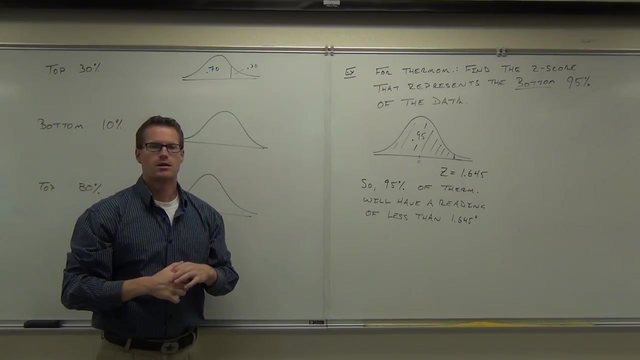 Does that make sense? this top 30%, This would be like 0.30,. yeah, How much would this be 0.70.. Okay, You all right so far, Yes. Now the thing is that you're not done. 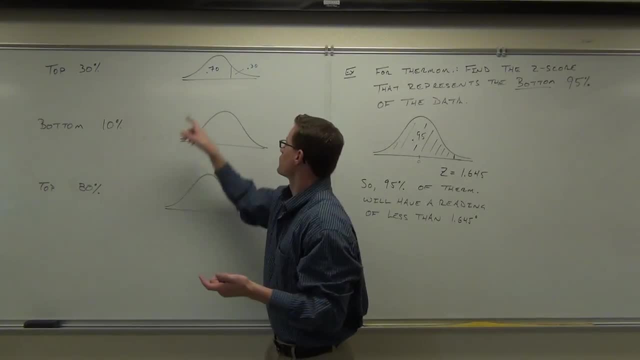 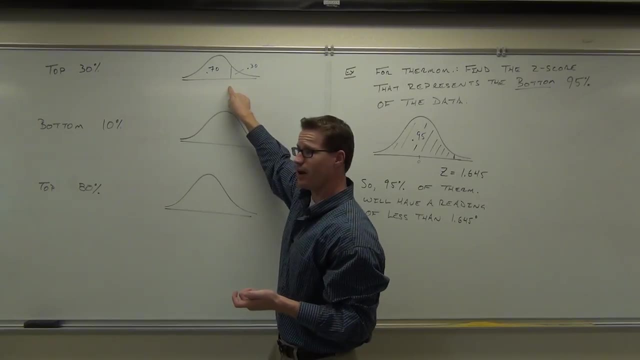 Right now you have areas on the board. Now, clearly, you're looking for the top 30%. However, all you really care about is finding that value right. You don't care really what shade it to be honest, You really don't. 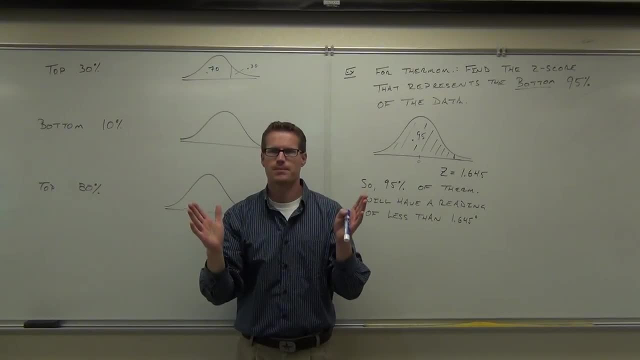 You're just trying to find the value that separates those two areas On your table. if I look up 0.30,, am I going to get the right thing? No, Why not? It's because it only does 0.70.. 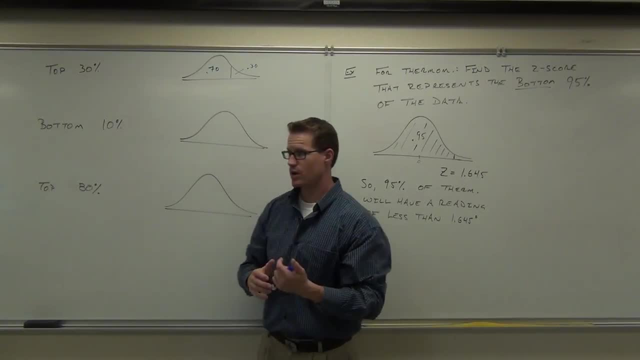 It only does areas to the left. So if I look up 0.30, you know what I would have. I'd have the bottom 30%, not the top 30%. So when you draw your picture, draw both sides of it. 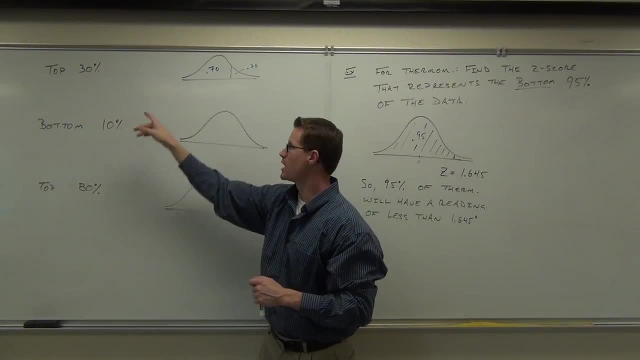 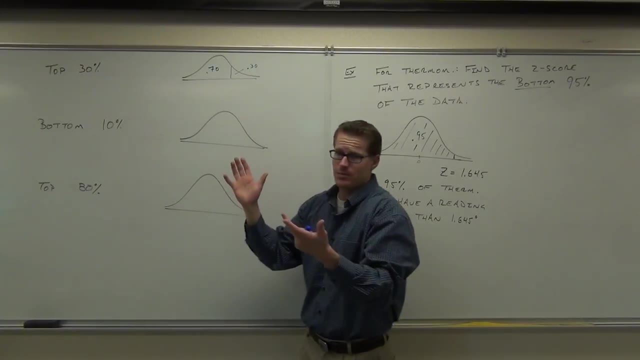 Draw both sides of it and just look at the area that's on the left. So the top 30%. you need to know that the top 30% is the same thing as the bottom 70%. It's the same, It's identical. 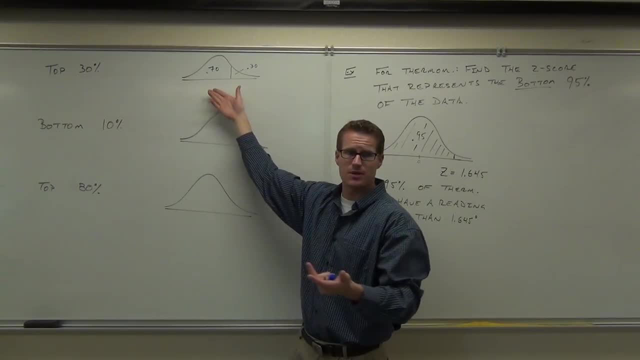 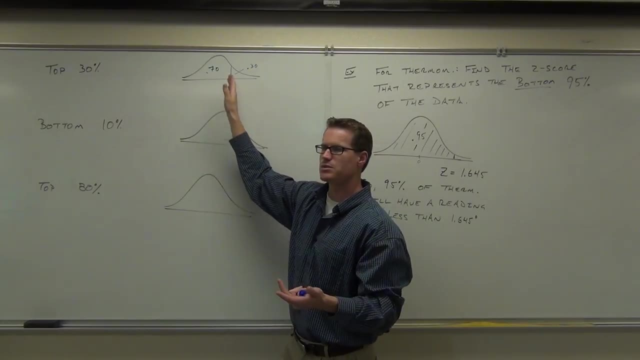 Same picture. If I had asked you for the bottom 70%, wouldn't you have drawn me that picture? I hope so, because it's the same. You just look up not 0.30, that's to the right. Your table only does to the left. 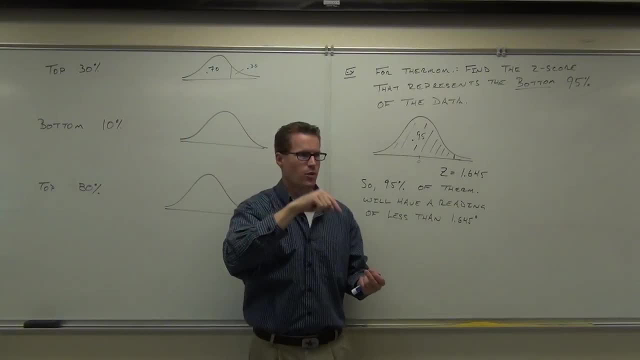 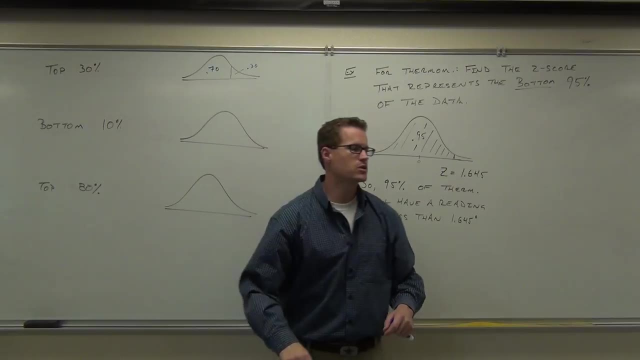 Your calculator only does to the left. If you plug in your calculator 0.30, it's not going to give you the right thing. You have to be smarter than your calculator and the table. So right now, if you have a calculator, do it two ways. 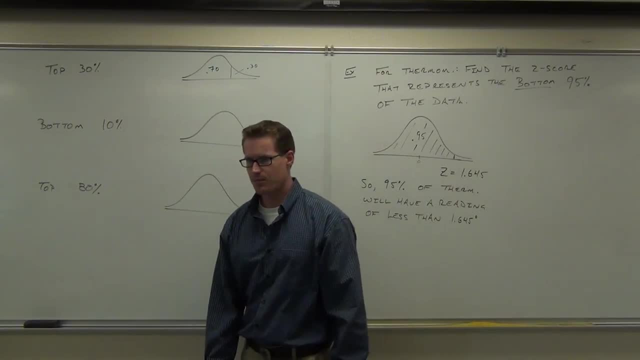 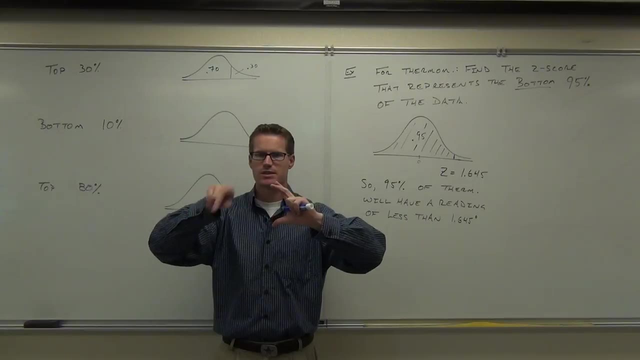 If you just have the table, you only have one way. You're going to go on the table right now and you're going to try to find an area of 0.70.. Should I be looking in the body of my table or the sides of my table? 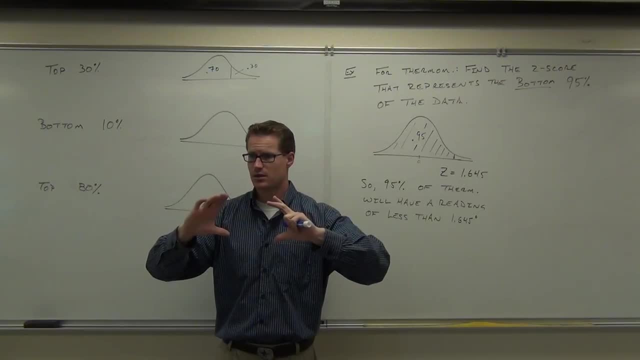 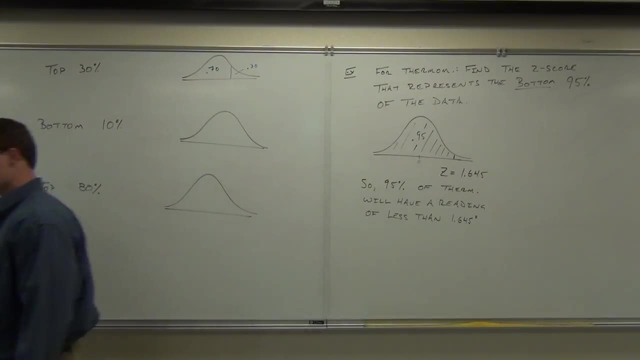 Which one? The area, The area which is the body, or the sides Body? Look up the body. 0.7000.. Most likely it's not going to be there. 0.7000, oh my gosh. 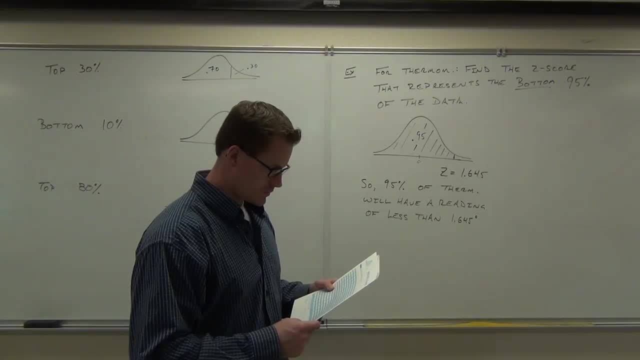 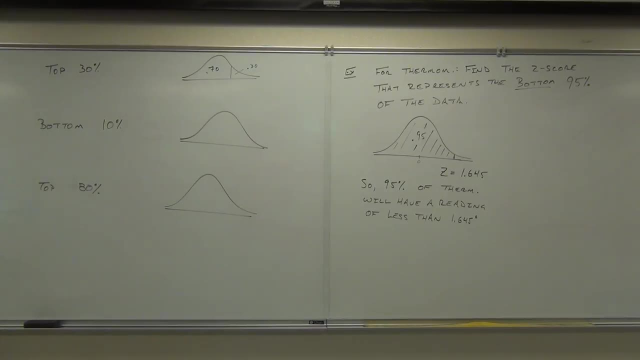 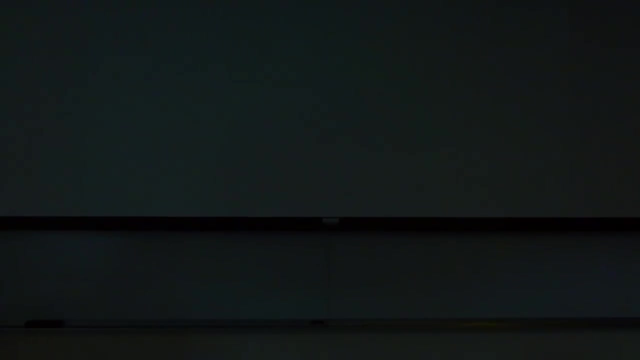 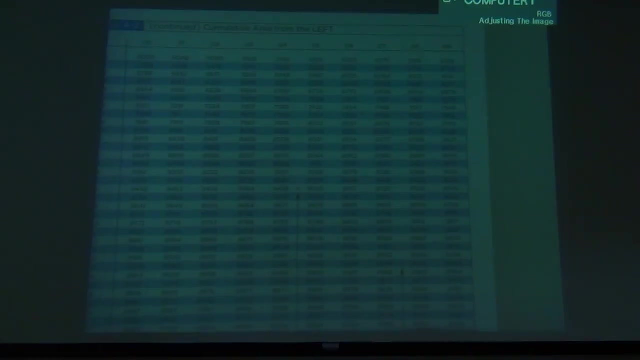 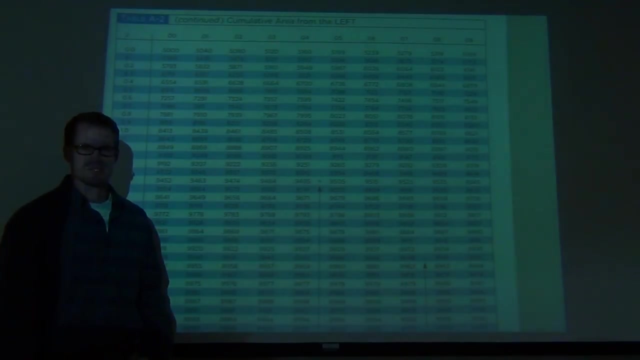 0.7000.. 0.53.. Let's look at that together, okay. Okay, Error. Why do I see a 0.7000?? I do point 7000.. I don't see a point 7000.. 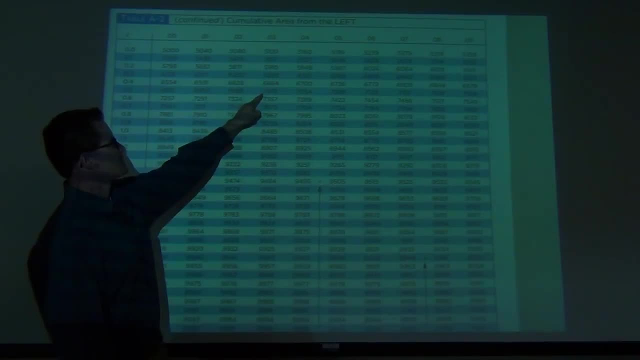 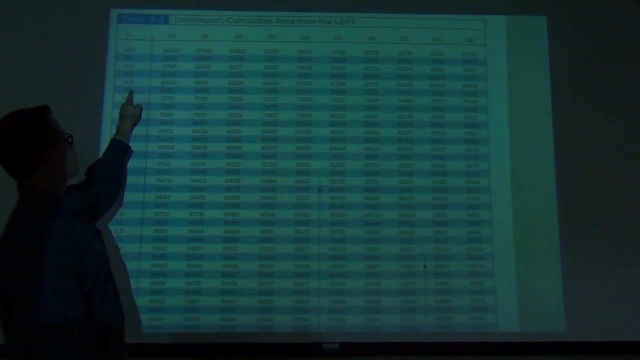 I see a .6985,. I see a .7019.. It's somewhere between there right, Which means your z score is somewhere between .5108.. .6108.. .6109.. .6108.. .6109.. .6109.. 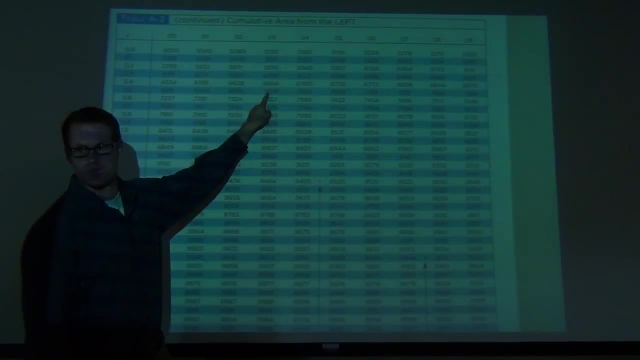 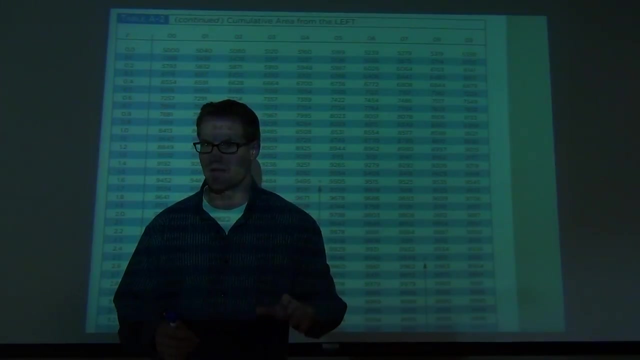 .6109.. .6109.. .6109.. 0.52 and 0.53,. are you following me? Notice how, if you really don't know what you're doing, this can get quite confusing, because you have areas which are all between 0 and 1, right. 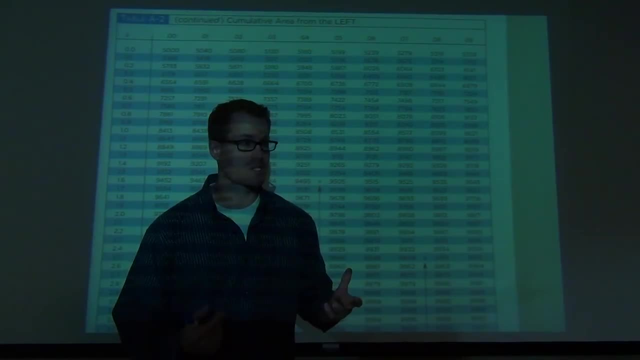 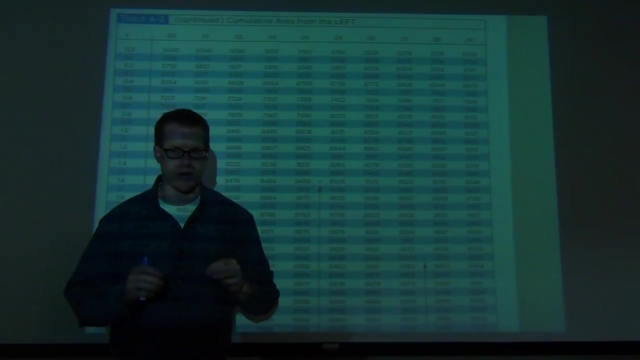 Right And you have z-scores, some of which are between 0 and 1, some z-scores are we're going to get a 0.6- something You have to really know what you're doing here and be aware. 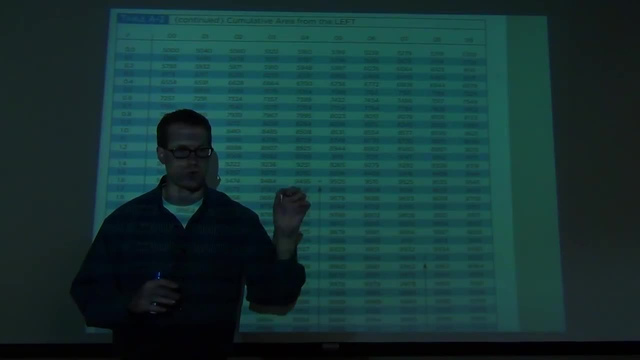 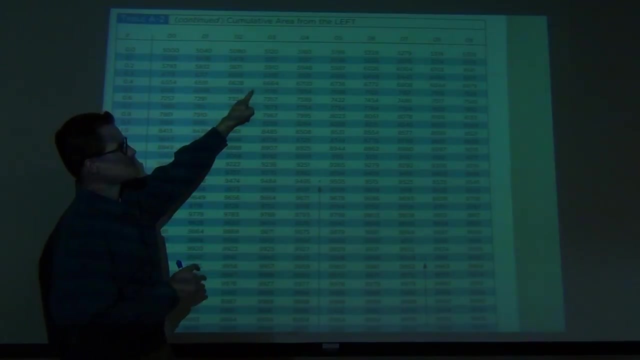 that your z-scores are not areas. your areas are not z-scores. we're going from one to the other. Are you okay with that? You've got to know that stuff. So here we're going. okay, we're looking at the 0.7000. 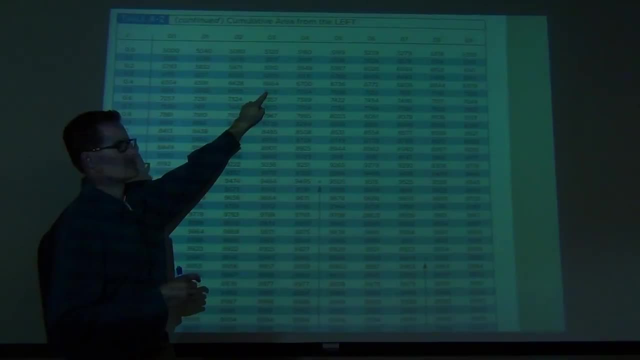 because that's our area. it's not actually there. Here's what we're going to do: Instead of actually averaging things, we're going to go to the one that's closest to. So what's it closest to? the 0.6985 or the 0.7019?? 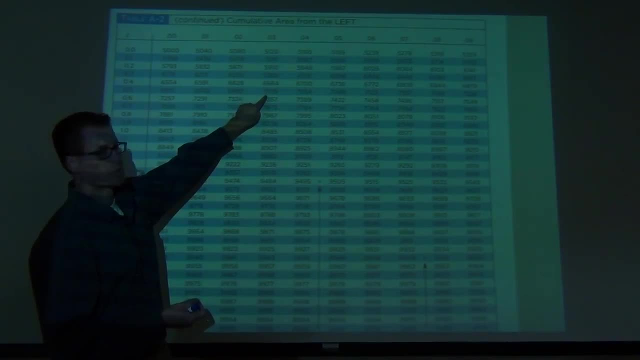 Closest to This one, This one, It's actually that one. This is 15.. This is 19.. This is 19.. This is 19.. 10 thousandths away. this is 19.. 10 thousandths away. this one's actually closer. 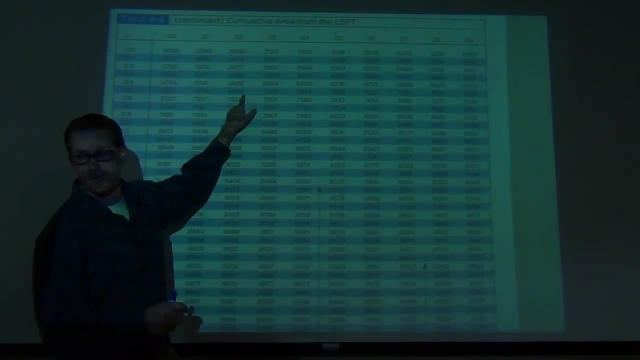 So let's just go with that one. We're going to estimate. this is going to be an approximation for us all, right? So we're going to identify what this z-score is. What is that z-score? again, 0.52.. 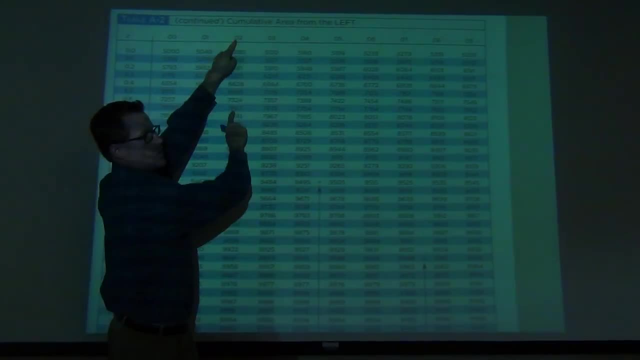 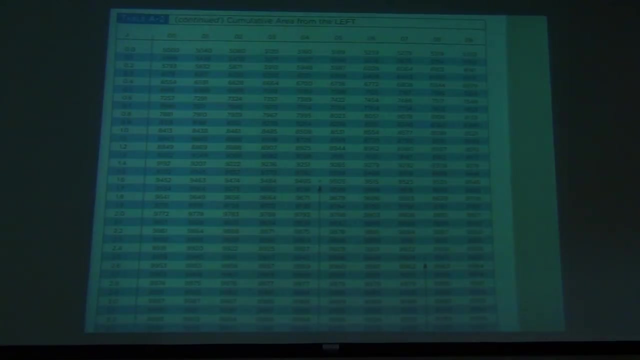 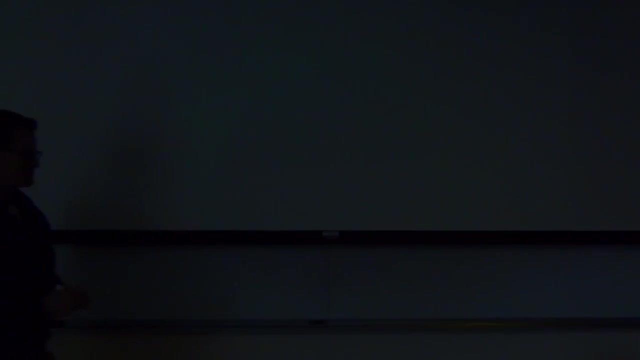 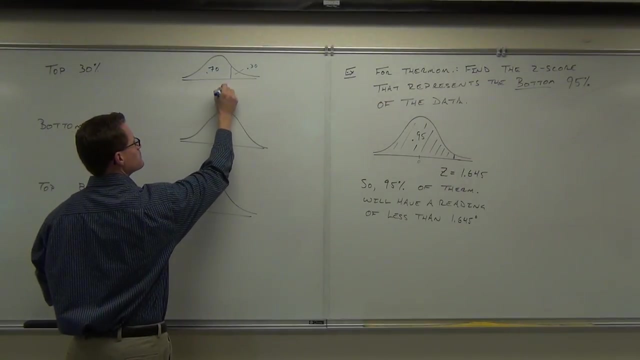 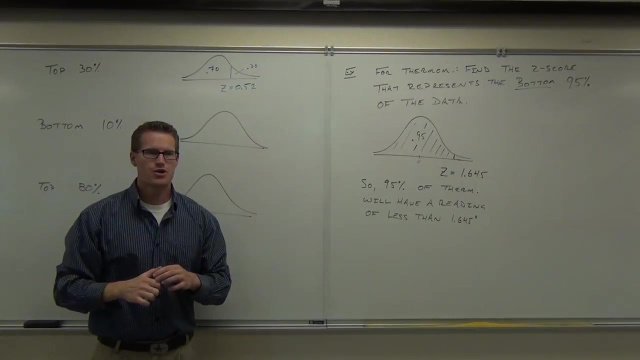 Okay, a 5.5 from here, and then that's the column which is giving me the 0.52, you with me, Look up your calculator. Vanna, On your calculator, are you going to look at 0.3 or 0.7?? 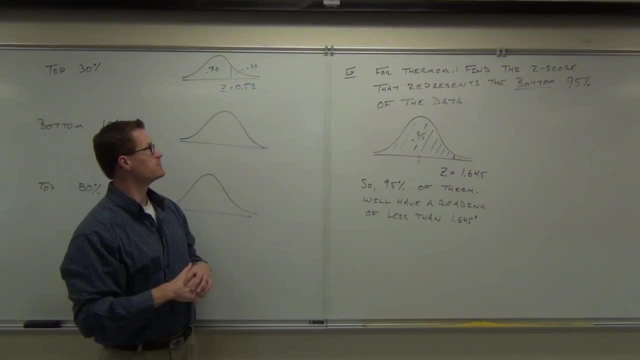 0.7.. Okay, did it give you a 0.52 after you rounded 0.52?? Try looking up. try this for me. Try looking at 0.30.. What 0.30,? try looking at the 0.30.. 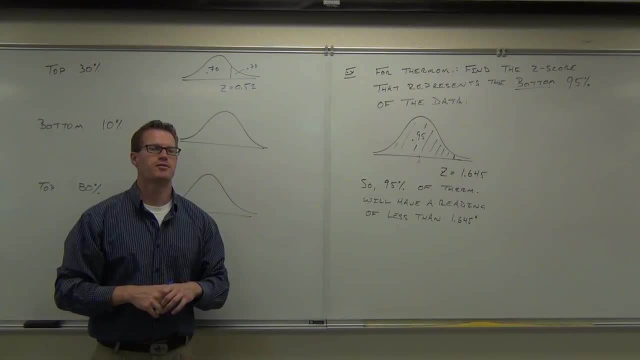 I'll bet you a million dollars. you know what it is right before you say it. I'll bet it's negative 0.52.. It's because I'm a genius. obviously These things are symmetrical, right? The bottom 30% and the top 30% will have the same numbers. 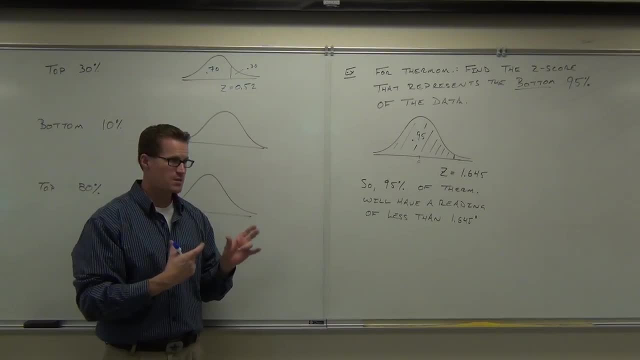 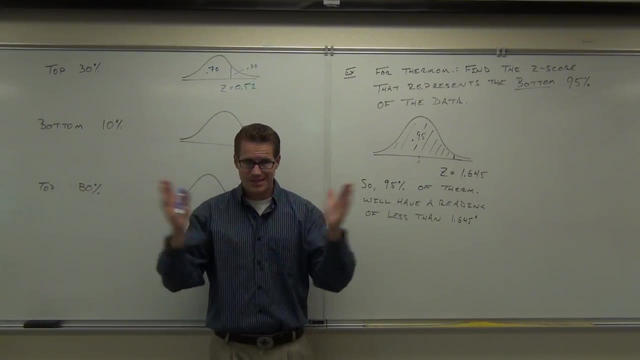 they'll be opposite assigned. The bottom 40% and the top 40% will have the same numbers. they'll be opposite assigned: Bottom 10%. It's symmetrical, right. It's zero in the middle, So the negative and the positive will be the same distance away. 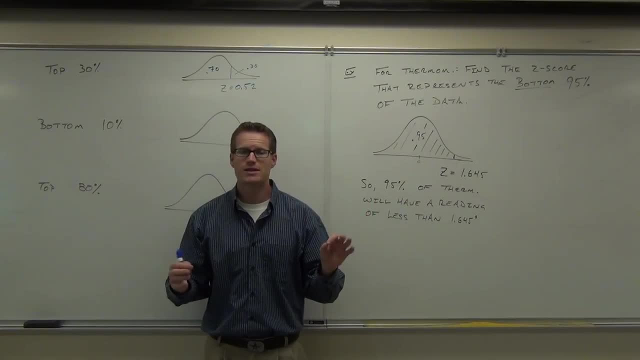 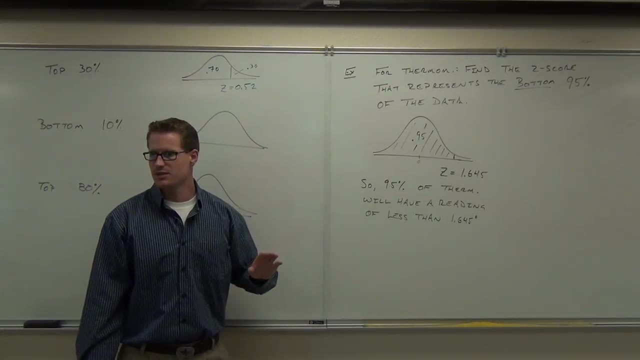 it's just you'll have a different sign. So there are a few ways to actually do this. if you really think about it, You could look at 0.30,. right, Just change the sign if you're on the right side of the zero. 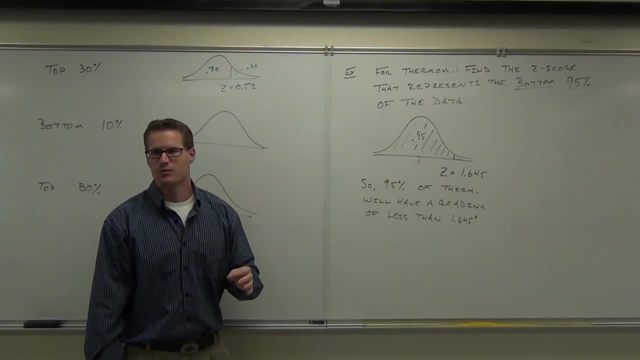 Or if you're on the left hand, then you don't do that. That's a little bit more confusing now, So I would recommend that you draw both of these areas, look at the one on the left all the time, and then you'll always be right. 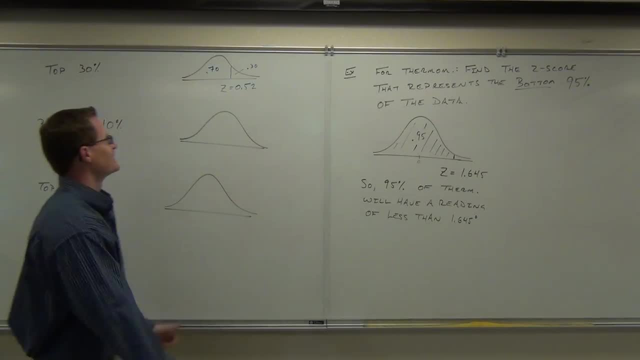 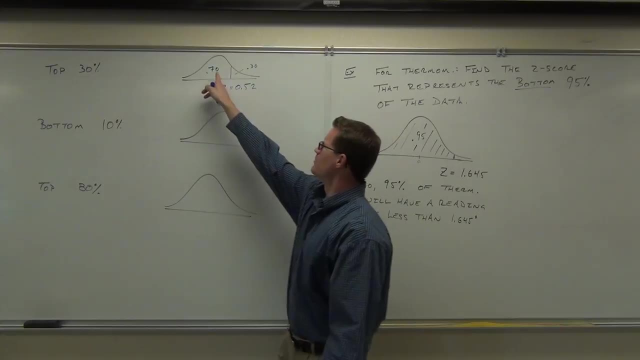 Does that make sense? Okay, good, I do need you to know the interpretation of this, because it is confusing. Wait a second. How is the? The bottom 70% and the top 30% 52%. that's not a percentage. 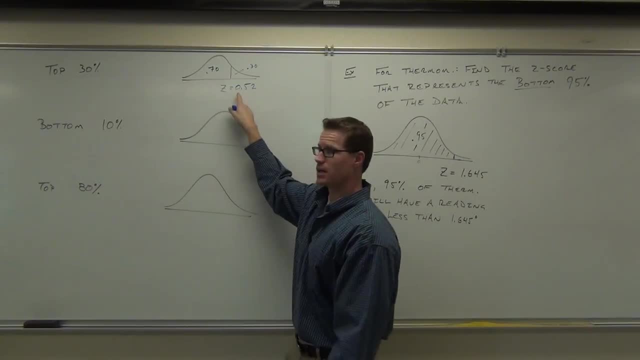 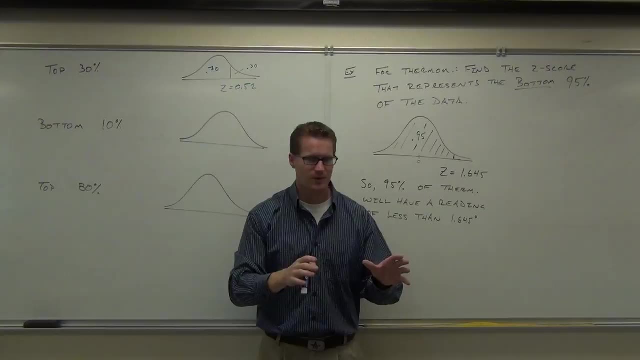 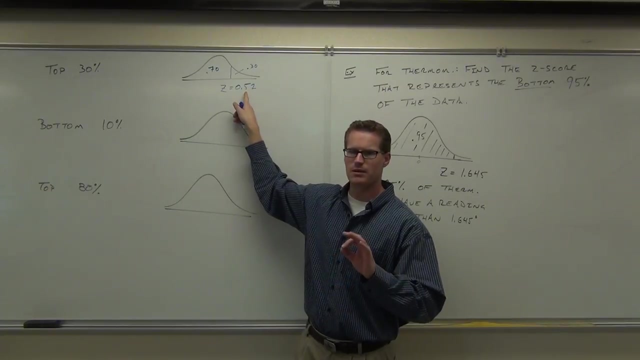 What is that? This is an area, this is a z-score, or a distance from zero. This is what this says. folks, You need to know this part. When I say that, you better know this part. What a z-score is is the number of standard deviations away from the mean. 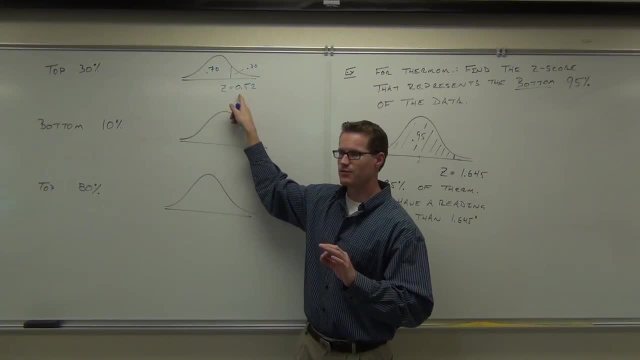 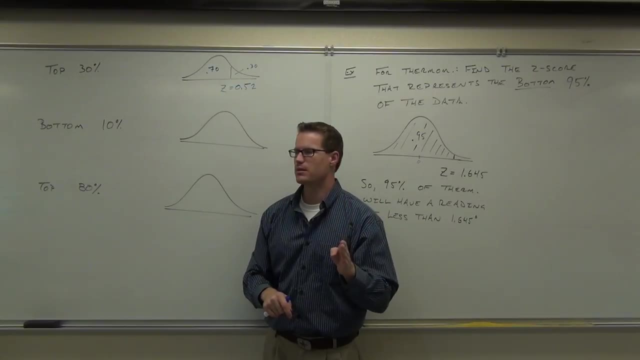 Do you remember talking about that? The mean is zero. This is the distance away from the mean according to the standard deviations. What it says is it's zero. It says it's just over half of a standard deviation away from that mean. That's how much it's going to represent an area of 70% below it. 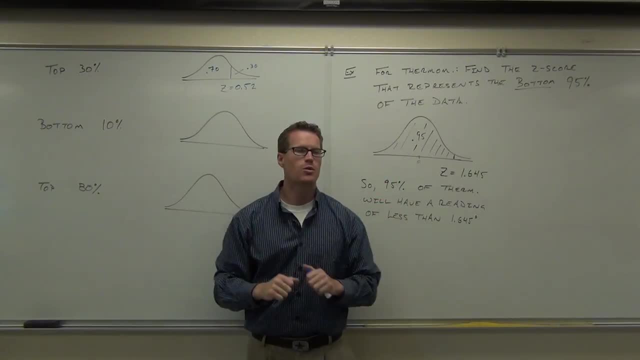 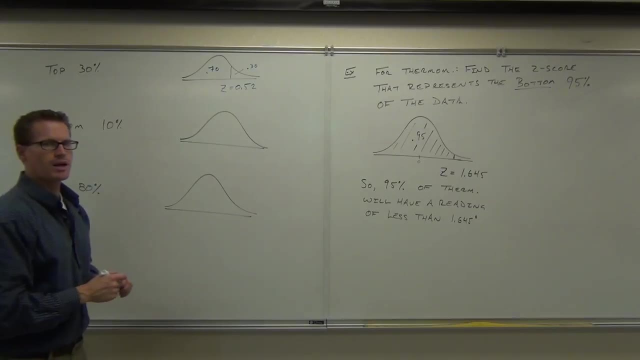 That's what that's interpreted as. Are you with me? Let's draw more pictures? We're not actually going to look these up because hopefully this one does it for you. yeah, Okay, let's do the bottom 10%. Tell me when I need to stop for the bottom 10%. 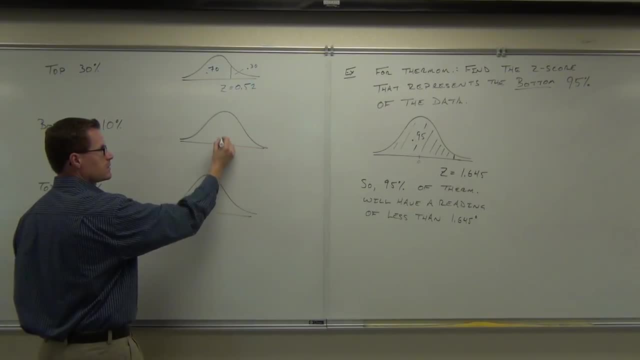 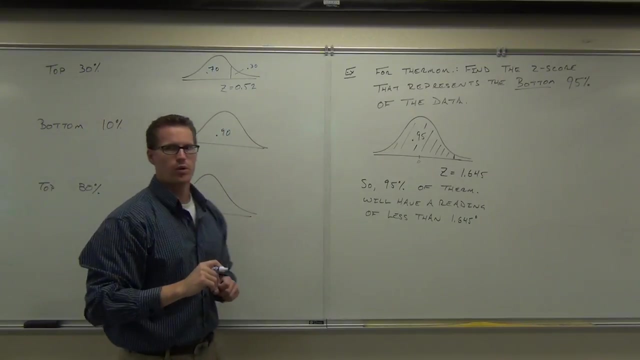 Here, Bottom 10%. This would be the Right there. Sure, Bottom 10%. this would be .10.. How much would this be On your table? would you look at .10 or .90? .10.. 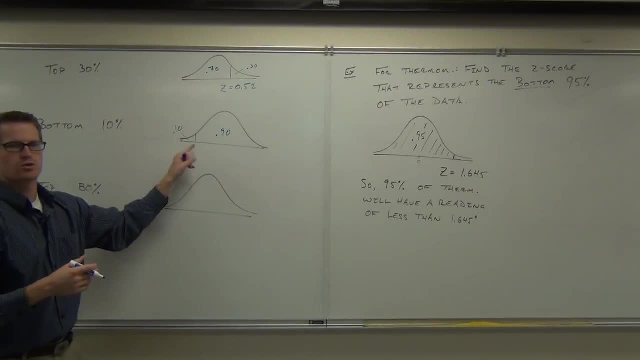 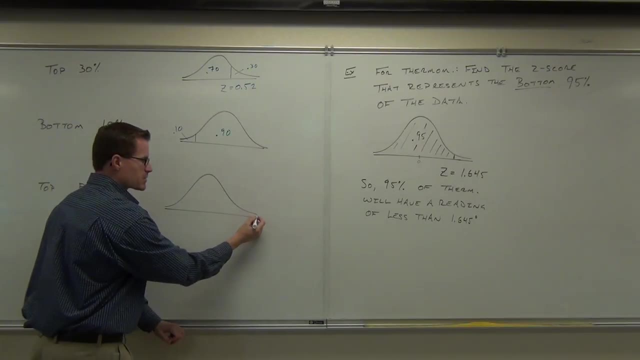 .10, the area to the left. That's going to give you the value. Remember, you're not finding another area, You're a kid in an area. You're finding the distance. now, Top 80%. tell me where I stopped, top 80%. 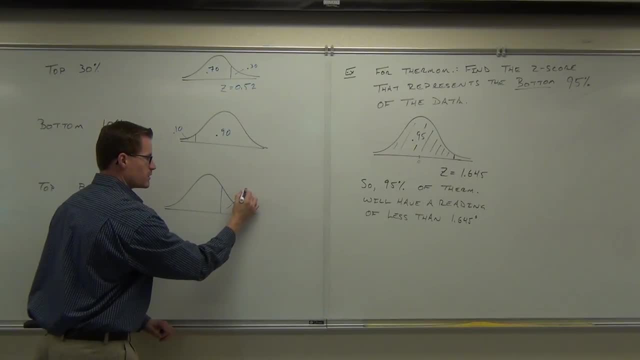 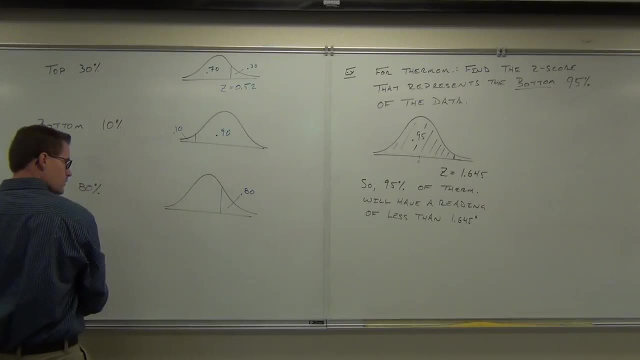 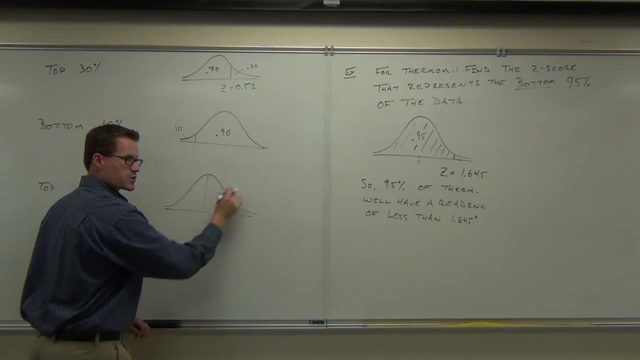 Here, Stop Top. You're saying this is 80%. That's what you just said. here, Stop Top 80%. This is the top 50%. I want more or less in my top More. This would be less. 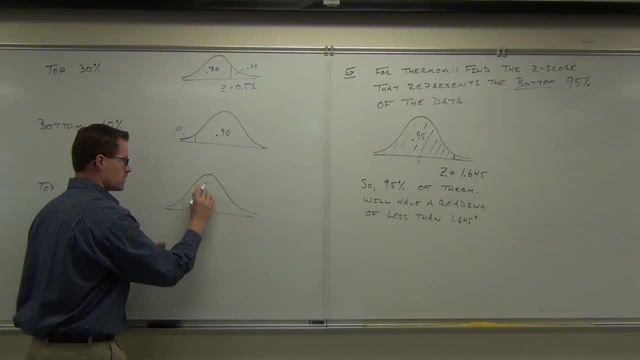 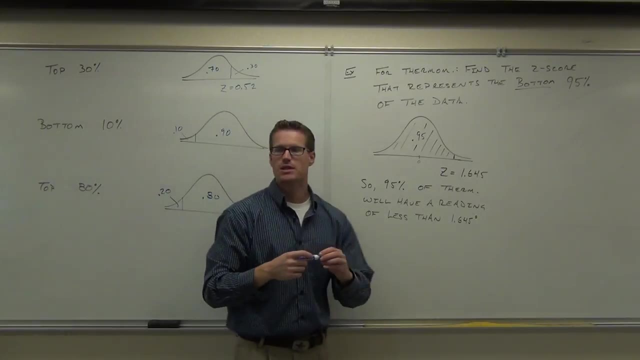 I want more. That's the top 80%, This is the bottom 20%. Bottom 20%, top 80%. same thing, same thing. Which would you look up here? .20 or .80? .20.. Clearly it's on the left. 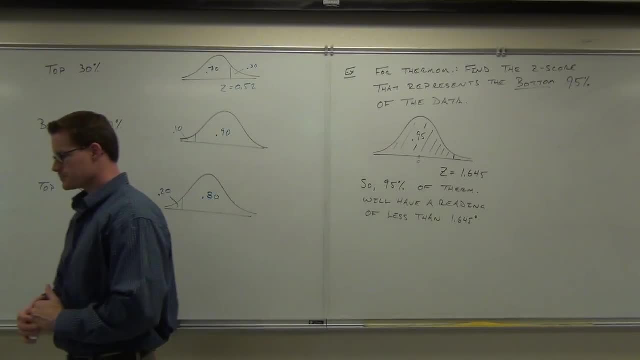 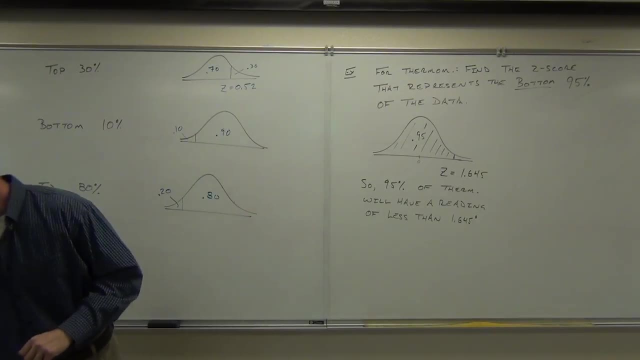 That's how you go from an area to a z-score. Feel all right with that. Yes, sir, Yes, One more example that we'll do. 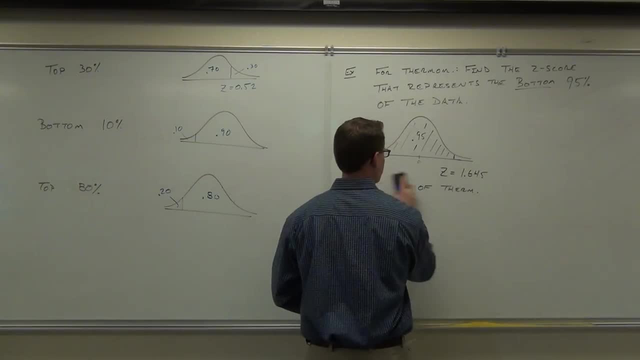 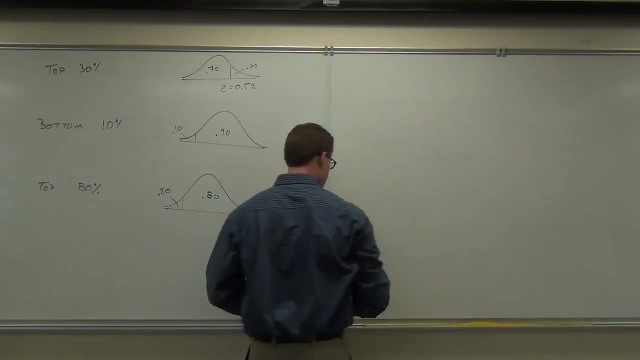 You know, oftentimes this company would probably not really want to know that it's strictly more than a certain reading or strictly less than. 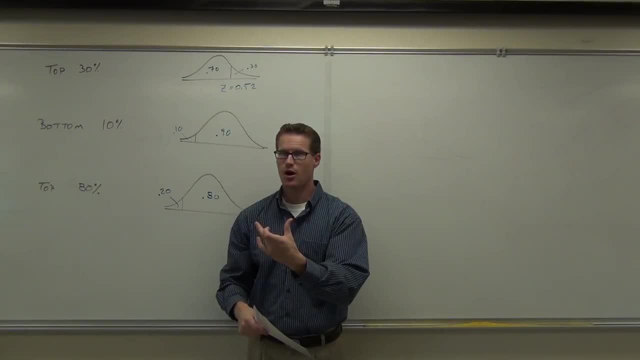 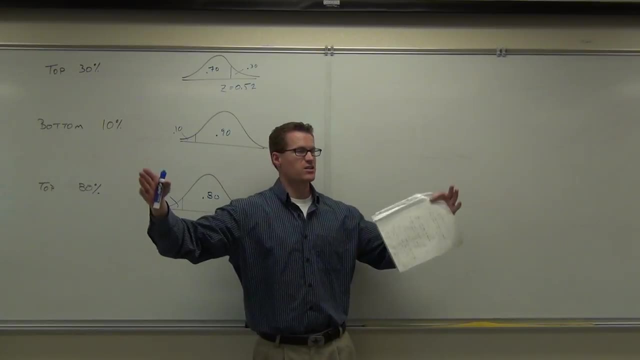 but probably between, because you don't want a thermometer. that's just always less than something right, Because you could be way way off. It just gives you a reading that's less than what it should be. We want something that binds it. 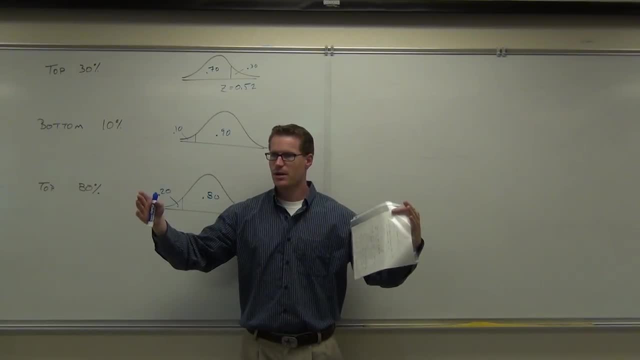 It says: okay, I know, like I'm 95% certain, that if I give you a thermometer it's going to read between this range. Don't you want to know that It's not going to be too high, It's not going to be too low? 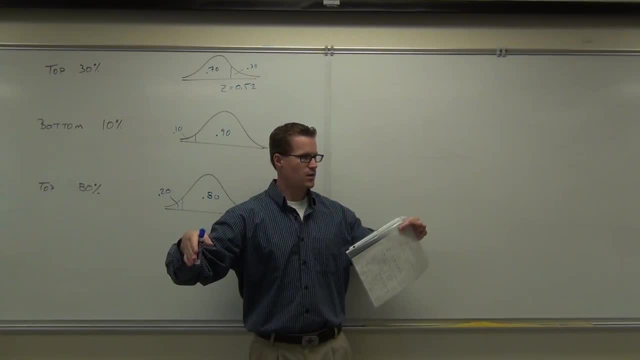 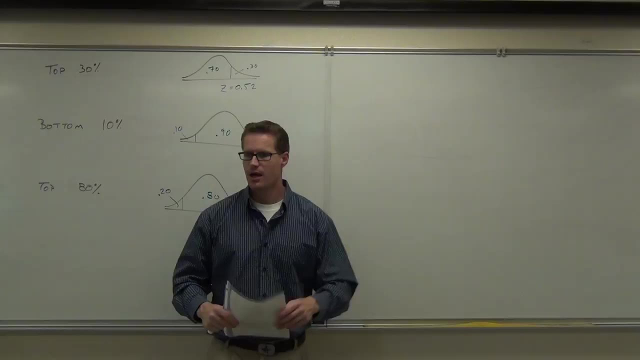 It's not going to be too low. It's going to be within this range, You with me. So what we're going to do is we're going to find the Z scores that give an area between the bottom 2.5% and the top 2.5%. 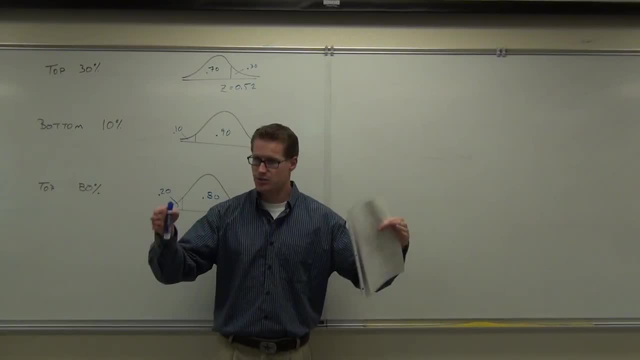 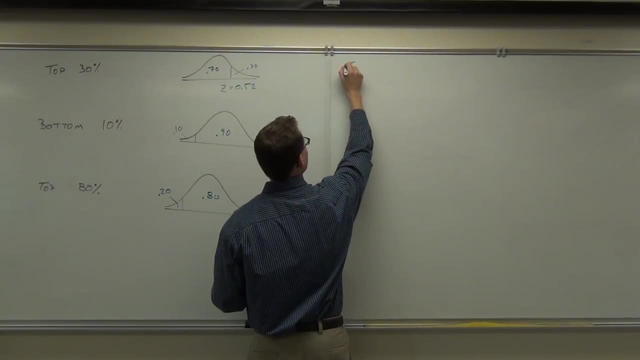 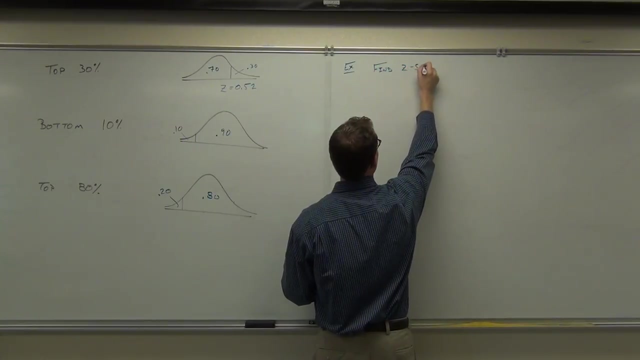 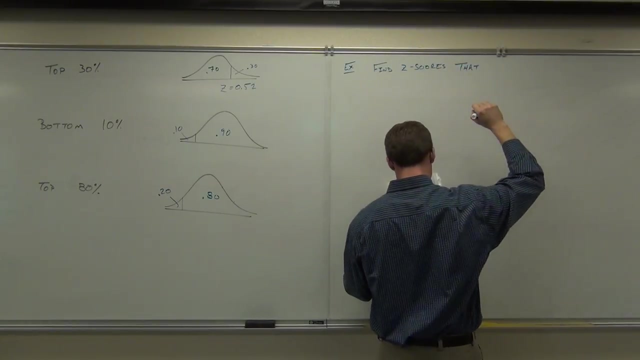 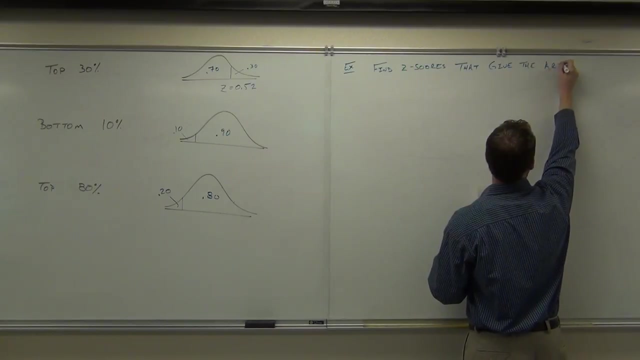 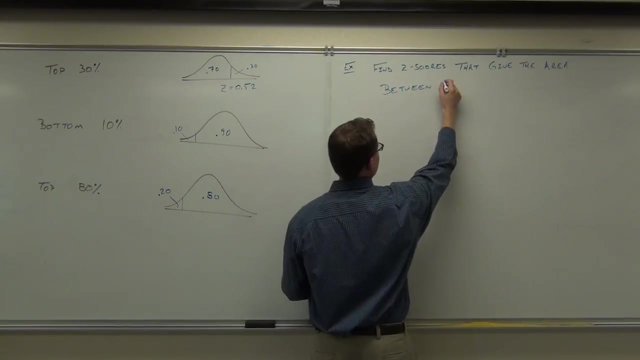 We want to bind it and say it's going to be between these numbers. That's what you're. we're 95 or 99 or whatever percent, certain that it's between these numbers. So find the Z scores That give the area between the top 2.5% and the top 2.5%. 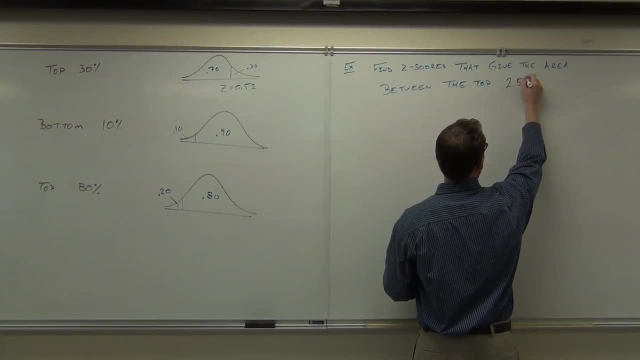 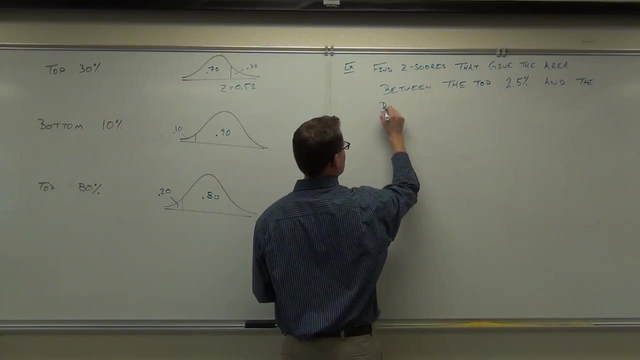 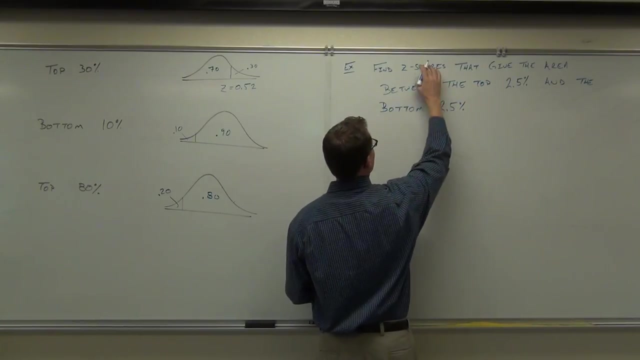 2.5%, The bottom 2.5%. Well, you know what? We're still going to have a picture. All these things are going to have exactly the same picture. You just need to know how to interpret the problem correctly. 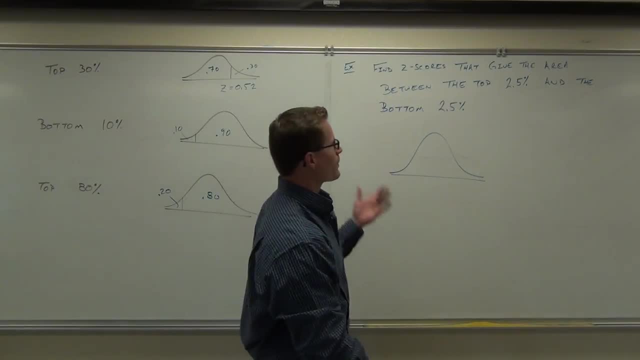 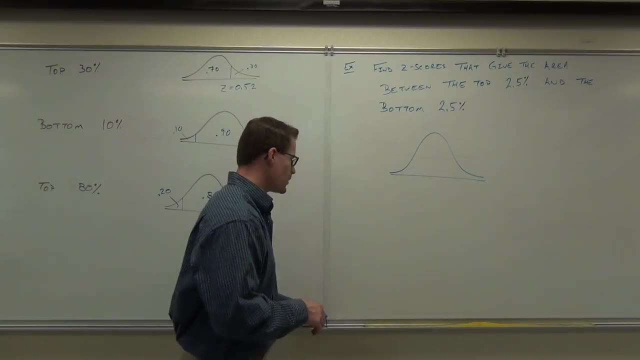 Okay, we don't want the z-scores to give the area between the top 2.5% and the bottom 2.5%. Let's identify where those things are first. So let's work on how about the top 2.5%? 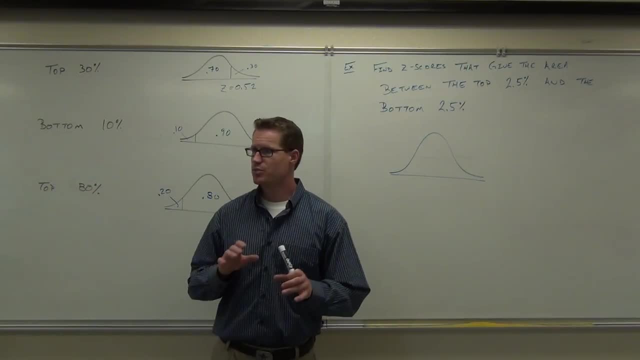 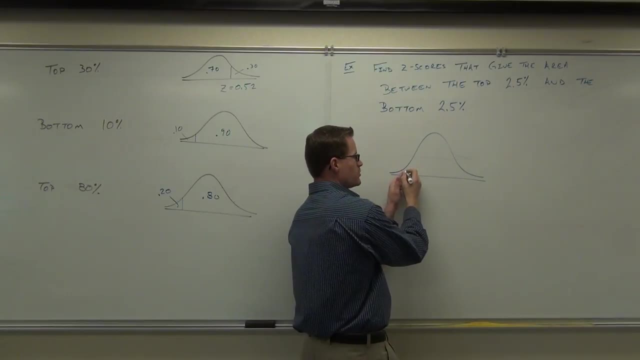 Tell me where I need to stop if I want to represent the top 2.5%. Start this way: The top 2.5%, Top Right here. Yeah, That's the top 2.5%, Yeah, No. 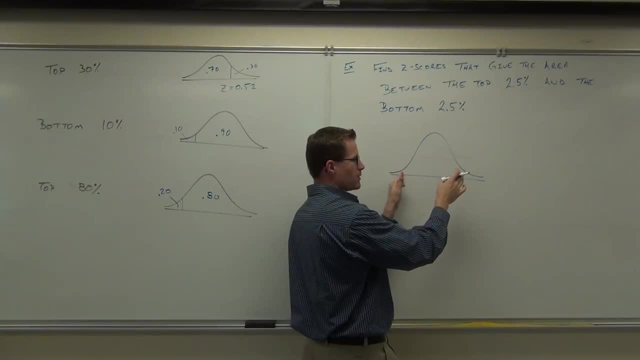 How much is above that line? Way more than 2.5.. I don't want to stop there. If I'm looking for the top 2.5%, this would be the top 50. This would be the top, maybe 30.. 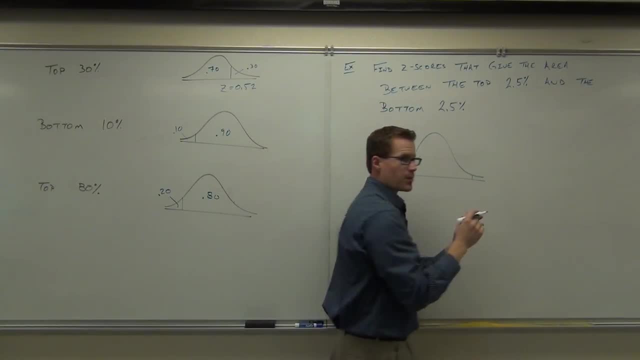 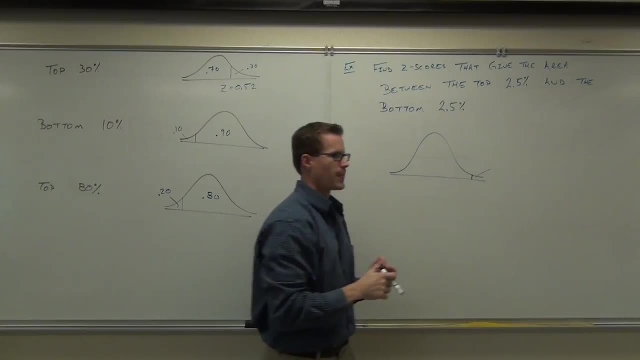 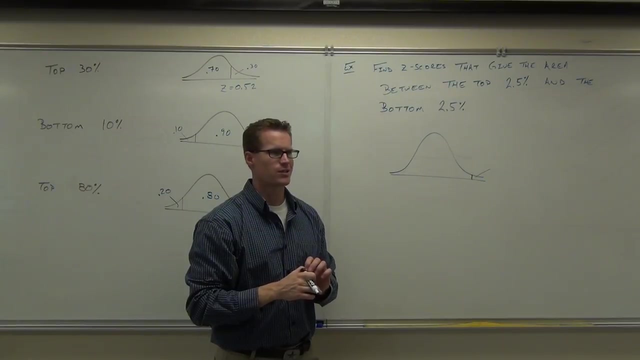 This would be like the top 10.. The top, The top is the one she left. The top. 2.5%. That's like right here, Oh, 2.5.. 2.5%, 2.5%. We don't deal in percentages, do we? 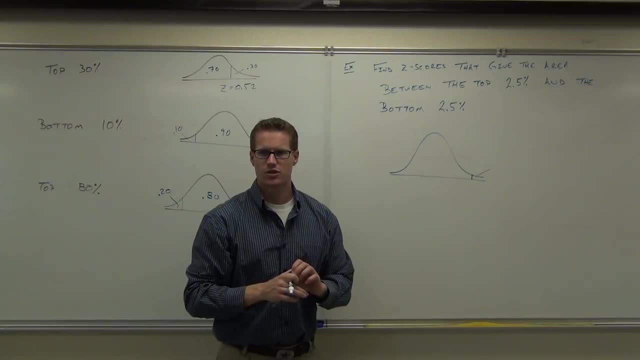 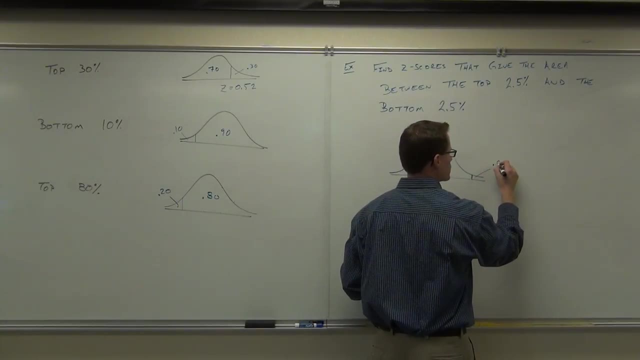 Your table's not in percentages, They're in percentages, They're in proportions. Change that to a proportion Point what: 0.25.. 0.25.. Yes, Move it twice The decimal. I'm talking about 0.025.. 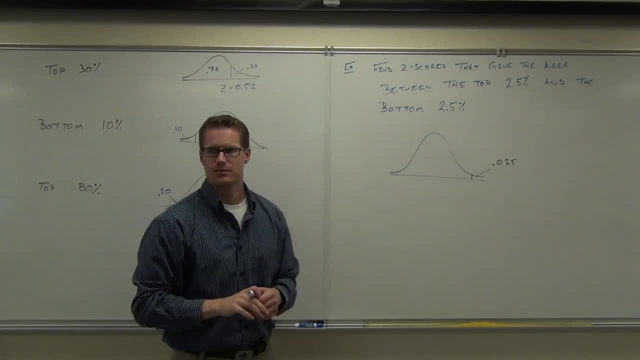 0.025.. Okie dokie, Okie dokie. Now let's find the bottom 2.5%. Tell me where I need to stop, Stop, Stop. That's the other one. It should be about symmetrical. 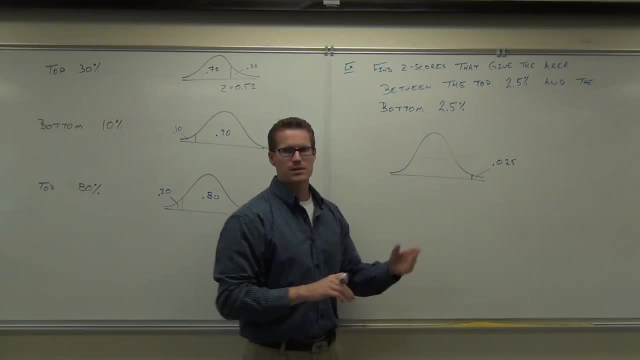 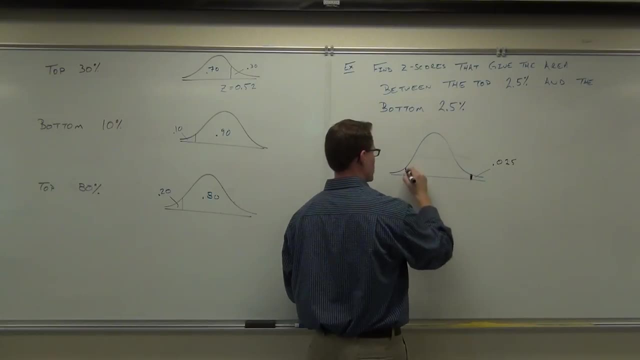 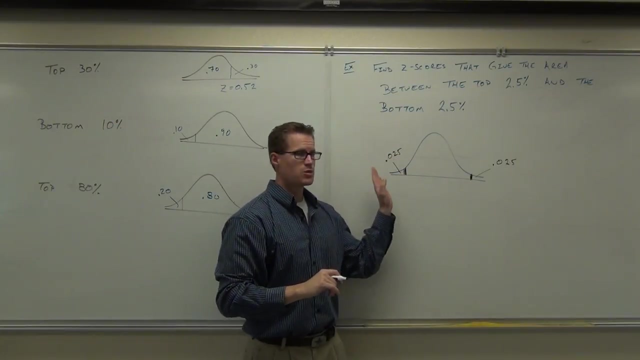 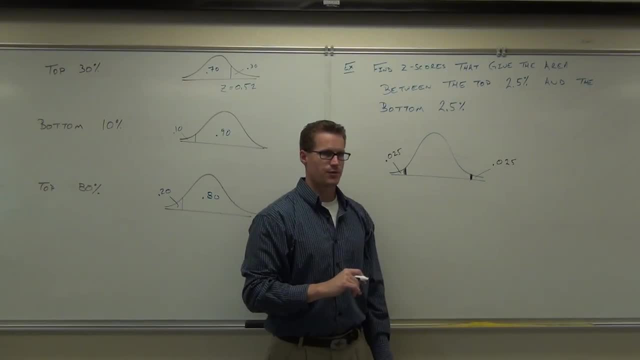 And what we're looking for is the area in the middle of that stuff. Yeah, Alright. Well, you know what We've got to find? both these z-scores. This is like two questions in one, Two questions in one. This one's going to be pretty easy to find. 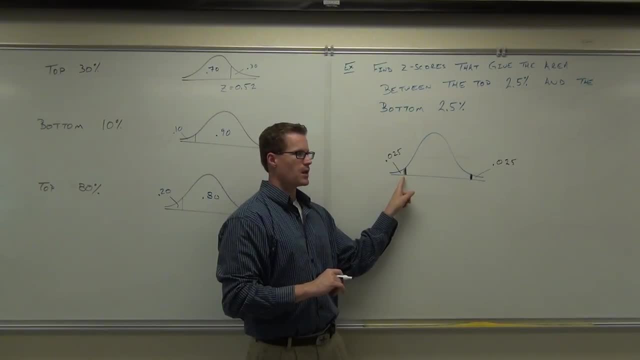 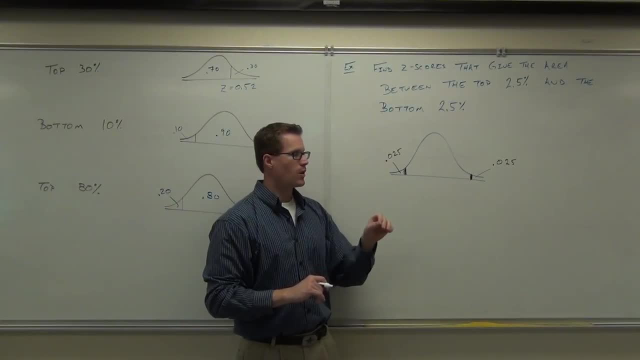 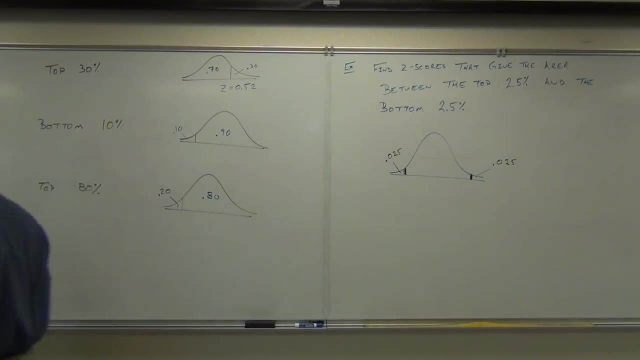 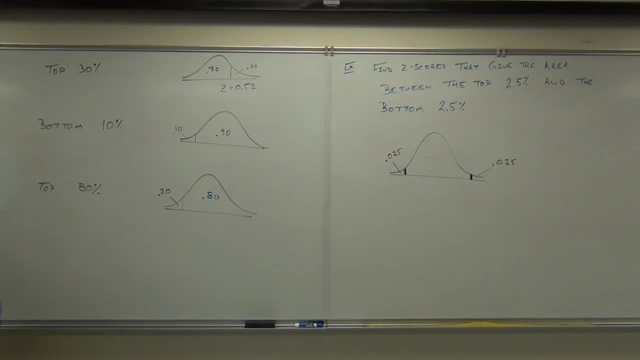 Negative, Definitely negative. I mean, it's not even listed on the positive right. If you notice this, hey, the positive z-scores start at 0.50.. Why is that? Because that's in the middle. Everything to that side would have an area greater than 0.50.. 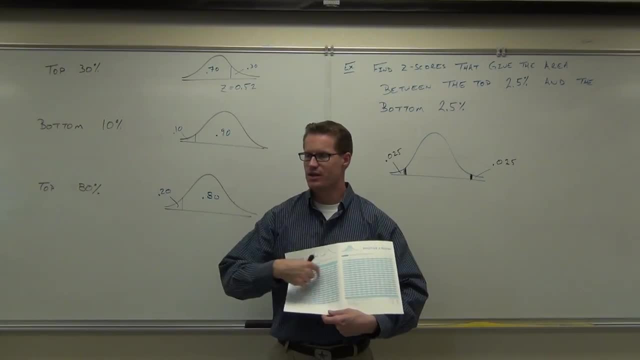 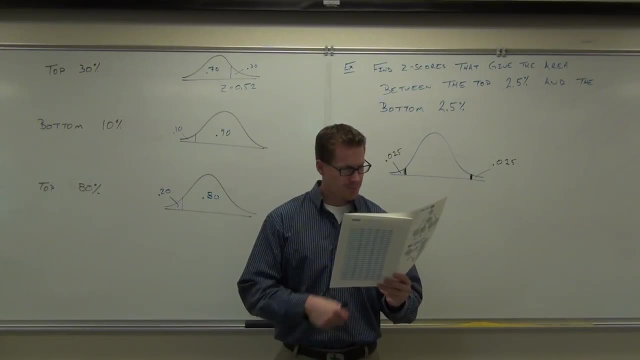 That's a positive z-score. These are all your negative z-scores that have areas less than 0.50.. So we have 0.025.. Hey, that one's exactly there, Did you find it? Yeah, That's kind of nice. 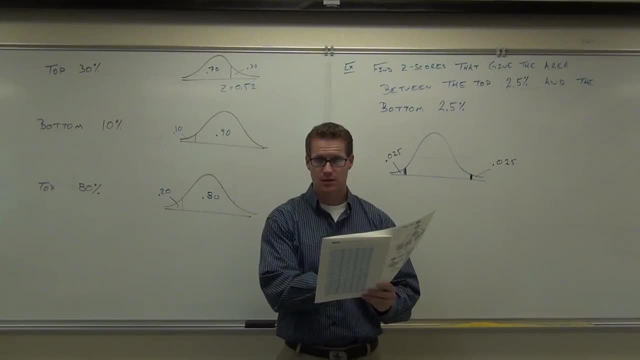 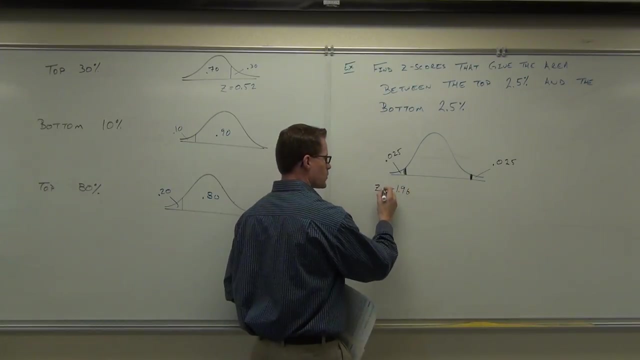 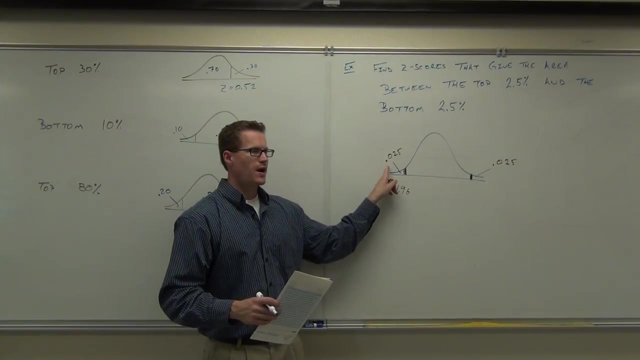 You got negative 1.96.. Did you find negative 1.96?? Everybody, Yes. So this is negative. Z-score is negative 1.96.. What this says is that 2.5% of your thermometers will have a reading of less than negative. 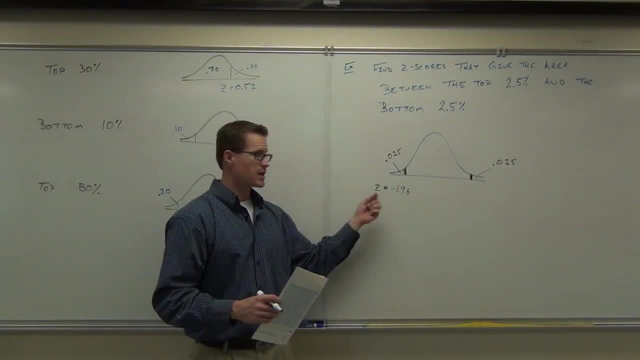 1.96 degrees when dumped in ice water, Just because right now, a z-score is the thermometer reading and a thermometer reading is a z-score for this one case. Follow. Now the question is: how in the world do I find this one? 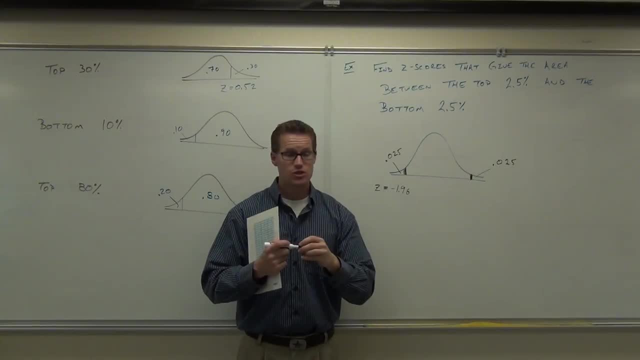 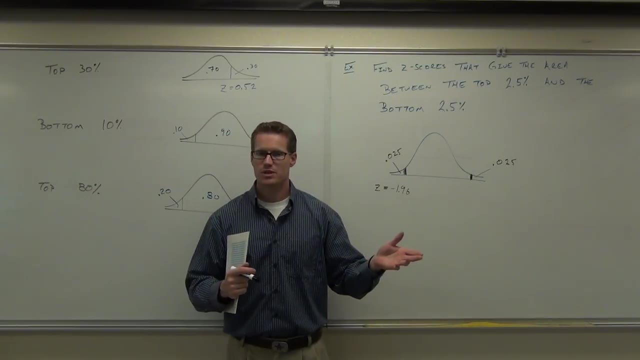 It's going to be a positive one. Well, wait a second. There's two ways. There's actually two methods. You can either look up the table and you kind of think about what the shape of this is, or you have to look something up. 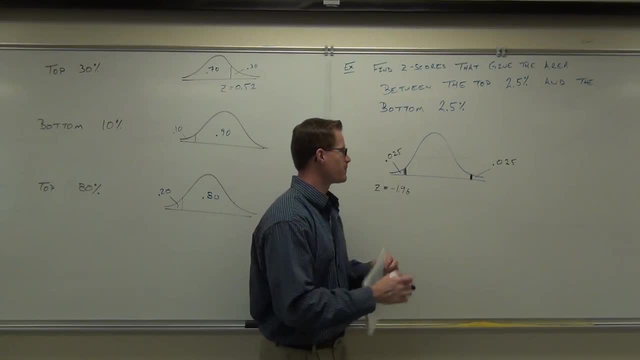 Let's do the look something up first. If I had to look something up, what would I look up? How much would I look up? What's the area to the left of this point? 0.97.. How'd you get that? 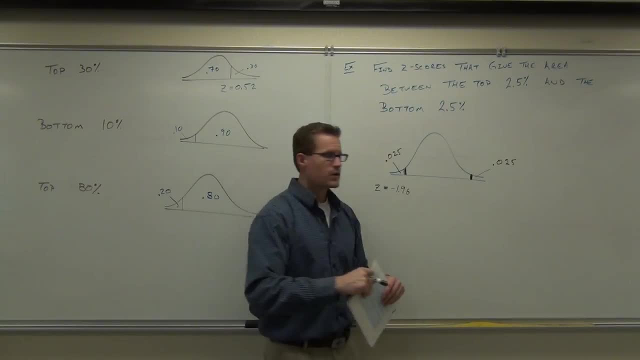 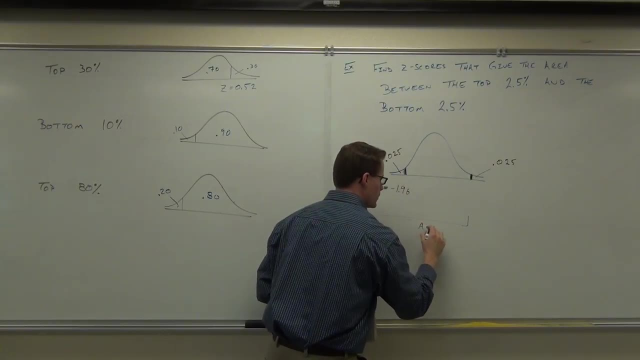 I took 0.025 minus 1.. OK, So if this whole thing's equal to 1,, then the area to the left of this one, the area, would be 1 minus that, or 0.0,- I'm sorry, 0.9,. what was it again? 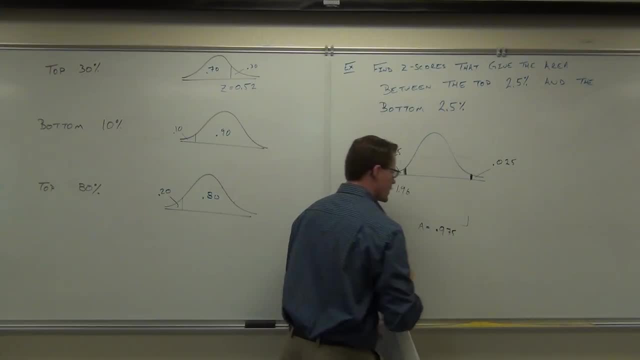 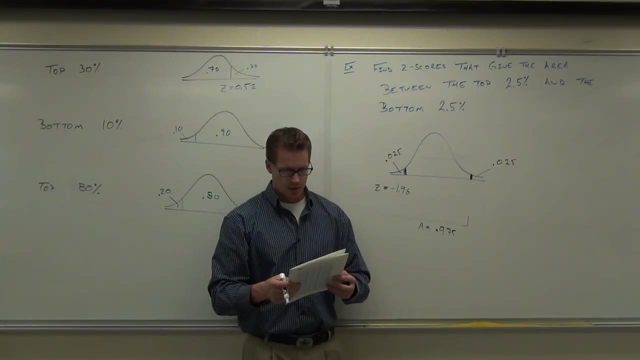 0.975.. OK, 0.975.. If you look up 0.975 on your table, do that or use your calculator if you'd like. I just want to verify this with you. Look up 0.975 on the area portion of your table. 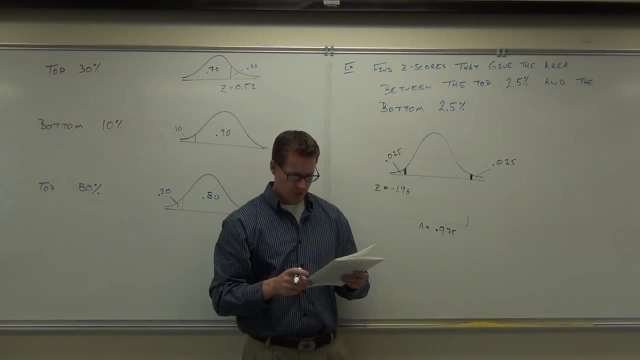 Now we're going to be in positive z-scores. now we're to the right of the mean. If you look it up, what do you think you're going to get? 0.975. Positive. Is that a coincidence? It's magic. 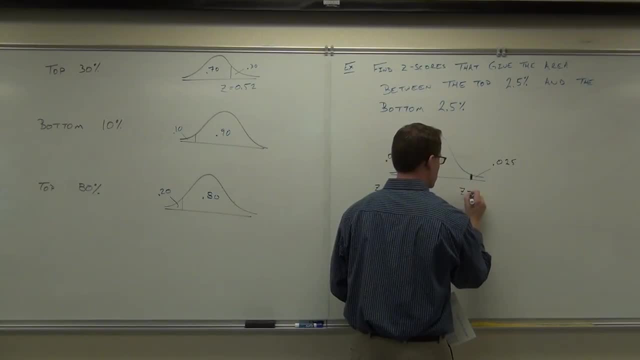 It's magic. It's magic, Clearly magic. I mean that's awesome, Crazy math stuff. I mean ridiculous. This is a symmetrical graph, right? So if I'm looking up the bottom and top of the same exact percentage, your z-scores are: 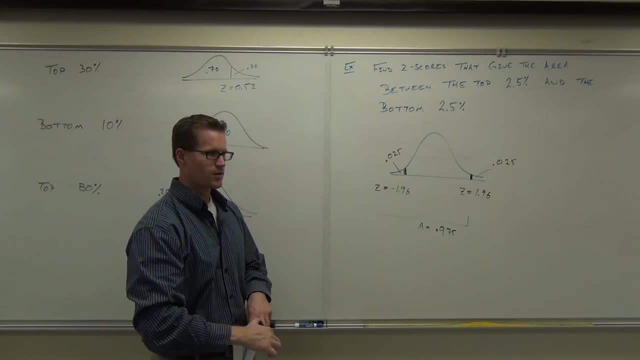 going to be identical, except for the sign in front of them. One's going to be the opposite of the other. So if you're looking at 0.025 and you need- I'm sorry- the bottom, you're going to get 0.975.. 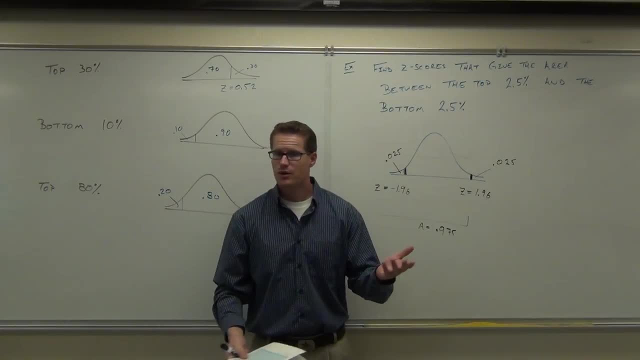 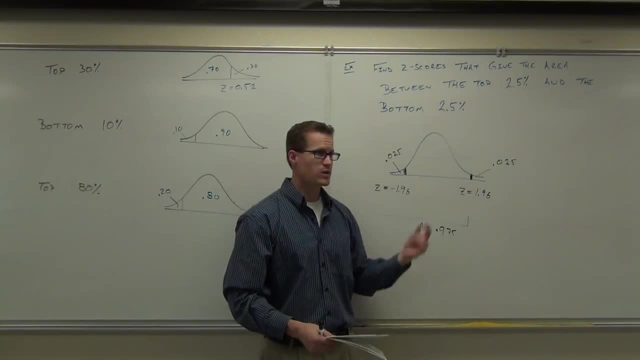 0.975.. It instantly changes. Okay, Let's put it on top. So now we're looking at the top: 0.975.. What's the last one you release? 0.975. 0.975. 0.975.. 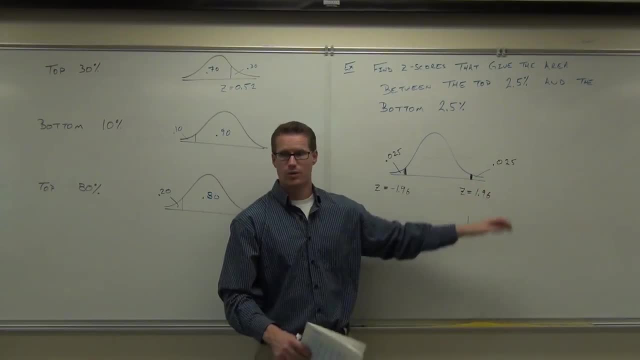 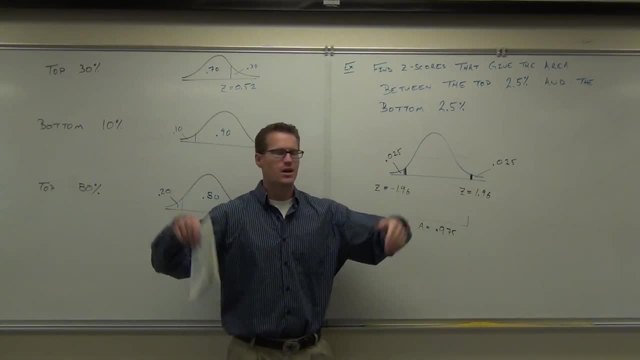 Are you still looking at the bottom? 0.975, 0.975?. No, You're still looking at the top: 0.975, 0.975. 0.975. 0.975. 0.975.. 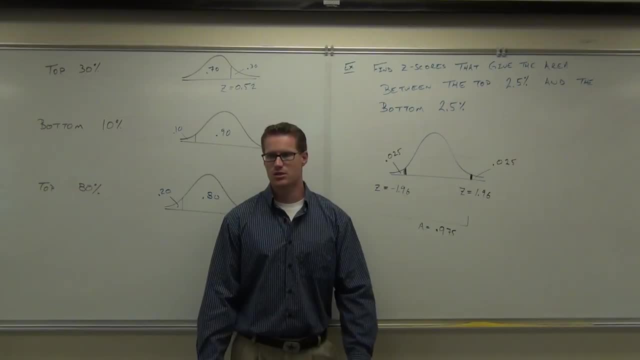 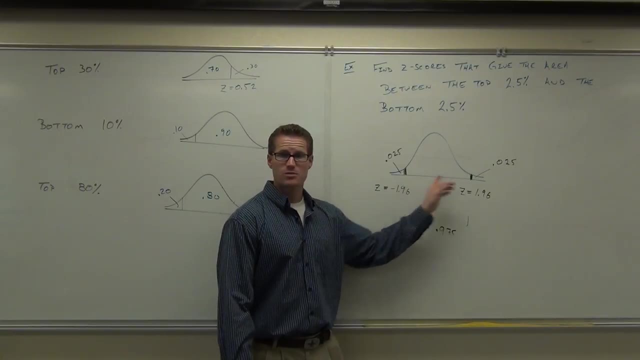 The area between the bottom 10% and the top 20%. can you do it, Or can you do it this way? No, No, you'd probably have to. you'd actually have to figure that one out. okay, But if they are symmetric and you look up, the same value, same percentage on each side, 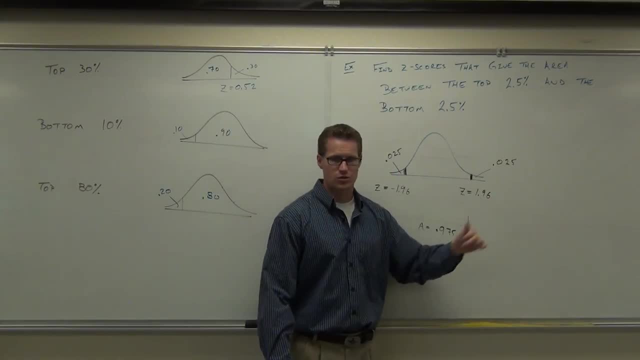 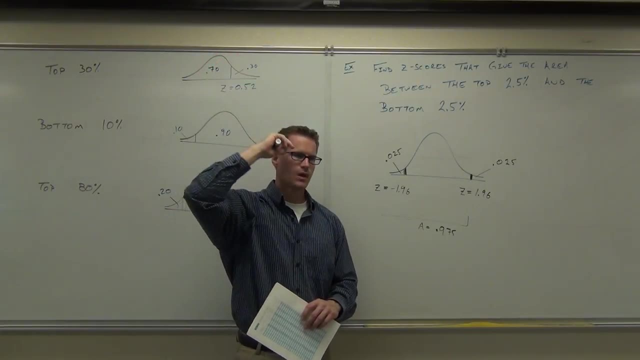 top and bottom. then, of course, you just change that sign. It is a symmetrical graph for a normal distribution. Would you guys feel okay about this? Let's do the interpretation. Do the interpretation. What's second? What's the second? 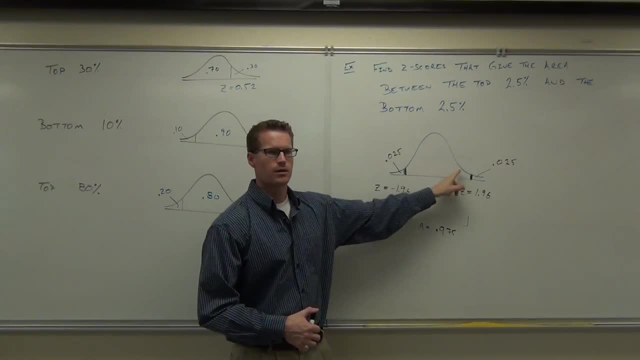 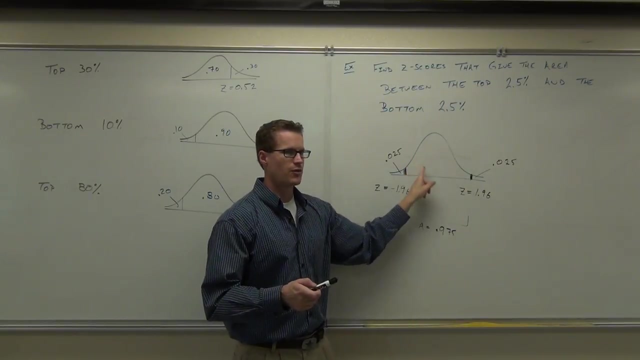 What's the percentage between your figure that out for me? Say it again: 95%. If you take one, subtract this subtract that it gives you the area between there. right, Here's what we just figured out. 95% of our thermometers will have a reading between negative 1.96 degrees. 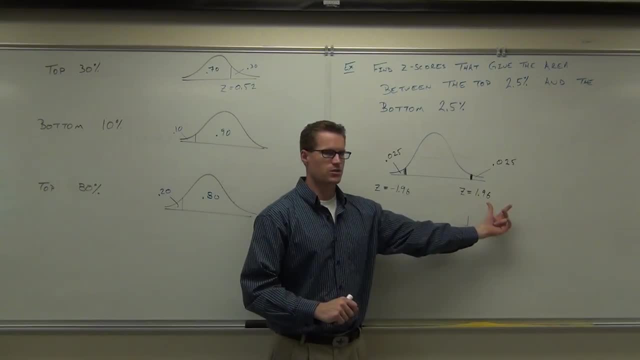 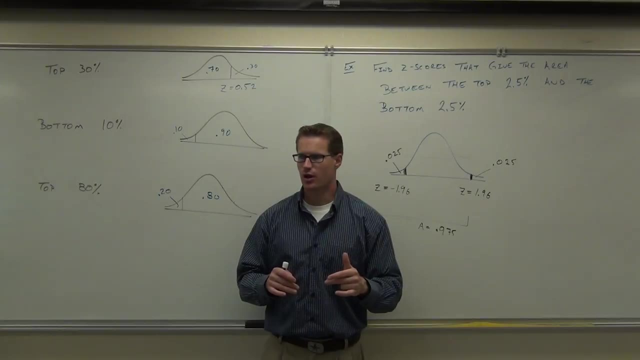 because again, the C-score is a degree for this case and 1.96.. 1.96.. 1.96 degrees. So basically negative 2 and 2 degrees. So we're saying we're 95% sure that our thermometers are going to be off by at most 2 degrees. 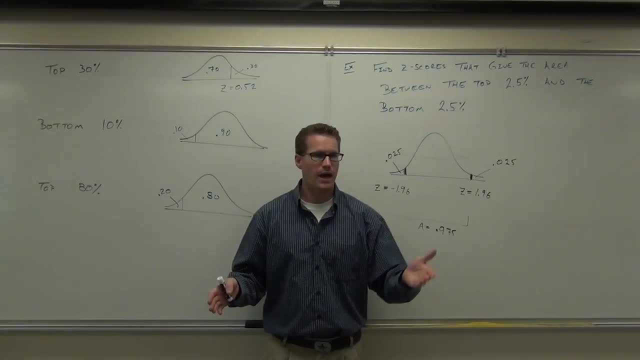 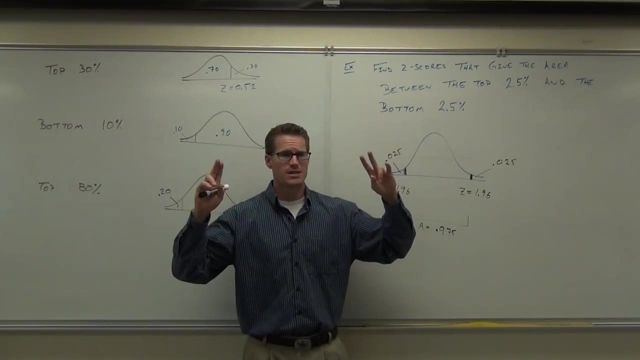 You with me From zero. That's kind of cool. You can market that. You can predict how many defective thermometers you have with that, how many defective If defective means outside of negative 2 or outside of 2, remember hey.